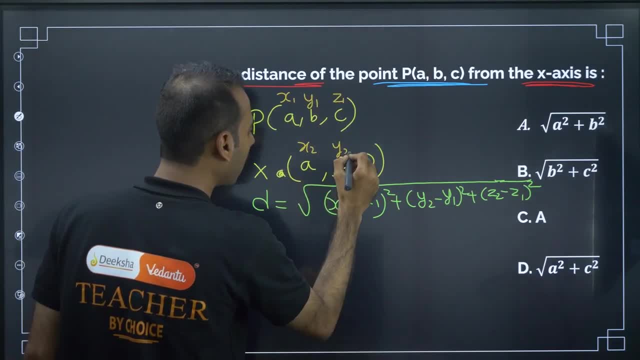 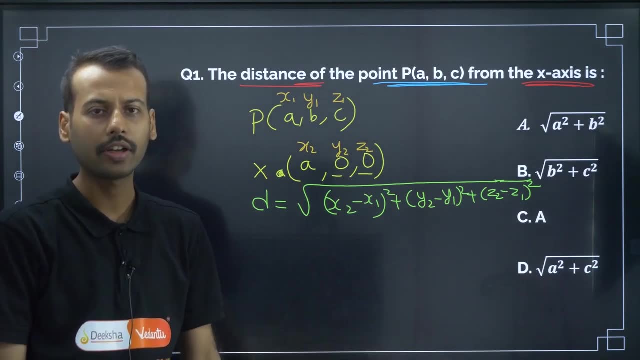 as y1, let me mark this as z2, x2, y2, z2.. This x2 minus x1 square plus y2 minus y1 square in two dimensional geometry, in 10 standard coordinate geometry. you might be already aware This is higher version. next version: x2, y2, one. 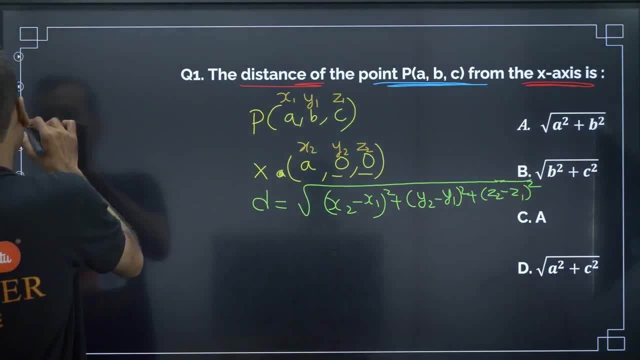 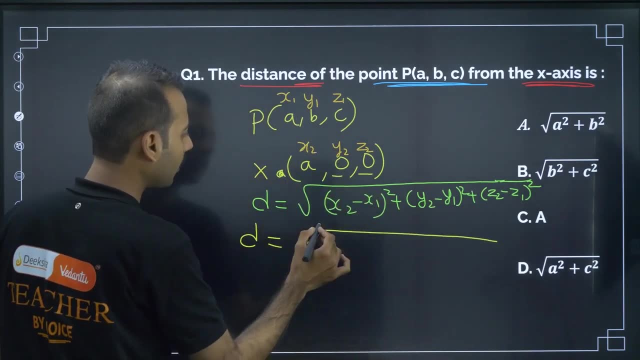 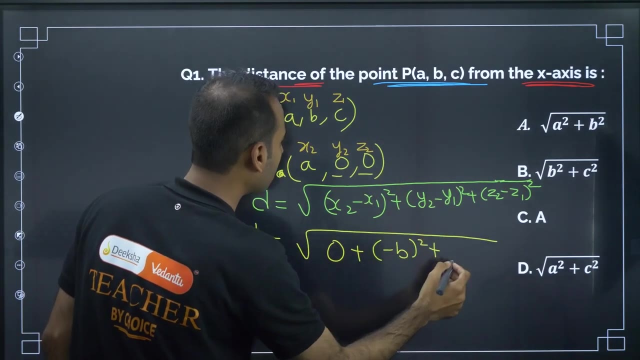 more variable we have to launch. then this becomes this: Now just use this formula and solve this. you will get the answer. Very easy question. So d is equal to root of x2 minus x1 is a minus a. 0 square plus y2 minus y1 is b square plus z2 minus z1 is c minus z1.. 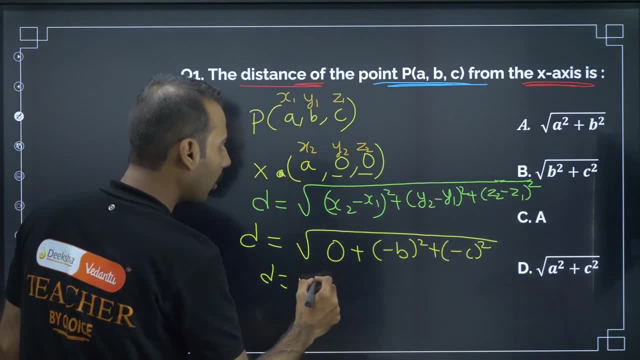 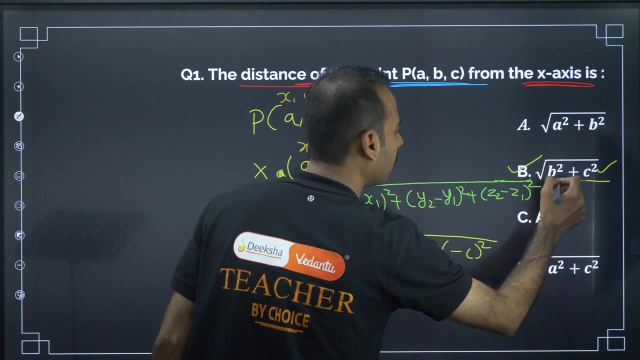 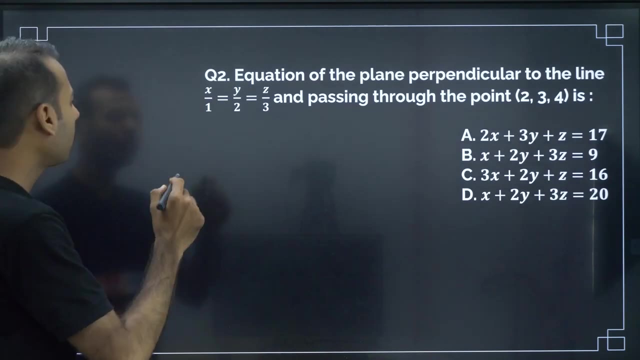 So d is equal to root of b square plus c square. Is there any such options? b square plus c square: Yes, b is the answer. b square plus c square is the answer Next, moving on to next question, The equation of plane perpendicular to the line. some information they have given. 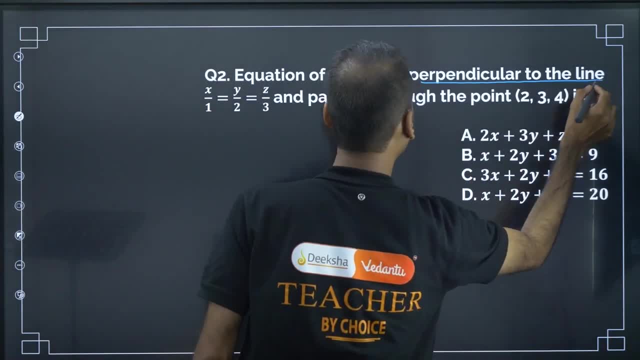 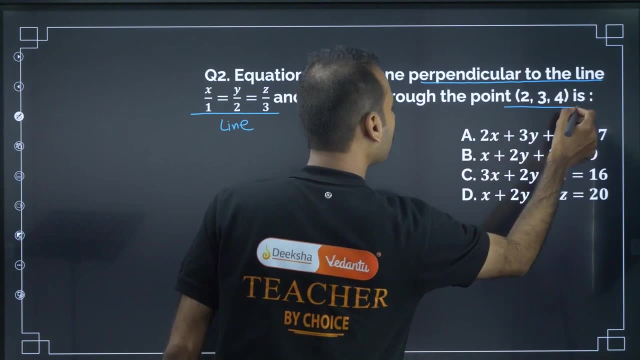 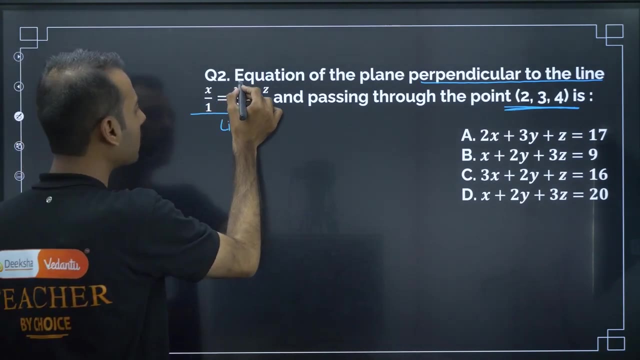 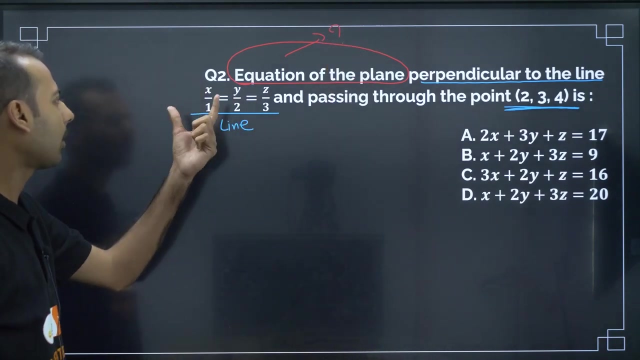 Equation of plane perpendicular to line one line they have given, This is line, they have given some line And passing through the point, passing through the point 2, 3, 4 is So some given information. what are they asking? equation of the plane, Equation of the plane perpendicular to some. 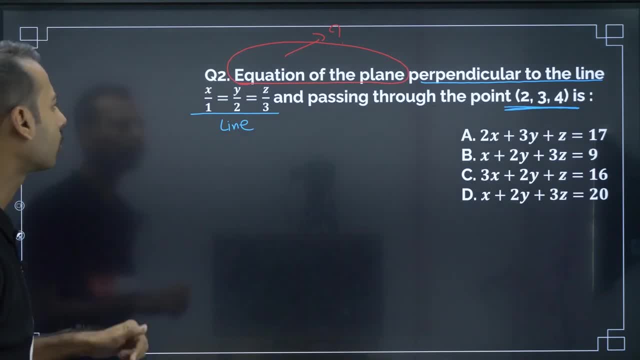 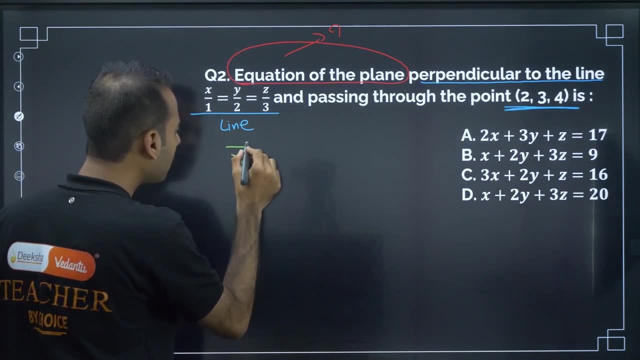 line they have given and, passing through the point, they have given one point also. So try to recall one synopsis point. Synopsis point: equation of plane. So equation of plane is given by r dot n is equal to r dot n plus r dot n minus, r dot n minus, r dot n minus. 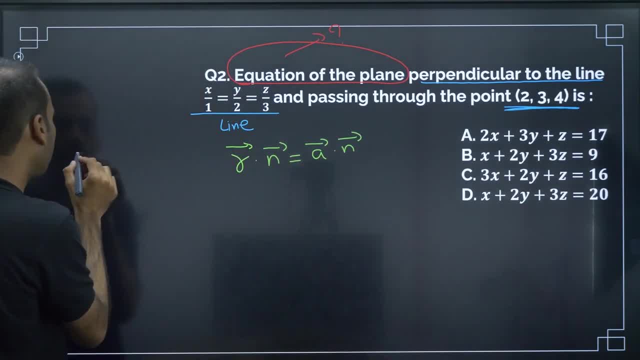 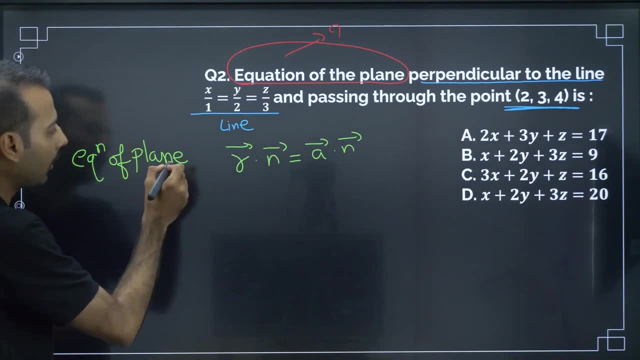 r dot Vector plan, original being equal to v. that is what is written here. That is equal to a dot n vector. equation of plane. equation of plane- Synopsis. I am writing with green pen. equation of plane will given by r vector dot. where this n vector is, n is normal. 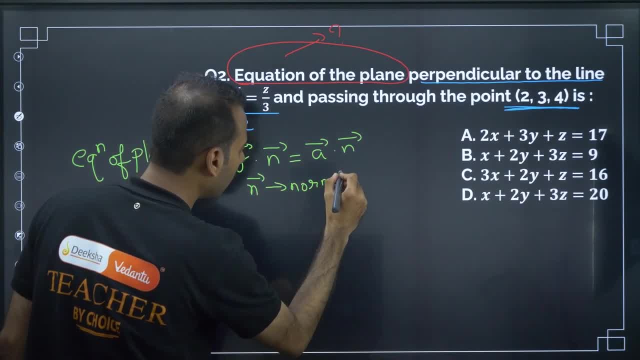 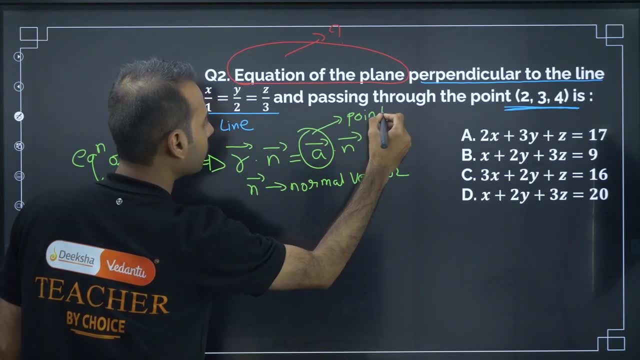 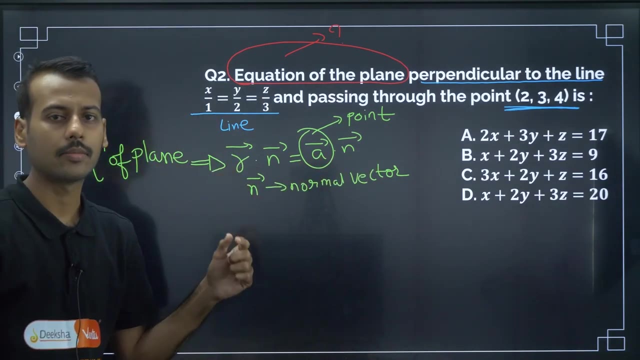 normal vector and normal vector, and this a is point, this is point. So they are interested in equation of plane, equivalent to equation of plane, And this a is going to continue on- of plane is given by where r is some arbitrary, some arbitrary vector: x y z, x i cap y z. so if 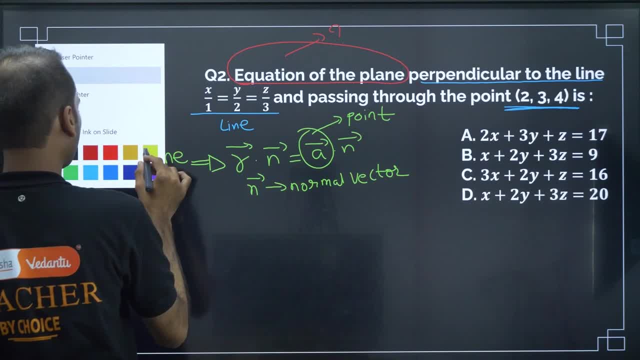 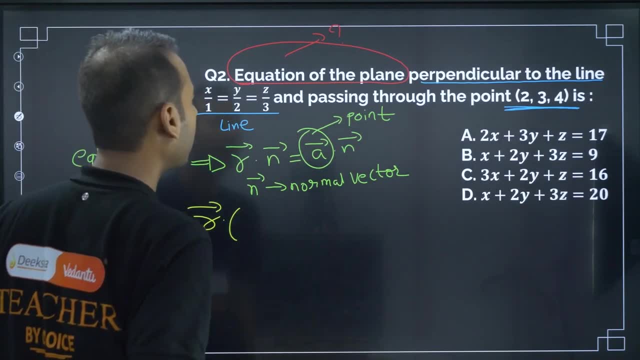 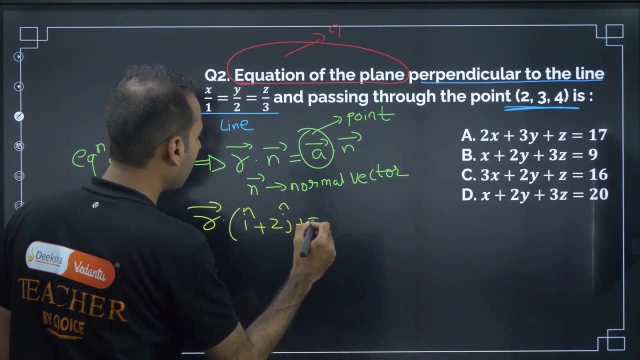 you open the book and if you see theorem, you will be able to relate this question with the theorem. so let me write this like this: r vector. let me write n vector. what is n vector? n perpendicular to the line that means they are talking about this. this is i cap plus 2 j cap plus 3 k cap. 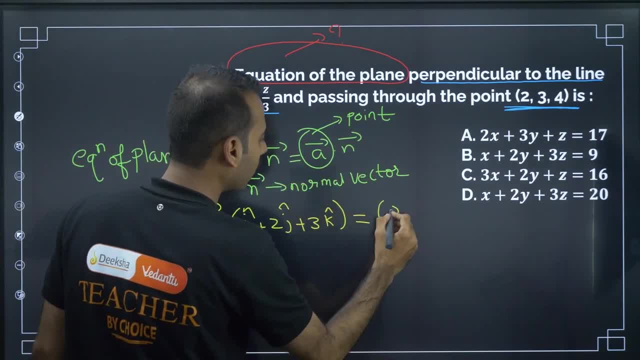 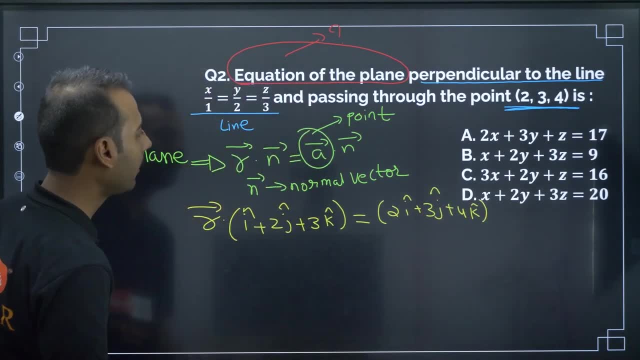 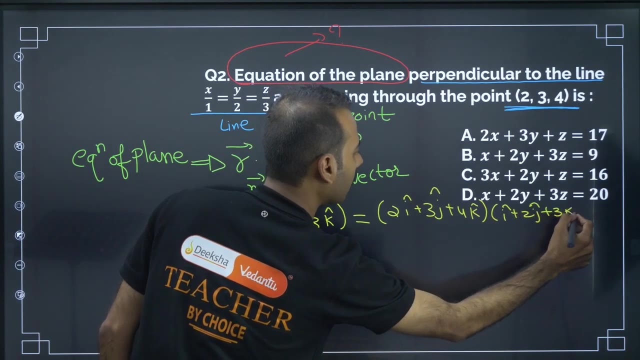 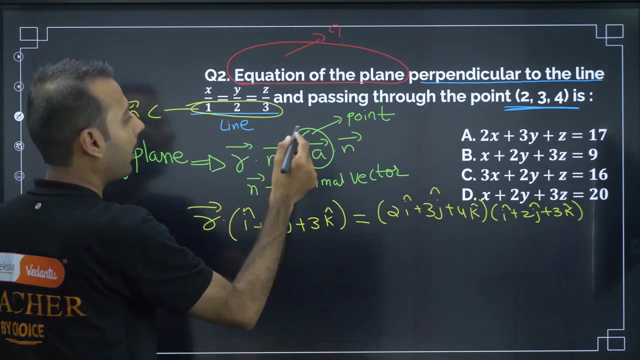 direction we got a point. point is 2, 3, 4, 2, 3, 4, 2, 3, 4 and then n vector. n vector is again same: i cap plus 2, j cap plus 3 k cap, 3 k cap. so generally this: this is for n vector and this: 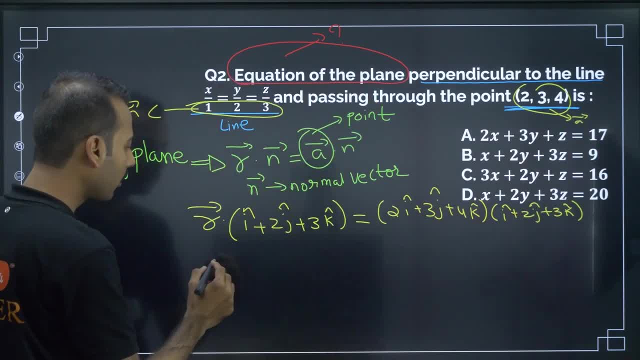 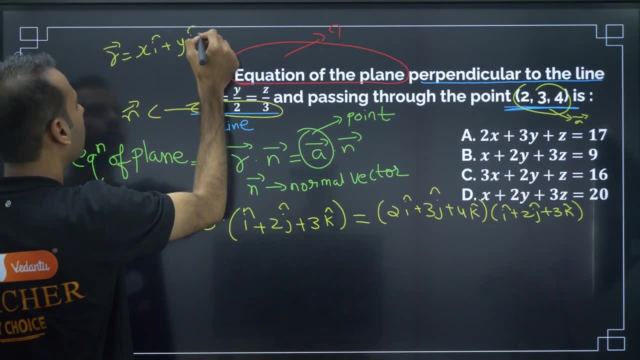 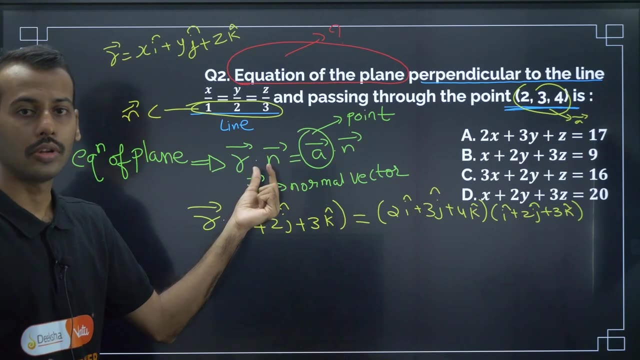 point is for a vector. so the story goes like this: r vector is what is r vector? r vector is x i cap plus y j cap plus z k cap. you open synopsis related to this in a crt book and you try to read that theorem. you add that to memory and solve some. 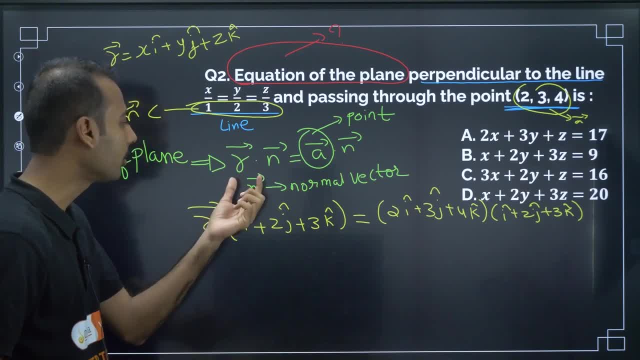 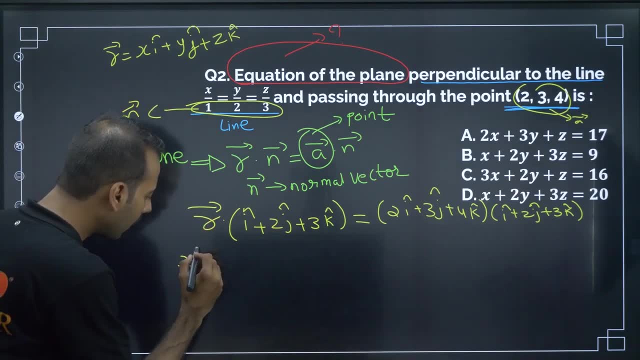 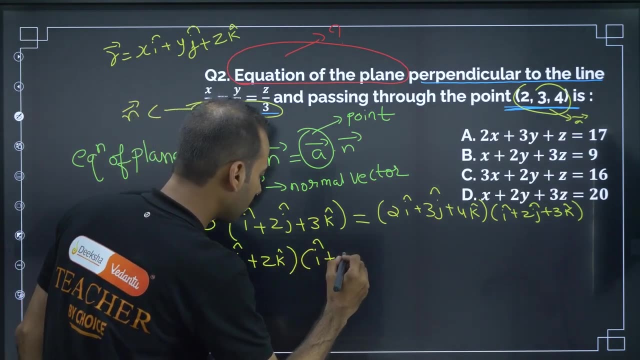 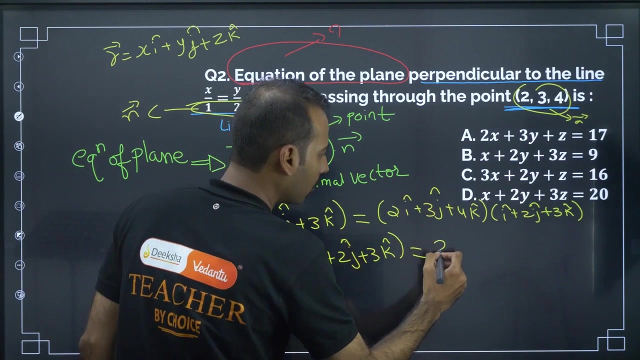 problems, if you are. if you want much detailed explanation about this, just add some comment to this video. i will help you there. so r vector x: i cap, x i cap plus y j cap, plus z k cap, and then i cap plus 2 j cap plus 3 k cap is equal to. now you go for multiplying 2 plus. 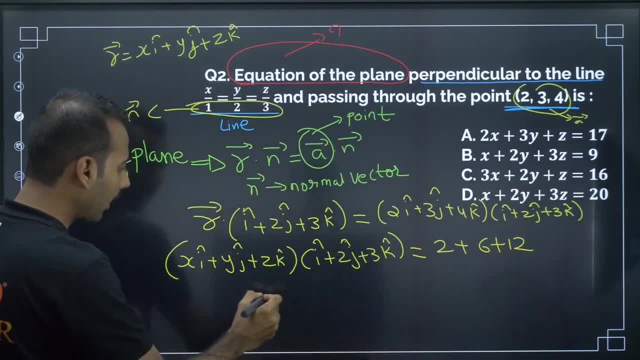 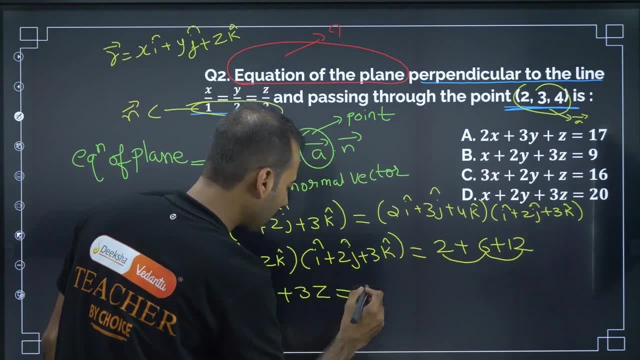 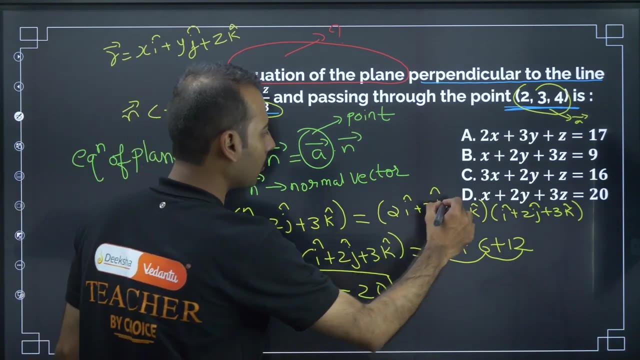 3 to the 6, 4, 3 is a 2 l. next, x, x plus 2 y plus 3 z is equal to 2 plus 6 8, 20. so is there any such option? x plus 2 y plus 3 z is equal to 20, plus 3 z is equal to 20. d is the answer. 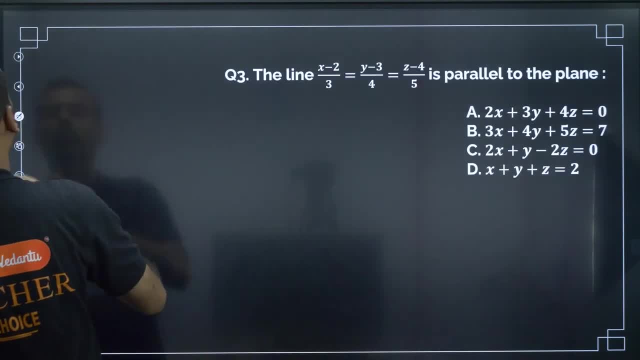 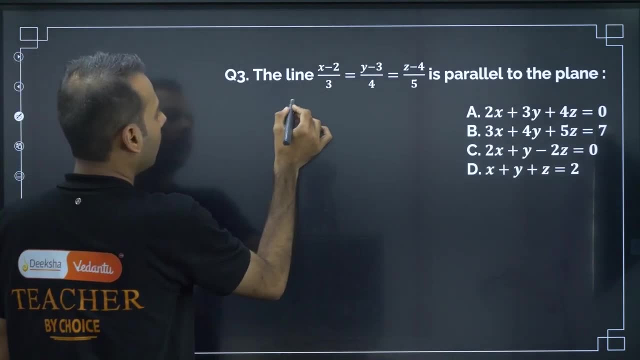 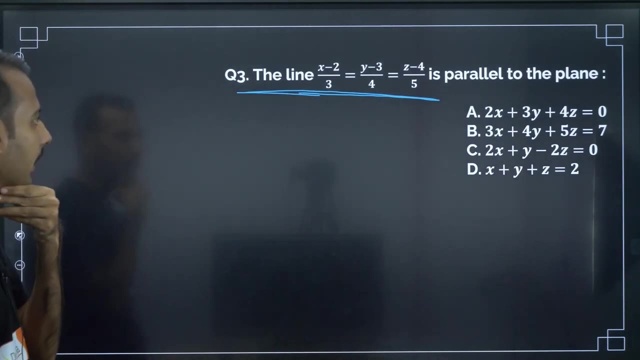 d is equal to 25.. the answer, moving on to next question. moving on to next question, the line is parallel to the plane. they have given one line. they have given one line is parallel to the plane. is parallel to which plane? is parallel to which plane? 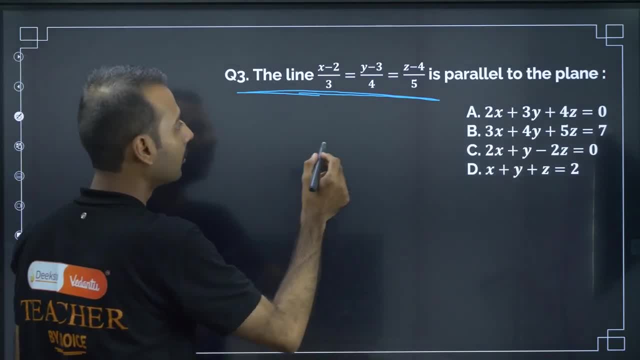 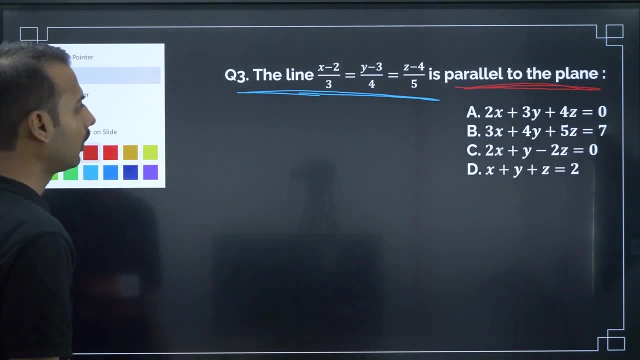 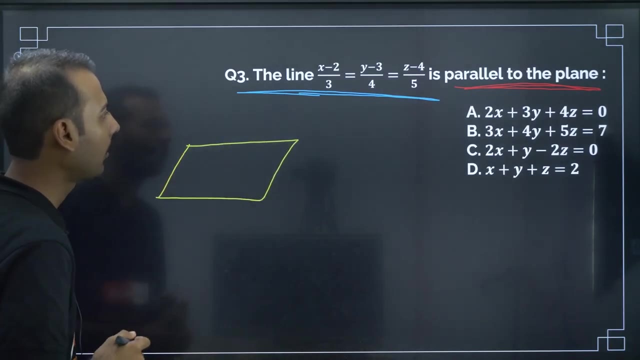 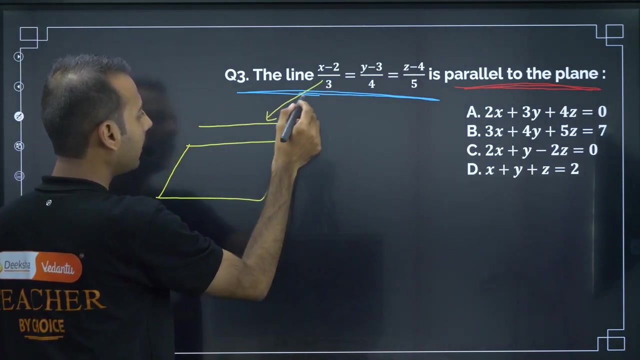 So for this, parallel to parallel to the plane, now, direction ratios of this line are and the line is parallel to plane. they have drawn one plane. what is that plane, we don't know- is parallel, the line, this line, this line is this and it has 3, 4, 5 as direction ratios. 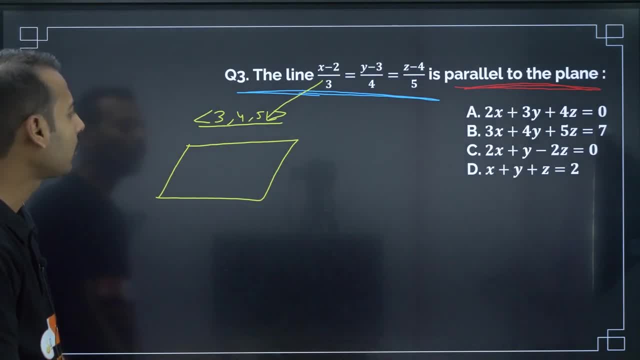 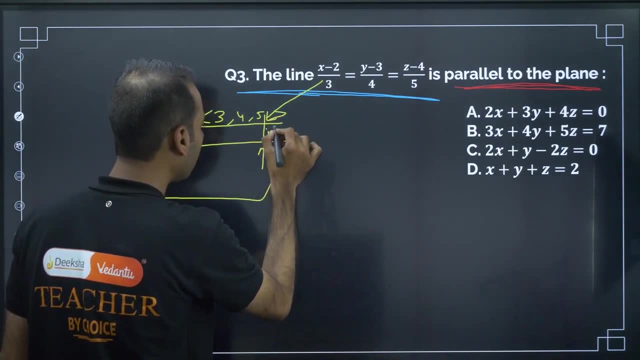 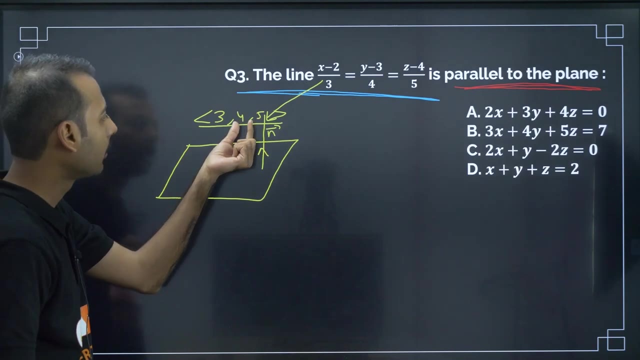 3, 4, 5 are the direction ratios- is parallel to the plane. now there is one plane, So it is very obvious that it will have one normal vector also. it will have one normal vector. now, what is that plane? so if I 3, 4, 5, now this is one vector, this is one vector. 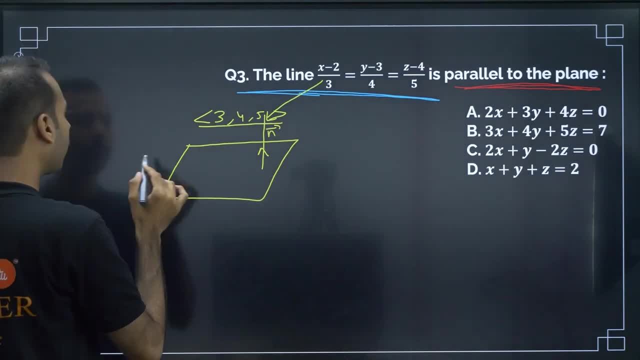 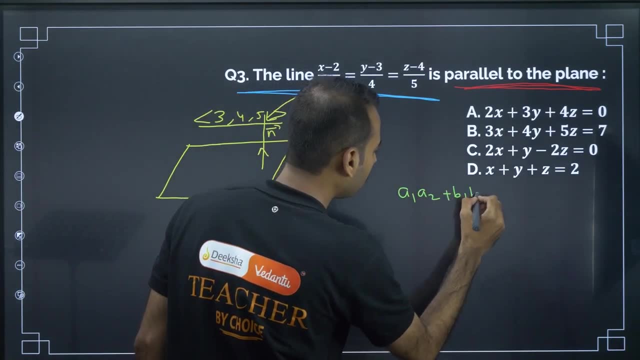 3, 4, 5 is direction ratios for this. now try to recall the condition for two vectors to be perpendicular. so for that A1, A2 plus B1, B2 plus C1, C2 equal to 0, then we will get 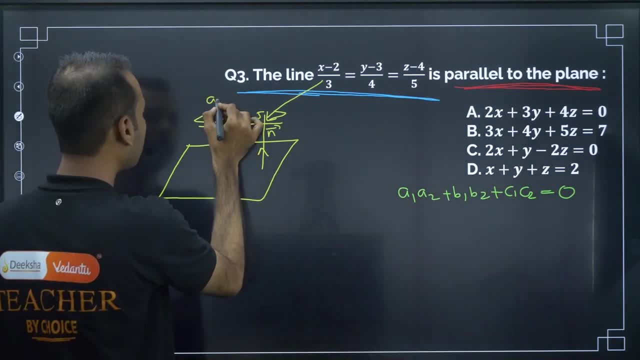 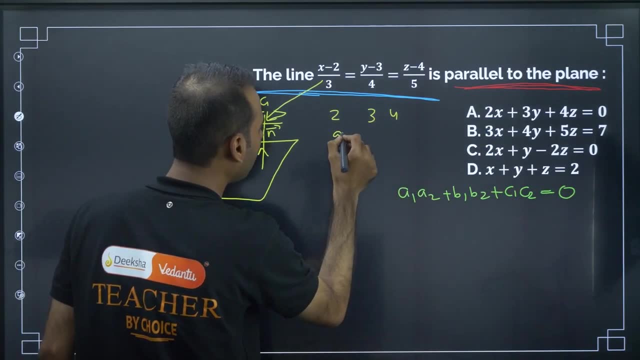 if that condition is satisfied, then that will be So. if I mark this as A1, B2.. C1, B2 equal to 0.. 1, c, 1. if i take first option, 2, 3, 4, 2, 3, 4, 2, 3, 4 as a, 2, b, 2, c, 2. if i go for a 1, a, 2, 3, 2's are 6. 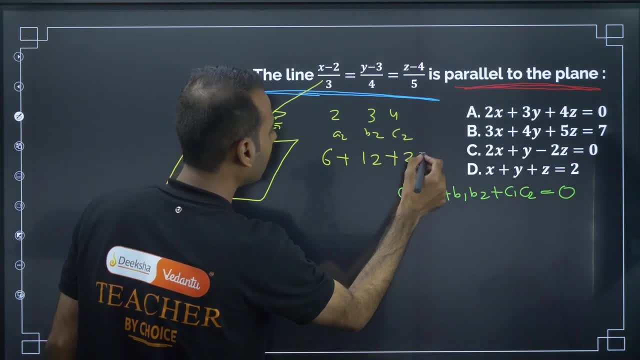 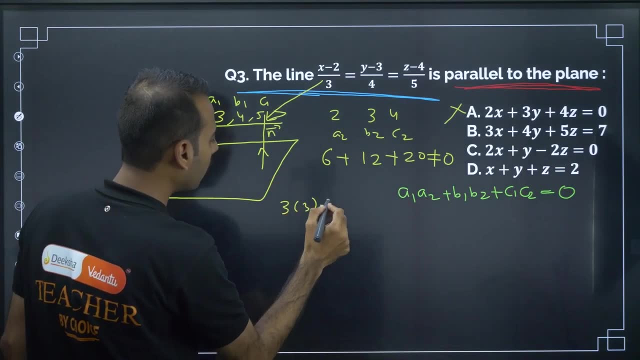 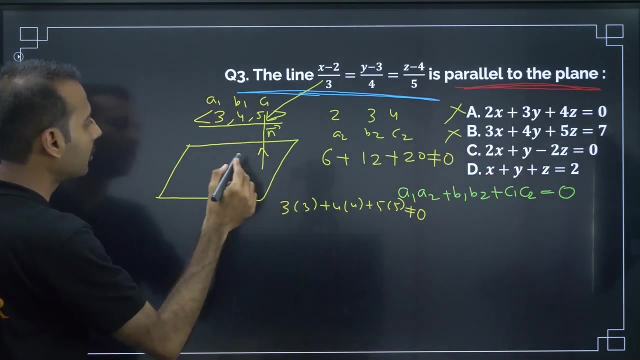 plus b, 1 b, 2 plus c, 1, c, 2, 4, 5's are 20. this is not equal to 0, so first option is eliminated. next, if i go for 3, 4, 5: 3, 3, 4, 4, 4, 4 plus 5, 5: not equal to 0, so second option is also eliminated. next, 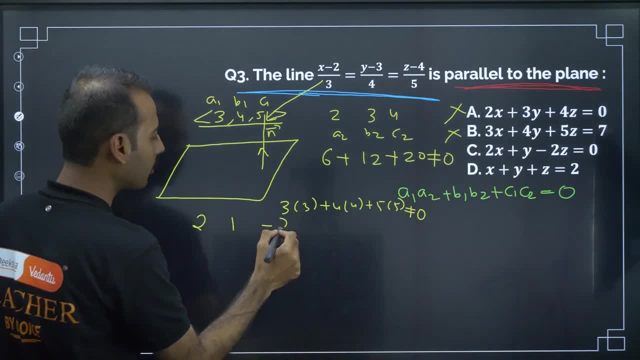 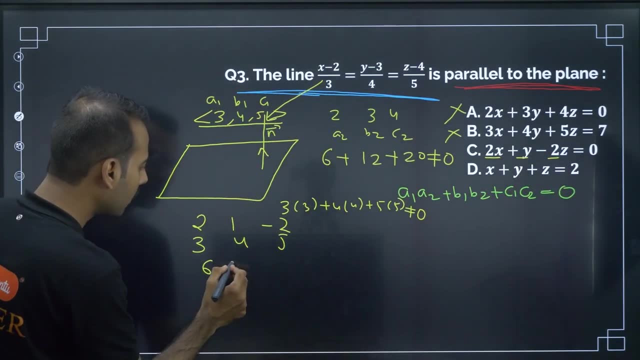 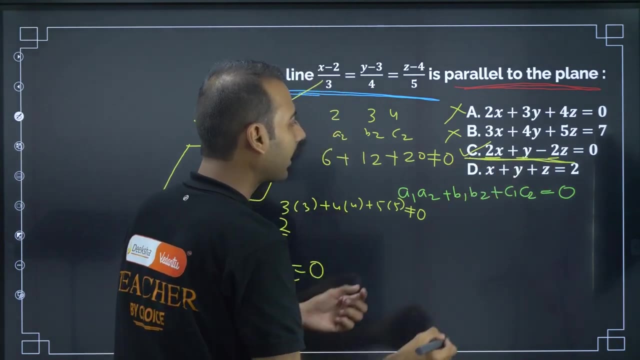 2, 1, 2, 1 minus 2. if i take this- 2, 1 minus 2- and if i go for multiplying this, 3, 4, 5, 2, 3's are 6 plus 4 minus 10 is equal to 0. so this plane, this plane, if i take direction, ratios of this plane. 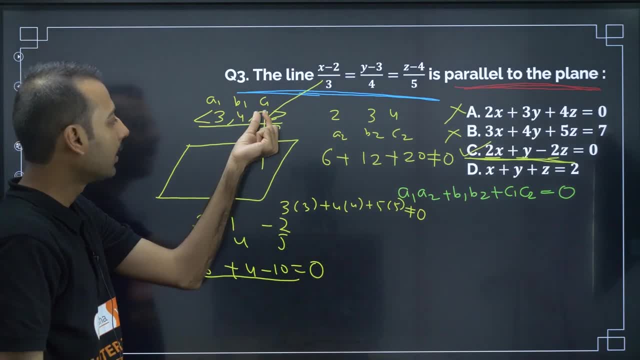 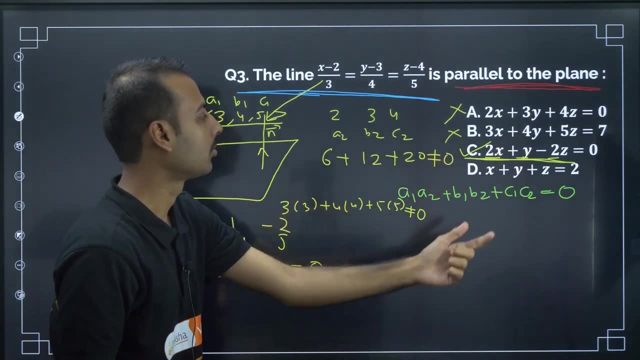 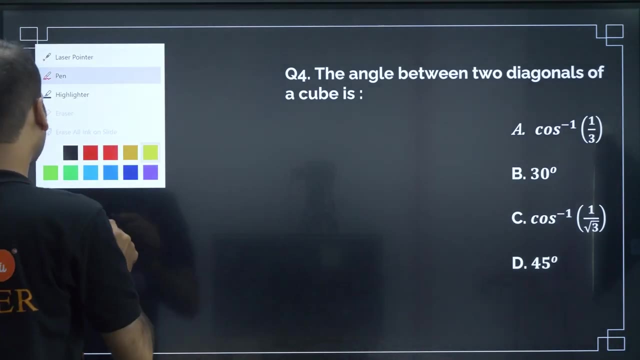 and if i direction ratios of plane means, that is, the direction ratios of this normal vector, this, these are the direction ratios of this. so if i am multiplying i am getting 2, that's 1. 2 is equal to 0. moving on to next question, the angle between diagonals of a cube is so the 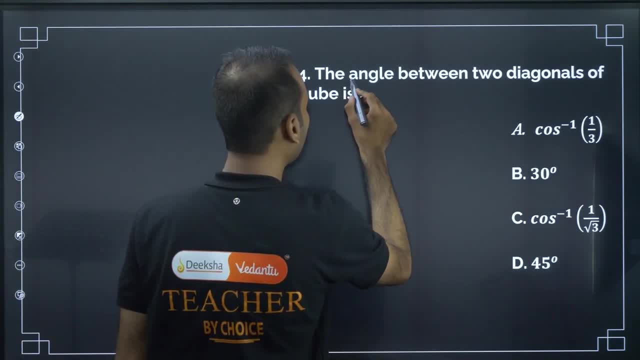 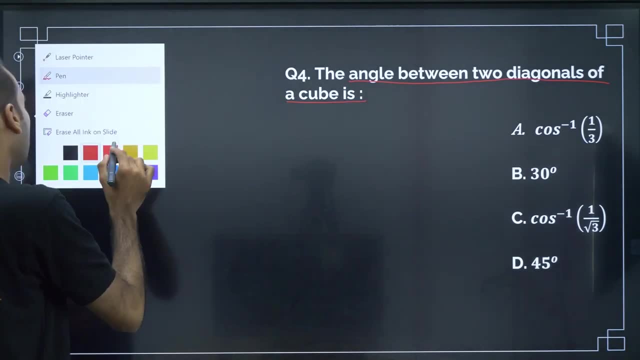 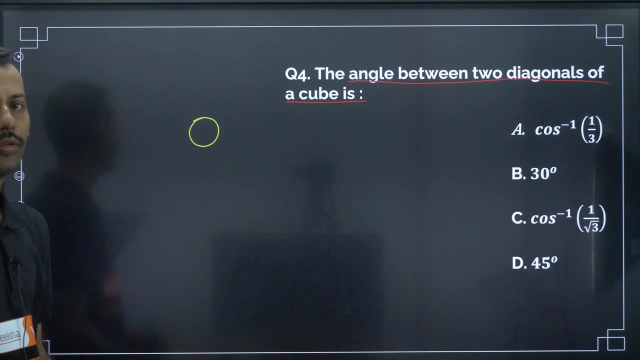 question is: angle between, angle between two diagonals of a cube? is angle between two diagonals of a cube is so some things we should be knowing. let me consider one cube. it will have many vertices. so if i consider one vertex as o, o, i will mark this as. 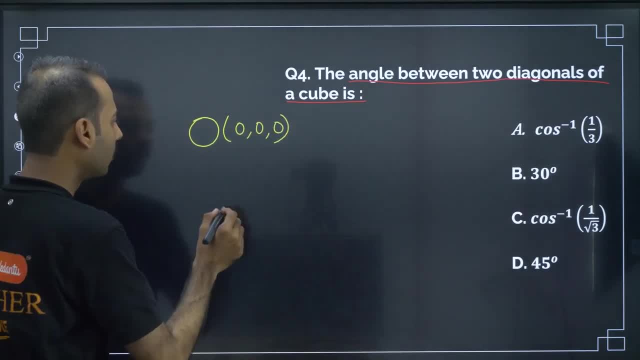 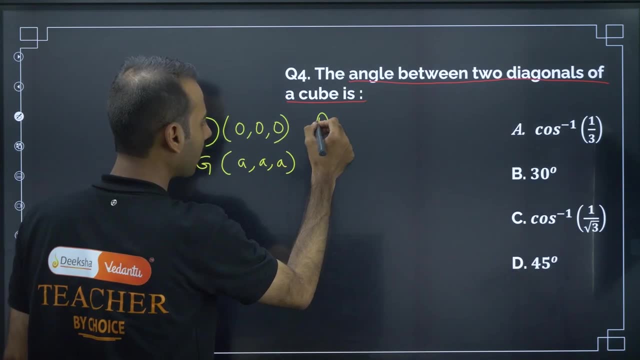 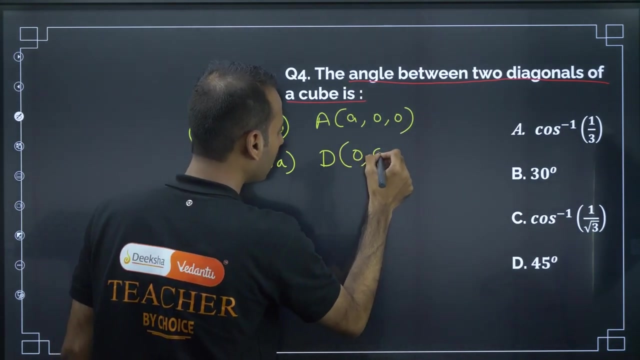 0, 0, 0 o. i am marking this as 0, 0. let me consider one more vertex g as a comma a, comma a. let me consider one more vertex. let me consider few more vertex a, 0, 0 and 0 a a. now, now, what are we supposed? 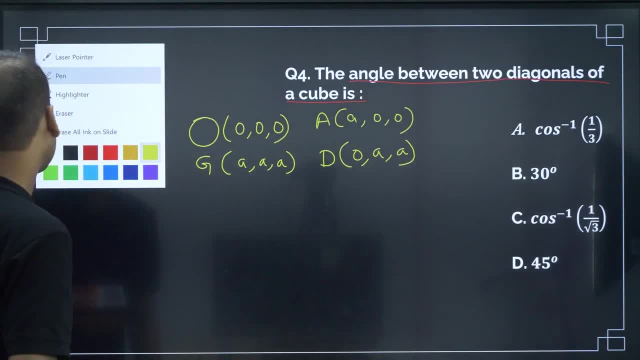 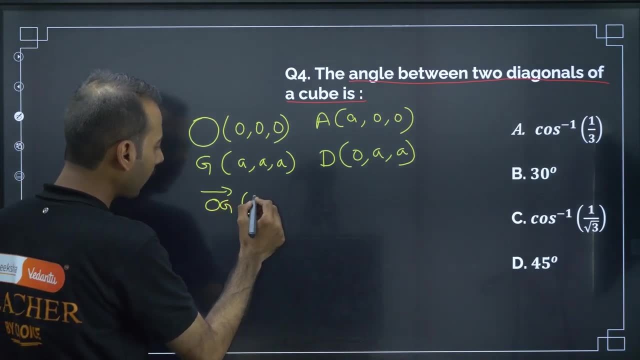 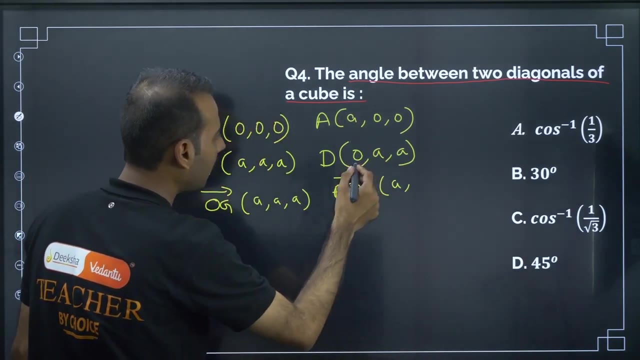 to do. the angle between two diagonals of a cube is. So let me find O G vector. if I am talking about O G, O G is one diagonal. So for O G vector we will get a comma, a comma a, and for a d vector and for a d vector, a a d. 0 minus a is minus a a a. Now they are. 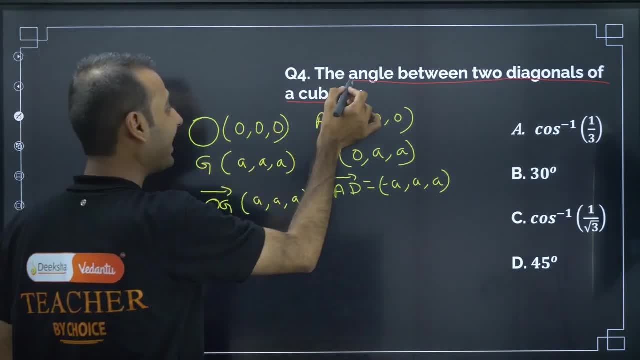 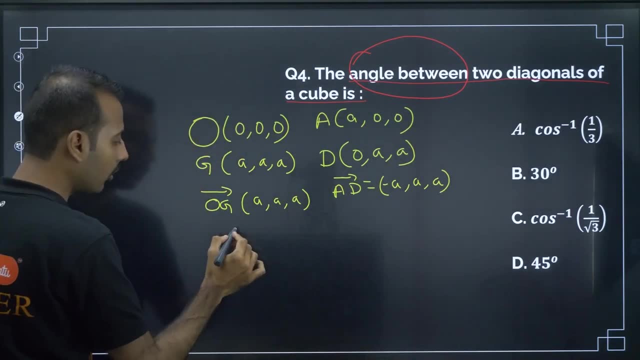 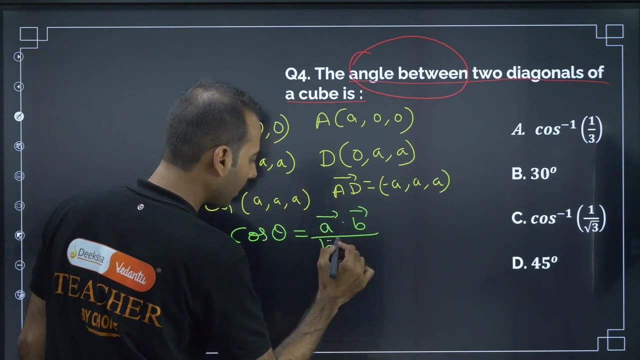 talking about angle between. what are they talking? they are interested in angle between, angle between. they want angle. So whenever we want angle generally, one formula we know: cos theta is equal to cos theta is equal to a dot b by magnitude of a, magnitude of b. 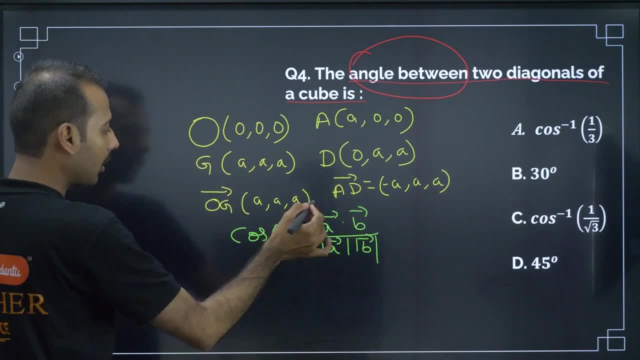 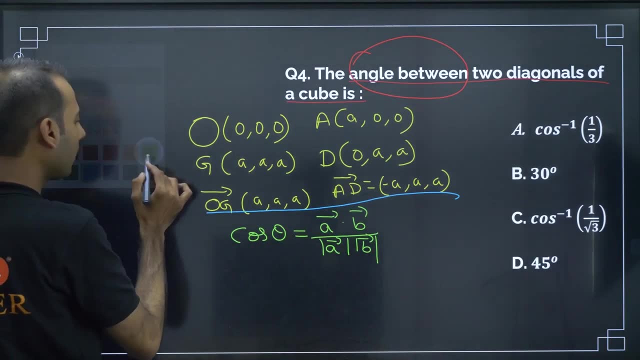 Now two vectors. we know two diagonals, we know these are two diagonals. So with the help of these two diagonals and using this formula, we can find. we can find a, a dot, b a, O G. this can be written as O G. 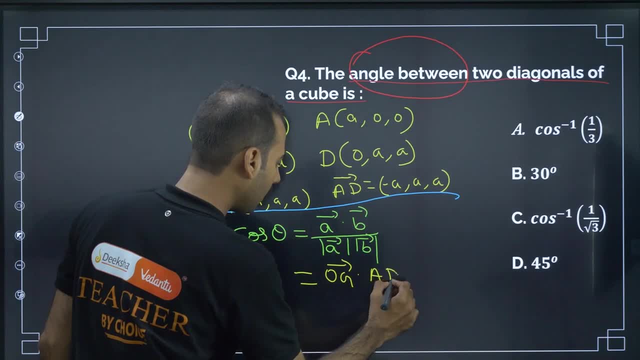 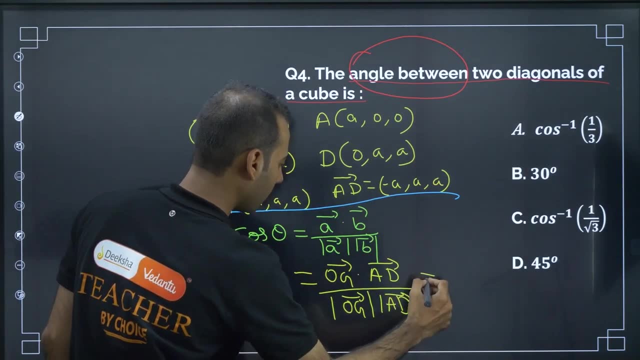 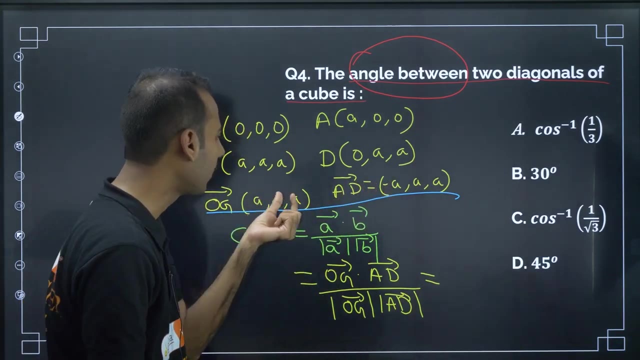 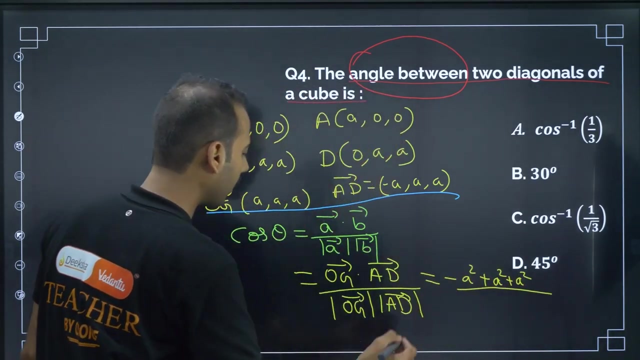 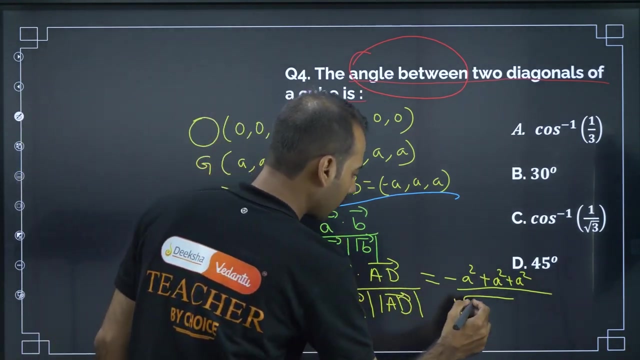 For O G, vector: O G, dot a d. if I multiply this and this, I will get minus a square plus a square plus a square divided by O G. For O G, if I take magnitude of O G, root of root, a square plus a square plus a square, 3 a square. and then this: a d a d, 3 a square, 3 a square. 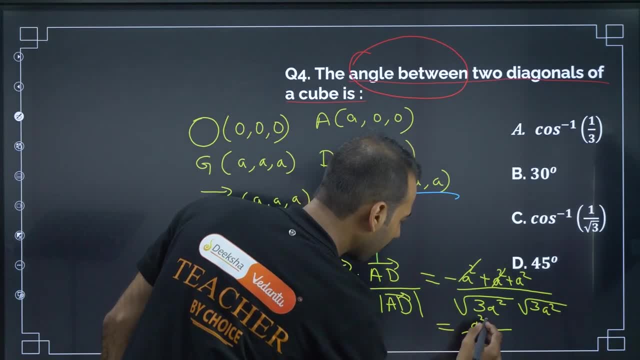 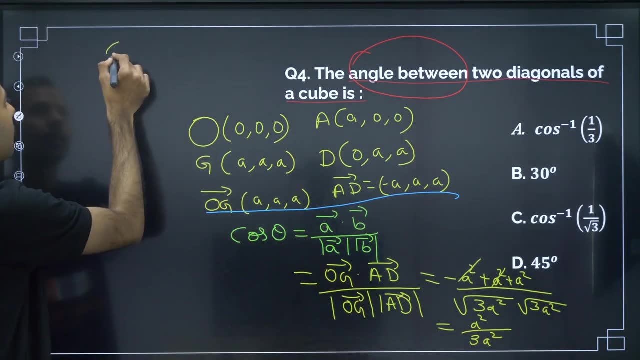 so this and this will get cancelled: a square divided by 3: a square, 3 a square. So which implies from here- I am writing here, since space is not there- cos theta is equal to cos theta is equal to 1 by 3, which implies, which implies theta is equal to cos inverse. 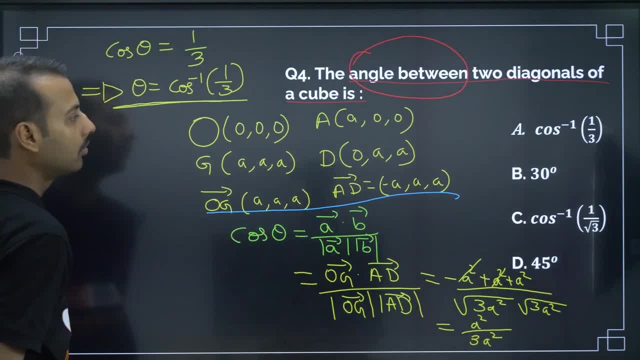 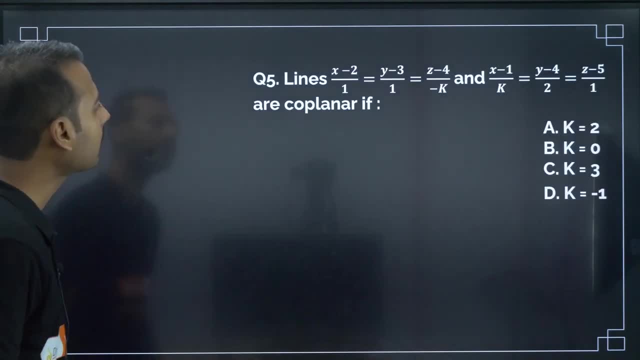 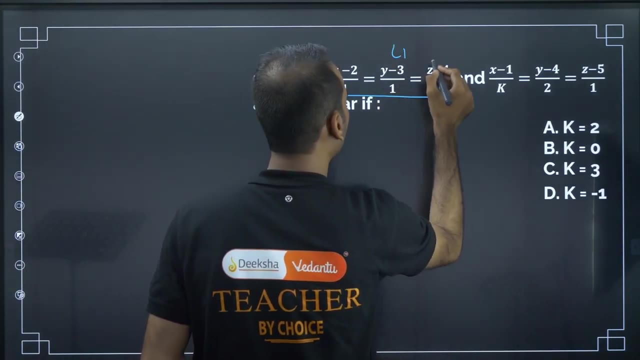 of 1 by 3. is there any such option? cos is the answer? Moving on to next question. is the answer moving on to next question? Lines x minus 2 by 1 and are coplanar if they have given two lines, line 1 and line 2, two. 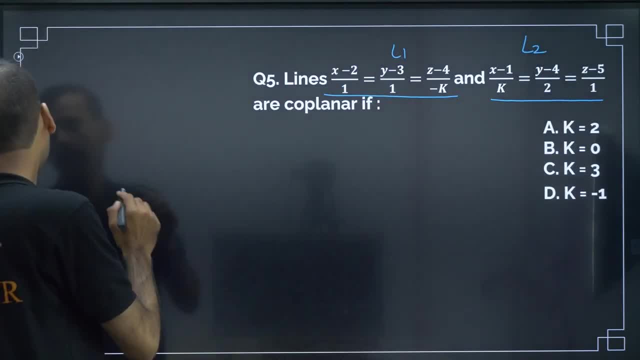 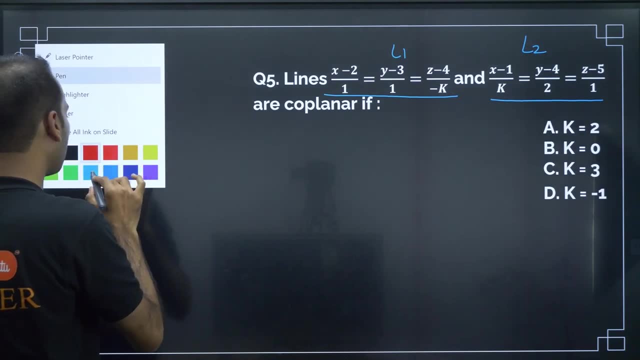 lines are given, They are coplanar. they are what coplanar? what are? they are coplanar, they are coplanar. they have only given us this. also, they are coplanar. line 1 and line 2 are coplanar if 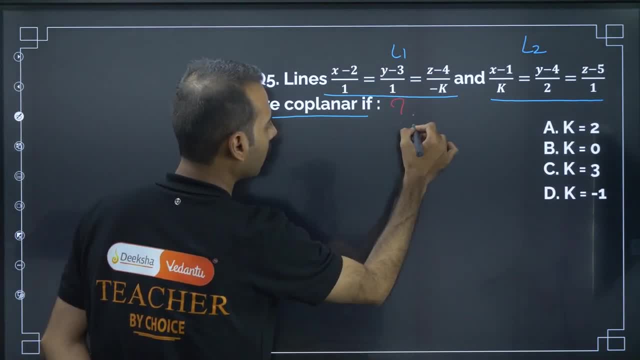 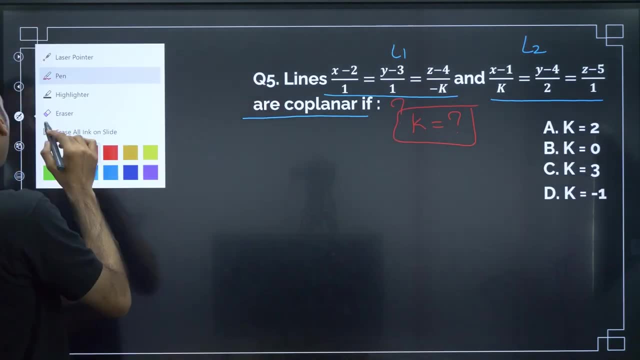 so what is the question? if some k values they have given, so they are interested, they are asking us to find k value. if you find k value, then that will be considered. Now try to recall the condition for coplanarity. two lines are coplanar. 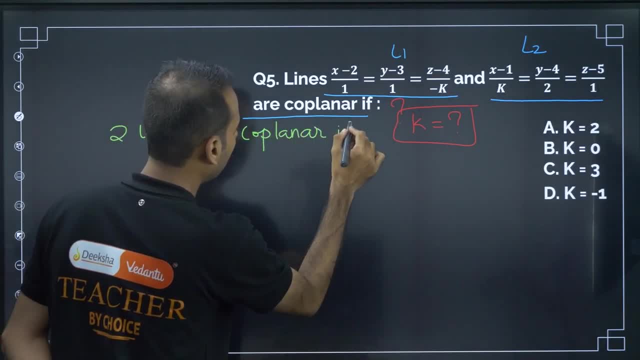 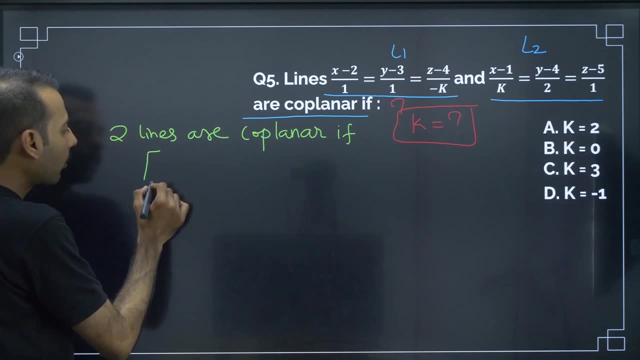 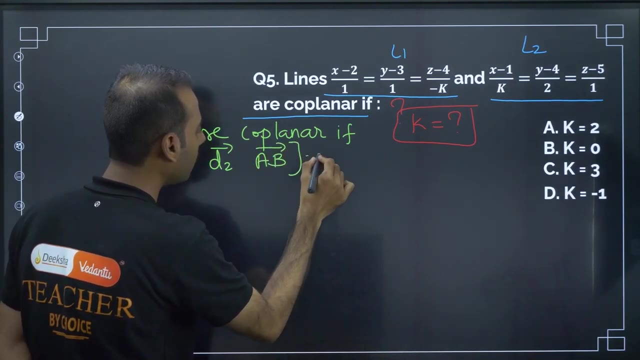 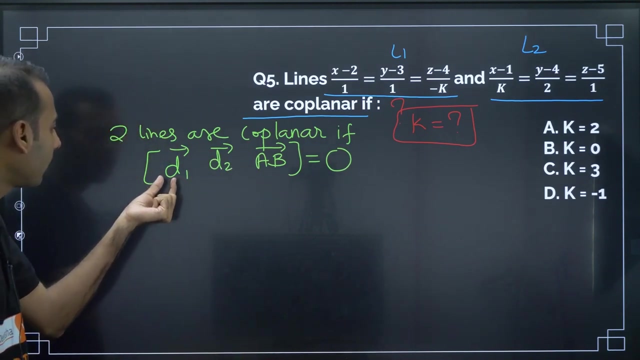 If two lines are coplanar. if scalar triple product of direction ratios of first one, second one and a b direction ratio of a- b is equal to 0, two lines are coplanar. that means two lines are lying in same plane. if direction ratios of first line, second line and a b is 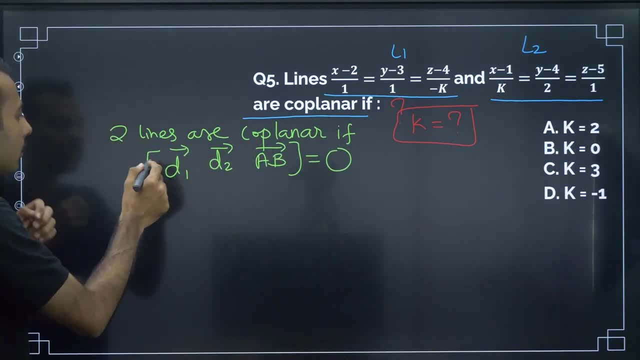 equal to 0.. What is this? I will tell, but this synopsis you should be knowing: scalar triple product of this is 0.. Now, if I go to, lines are coplanar if: if this is the case, so lines are coplanar if 1, 1 minus. 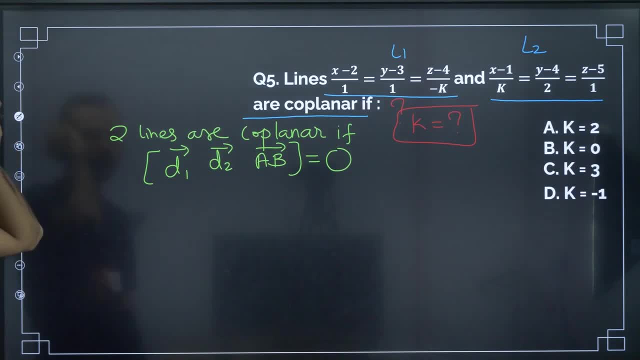 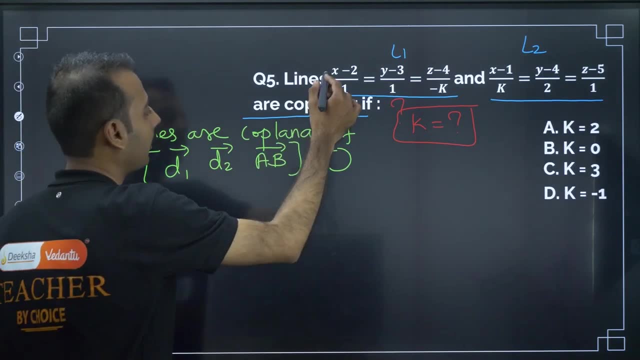 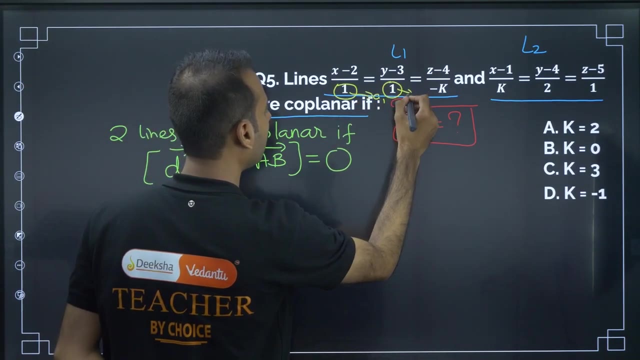 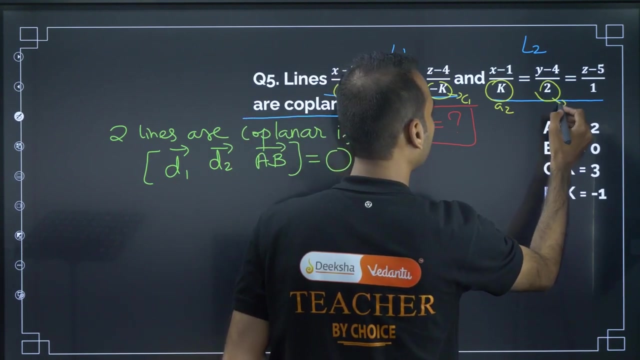 k, k, 2, 1. two lines are coplanar if d 1, d, 2, a b is 0. now try to recall whenever the lines. generally We call this as a 1, b, 1, c, 1 a, 2, a, 2, b 2 and c 2. these are direction ratios and this x. 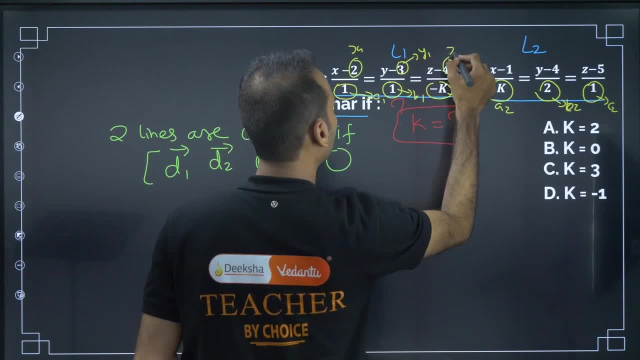 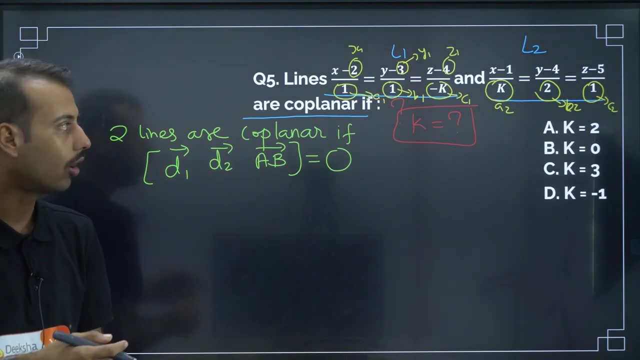 1 y 1 z 1 for this how I am writing, why I am writing a 1, b 1, c 1. so you should be. you should practice all the theorems. Theorems are very important, So you should be. you should practice all the theorems. 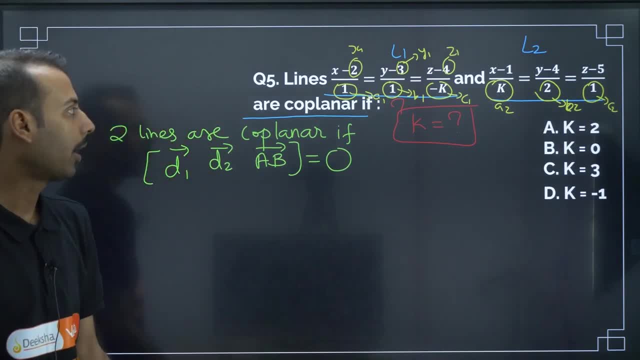 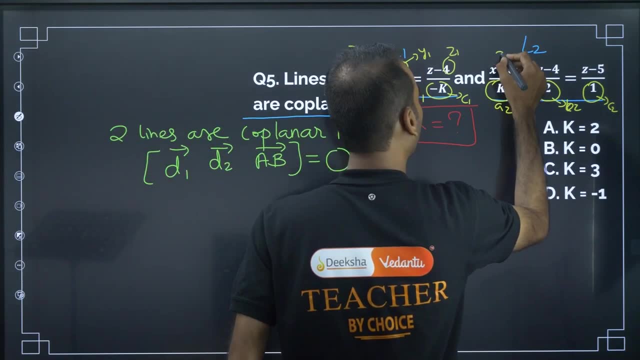 All the theorems you should add in your mind, and also you should be able to recall it is based on which concept. so then only you will be able to solve. So that's why generally, theorems are studied, so that whenever any problem comes, you will. 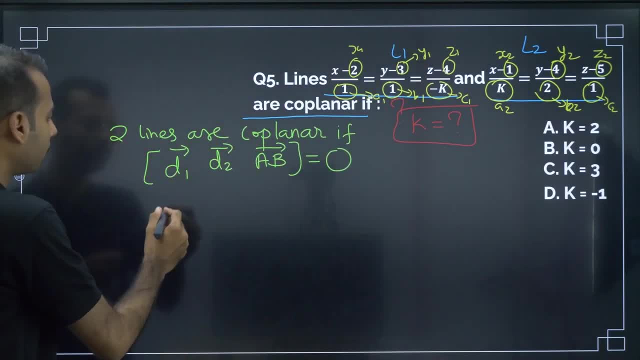 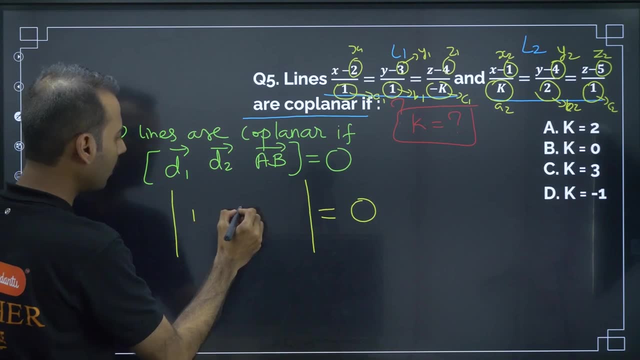 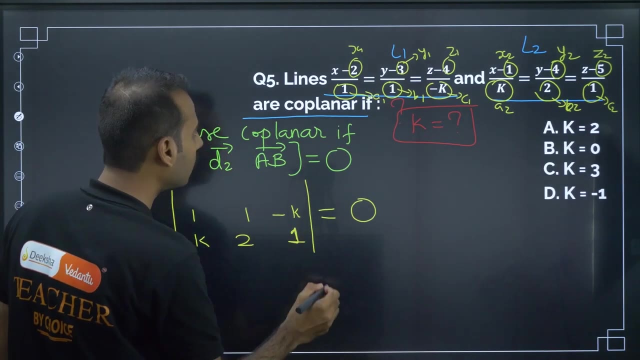 be able to relate or coplanar. if now the condition is like this: 0 direction ratios of first one, if I write 1, 1 minus k, And direction ratios of second, k, 2, 1, k 2, 1. also a b or a b, a b is equal to x, 2 minus. 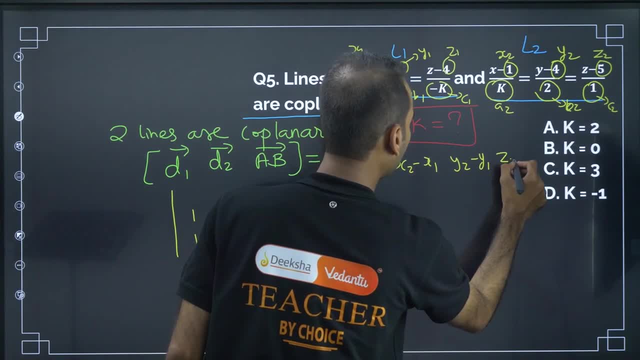 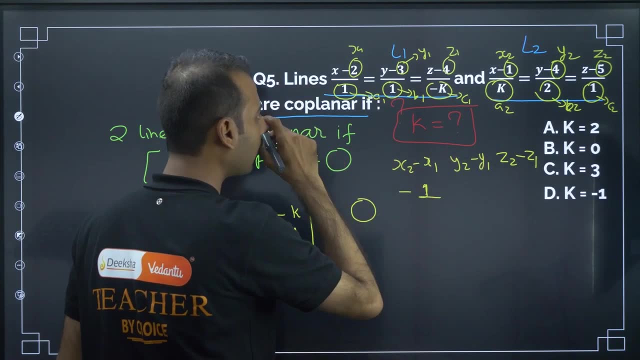 x 1 y 2 minus y 1. z. 2 minus z 1. x. 2 minus x. 1 is 1 minus 2 is minus 1 y 2 minus y. 1. 4 minus 3 is 1 z. 2 minus z. 1. 5 minus 4 is 1.. 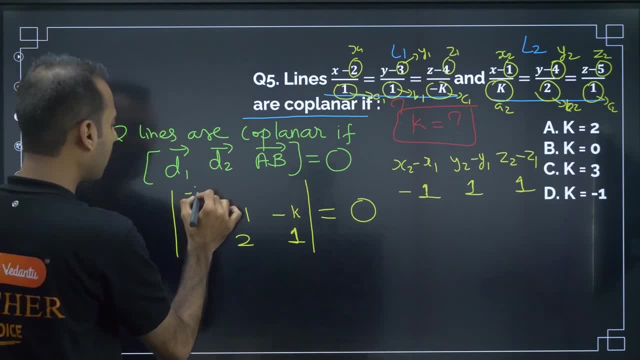 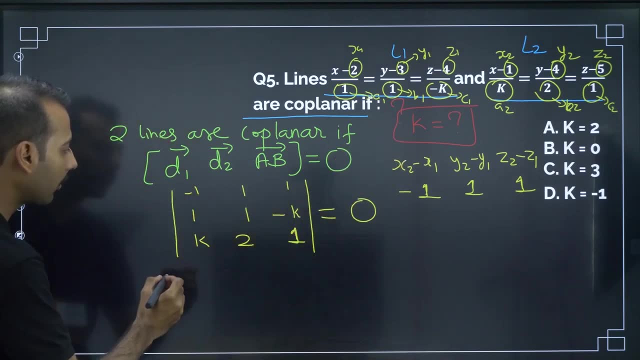 So Now we have to place a b in place of a, b minus 1, 1, 1.. Now we have to solve this determinant. we have to solve this determinant and then, whatever is the value of that will be the answer: minus 1, 1 plus 2, k minus 1. minus 1, 1 plus k- square. 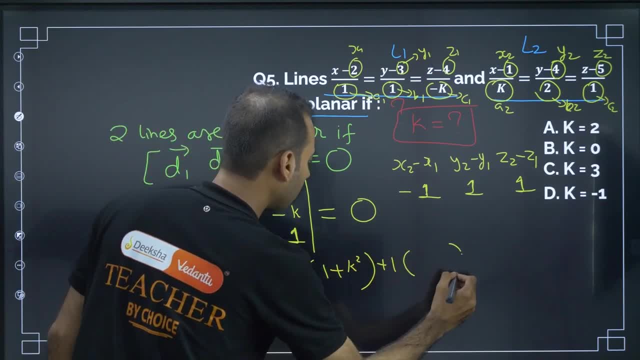 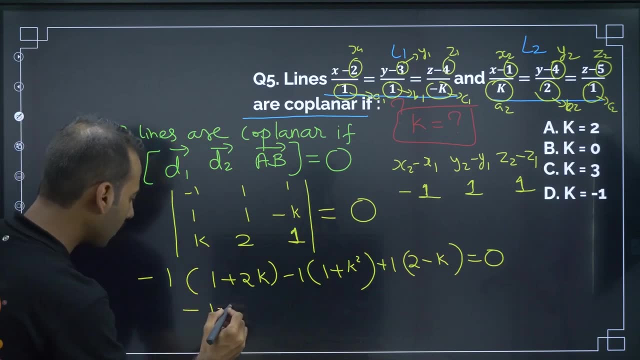 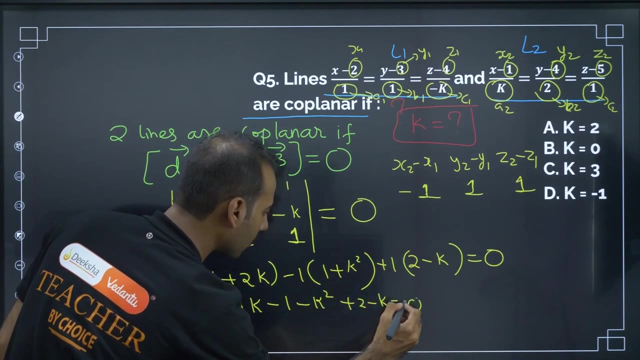 1 plus k, square plus 1 plus 1, and then 2 minus k. 2 minus k is equal to 0.. So So, minus 1 minus 2 k, minus 1 minus k, square plus 2 minus k is equal to 0, if I simplify. 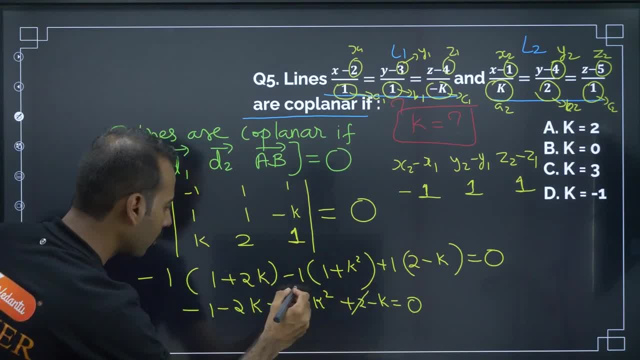 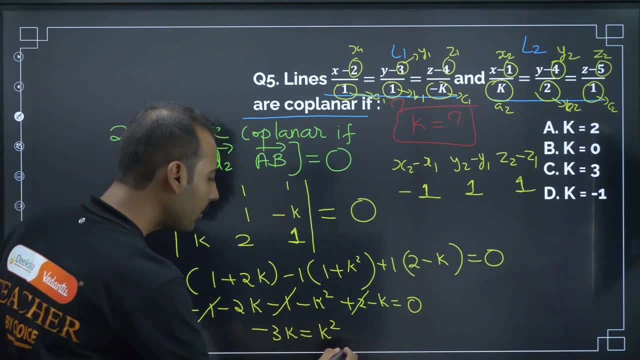 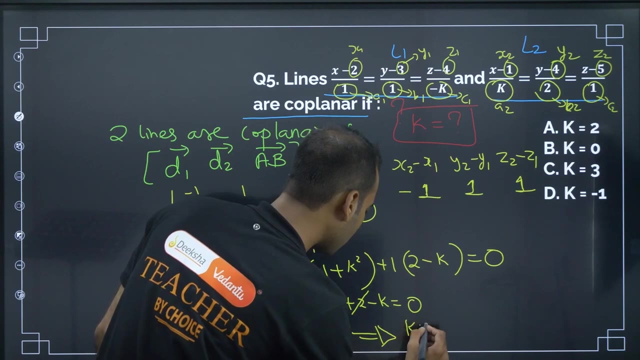 this equation: minus 1, minus 1, 2 positive, 2, negative, 2 get cancelled. minus 3, k is equal to k square, which implies which implies minus k is equal to, which implies k is equal to 0.. Or k is equal to: 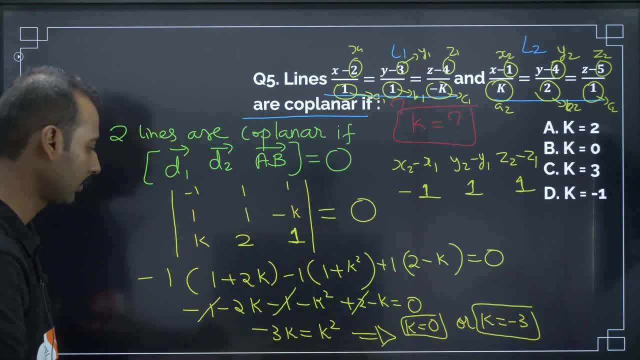 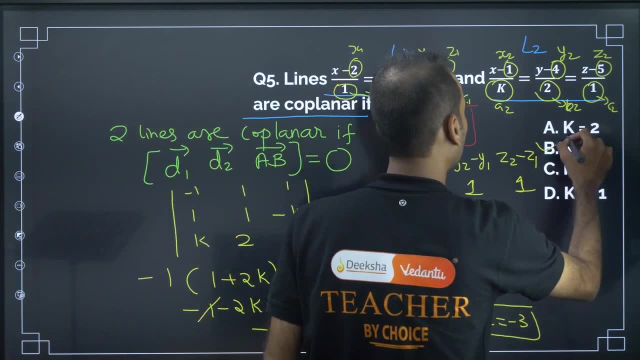 Minus Minus 3 k. So these are the two options. so k is equal to 0 or k is equal to minus 3.. So k is equal to 0, is available in the options. so, as per the availability, we have to mark. 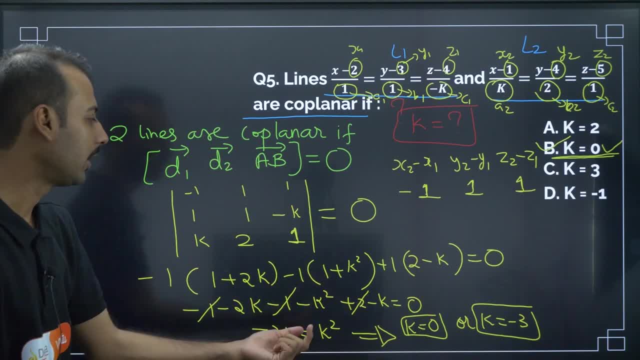 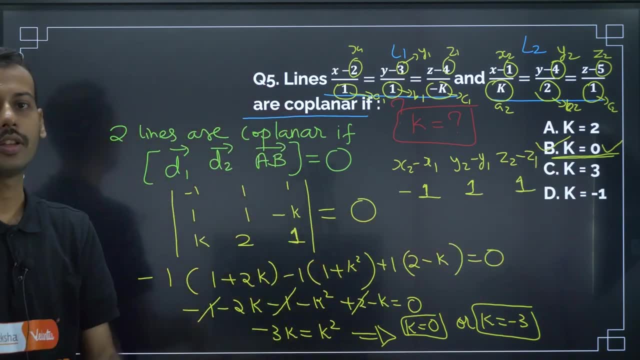 k is equal to 0 anyways, in CET they will not ask multi correct. So k is equal to 0 or k is equal to minus 3? what if k is equal to minus 3 is also given and k is equal to 0 is also given in the exam? what will you do? you just mark anyone then? 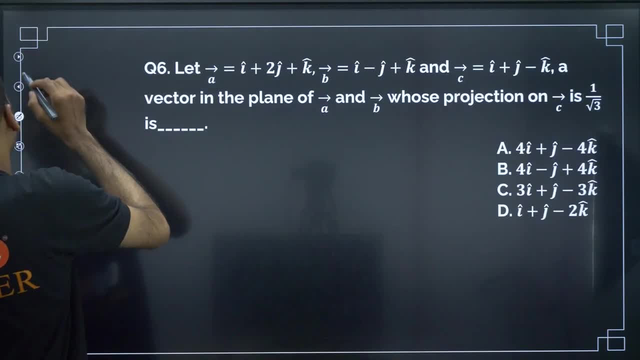 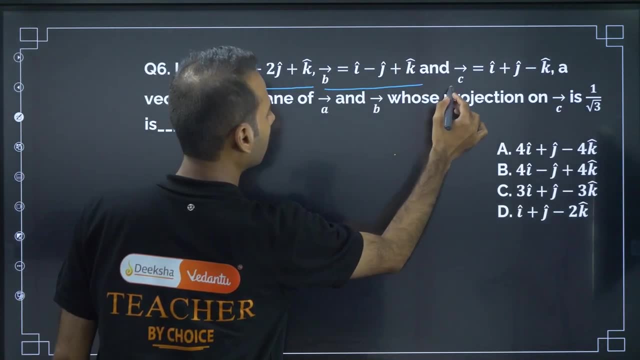 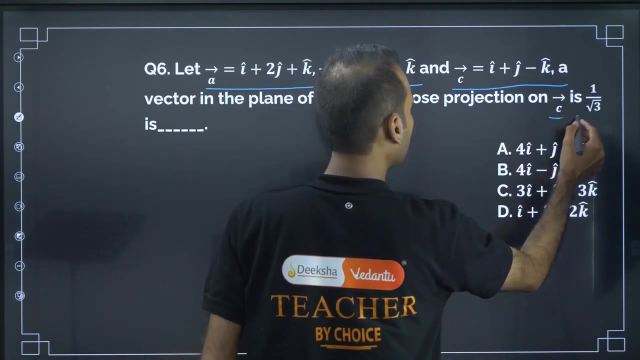 that question will be considered as grace. Anyways, That's it It marks. so, moving on to next question, They are given some information like: a is equal to b, is equal to c, is equal to a vector in the plane of a and b whose projection on c is this: 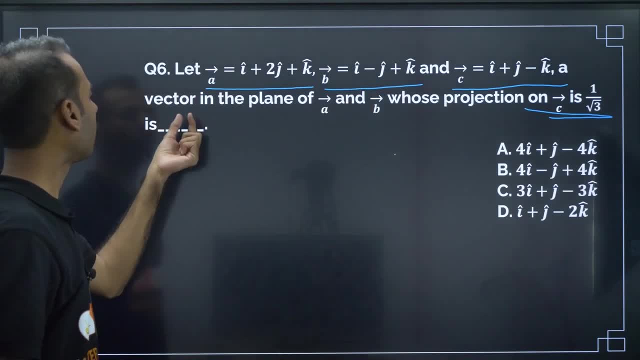 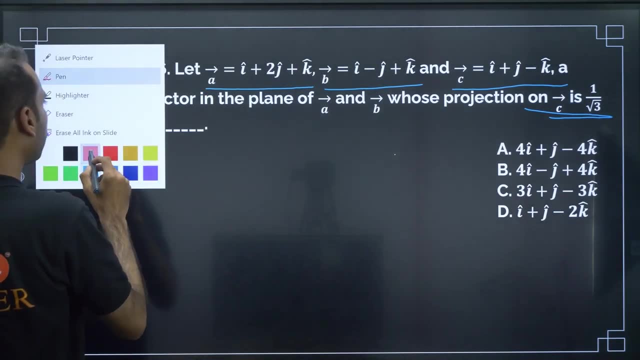 So what is the question? Let a is equal to b, is equal to c, is equal to vector in the plane of a and b whose projection on c is this. So what are they asking? They are Asking to find Vector in the plane of a and b. 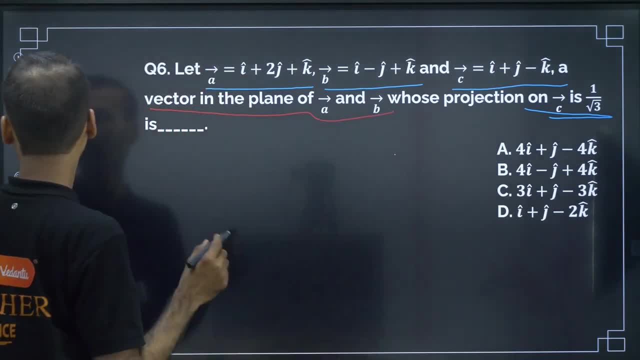 Is equal To this And how to find it For Vector in the plane of a- b. so they are talking about vector in the plane of a and b. generally, vector in the plane of a and b is given by: r is equal to a plus lambda b. now what is r? r is a in place of 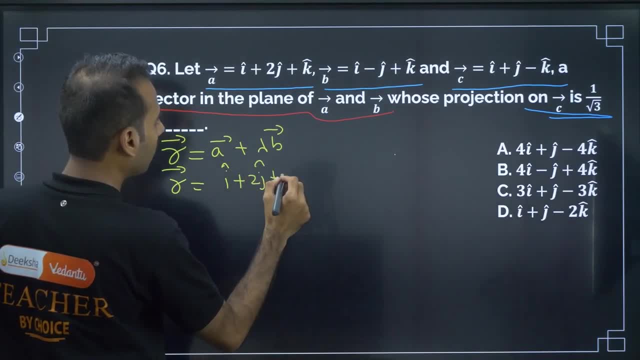 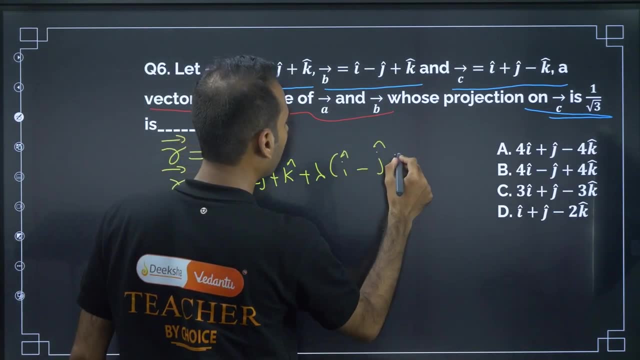 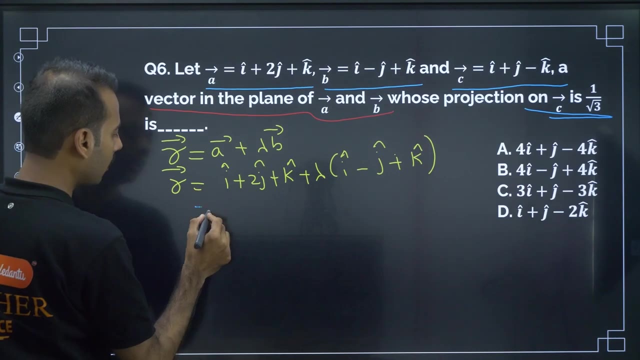 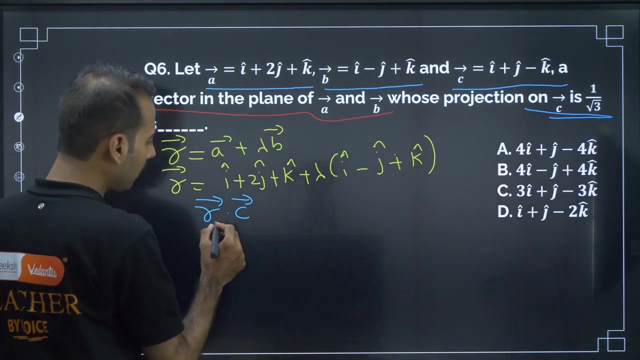 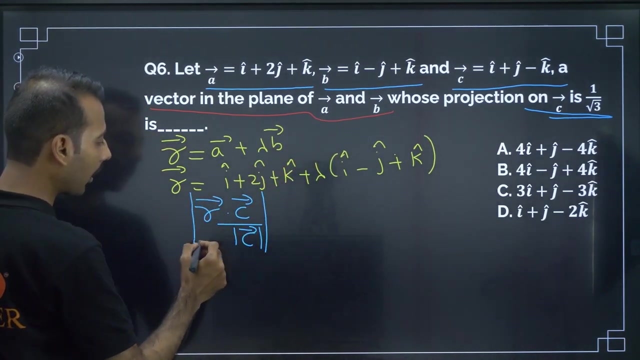 a, i, 2, j, 2, j plus k plus lambda b is i cap minus, j cap plus, whose projection? so try to recall the formula for projection- r dot c projection is given by r dot c. by c means we are projecting this, whose projection on c is one root three. now if you take magnitude. 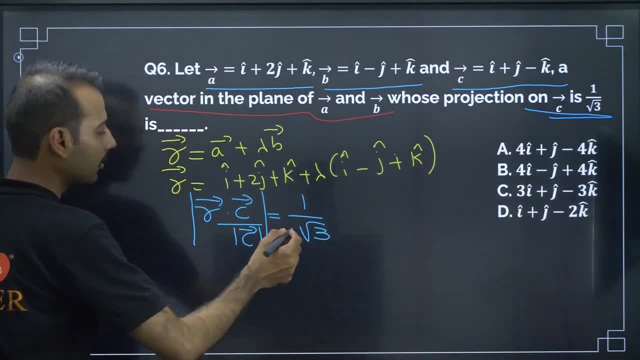 of this you are going to get one by root three. this is the given thing. so, given a projection of whose? projection on a? so i am assuming that projection of a and b in the plane means r, dot, c. we are projecting ANDREW defendment, uneasy esti. 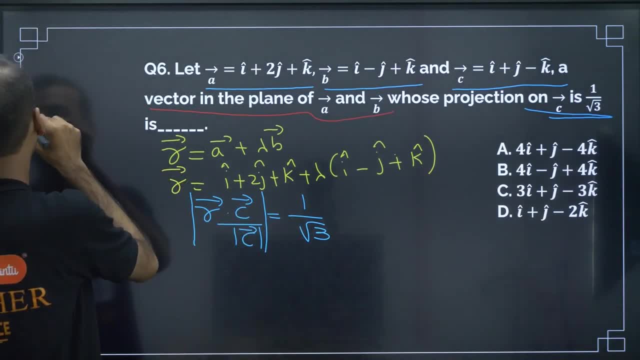 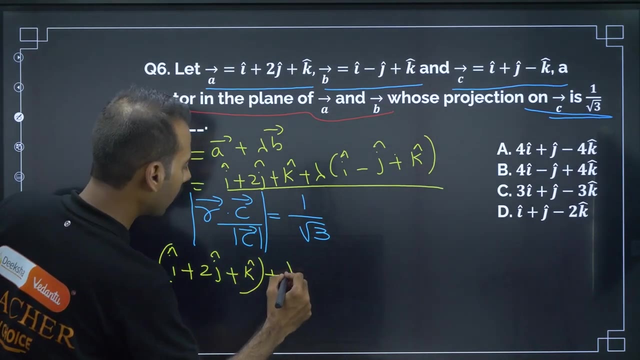 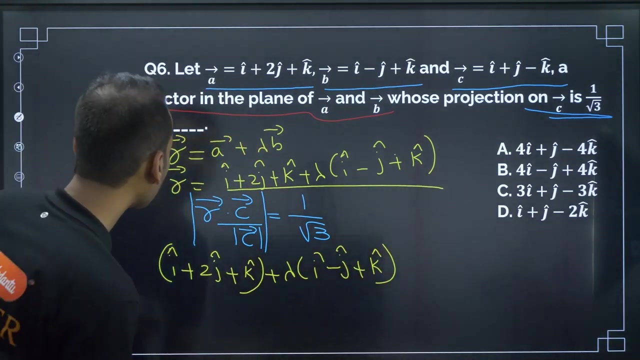 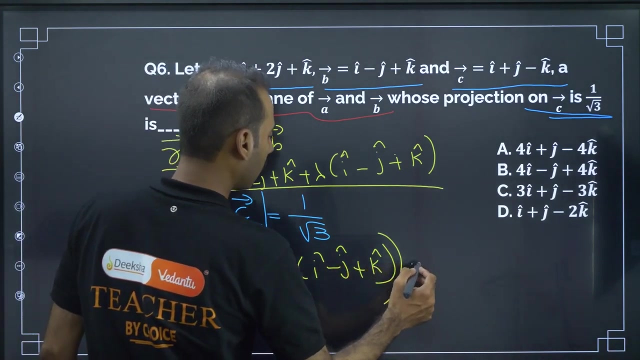 r vector on c. so projection on is 1 by root 3. this is the given information. so with the given data r is equal to. let me copy this and paste: i cap plus 2 j cap plus k cap plus lambda. i cap minus j cap plus k cap a plus lambda b dot c. dot c means now you write c vector. what is that c vector i? 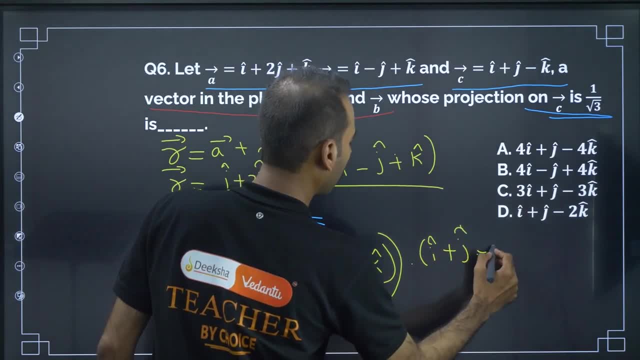 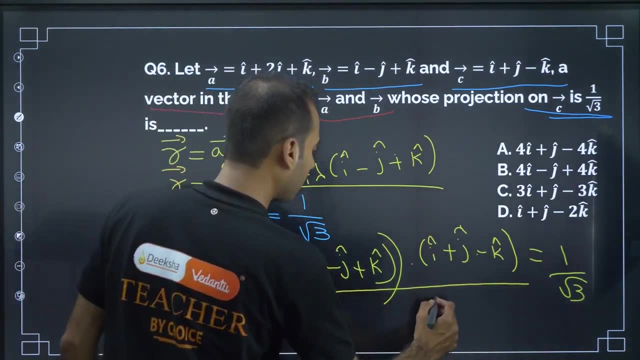 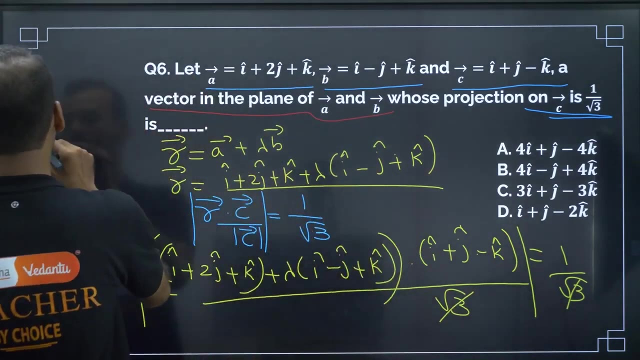 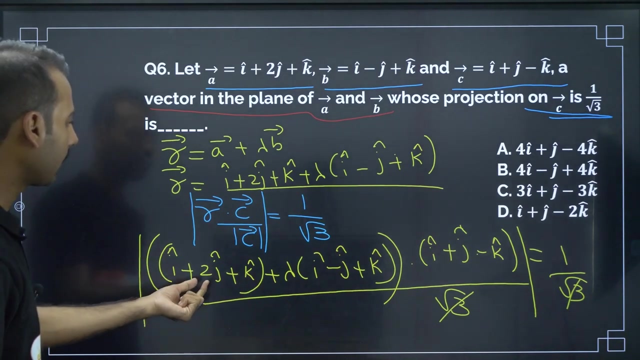 i, j minus k is equal to 1 by root. 3 is equal to 1 by root 3 and projection of c is also 1 by root 3. this and this get solved here. 1 modulus is there. 1 modulus is there. so let me erase few things so that it will be easier for me to simplify, or else i can simplify. 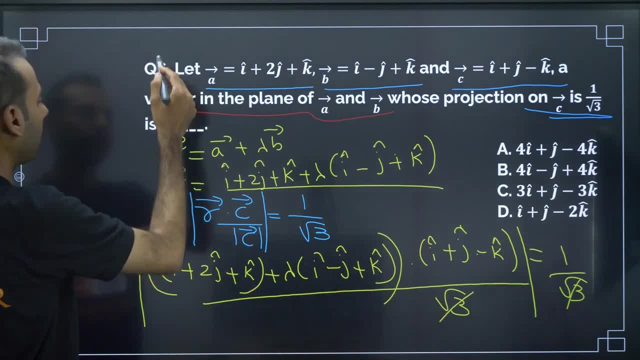 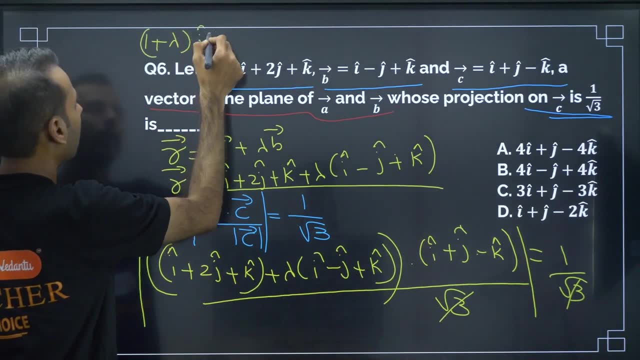 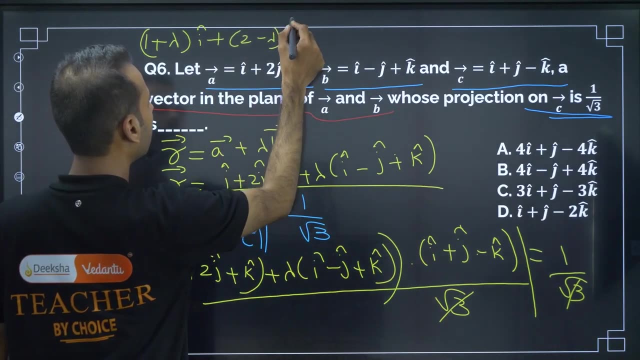 it here also. let me write here in the numerator at the top: 1 plus lambda i. this is 1 plus lambda 1 plus lambda i, 2 minus lambda, 2 minus lambda j plus 1 plus lambda i, 2 minus lambda j plus 1 plus lambda i, 2 minus lambda j plus 1 plus lambda j. 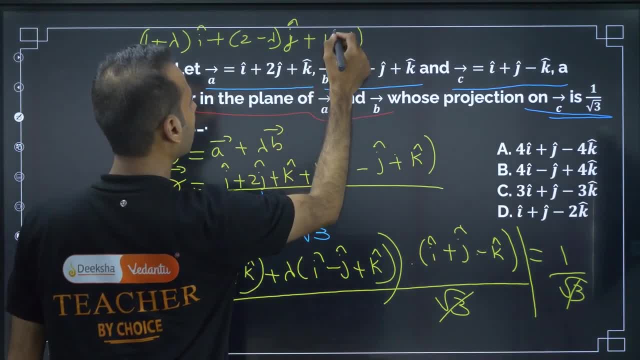 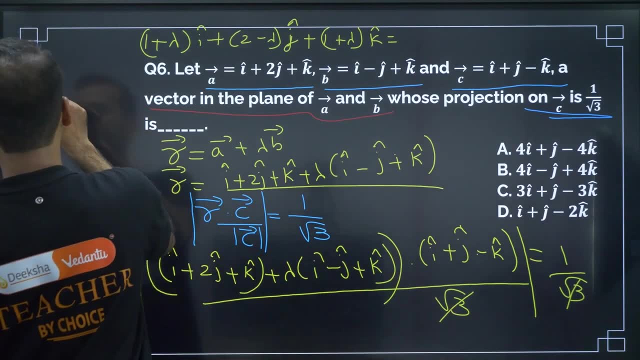 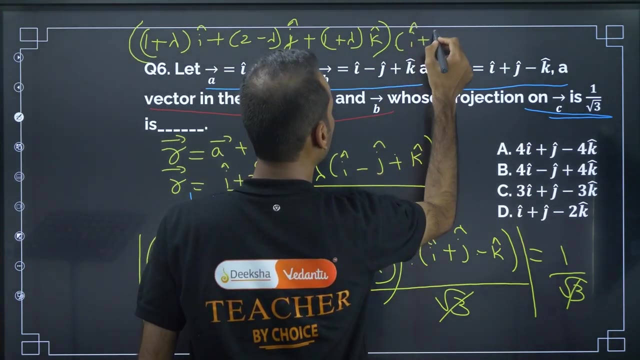 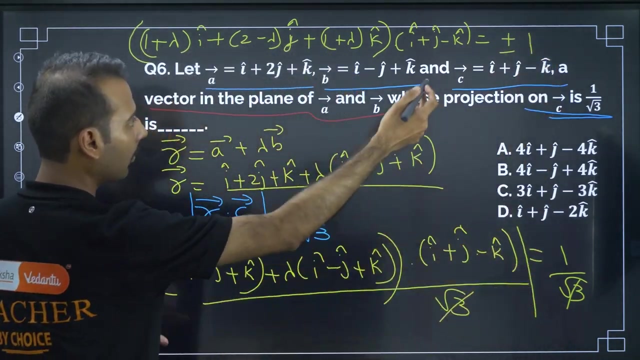 1 plus lambda 1 plus lambda k cap is equal to plus lambda dot. still dot is there. let me remove this. i plus j minus k. i plus j minus k is equal to 1. so whenever you are removing this modulus, you will get plus or minus 1. so let me remove few things from here. now we have to multiply. 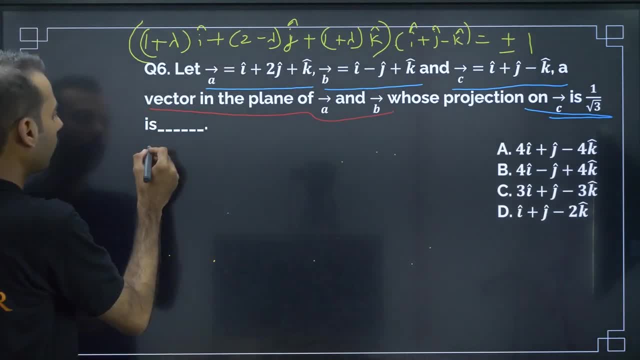 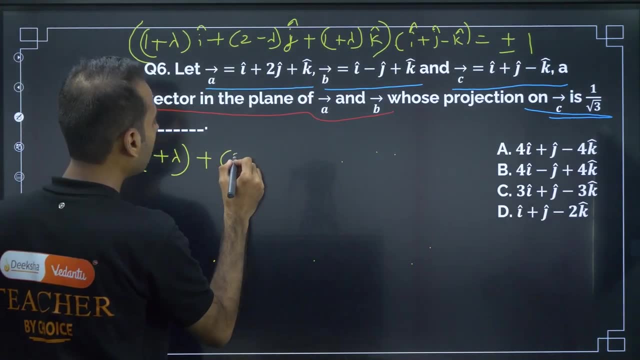 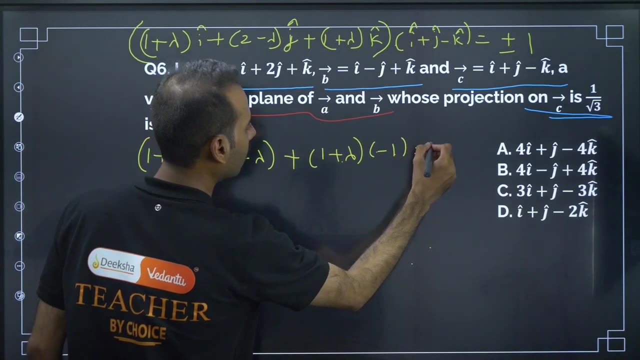 this and we will get plus or minus 1, so let me remove few things from here. now we have to multiply this 1 plus lambda. so for that let me write 1 plus lambda, this 1 plus lambda, and i plus 2 minus lambda, 2 minus lambda plus 1 plus lambda. 1 plus lambda minus 1 is equal to plus. 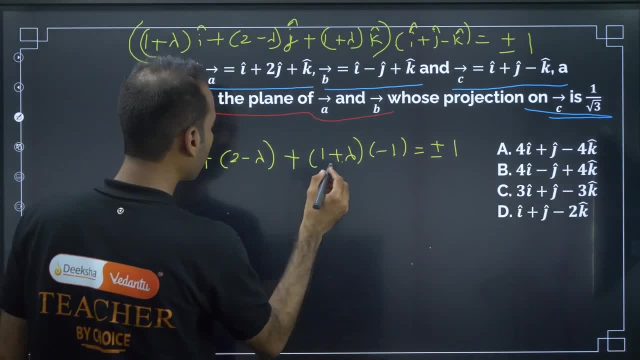 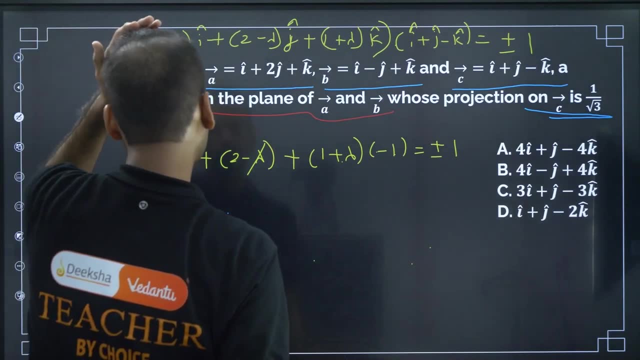 or minus 1. so 1 plus 2 plus 1 is for positive lambda- negative lambda, we can cancel. so 1 plus 2 is for positive lambda, negative lambda, we can cancel. so 1 plus 2 is for negative lambda, we can cancel. sorry, sorry, sorry and let me remove this. let me remove this. let me simplify it. 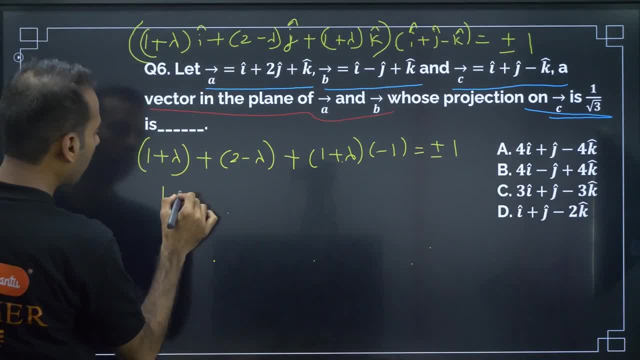 sorry, sorry, sorry, and let me remove this. let me remove this. let me simplify it. sorry, sorry, sorry, and let me remove this. let me remove this. let me simplify it properly. so if i simplify properly 1 plus properly. so if i simplify properly, 1 plus properly. so if i simplify properly: 1 plus lambda plus 2 minus lambda plus 1, not plus. 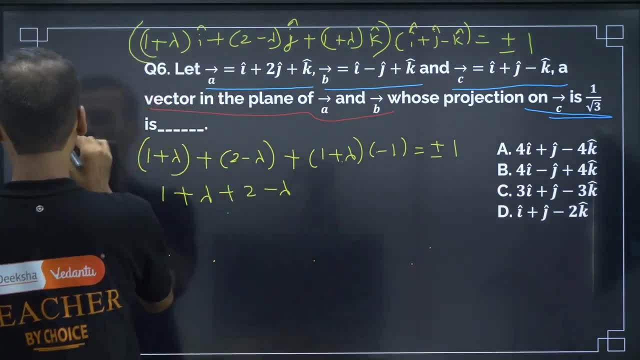 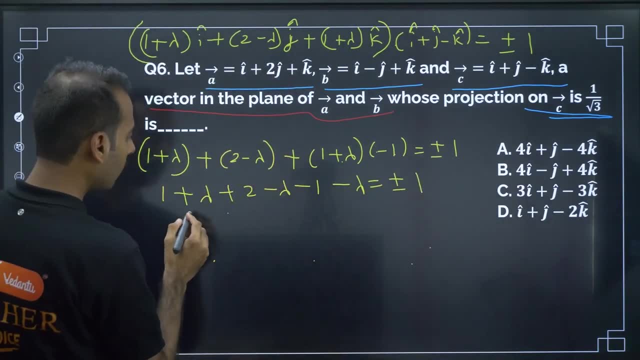 lambda plus 2 minus lambda. plus 1, not plus lambda. plus 2 minus lambda. plus 1, not plus 1 minus minus 1. minus lambda is equal to 1 minus minus 1. minus lambda is equal to 1 minus minus 1 minus lambda is equal to plus or minus 1. now positive 1. negative 1. 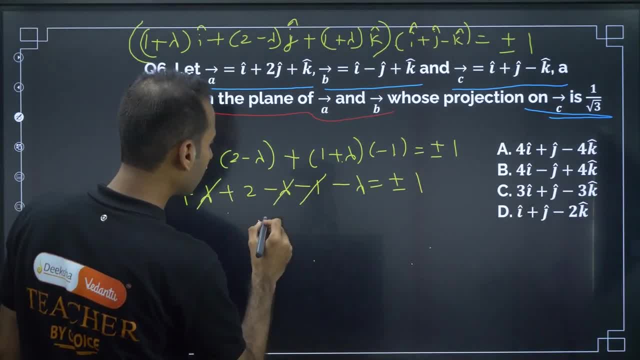 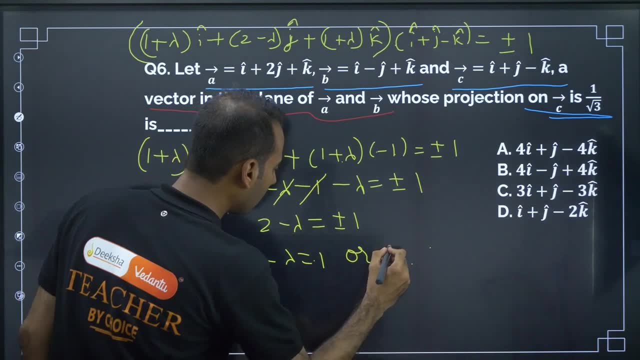 plus or minus: 1. now positive: 1. negative. 1. plus or minus 1. now positive: 1. negative. 1. cancel. positive lambda- negative lambda. cancel positive lambda- negative lambda. 2 minus lambda is equal to plus or minus 1.. So 2 minus lambda is equal to 1 or 2 minus. 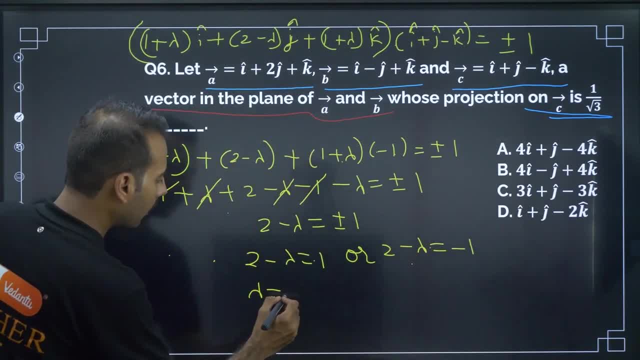 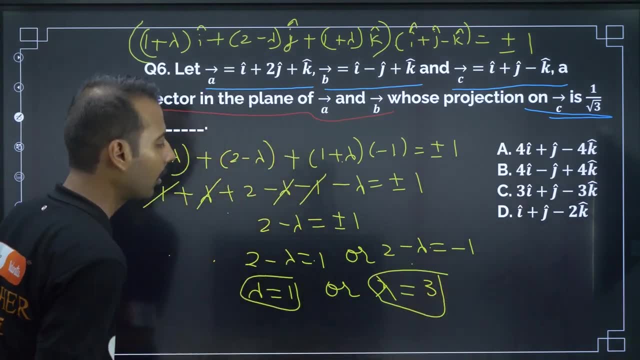 lambda is equal to minus 1.. That means lambda is equal to 1 or lambda is equal to 3, lambda is equal to 1 or lambda is equal to 3.. Now lambda is equal to 1 if I keep in R, if I. 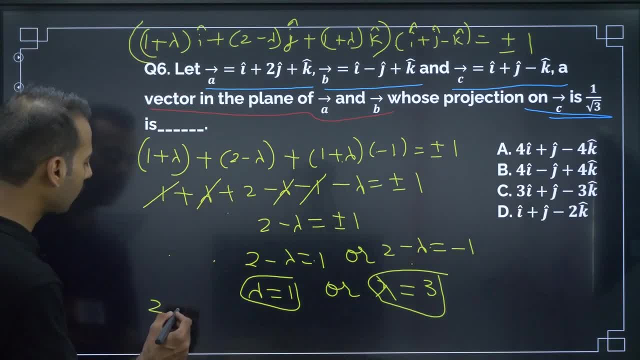 I keep, lambda is equal to 1 here, then I will get 2. and what about this 1 and lambda? if I keep here 2, is there any such option? 2 1, 2. there is no option. 2 1, 2. if I take, lambda is equal to 3 and 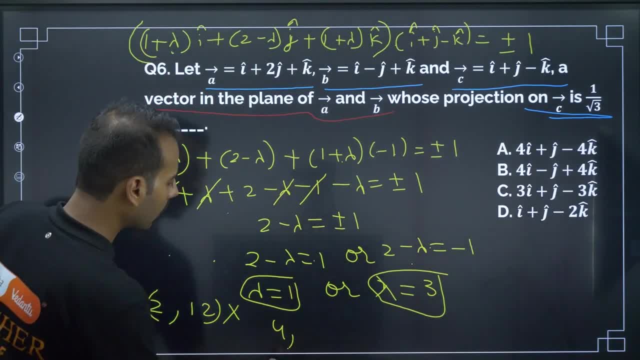 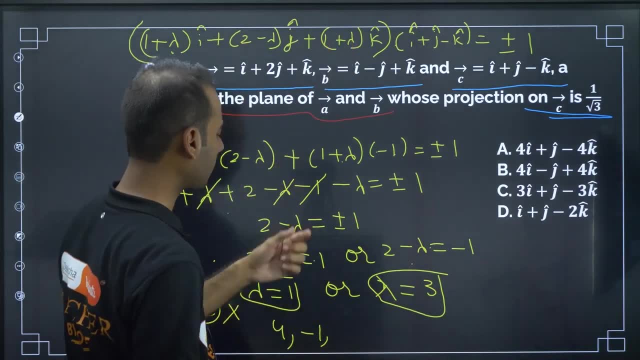 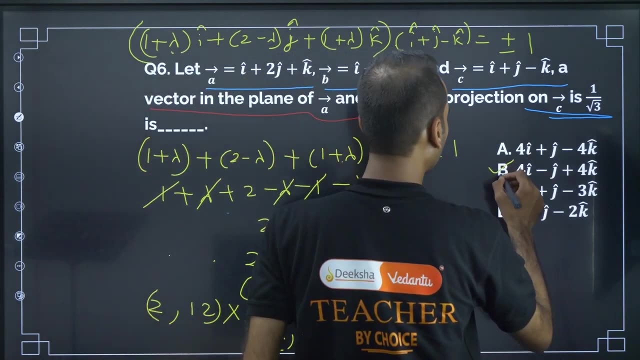 I will place here 1 plus 3, 4. 1 plus 3: 4 lambda is equal to 3. if I place 2 minus 3 is minus 1. lambda is equal to 3. if I place 1 plus 3 is 4, 4 minus 1, 4, 4 minus 1, 4. so answer for this is: 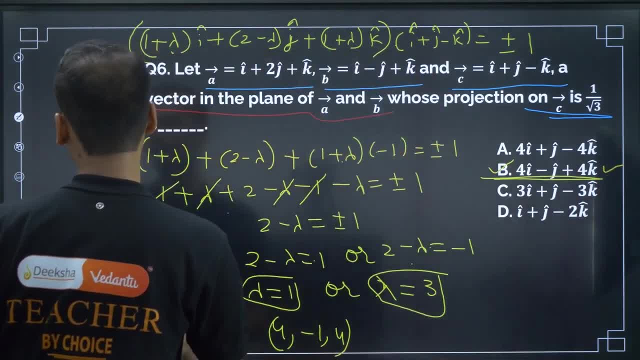 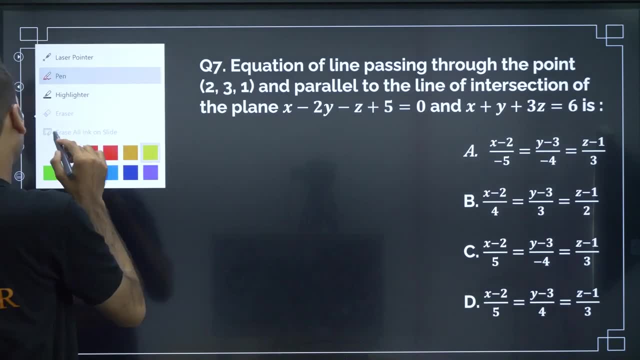 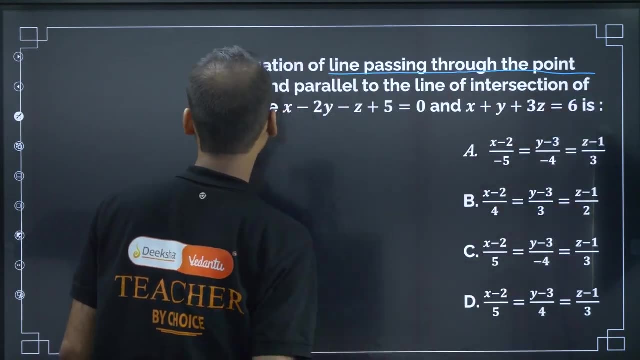 b, b is the answer. next, moving on to next question, the equation of line passing through the point and parallel to the. so some information they have given. equation of line passing through point. equation of line passing through the point 231 and parallel to the point 231. 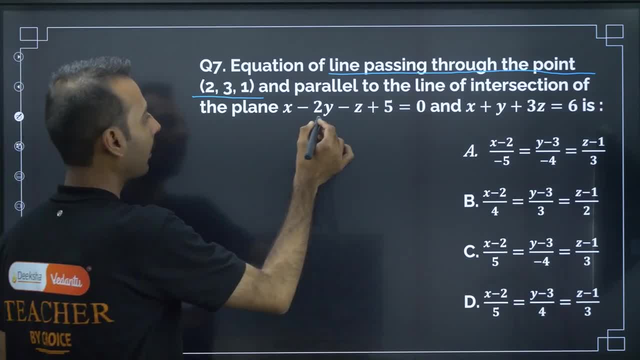 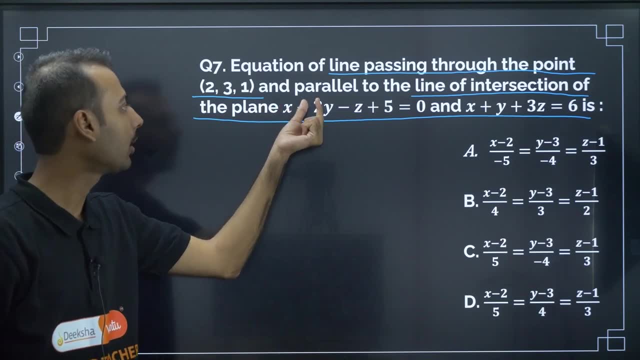 the equation of line passing through and parallel to the and parallel to the line of intersection of this. and this is equation of line passing through one point- One point they have given- and parallel to the line of intersection of this and this. So what are they asking? equation of 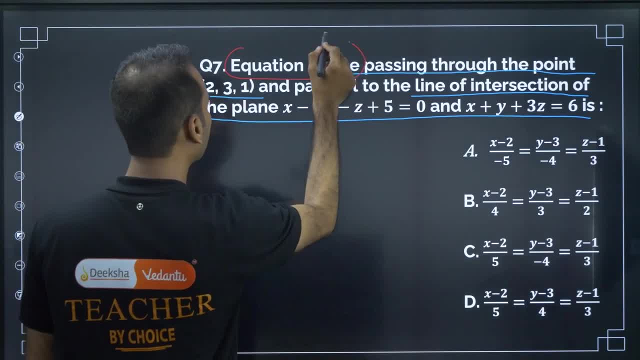 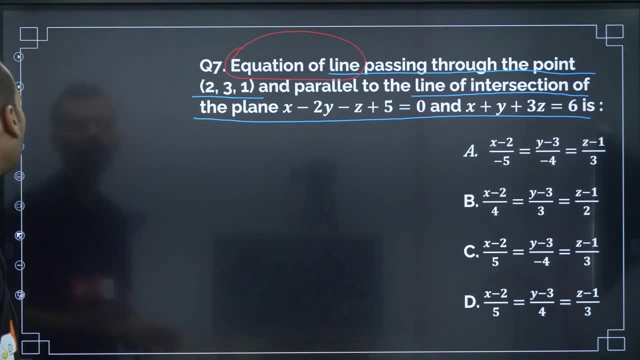 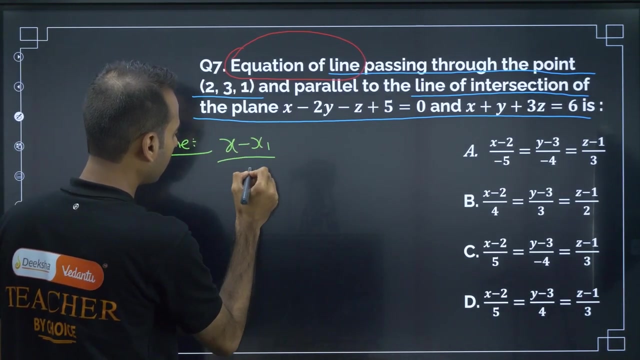 line. They are interested in equation of line. They are asking us to find this. Now, how to find this? c r, c? r. equation of line generally, equation of line also. all these are in in cartesian form. so equation of line. equation of line is given by x minus x, 1 by a, equal to y minus y, 1 by b. 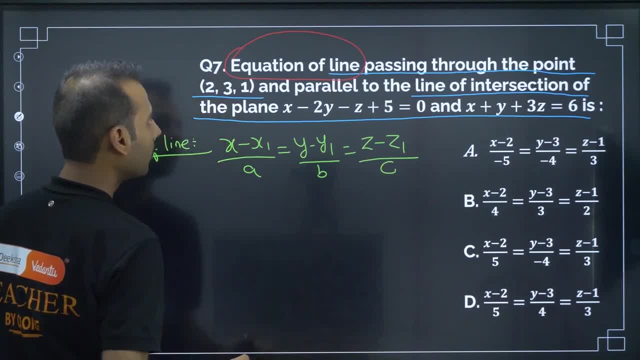 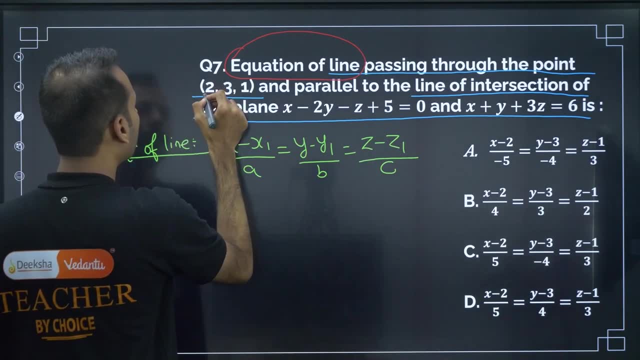 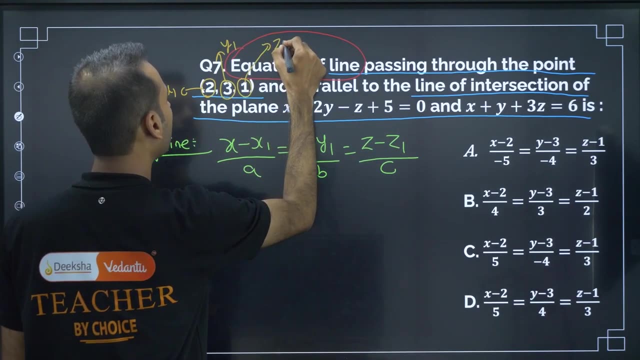 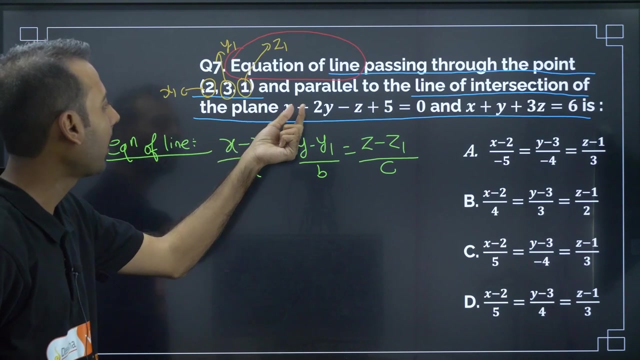 equal to z minus z 1 by c. so x, 1. equation of line passing through the point, one point they are given, what is that point? x 1, y 1 and z 1. equation of line passing through this point. equation of line passing through point and parallel to the line of intersection. 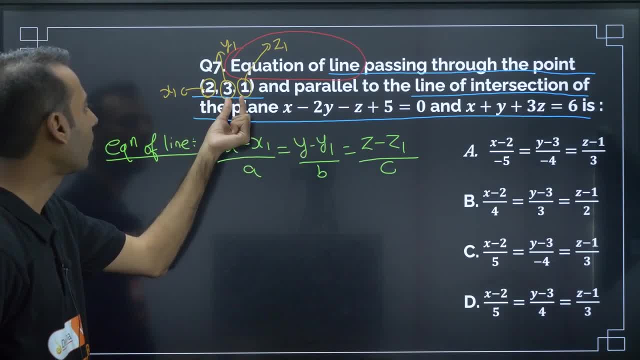 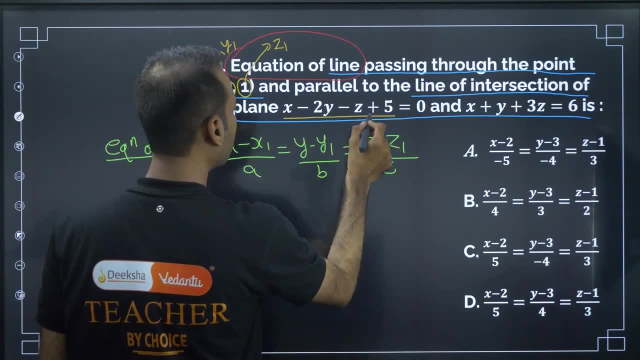 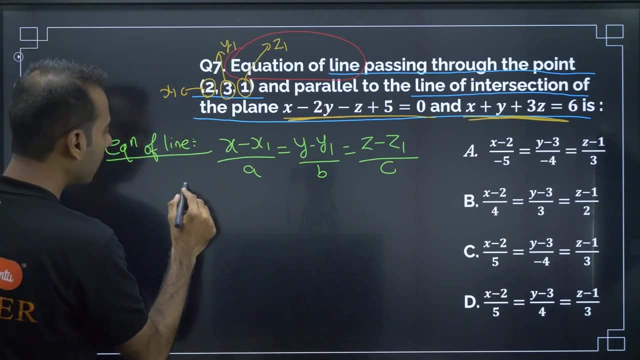 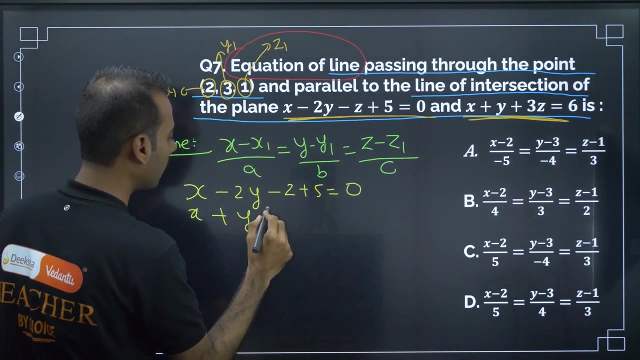 so try to recall this concept. equation of line. if one point is given generally and parallel to the, now, whenever they are talking about parallel to parallel to means, from here we will get direction ratios. now how to find direction ratios? try to recall: in 10 standard, if two equations are given: y, z plus 5 equal to 0. x plus y plus 3, z is equal to 6. try to. 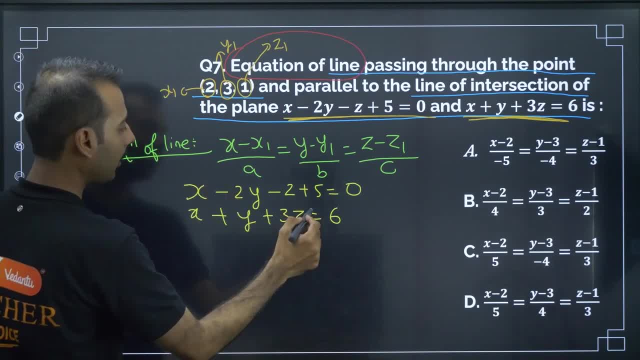 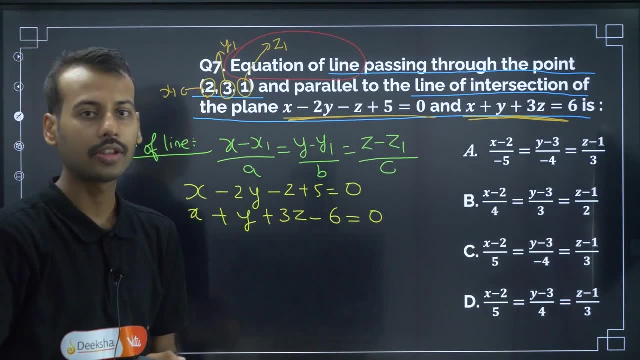 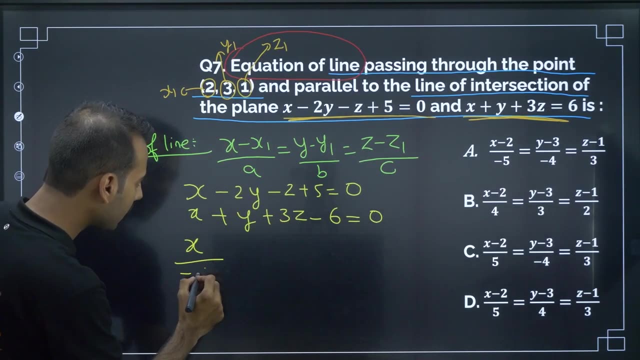 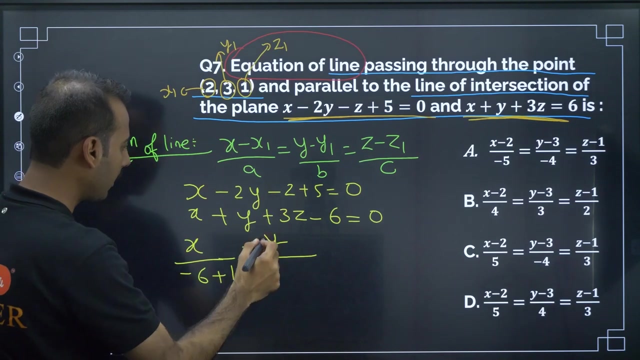 recall, in 10 standard, in 10 standard we used to solve. we used to solve two equations using cross multiplication method and then we used to find x, y, z values. here i will write: x minus minus 6 minus 6 plus 1 is equal to y divided by y, divided by 3, 3 plus 1. 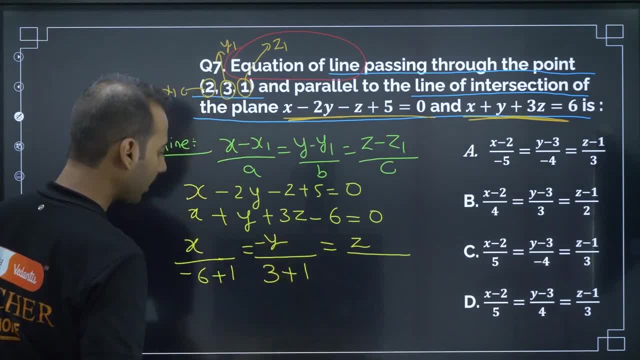 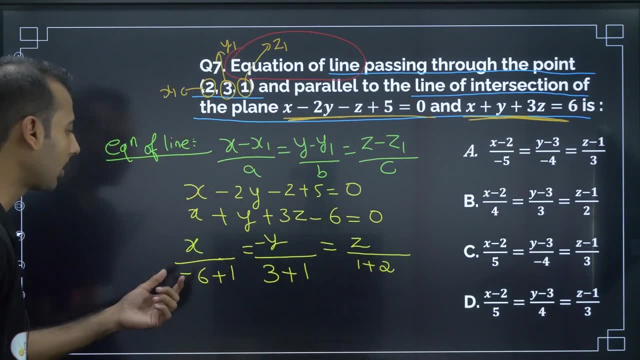 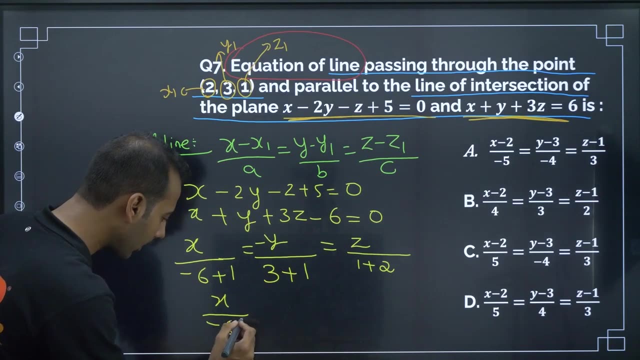 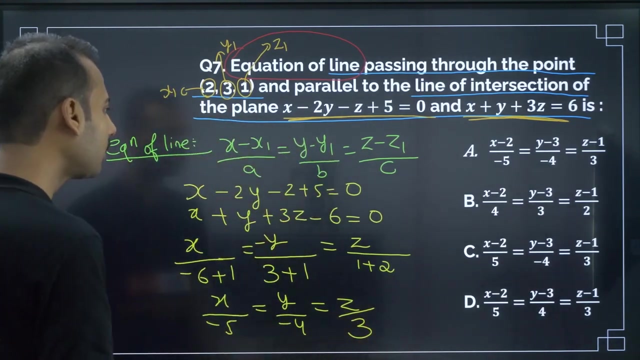 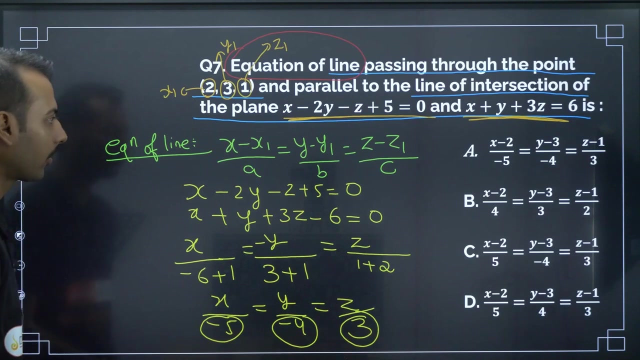 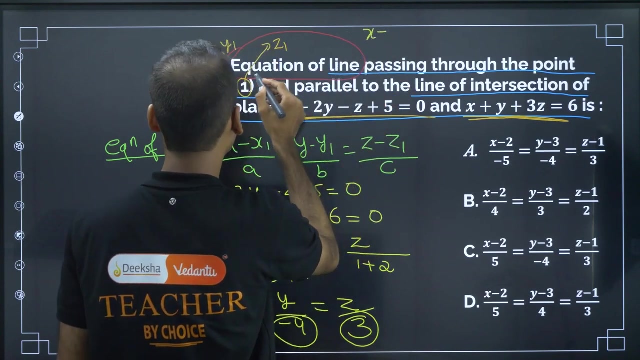 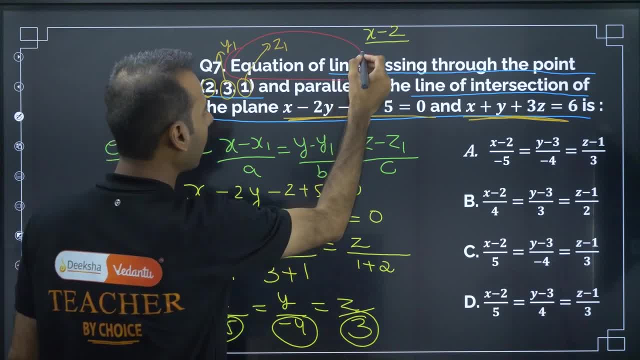 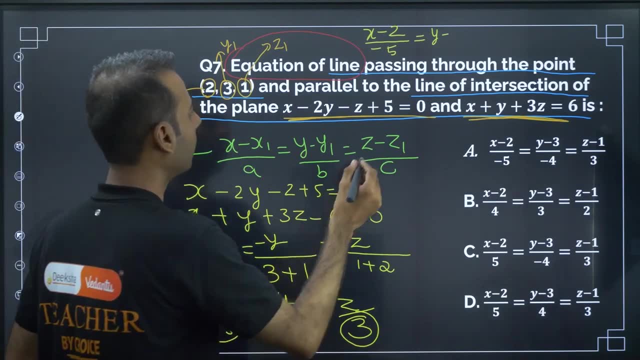 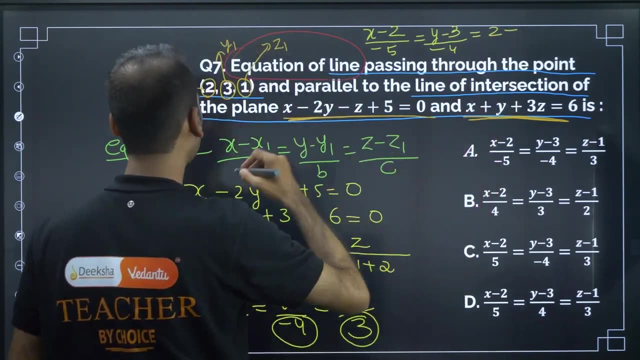 of x1, I will write 2 divided by. here we are getting minus 5, y minus y1 in place of y1. what is y1? y1 is 3 by y1 is 3 by minus 4 is equal to z minus z1. what is z1? z1 is 1. z1 is 1 by a. 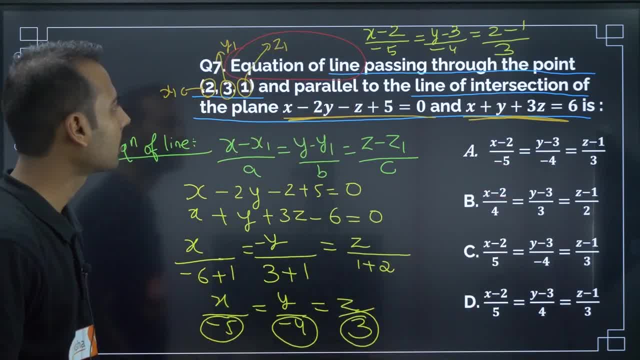 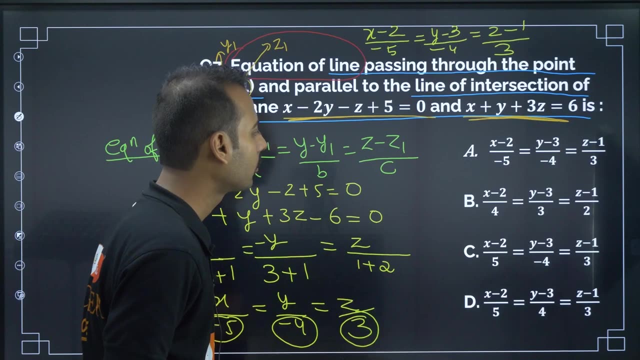 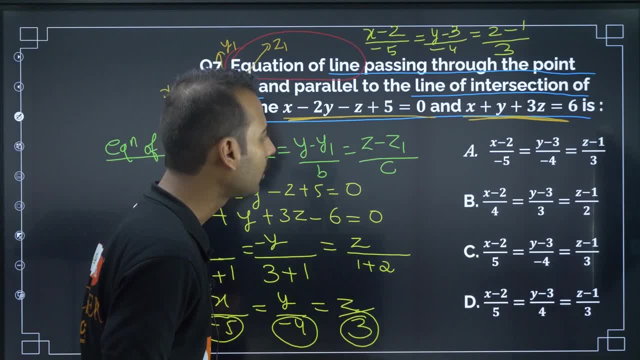 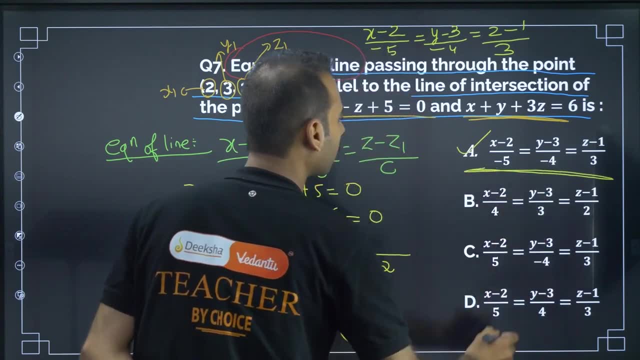 minus 5 minus 4, 3 minus 5 minus 4, 3 is 2 y minus 4. a is the answer. minus 5 minus 4: 3. okay, so a is the answer. try to go through the synopsis. these are all previous year questions, so very. 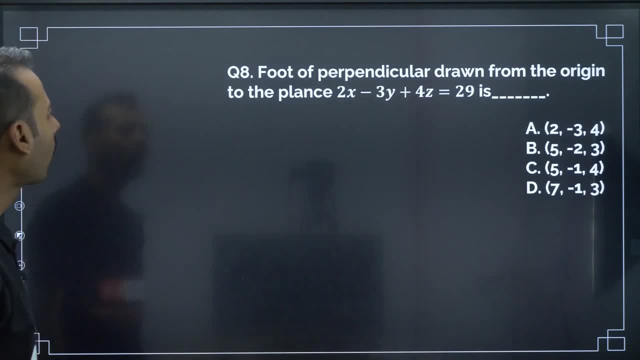 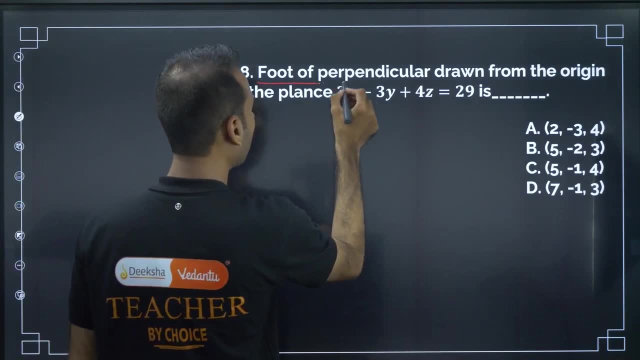 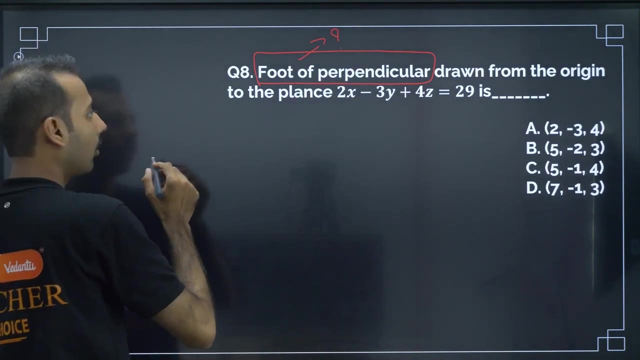 important synopsis and the foot of perpendicular drawn from origin to the plane is so the question is: what are they asking? they are asking foot of perpendicular. this is the question: foot of perpendicular drawn from from where they are drawn, from origin to the plane is now, what are they? 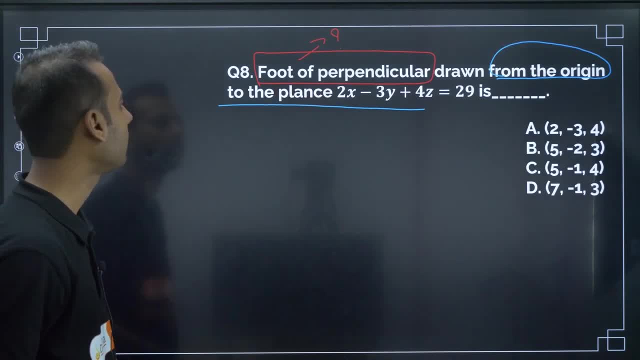 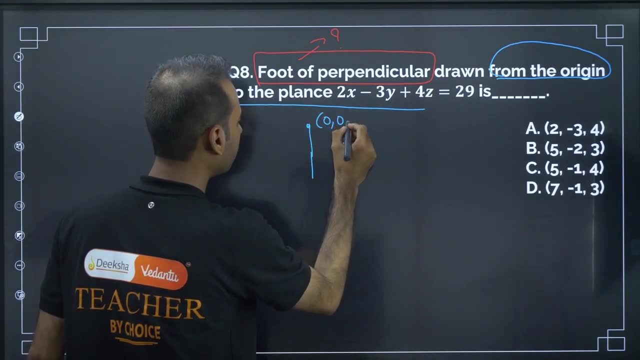 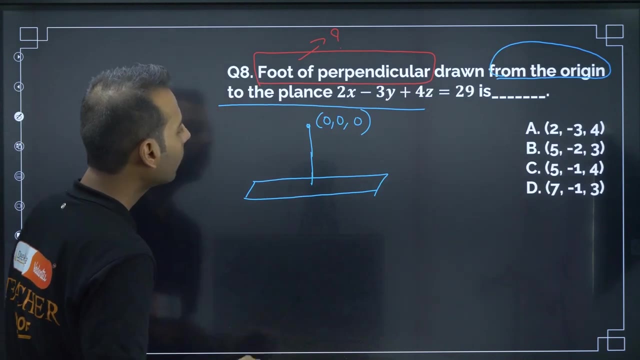 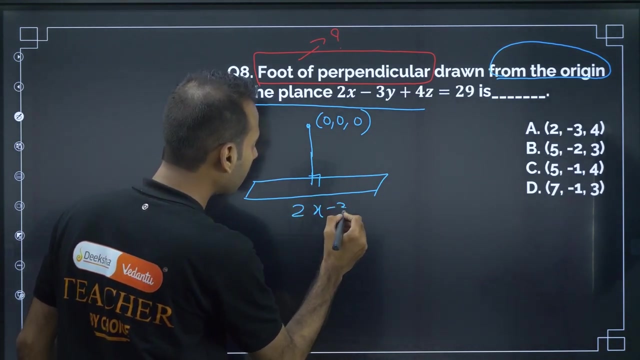 asking once again. i will represent it once. i will represent it visually: foot of perpendicular drawn from origin. foot of perpendicular. they are talking about this- drawn from origin to the plane. this 2x minus 3y plus 4z is equal to 29. i hope you might have. 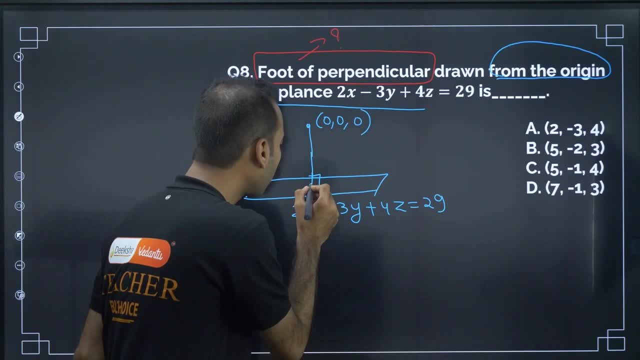 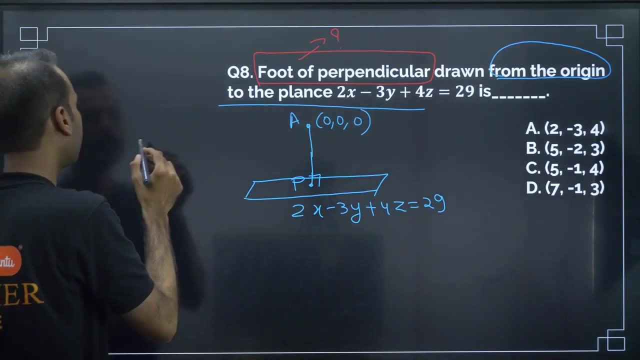 understood what they are asking. foot of perpendicular, which is the foot of perpendicular, this, let me mark this as a, let me mark this as p. so foot of perpendicular means what are they asking? they are asking what is this p, coordinates of p drawn from origin to the plane. this, this is 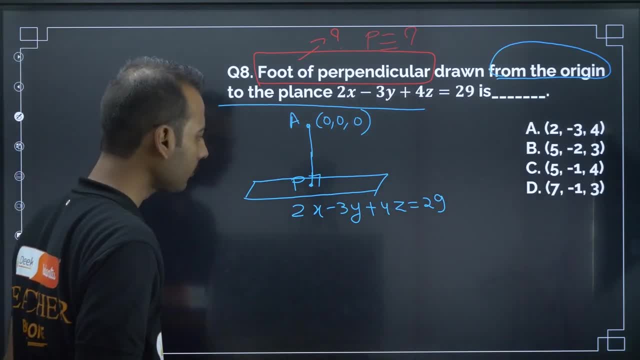 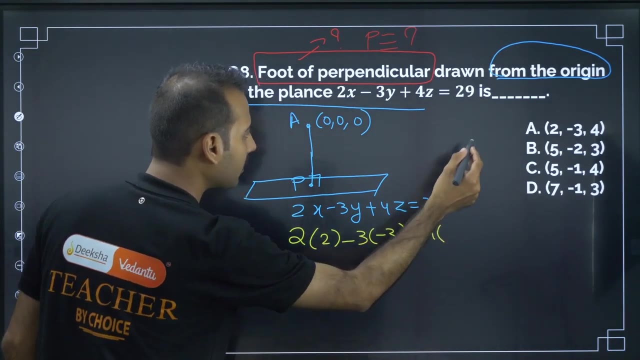 the plane. so how to approach this now that foot of perpendicular is lying on this plane. so any, if i try to substitute any one of this- 2, 2 minus 3 minus 3 plus 4- that means that point has to satisfy this. so if i am substituting here, i will check whether we are getting answer 4. 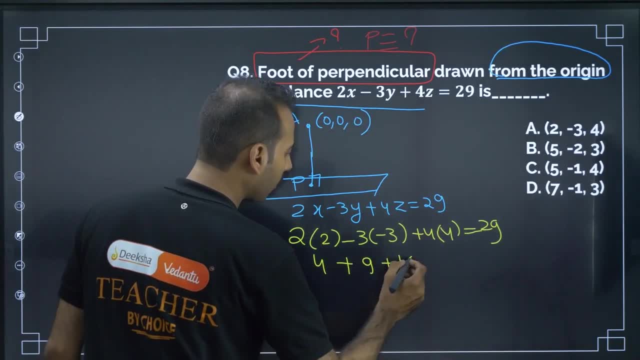 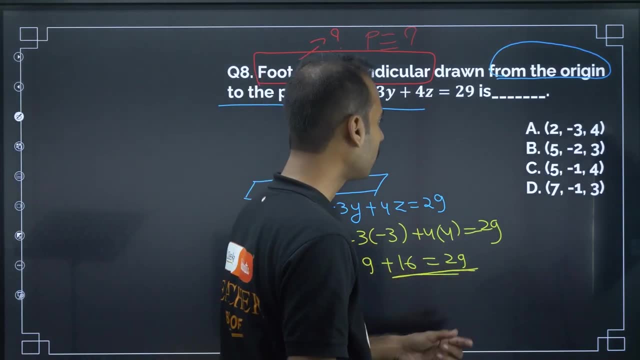 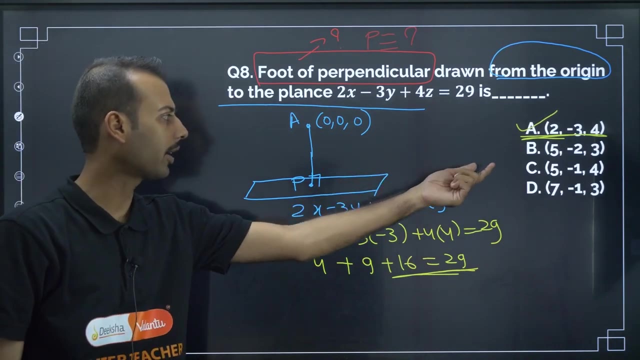 plus 9 plus 16, 16 plus 4, 20, 29 is equal to 29. so 29 is equal to 29 means 9 is equal to. so we can consider 2 minus 3, 4. now in exam generally, i will mark and i will move, but if you want to go for another option, whether 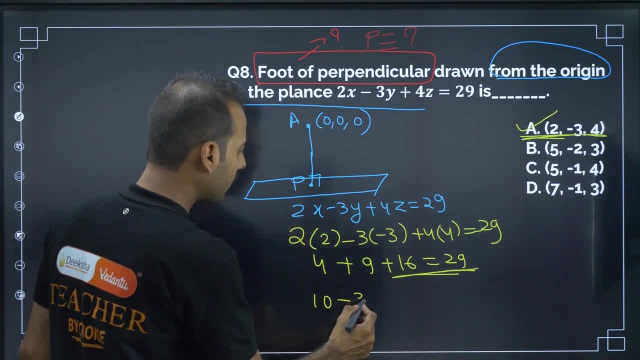 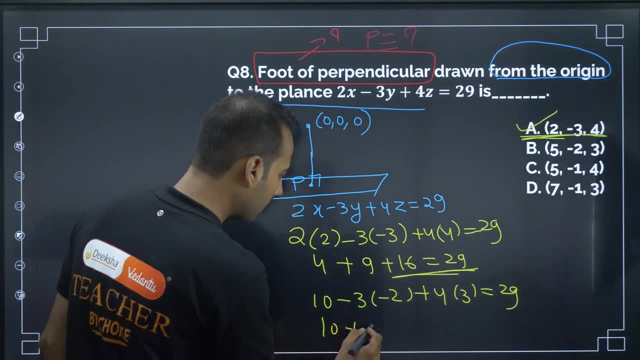 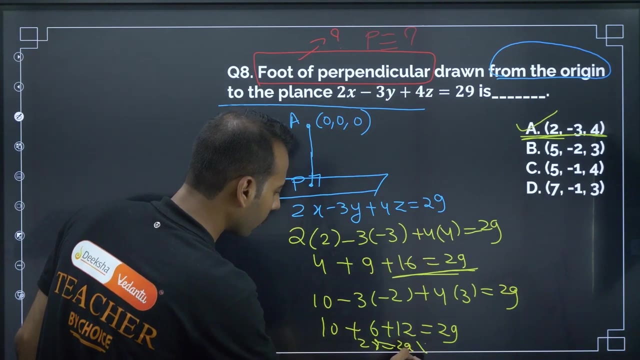 it is correct or not, you can go: 2: 5 is a 10 minus 3 minus 2 plus 4: 3 equal to 29. so 10 plus 6 plus 12 equal to 29. is it possible? this is 28 equal to 29, not possible. so. 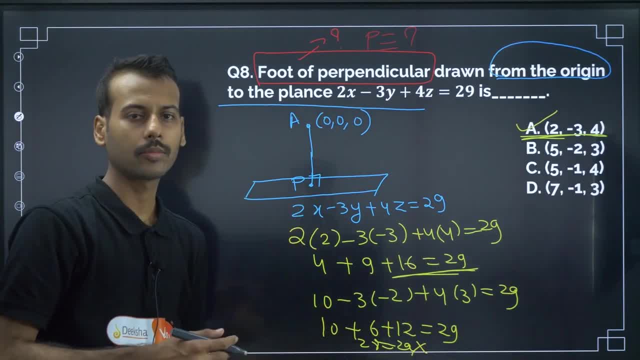 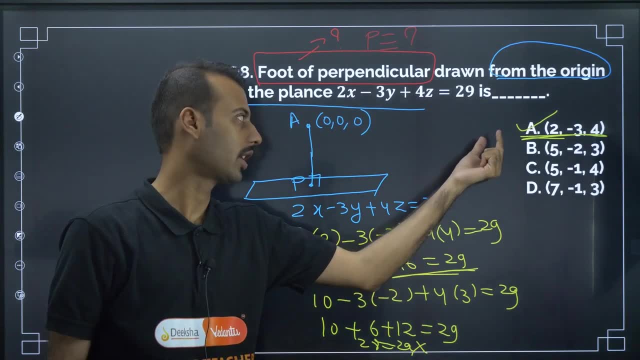 eliminate this. answer is 2 minus 3, 4. anyways, using method also we can solve. if you want me to solve using method, also we can solve. if you want me to solve using method, also we can solve using method. generally in exam we will find the shortest method which will save less time, which? 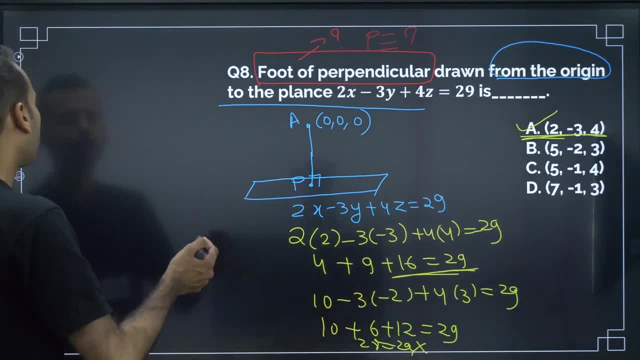 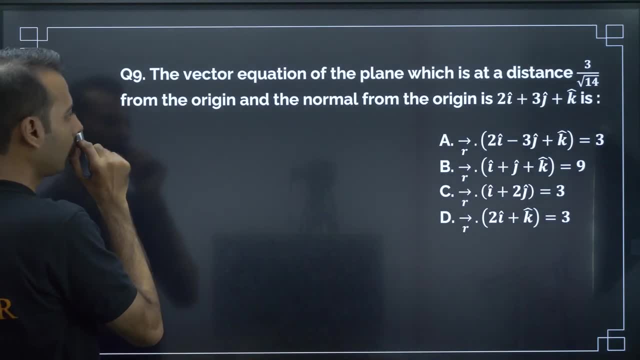 we require less time, so generally we go for substitution. if you want me to solve using method, i am ready to just add one comment next. moving on to next, the vector equation of the plane. so what are they asking in this question? the vector equation of plane. they are asking to find 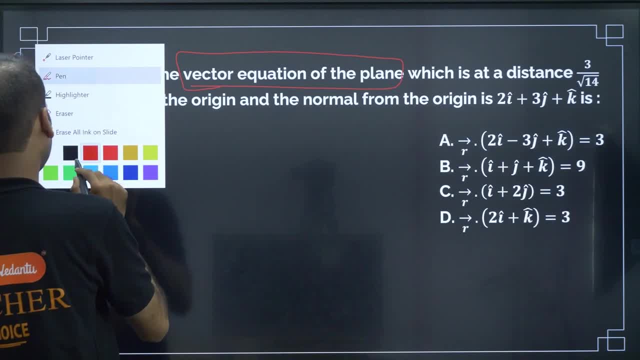 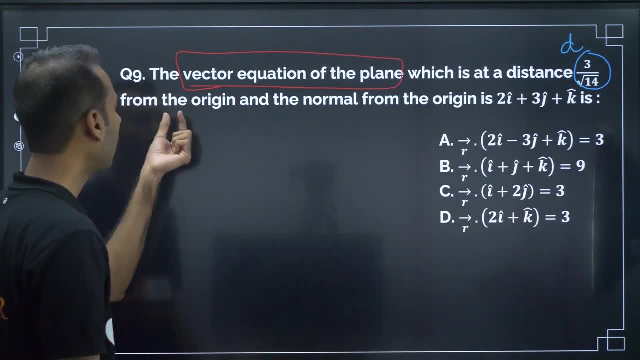 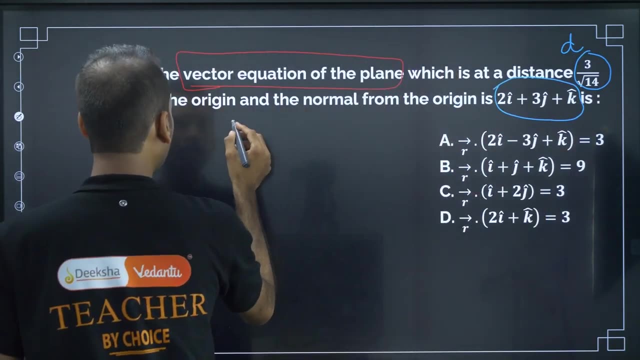 vector equation of plane which is at a distance. some information they have given which is at a distance, distance is the which is at a distance from origin and normal from origin. is this normal from? So d value they have given, d value is 3, by root 14 and origin normal from. 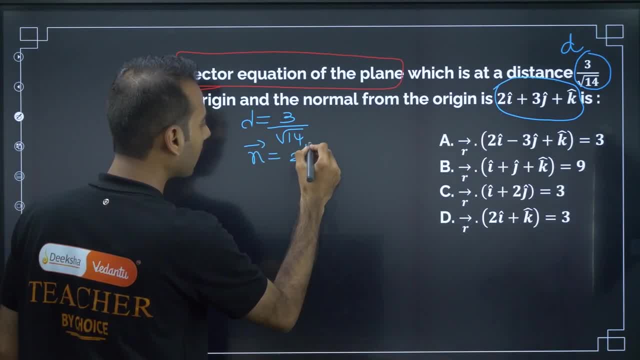 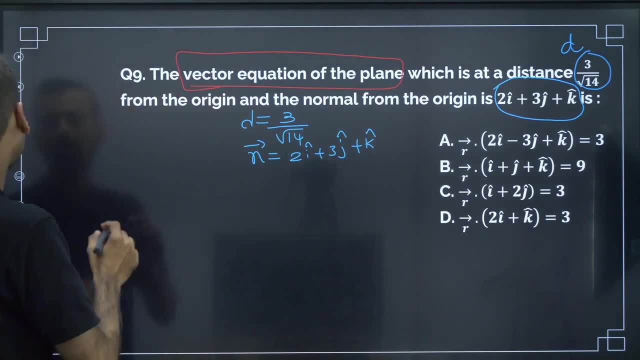 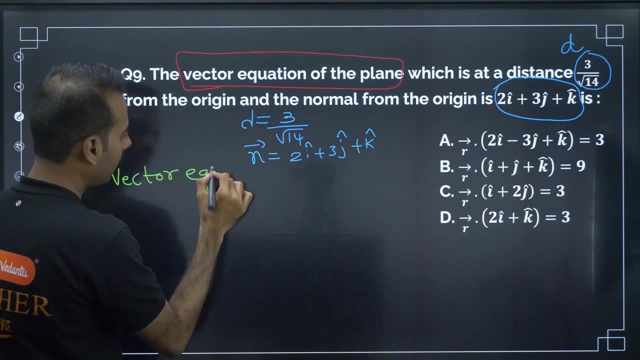 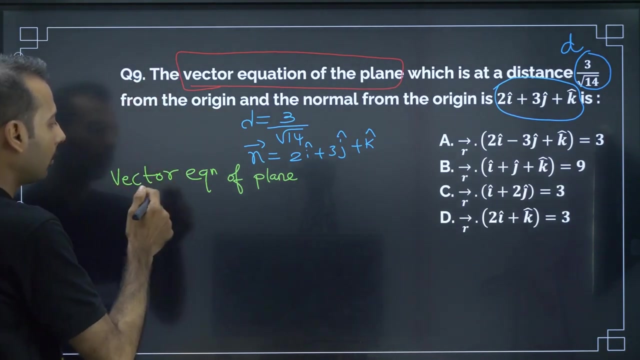 origin means n vector. also they have given 2 i cap plus 3 j cap plus k cap, The vector equation of plane. now try to recall vector equation of a plane, vector vector equation of plane. vector equation of plane which is at a distance of of plane is given by r dot. 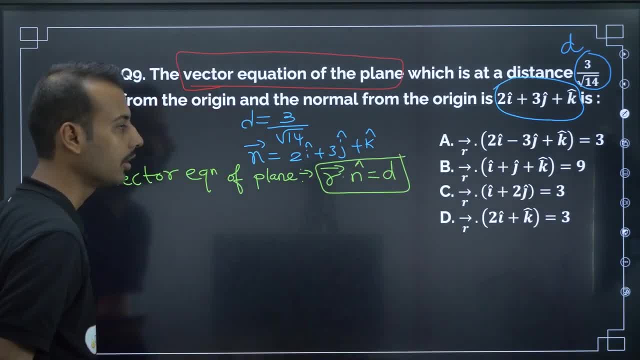 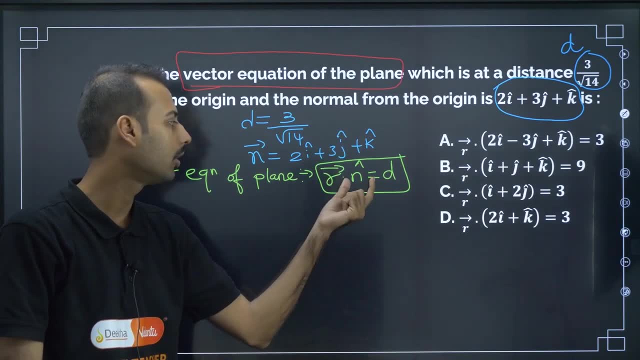 n cap is equal to d. try to recall this. one derivation is there. go through the derivation and you should be able to recall the moment you see this question. You should, The moment you see this question, you should be able to recall this synopsis. So r, r vector is what is that? r vector? the vector equation. 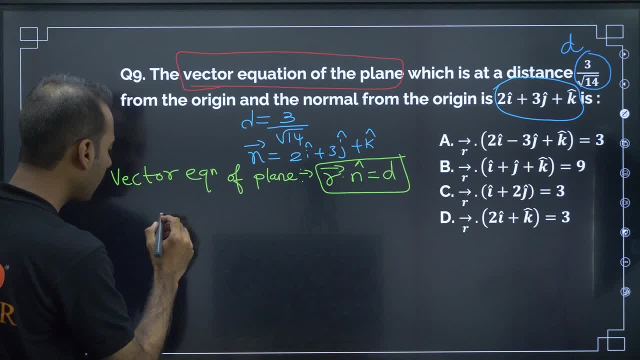 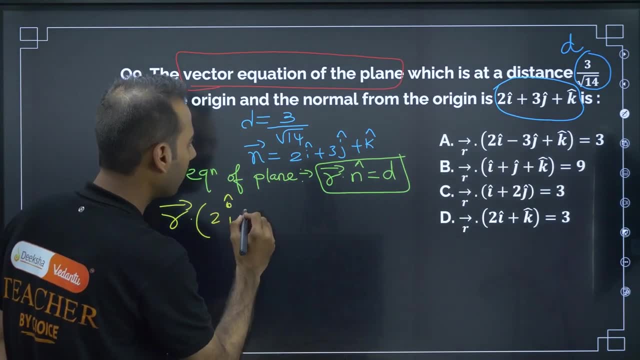 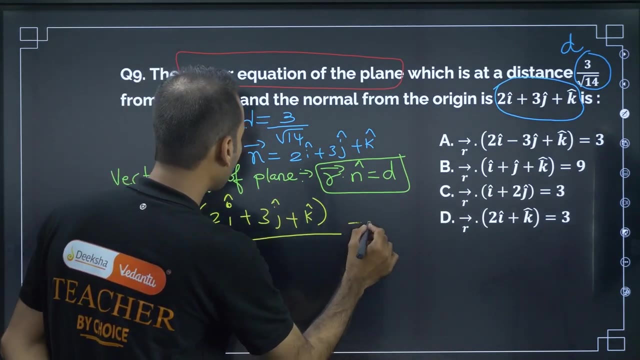 of plane r vector in place of r. let me write r only r dot n cap n cap means 2 i cap. 2 i cap plus 3 j cap plus k cap divided by. divided by is equal to d in place of d. let me write: 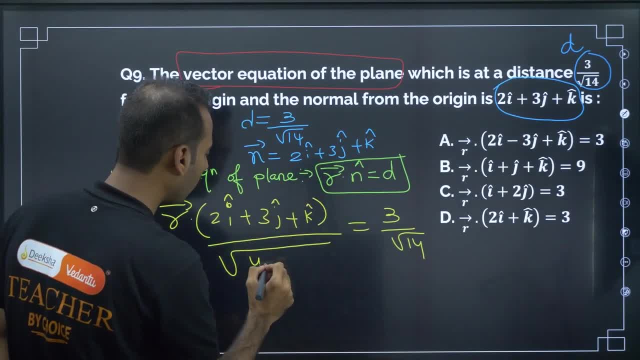 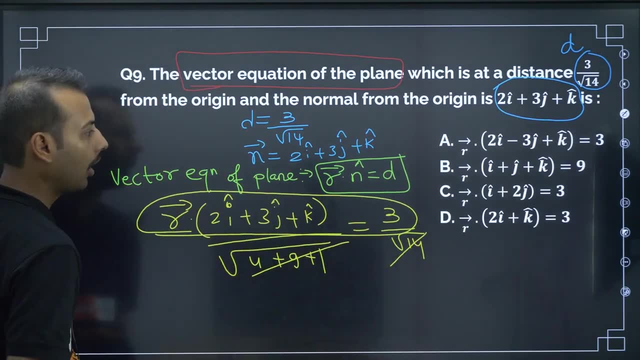 this root 14. to make this n cap, we have to write 4 9 1, 4 9, 1. if I cancel this and this, so we are left with. this is the vector equation of plane r: dot 2, i plus 2, i plus 3 j plus. 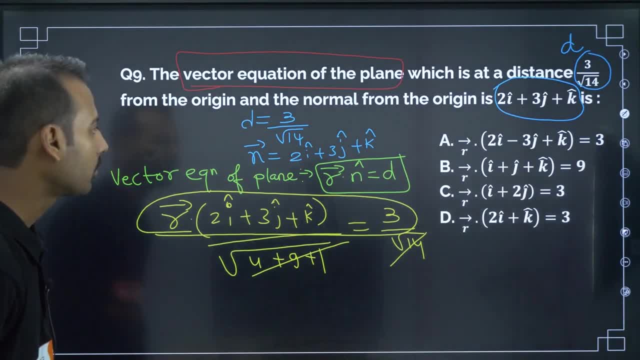 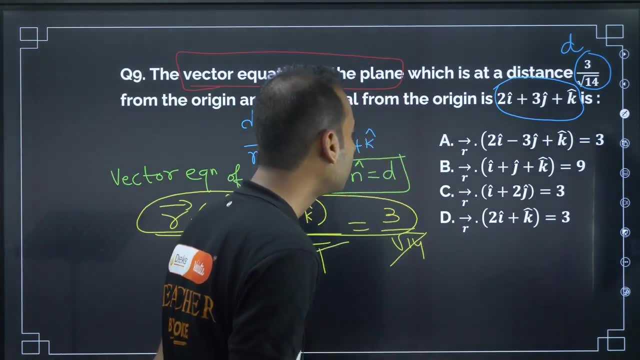 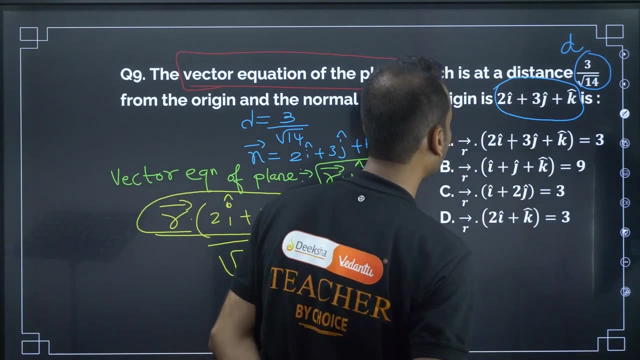 k. So is there any such options? is equal to 3. first option is like this, but there is some mistake in the option, So you correct that it. It should be like this: 2 i plus 3 j plus k cap. So a is the answer we want to next. 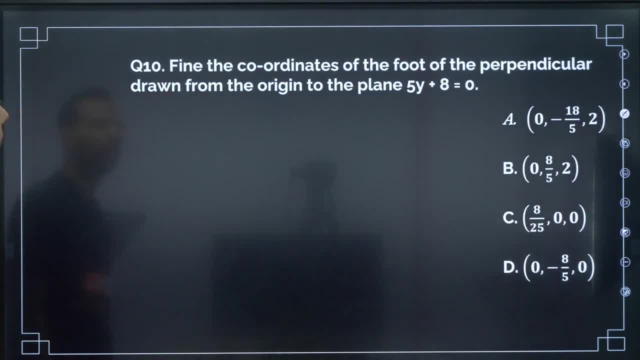 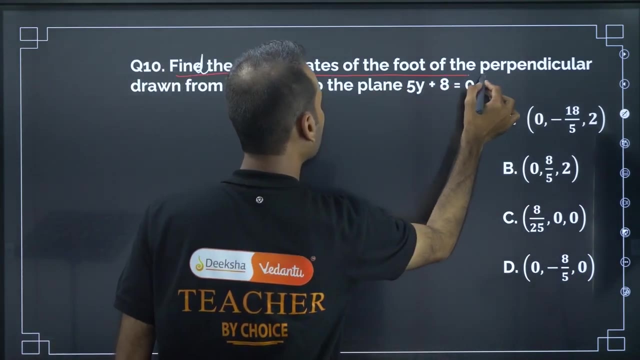 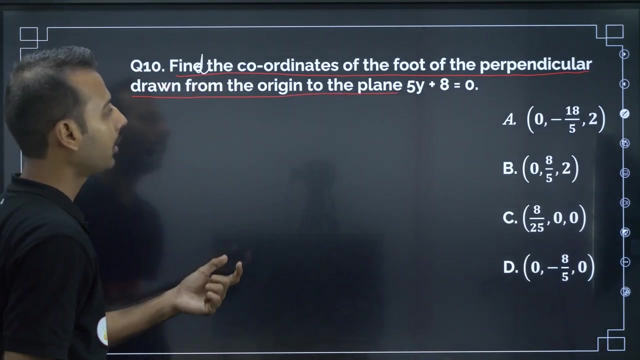 question: find the coordinates of foot of perpendicular drawn from origin to the line. find the coordinates of. what is the question? find the coordinates. we have to find the coordinates of perpendicular drawn from origin. So they are asking to find the coordinates of foot of perpendicular. let me draw the diagram. 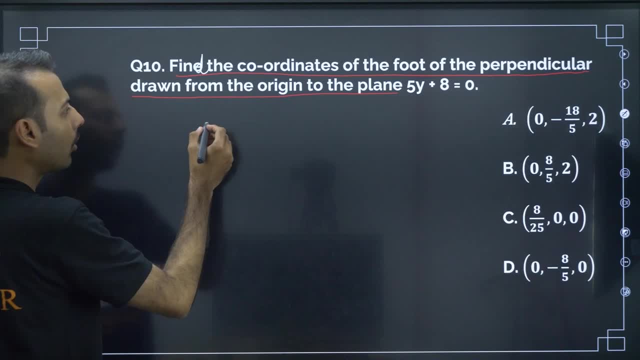 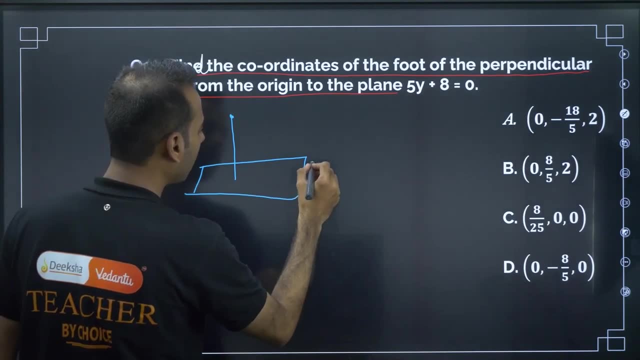 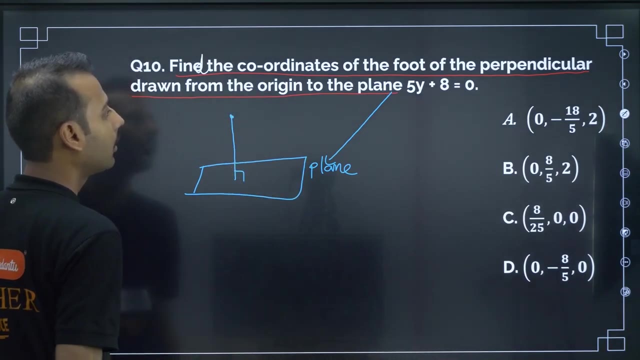 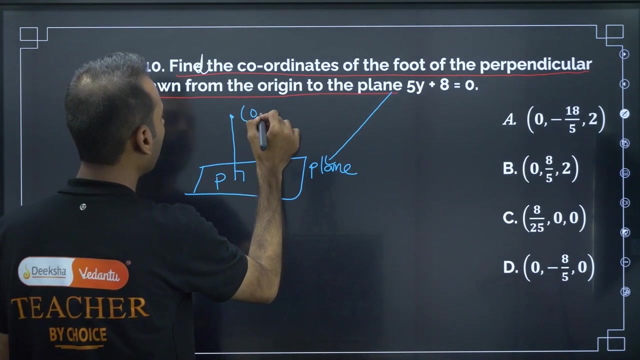 for this, after drawing diagram, we will get. find the coordinates of foot of perpendicular plane. they have considered one plane, this plane. find the coordinates of. find the coordinates of foot of perpendicular p. Let me say this: drawn from origin. they are drawing from origin 0, 0, 0 to the plane this. so find the coordinates. 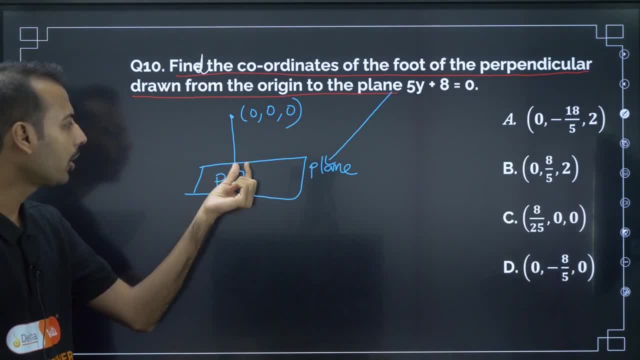 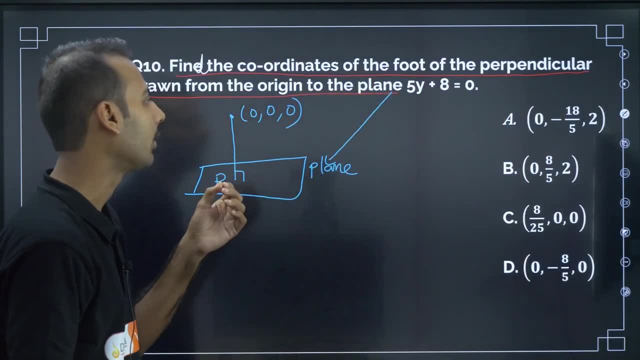 of foot, of perpendicular means. they are talking about this. this point p is lying on this plane. so generally, if i am one student and if i am going to exam, then i will go for option verification, although we can go for normal method also, but it will take lot of time. again, we need to recall the 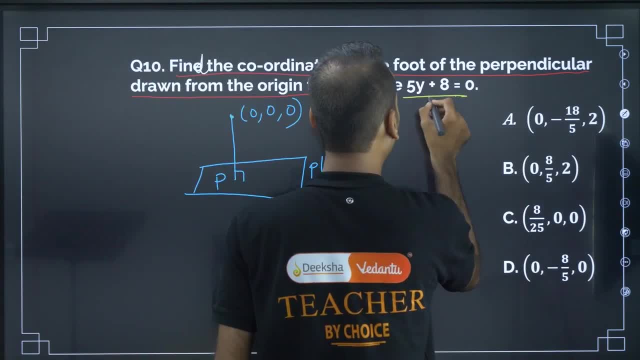 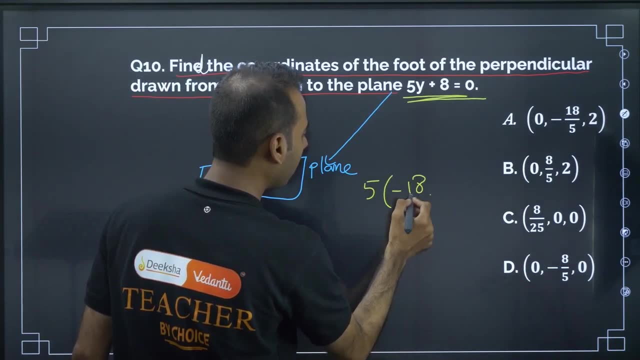 concept, all those things, why all those things? in exam time? 5y plus 8 is equal to 0, so 5y. now, if i go for first option, 5 minus 18 by 5 plus 8, equal to 0. is it possible? not possible, that means a is. 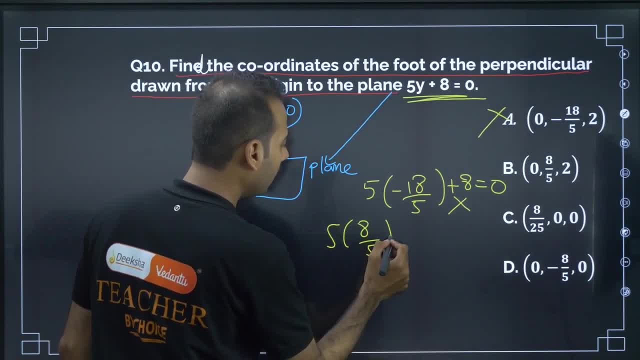 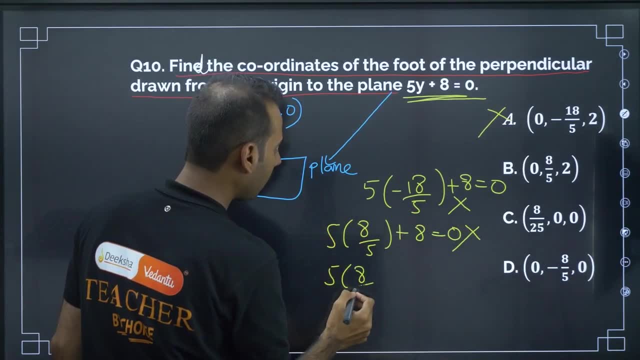 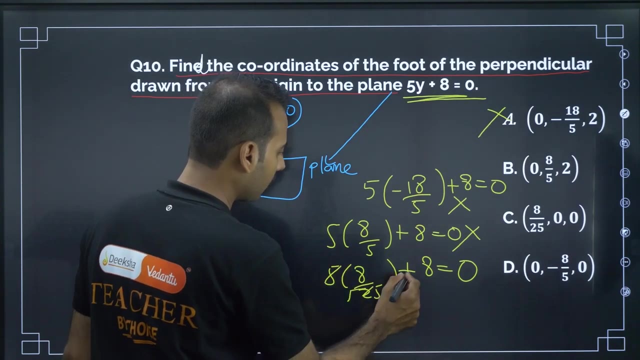 wrong. next 5: 8 by 5. 8 by 5 plus 8 is equal to 0. 5- 5 gets cancelled- not possible. next 5: 8 by 25 plus 8 is equal to 0. is it possible? 5, 5. not possible. so we are left with only one option. d option, ultimately, this: 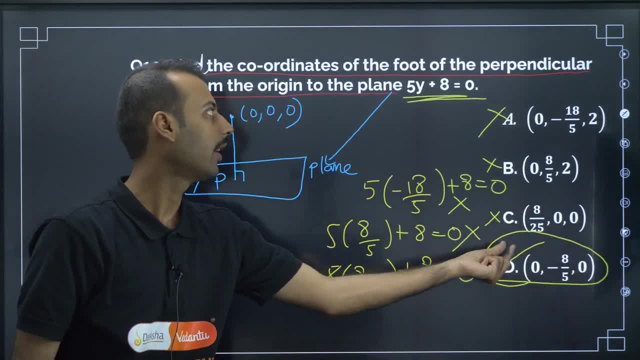 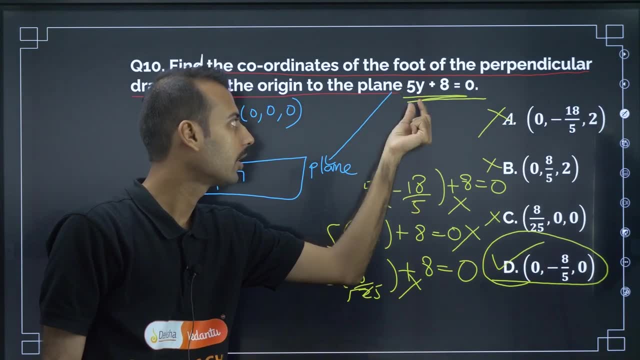 has to be right or i in exam hall. i will not check blindly, i will mark this. but if you want now, for now, you check 0. if you place there is no minus 8 by 5. if you place 5, 5 again minus 8 plus 8 is. 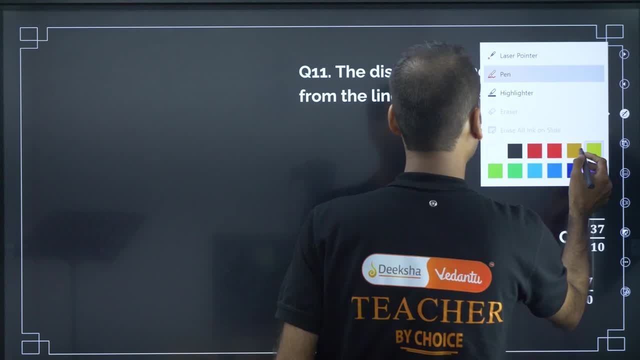 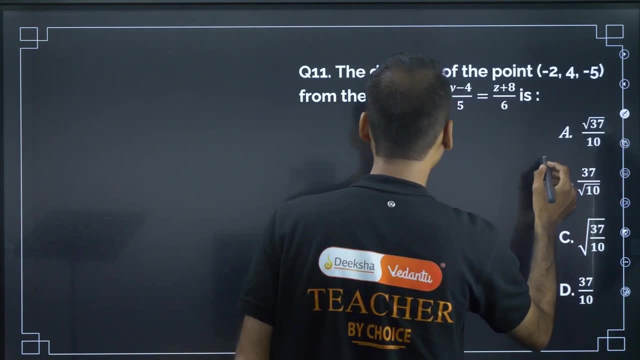 0. so answer is d. moving on to next question. moving on to next question: the distance of the point from the line, the distance of the point from the line, the distance of the point from the line. so what are they asking? they are asking distance of the point from one line. they have given one. 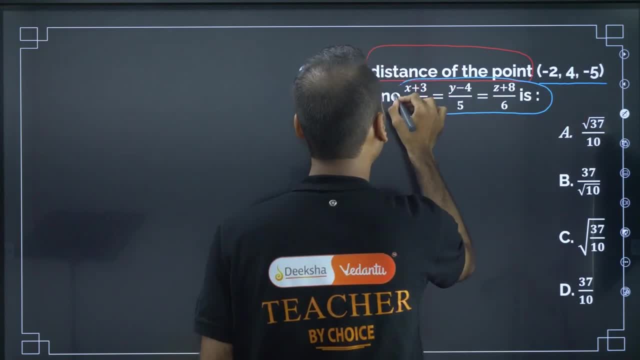 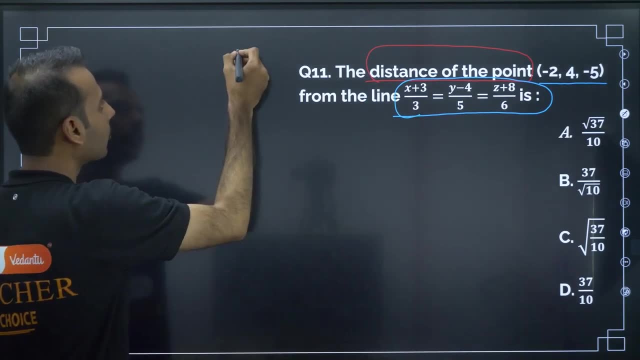 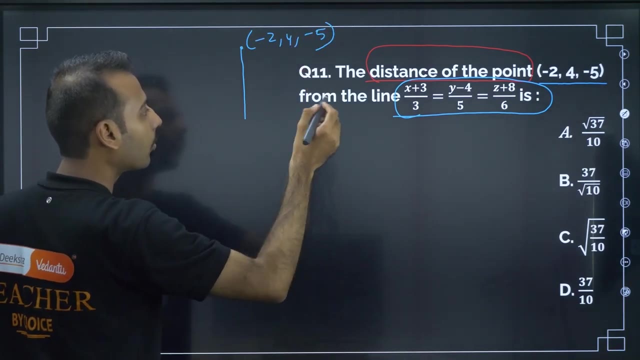 point and one line also they have given. so distance of the point. how to solve this distance of the point? let me draw that diagram. there is one point, what is that? point minus 2, 4 minus 5. distance of the point from line. one line they have considered. what is that? line x plus 3 by 3. 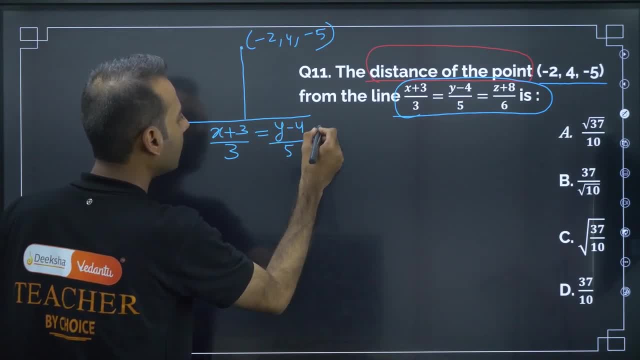 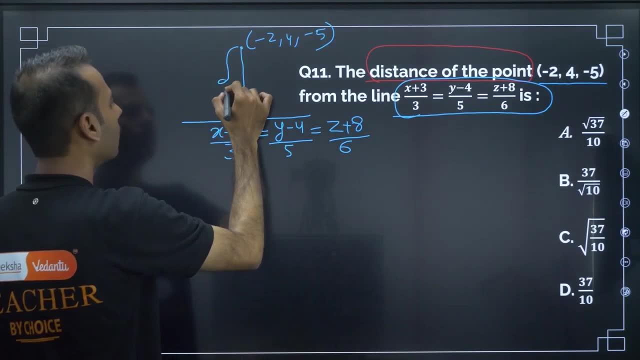 and then a minus 3 and further, and 1 by 3 is equal to y, minus 4 by 5 is equal to z plus 8 by 6, the distance of the point from the line. so they are talking about this distance, distance of the. 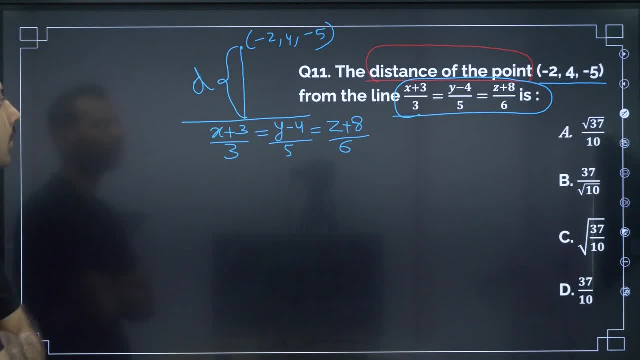 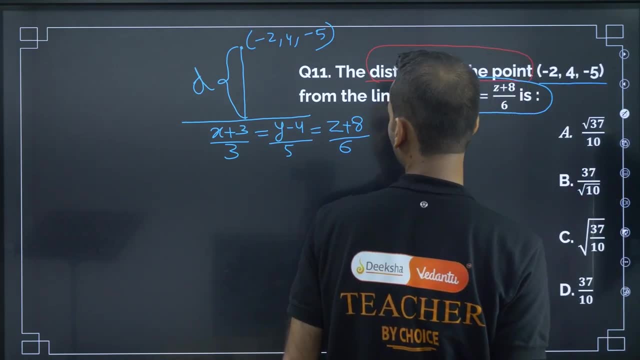 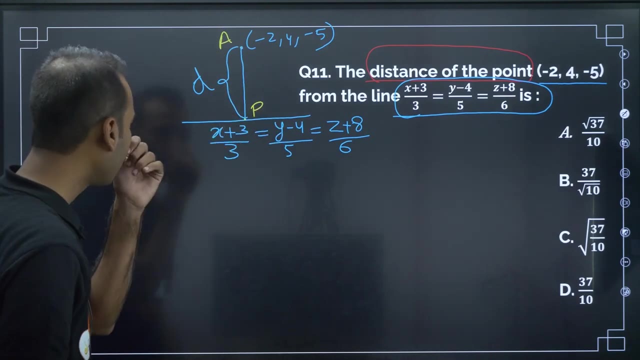 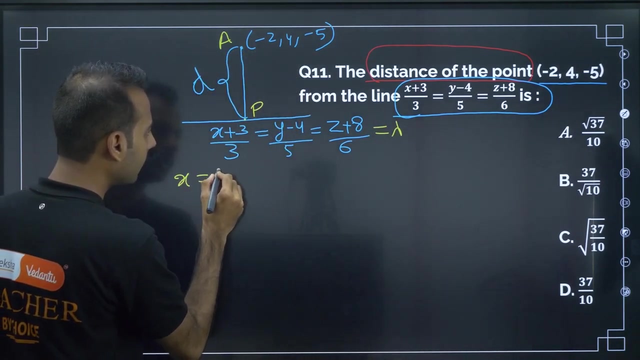 point from the line is: what is this distance? they are asking now how to approach this problem. see, here, let me mark this- says a. let me mark this as some point which is Now: let me equate this to lambda. let me equate this to lambda. So x, x is 3 lambda. 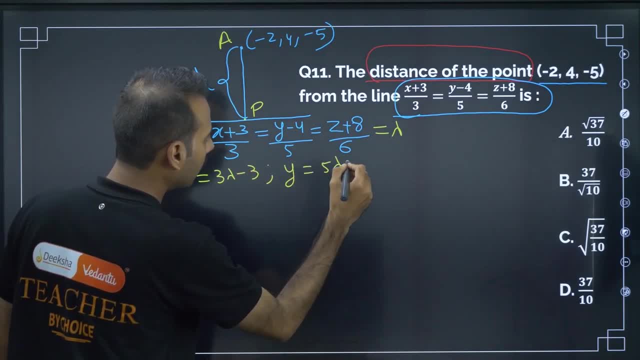 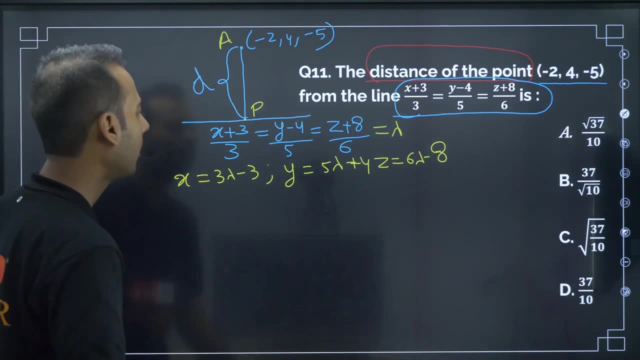 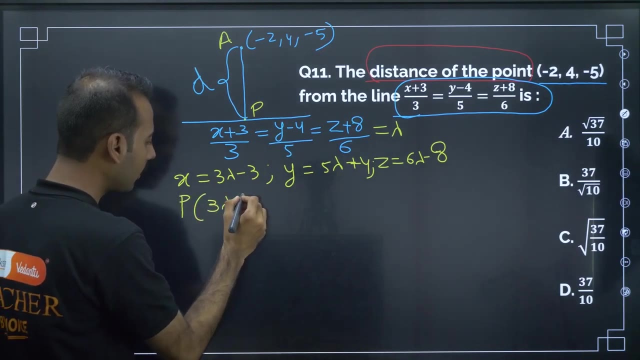 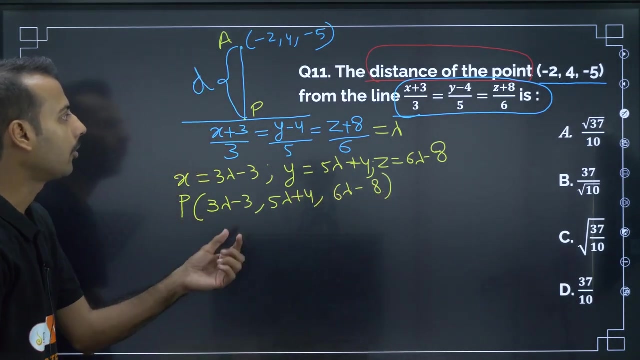 minus 3, y is 5 lambda plus 4, z is 6 lambda minus 8, 3 lambda y is this. So p? p point is 3 lambda minus 3, 5 lambda plus 4 and z 6 lambda minus 8.. What I am doing? I just 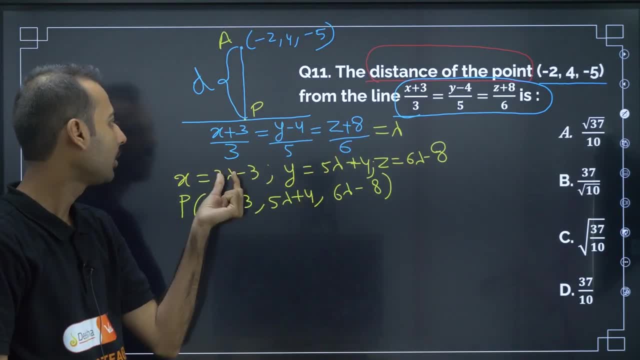 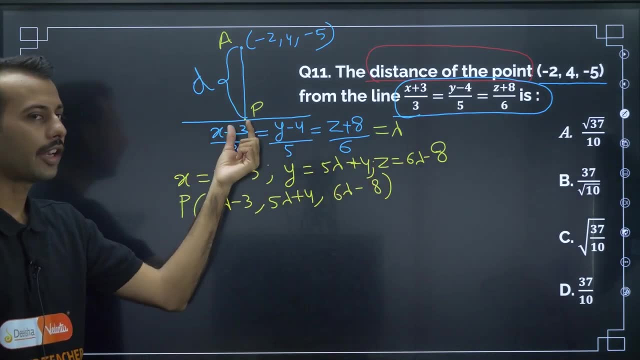 they have given equation that I am equating to lambda, So x will be 3 lambda minus 3, y is equal to 5 lambda plus 4, z is equal to 6 lambda minus 8, that x, y, z means any. 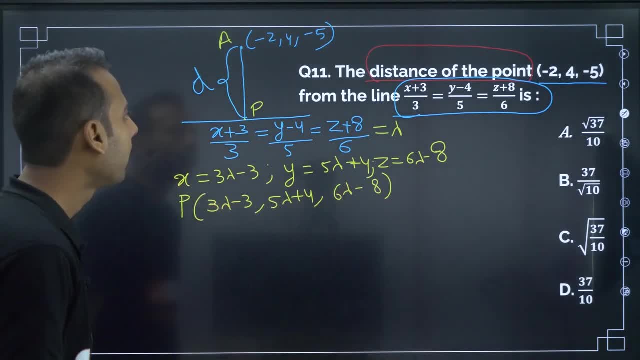 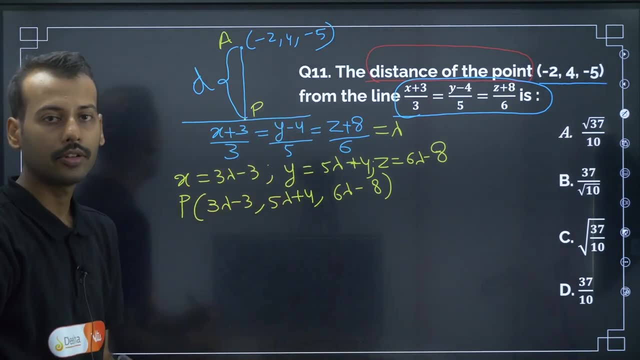 point on this line. So p will be in this form. Now the reason why I am doing this. you go through this because distance of a point from line, this Concept, this topic is very important. multiple questions are there, So now one concept. 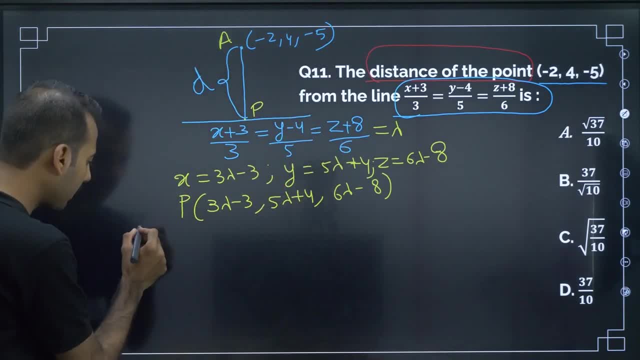 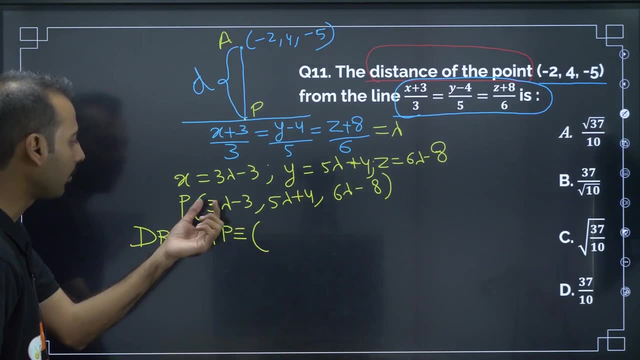 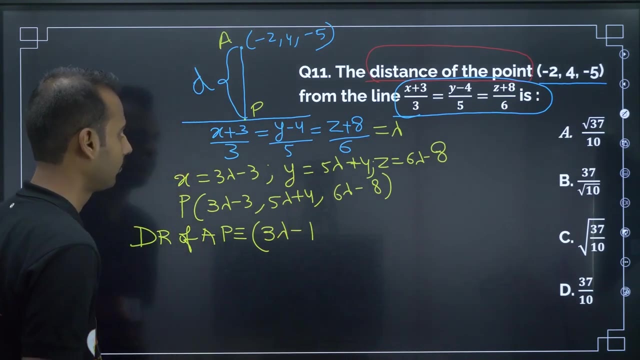 we know what is that concept. If I talk about direction ratios, direction ratios of a p, a p, what are the direction ratios of a p, This minus this, 3 lambda minus this, this minus this? we have to do, Try to recall how to find if two points, a, 1,. 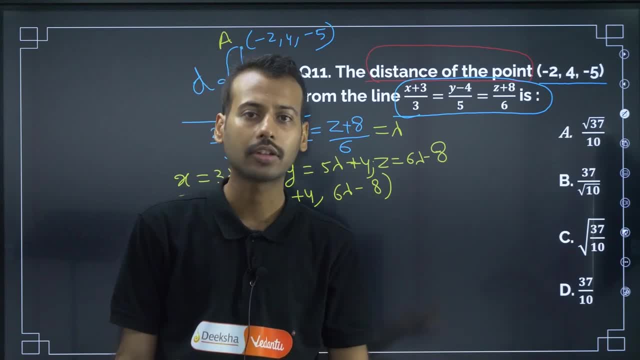 a, x 1, y 1, z 1, b, x 2, y 2, z 2, they are given direction ratios x 2 minus x 1, y 2 minus y 1, z 2 minus. to find direction ratios in node point in NCRT book they have given. 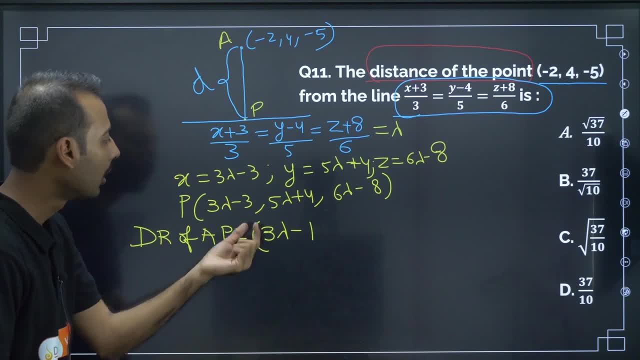 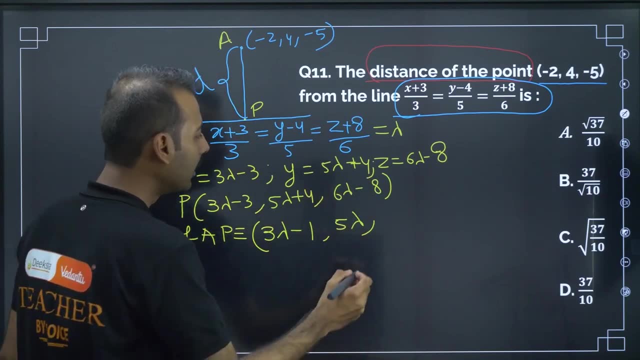 So go through NCRT book if two points are there, how to find direction ratios. Next, 5 lambda plus 4 minus 4.. So 5 lambda, 6 lambda minus 8 plus 5, 6 lambda, 6 lambda minus 3,. 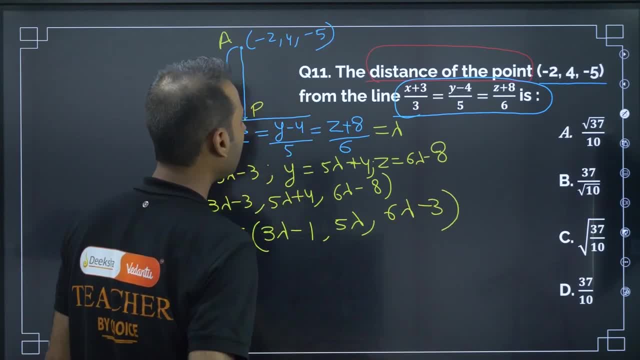 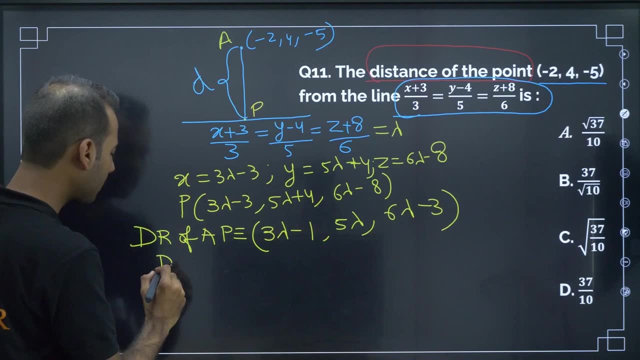 minus 3,, minus 3 plus minus 8 plus 5.. So this is okay, fine. direction ratios of a p. is this? Now, what about direction ratios of line, of a line? direction ratios of a line. 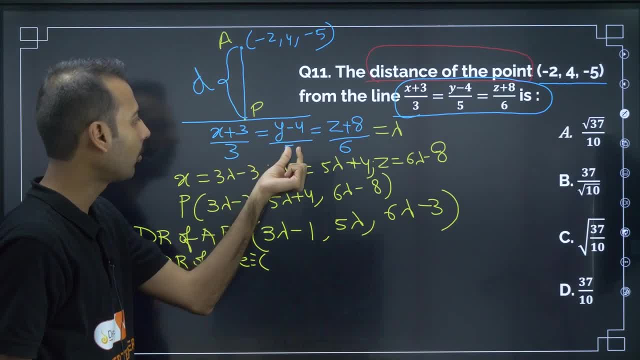 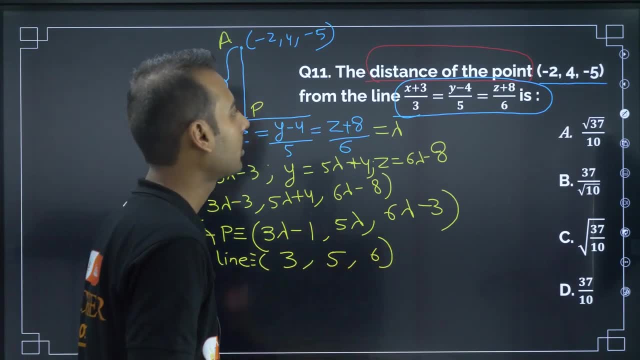 Try to recall straight line, this line concept. this denominator indicates direction ratios, so 3,, 5,, 6.. Now one concept should come to your mind. what is that concept? If two lines are perpendicular, then a 1, a 2, b 1, b 2, c 1, c 2,, b 1, b 3,. c 2, a 1, a 2, b 1, b 2, c 1, c 2, b 1, C 1, c 2, a 1, a 1, b 1, b 1.. 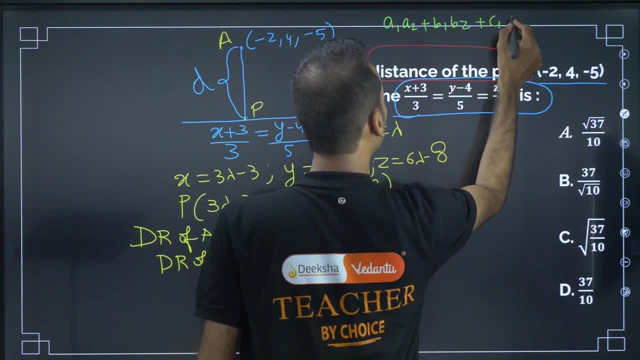 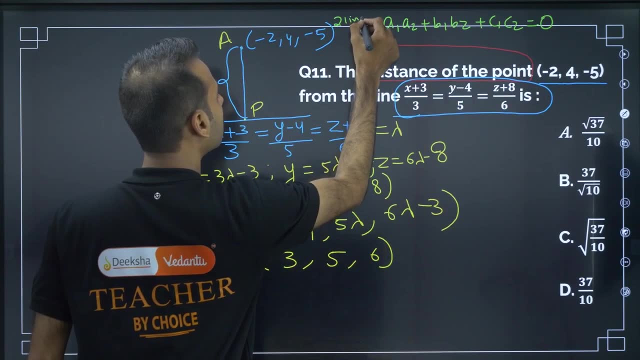 If two lines are perpendicular, then if a 1, a 2, b 1, b 2, c 1, c 1, c 2, c 1, b1, b2, c1, c2 is equal to 0, two lines are perpendicular, two lines are perpendicular. 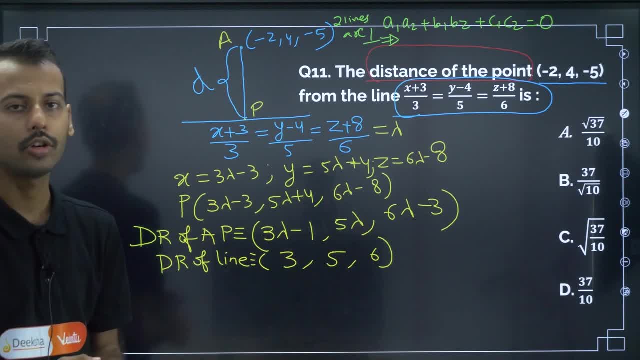 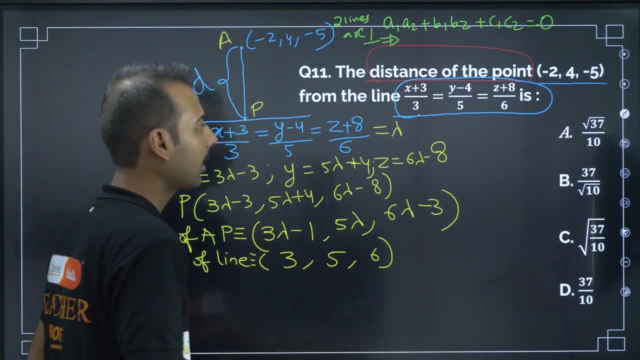 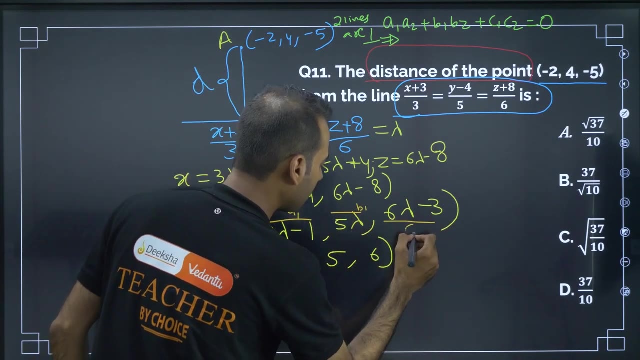 then this is the condition. this condition- in one of my previous videos i already discussed this- is very important. again and again, we have to discuss this. you should be knowing now if i mark this as a1, b1, c1, a2, b2, c2, if i mark this as a1, this as b1, this as c1, this as a2, b2 and c2, and if i 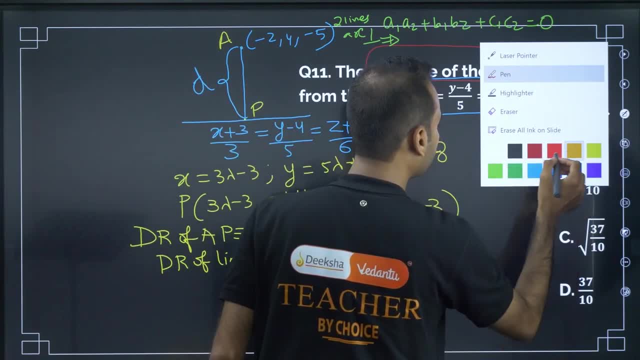 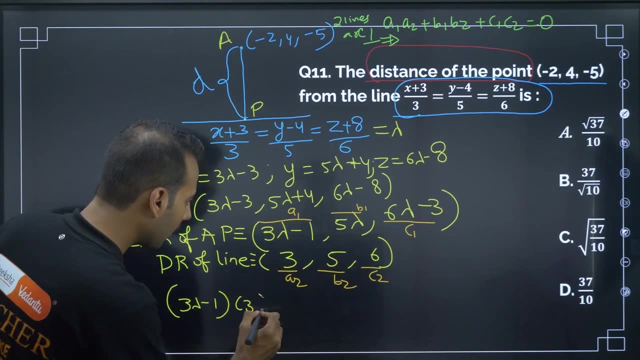 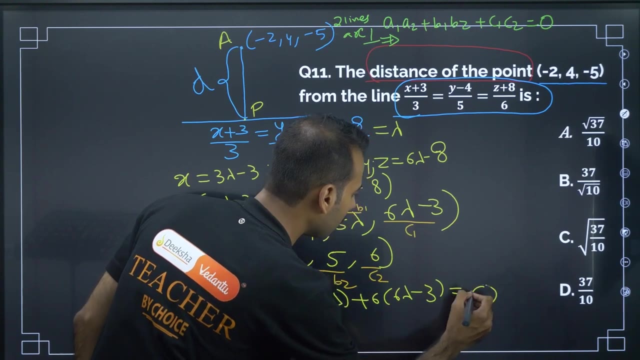 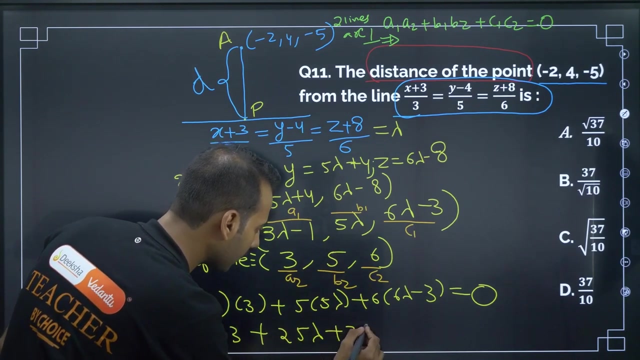 substitute in that. if i substitute in that, then i am going to get a1, a2, b1, b2, 3 lambda minus 1, 3 plus 5, 5 lambda plus 6, 6 lambda minus 3 is equal to 0. so 3 lambda 3, 3 is a 9 lambda minus 3 plus 5, 5 is a. 25 lambda plus 6, 6, 36 lambda minus 6, 3 is 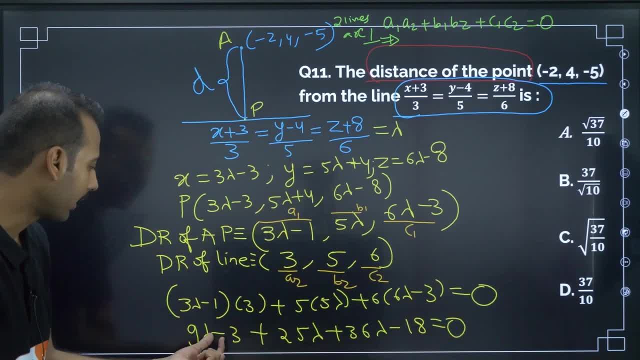 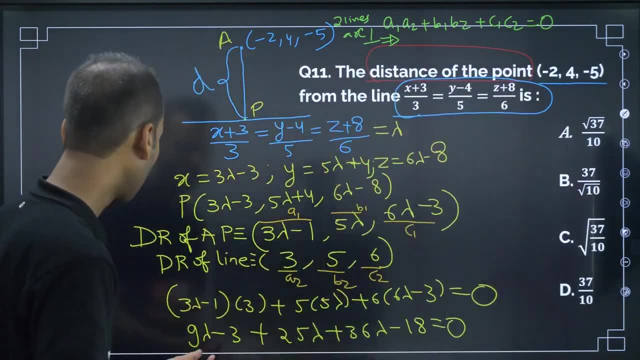 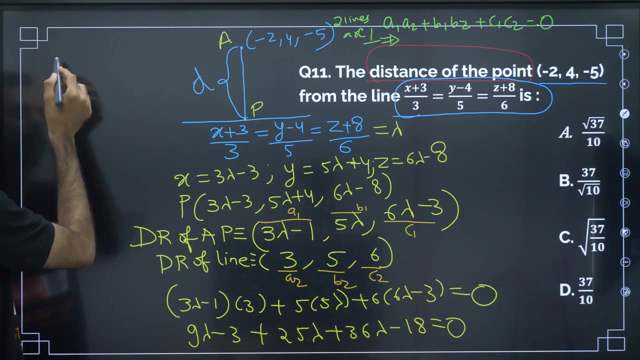 a 18 is equal to 0. now if, from here, if i find 9 lambda, 25 lambda, 70 lambda, let me remove few things to simplify this, or else, after simplifying this, shall i remove few things or shall i write here. i am writing here because, anyways, again, that might also be 9 lambda 25. 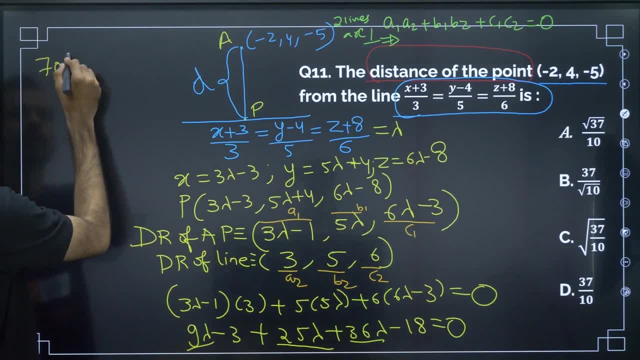 lambda, 36 lambda. this is equal to 70 lambda, 70 lambda and then minus 3, minus 18, minus 21. if i transpose to other side is it becomes plus 21. 21 can be written as 7 into 3 and this can be written. 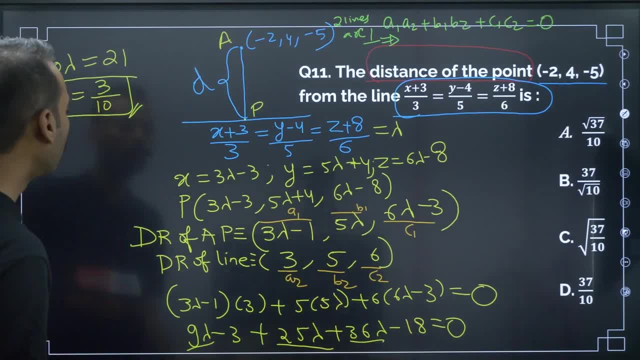 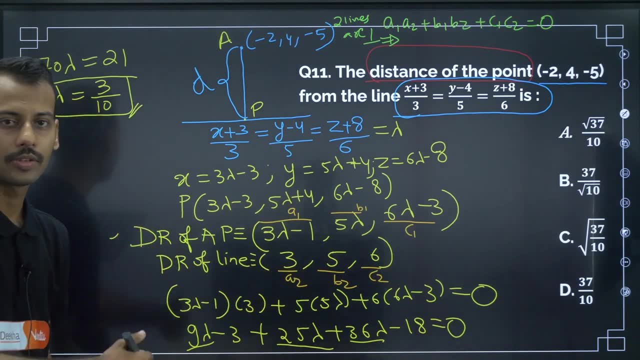 as, so lambda is equal to 3 by 10.. now, p point is this. p point is this: 3 lambda minus. let me remove all this. if you want to make a note of this, make a note of this, or if you want to take screenshot. 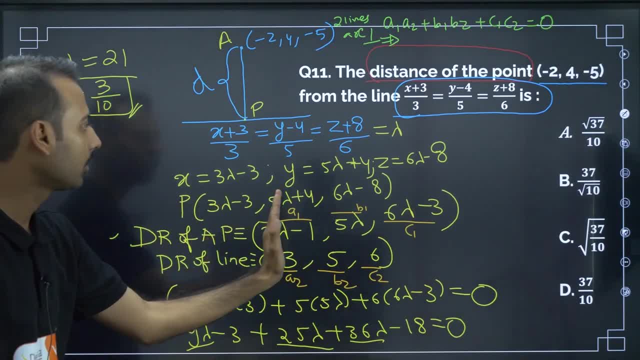 you take screenshot, it is up to you. lambda value is equal to 3 by 10 and this is equal to 3 by 10, is this? i am removing these few things from here, so lambda value is this, so let me write p 3 lambda. 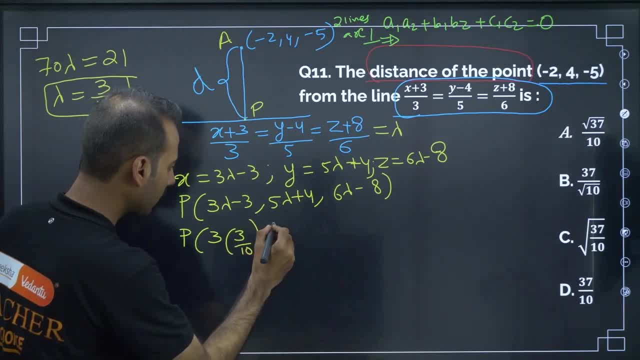 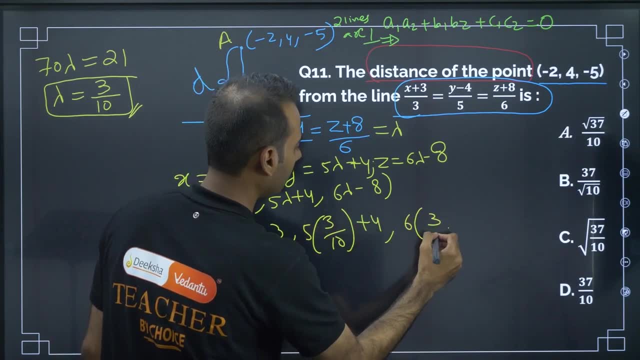 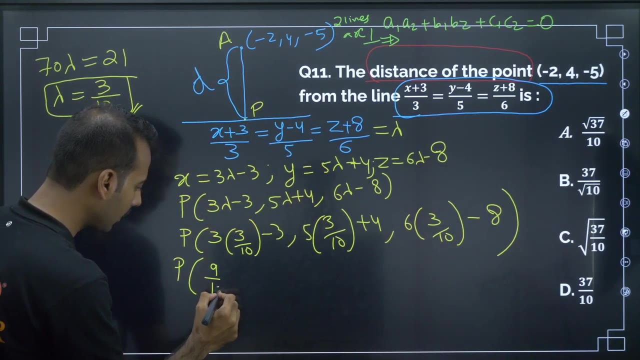 value is 3 by 10, 3 by 10 minus 3, comma 5, 3 by 10, 3 by 10 plus 4, comma 6, 3 by 10 minus 8. next for p: 9 by 10. just simplification, nothing much creative. five ones are five, twos are: 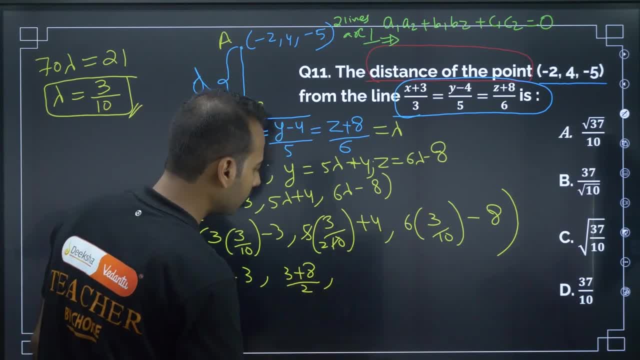 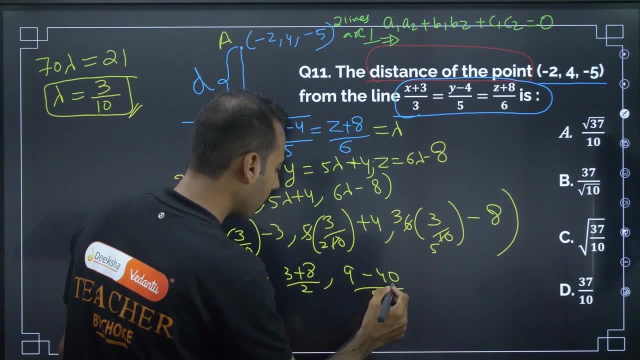 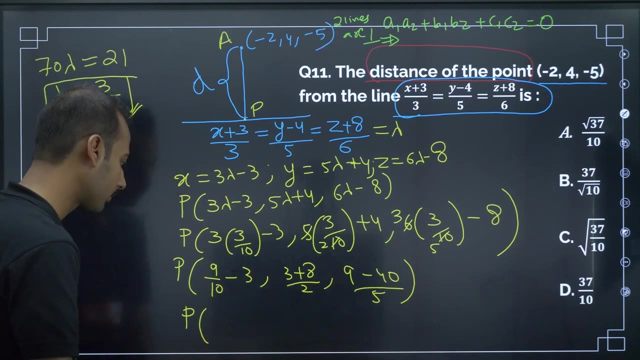 three plus eight by two. next for this, if i write three, for this, if i write five, three, three is a nine minus forty by five, so p can be written as nine minus thirty. nine minus thirty is minus twenty, one by ten comma, eleven by two, and that is minus thirty one by 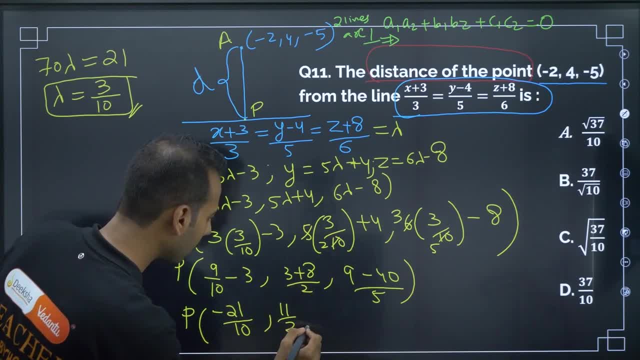 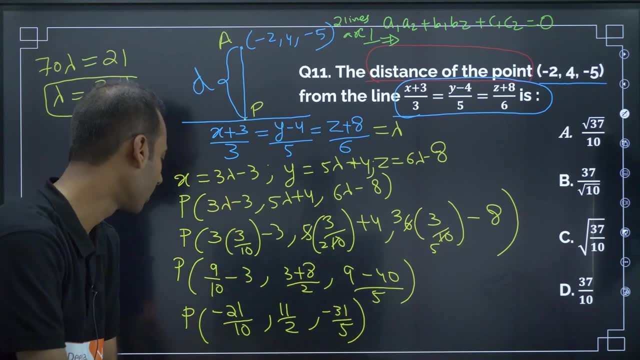 ten comma, eleven by two, and that is minus thirty one by two, and that is minus thirty one by two and that is minus 31 by 5 minus. check all the numbers whether they have, whether they are correct or not. p, p value. i am getting 9 minus 30 by 10, minus 21 by 10, 3 plus 8 by 2. okay, 9 minus. 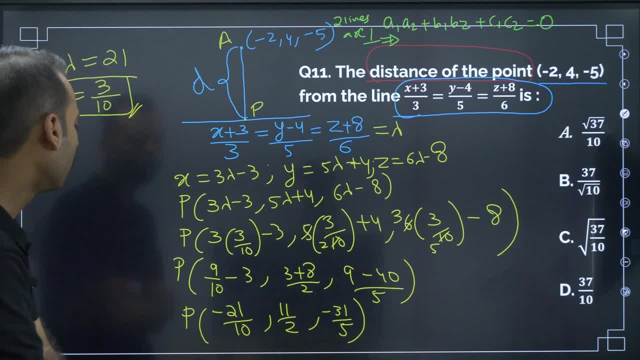 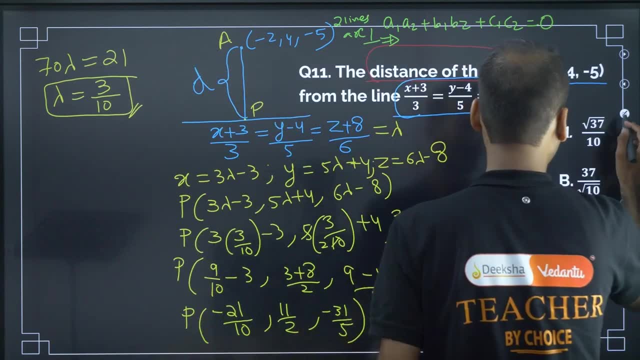 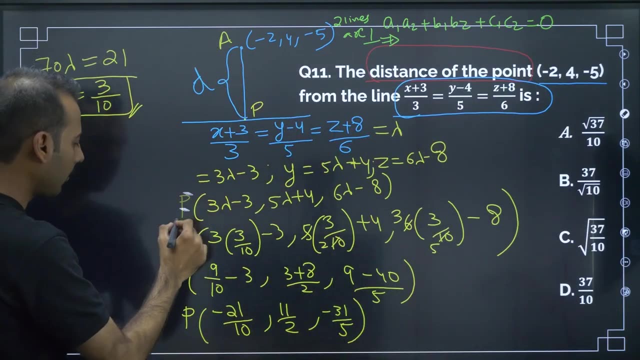 40 by 5, 1 by 11 by 2. okay, all this is fine. so if any calculation mistake, addition subtraction might be mistake, apart from there will not be any mistake. concept is this only next? let me erase few things. what things i will erase? let me erase all this. so finally we got p. 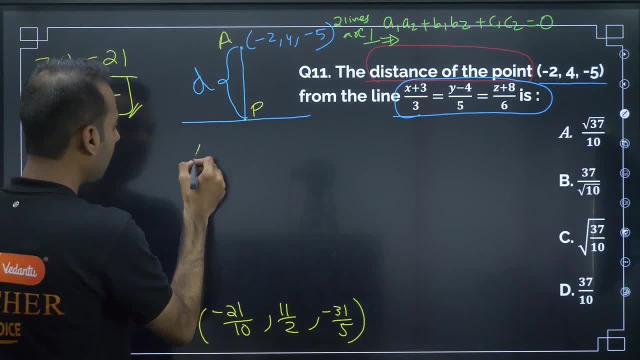 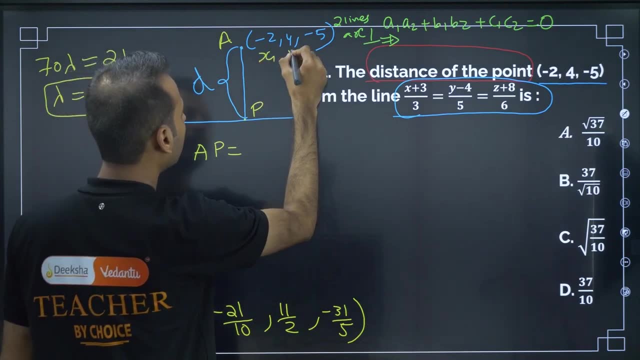 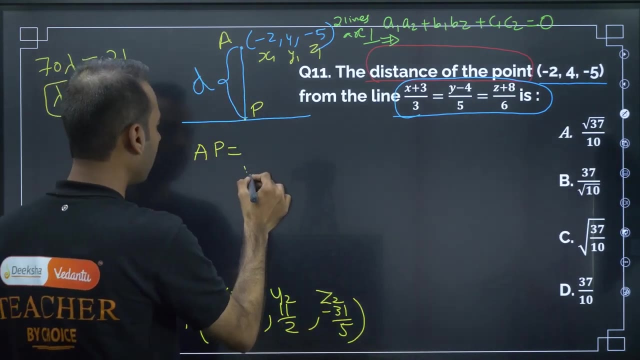 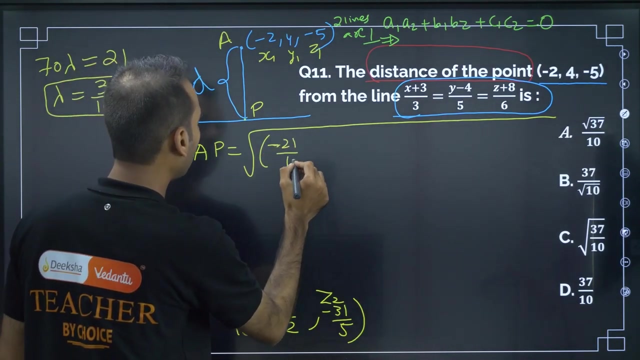 p, we got this, a, we got this, so a p, a p is equal to, a p is equal to. if i mark this as x1, y1, z1, if i mark this as x2, y2, z2, so under root of a p is equal to under root of x2 minus x1. x2 is minus 21 by 10 minus x1 is 2 square plus y2, y2 is: 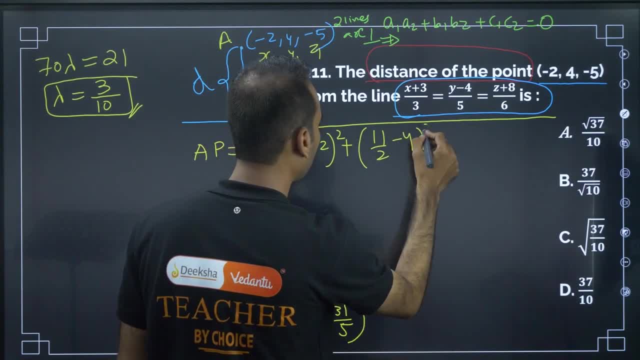 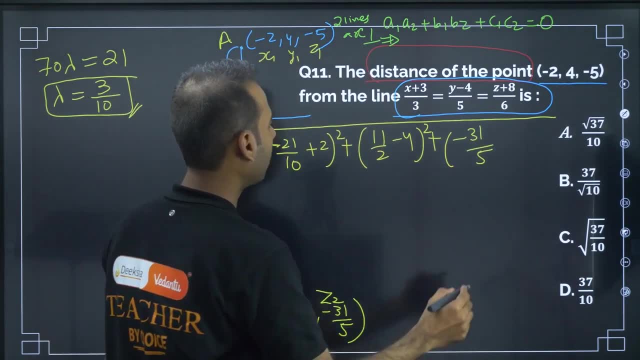 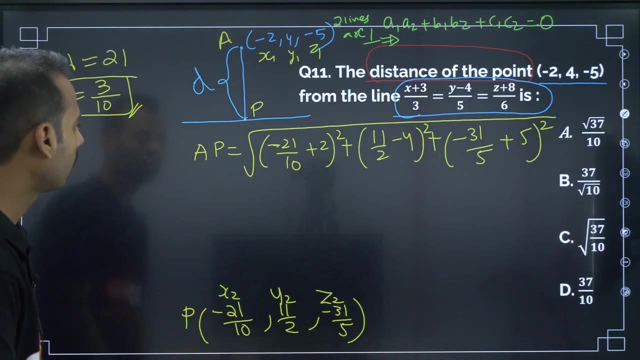 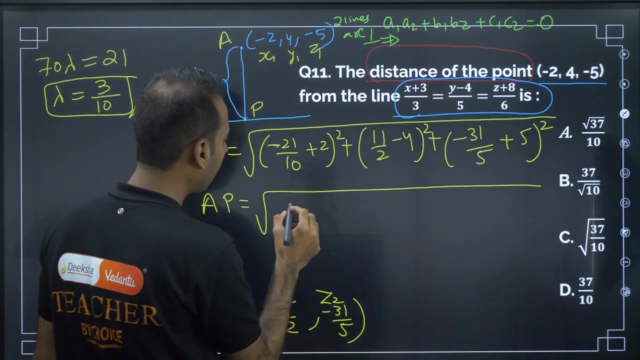 11 by 2. 11 by 2 minus 4 square plus. z2 is minus 31 by 5, 31 by 5 plus 5 pi square. so next: ap is equal to. ap is equal to root of 21 plus 20 is minus 1 by 10, square plus. 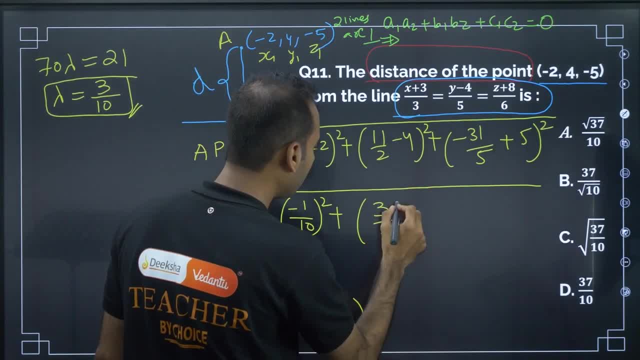 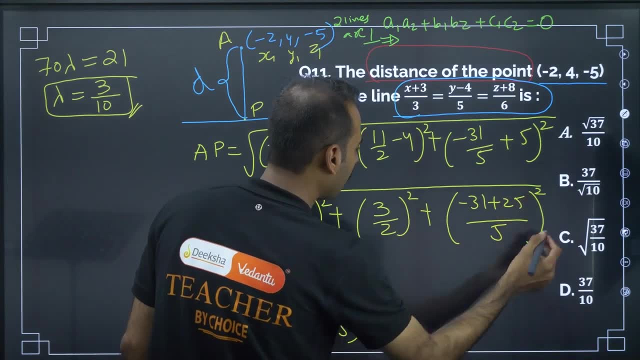 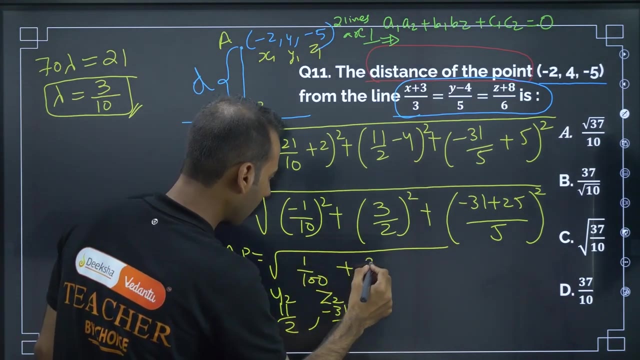 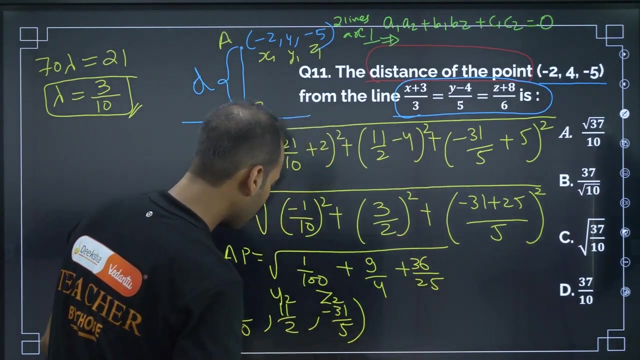 11 minus 8 is 3 by 2 square plus 31 plus 25 by 5 square. so ap is equal to is equal to 1: 1 by 100 plus 9 by 4 plus 6 by 636 by 5 square is 25.. So further, if I go for further simplification, 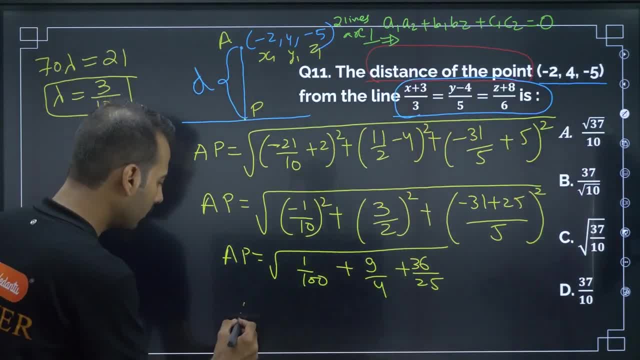 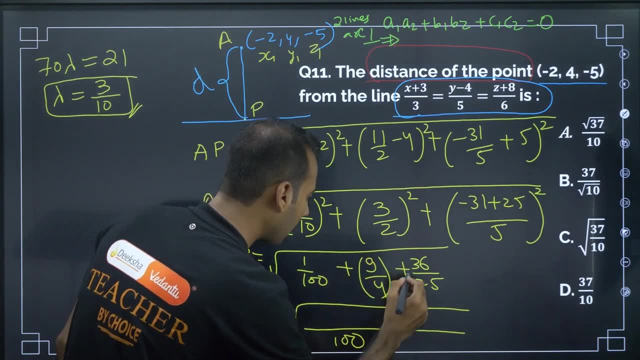 let me remove the things Now. if I take LCM, if I take LCM, AP is equal to under root of here, LCM is 100. So I have to multiply this with 4 and this with 25.. Now this becomes 1 plus. 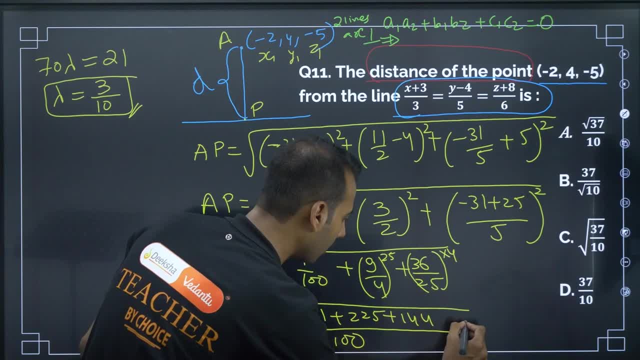 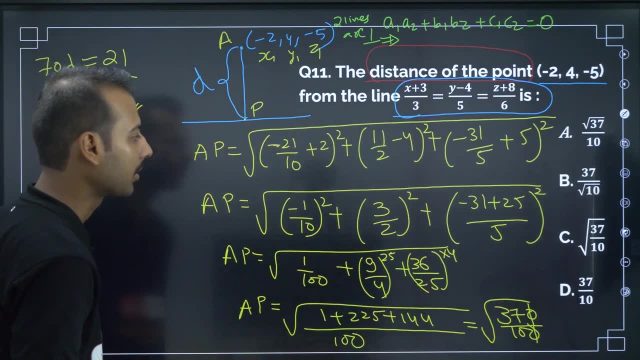 225 plus 144. this is equal to under root of 370 divided by 100. So 0 and 0. if I cancel root 37 by 10, c is the answer. Moving on to next question, The perpendicular distance of the point. 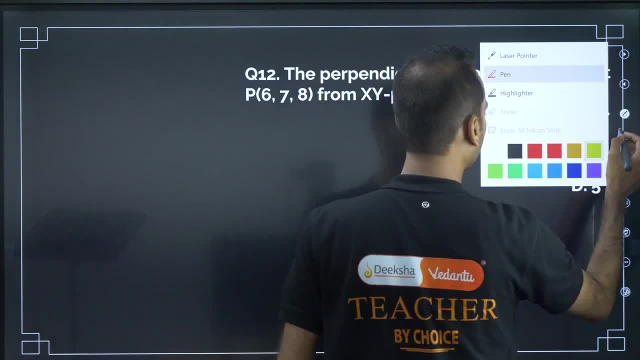 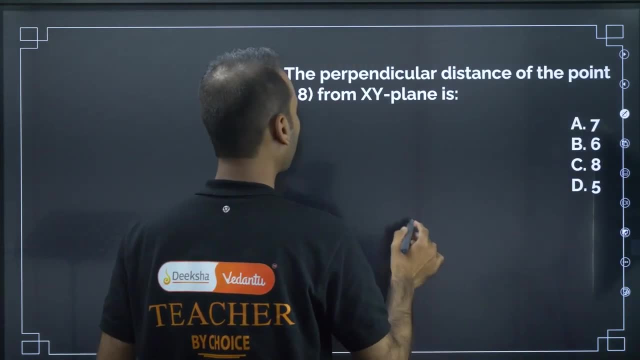 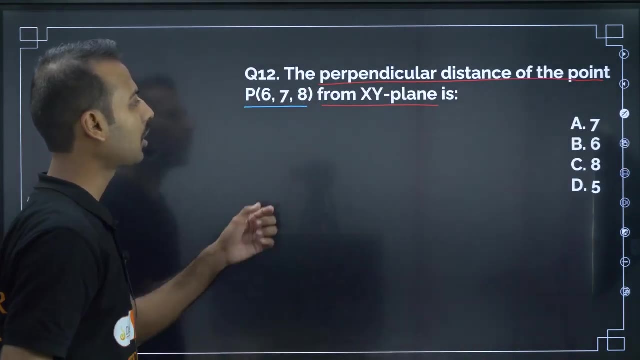 from x y plane is very easy question just based on synopsis only and based on theory knowledge only. we have to solve this. The perpendicular distance of point from x y plane is very easy question just based on synopsis only, based on theory knowledge only: from x y plane. they have given some point: perpendicular distance of this point from. 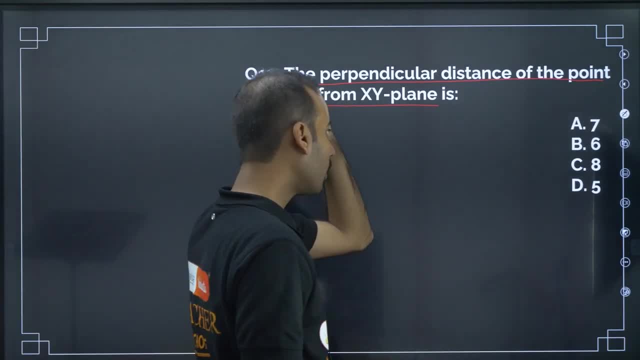 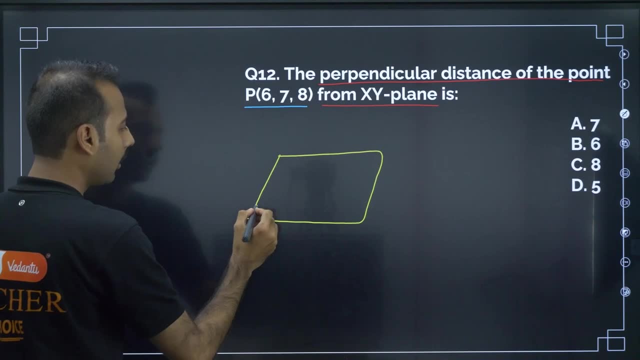 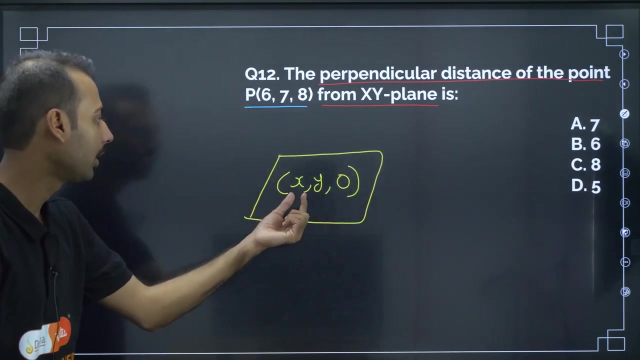 x y plane is Now in x y plane, so in x y plane let me draw x y plane. in x y plane we are having some x values, some y values and z value is for sure 0 in x y plane. this is the perpendicular distance of this point. one point is there: 6, 7, 8.. 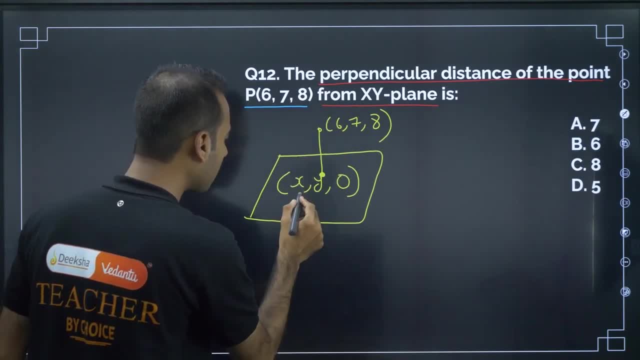 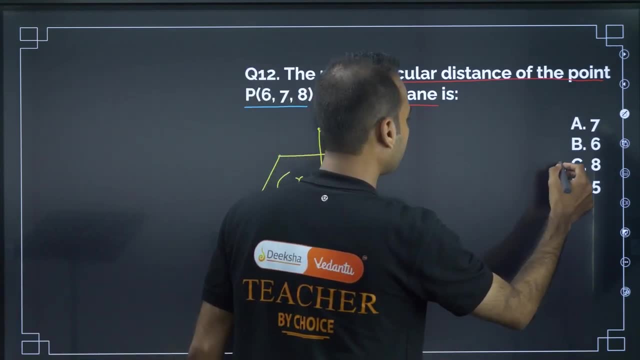 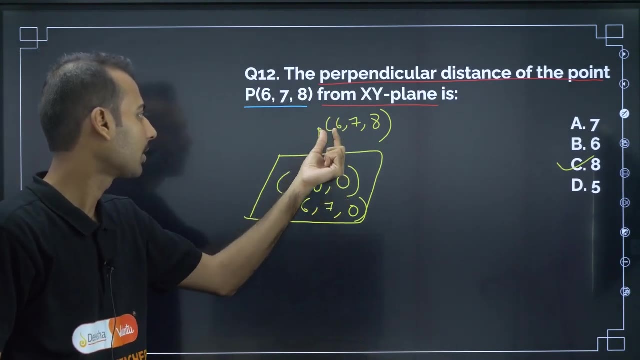 They are talking about perpendicular distance. perpendicular distance means 6, 7 and 0.. Now if you take distance formula, you will get answer as 8 8 is the answer, or else directly. also we can see here using distance formula directly we can do: x 2 minus x 1. x 2 minus x 1 square is 0 square. 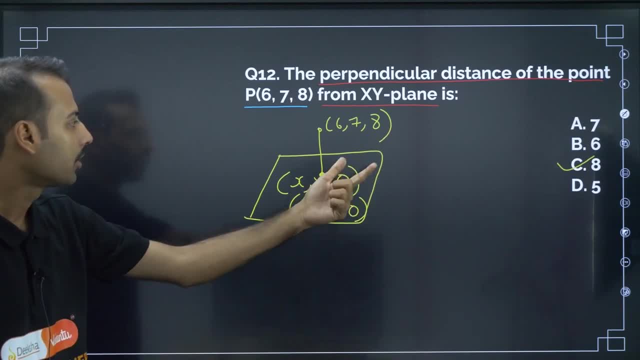 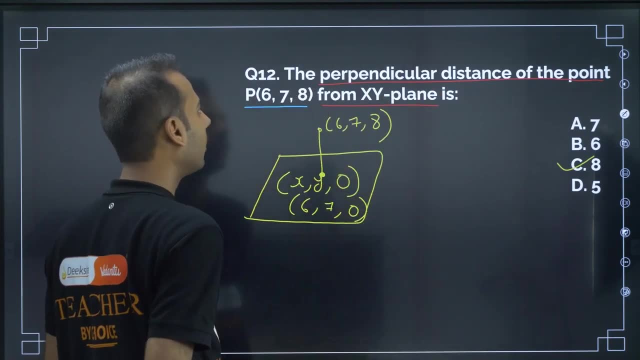 0 square and this is root of. So perpendicular distance is 8. very easy question if such question comes just within seconds, within 10 seconds. So this is the answer. So this is the answer, So this is the higher, the Olympic flower playing only when into chronic training Mu. 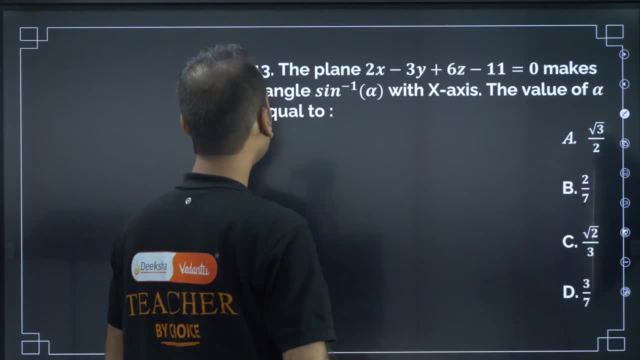 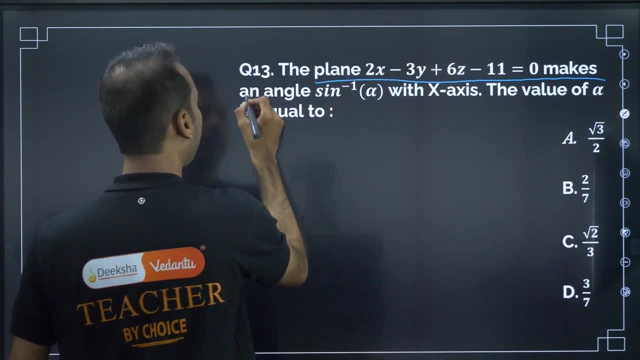 Wa at饺 16 seconds or within five, only marking time it will take. So such questions nobody should do. going on to next question: the plane makes an angle of sin inverse. So some information they have given the plane there is: 1. plane makes an angle of sin inverse. you already. 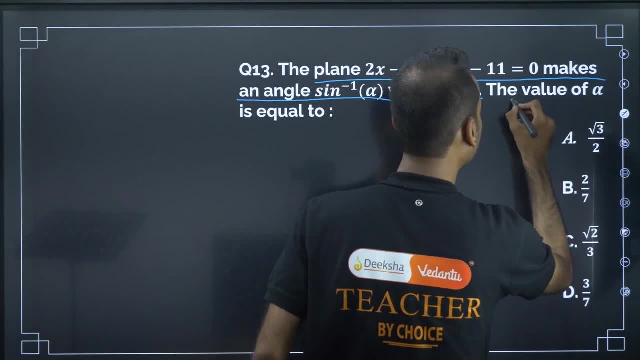 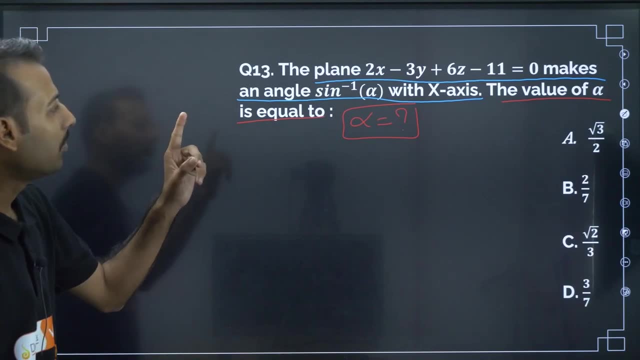 alexis, the value of alpha is equal to. So what are they asking? the value of alpha is equal to. they want value of alpha alpha value. there the plane makes angles, sin alpha with x Malchus. so and in can say that in this. how so? Nava will be a Video on, just like. 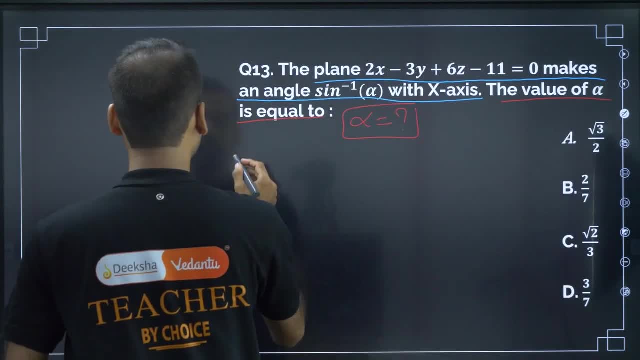 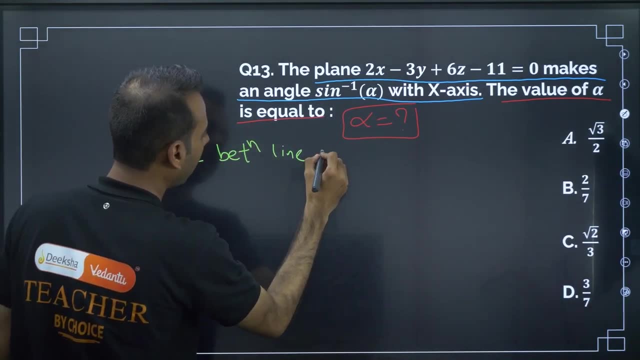 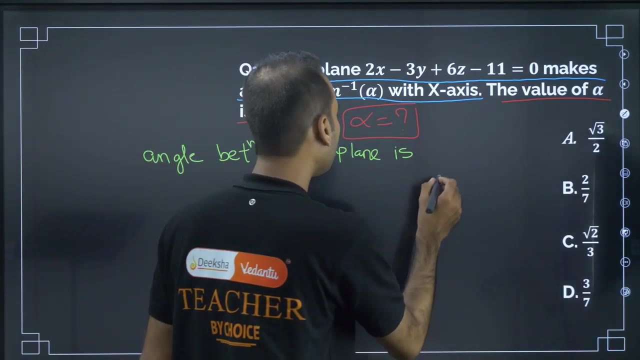 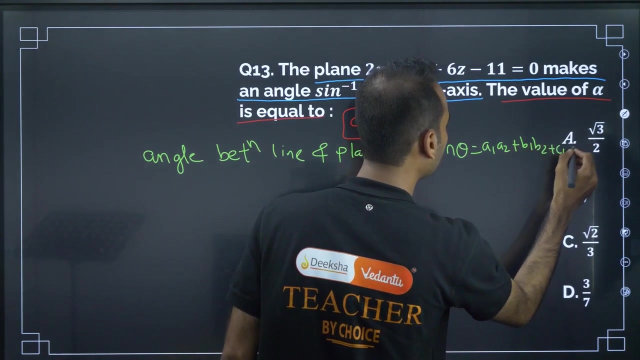 you have some cinfashion or video, you have some in letter, such as: okay. So what is that? to recall synopsis. synopsis: angle between angle between line and plane. angle between line and plane is angle between line and plane is sin. theta is equal to a1, a2, b1, b2, c1, c2. 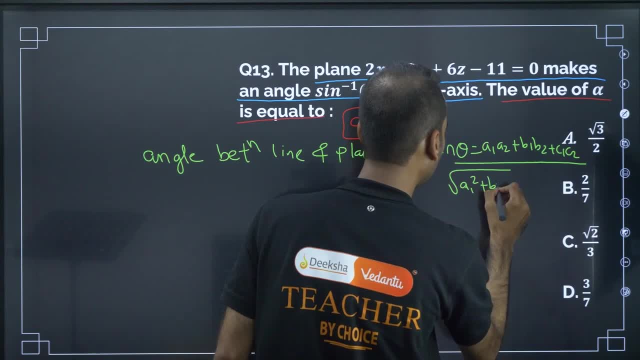 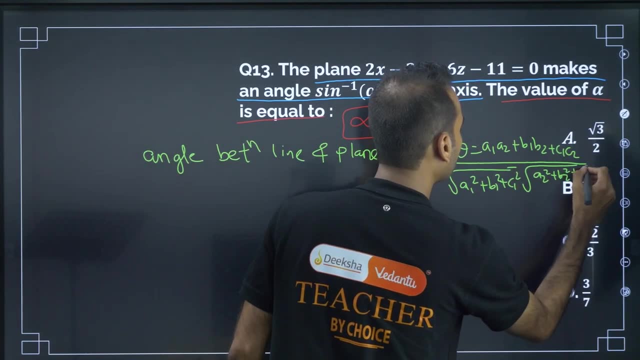 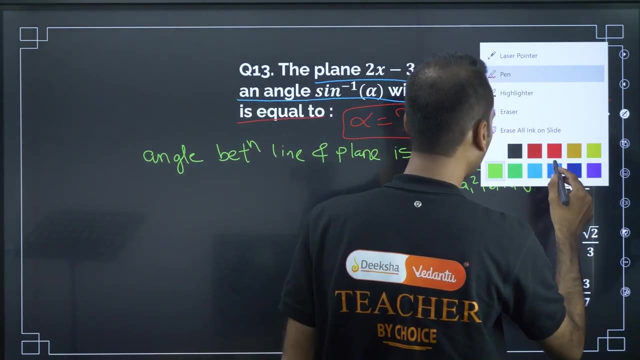 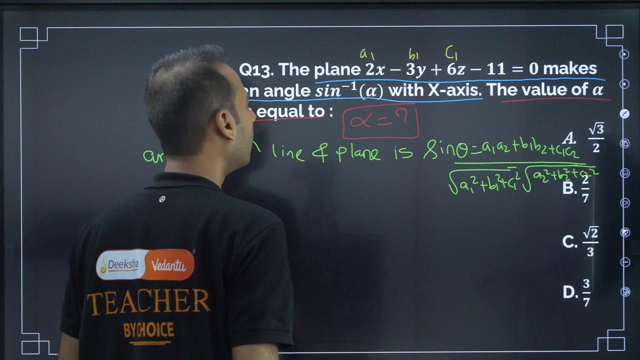 by root of a1 square, b1 square, c, of a2 square, b2 square, c2 square. this synopsis point you should be knowing now. also few more things you should be able to recall at this point of time. that is a1, is this b1, is this c1, is this makes an angle with x axis for x axis. 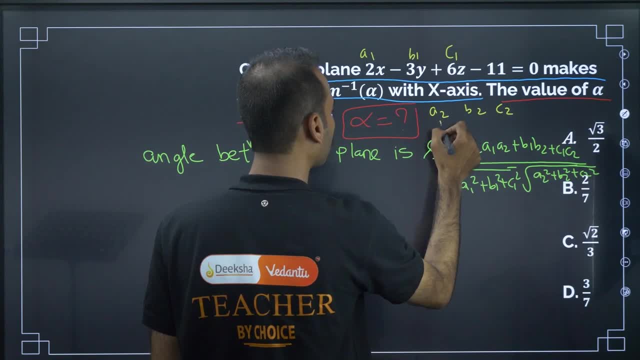 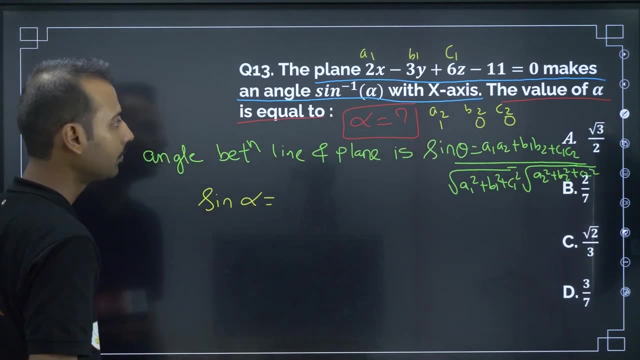 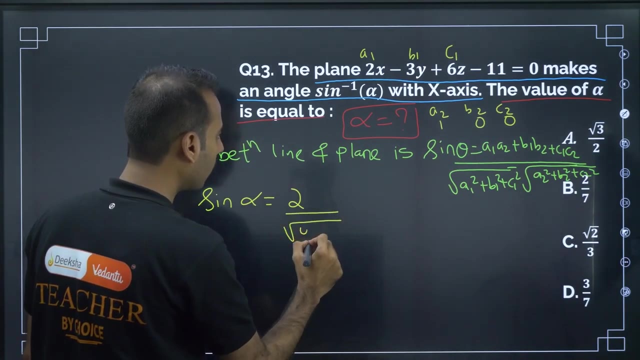 a2, b2, c2.. Then ratios will be 1, 0, 0. now sin theta here that angle is sin alpha. that is equal to a1- a2. if you multiply b1, b2, c1, c2 by root of a1, square 4, 9, 36 by root of this is 1, so this: 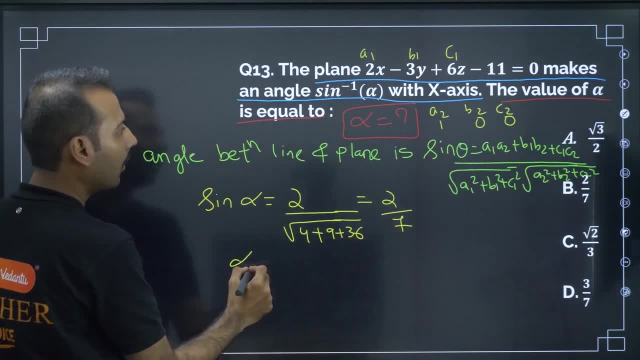 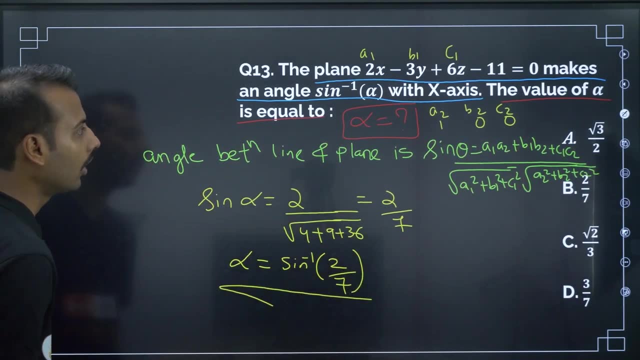 is equal to 2 by 7. now alpha. alpha is equal to sin inverse of 2 by 7. so what are they asking? value of alpha is equal to angle. angle is sin inverse 2 by 7, sin inverse 2 by 7 makes: 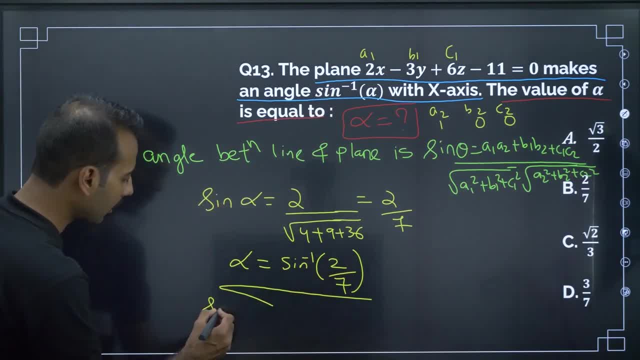 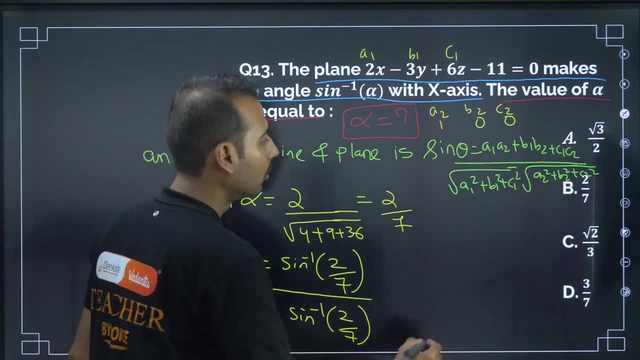 an angle. What is this angle Angle? they have given as sin inverse alpha. sin inverse alpha is equal to this sin inverse of 2 by 7. that means alpha is equal to 2 by 7, c is the answer, moving on to next question. 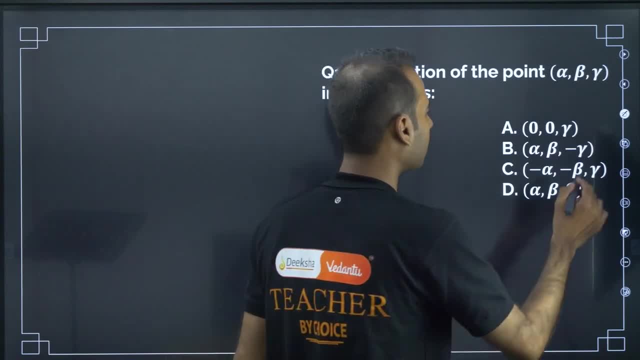 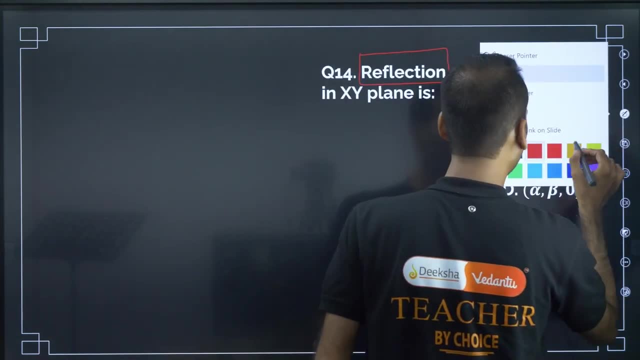 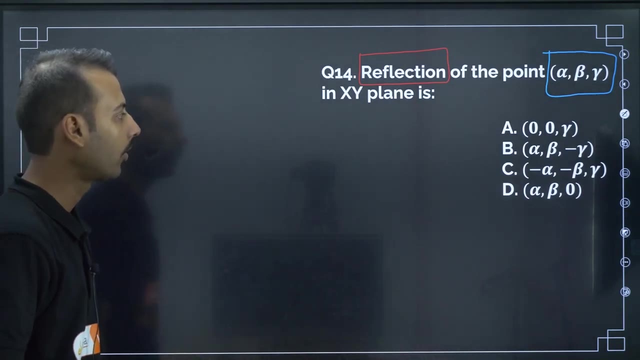 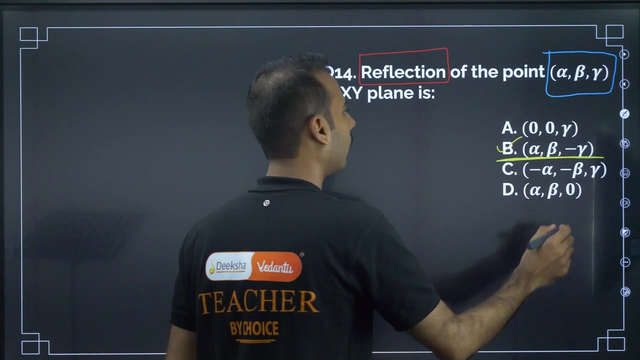 The reflection of the point. alpha beta gamma in xy plane is So the question is: they want reflection, reflection of the point, of which point alpha beta gamma of alpha beta gamma in xy plane is. So alpha beta gamma? answer is alpha beta minus gamma. alpha beta minus gamma. 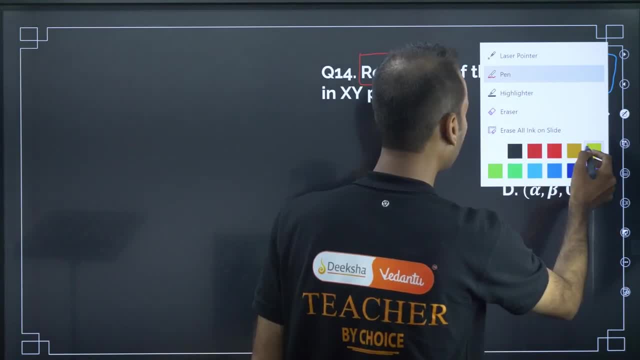 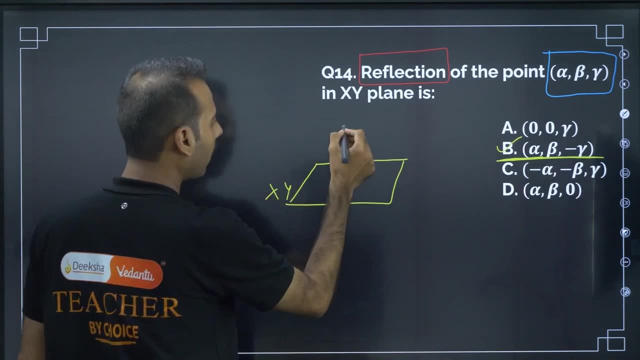 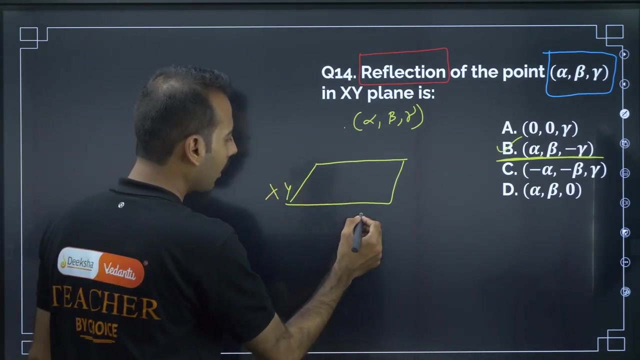 You should know this, you should understand this own understanding. how much ever it is possible. I will explain from my point, from my side. Let me consider xy plane. xy plane- I have considered point- is alpha, beta and gamma. Now, about this: they are reflecting. about this: they are reflecting after reflecting. 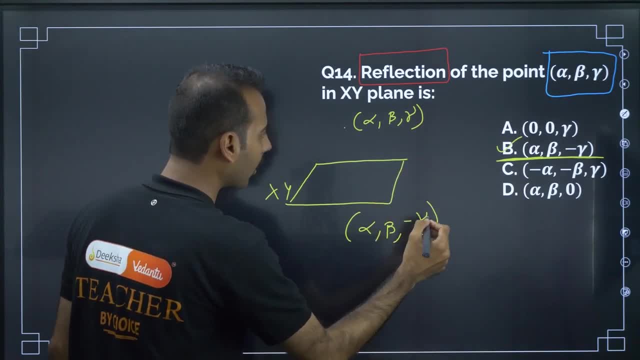 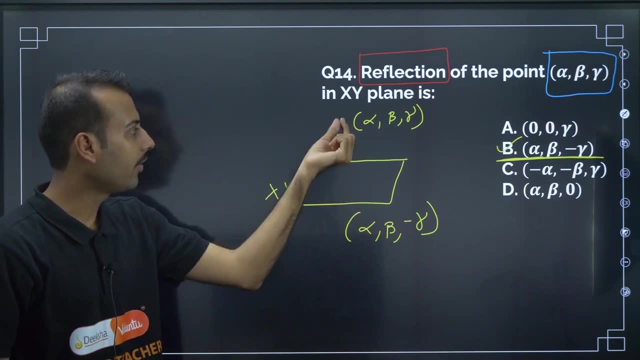 this will be alpha beta only and that will become negative gamma. Because, if you observe, here, here we are moving only in one direction, only in one direction, and we are moving in z direction only whenever we are moving in z direction, only z coordinate. 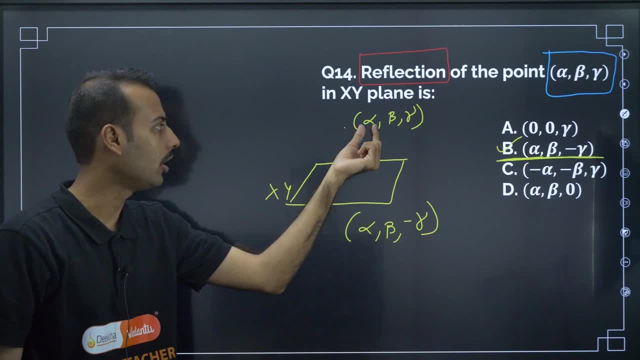 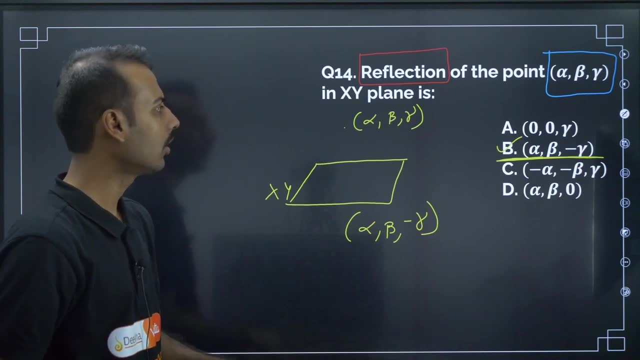 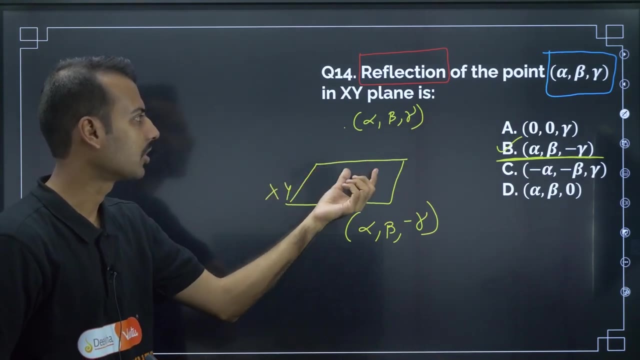 only z coordinate, Z coordinate changes remaining remain same. only x and y remain same, alpha beta, and this becomes negative. So alpha beta minus gamma. So if you have solved some problems related to reflection of point in straight lines, then it is extended version here also. it is very easy to understand they are talking. 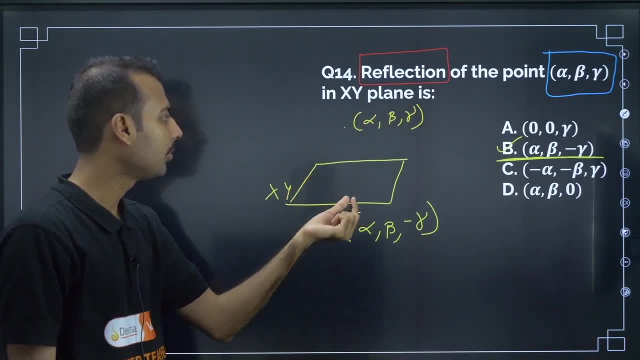 about reflection in xy plane. xy plane they have considered. Reflection means if you observe this point, the reflected point will be here. very obvious common sense. So this point will be here. here we are moving in alpha beta only. we are moving in one direction. 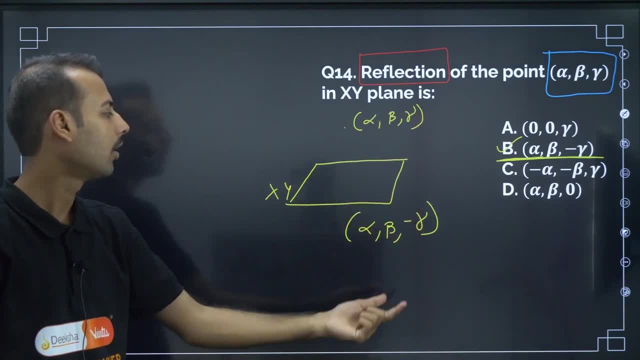 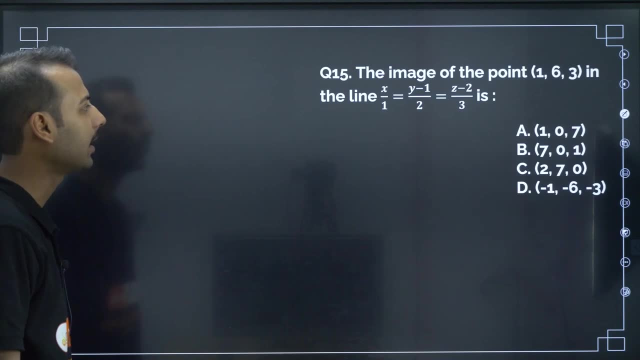 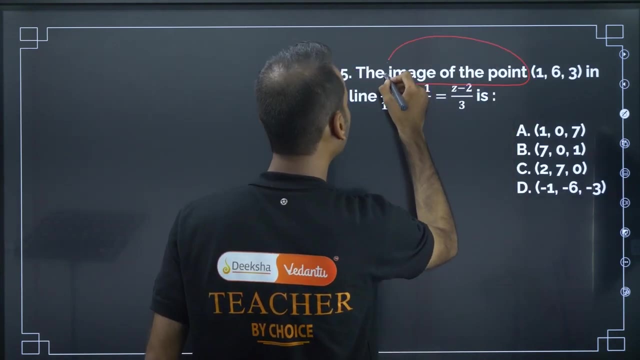 so only one coordinate: in which direction we are moving? z direction. we are minus gamma. is the answer. Next, moving on to next question: The image of the point in the line they are talking about. what are they asking? They are asking image of the point. image of the point. this is the question. image of 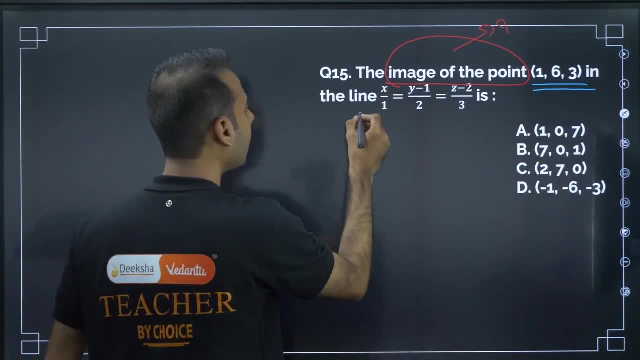 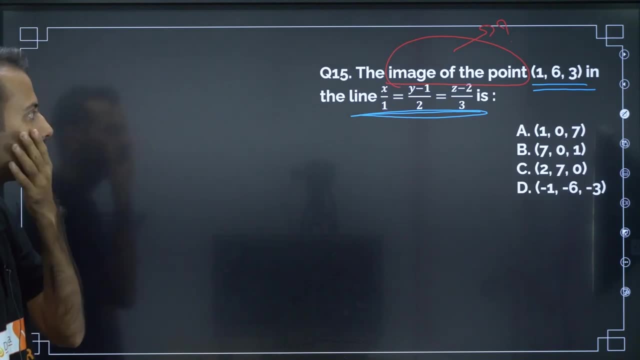 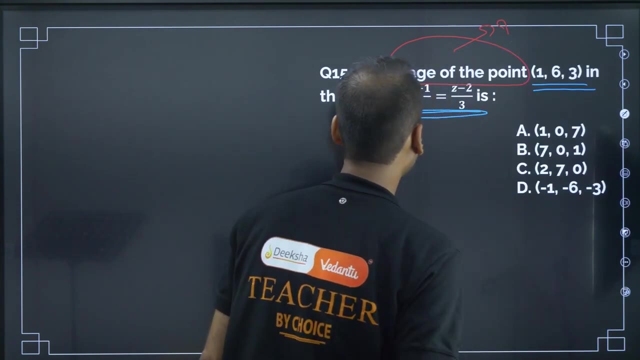 the point Which, point 163, in line, in line. So they are asking us to find image of the point 163 in the line, this line. Now one concept you should be able to remember at this point of time: image of the point. 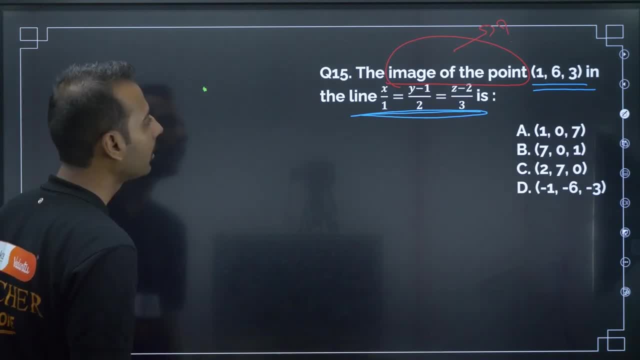 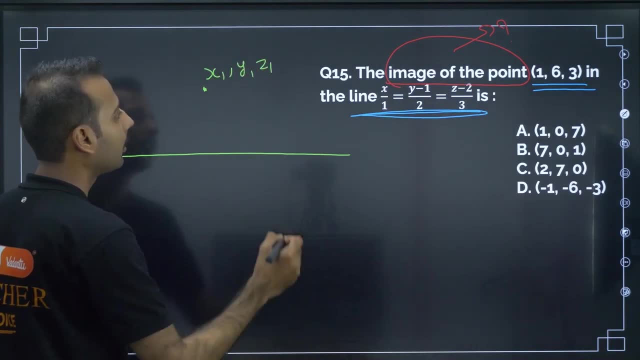 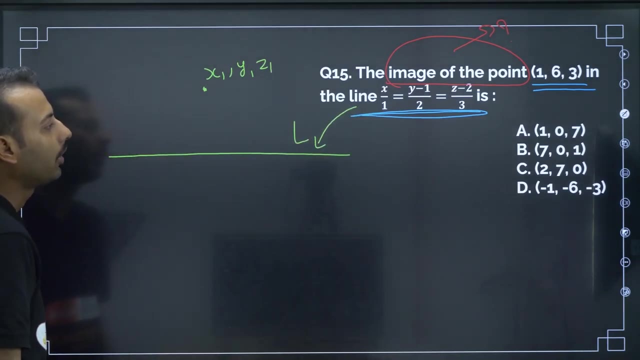 Image of the point. there is one point here. there is one point and there is one line here. This point is x1, y1. Z1,. this point is x1, y1, z1.. Line is: whatever this line, let me mark this as line L. image of the point in line. 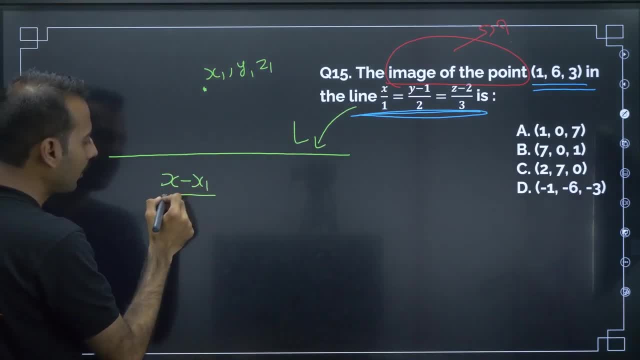 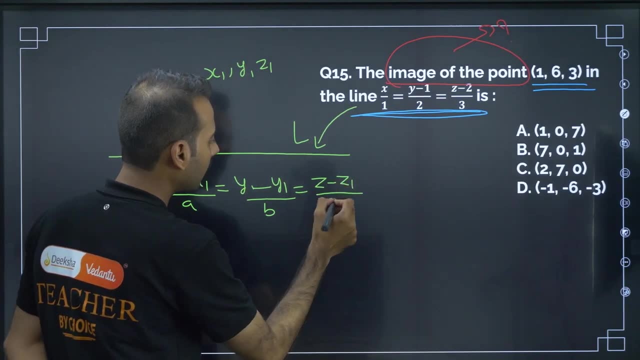 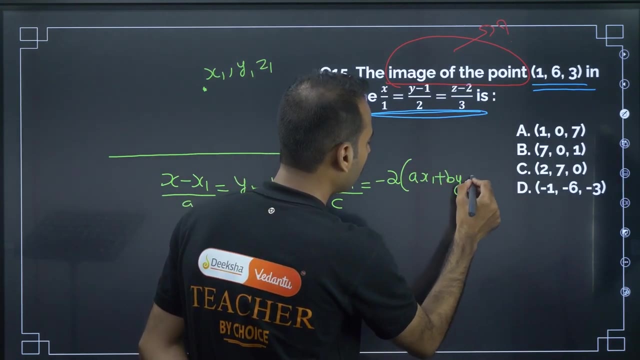 Is given by x minus x1 by a is equal to y minus y1 by b is equal to Z minus Z1 by c is equal to minus 2.. ax1 plus by1 plus c is minus er. x1 plus x1 by a is equal to z minus z1 by c. 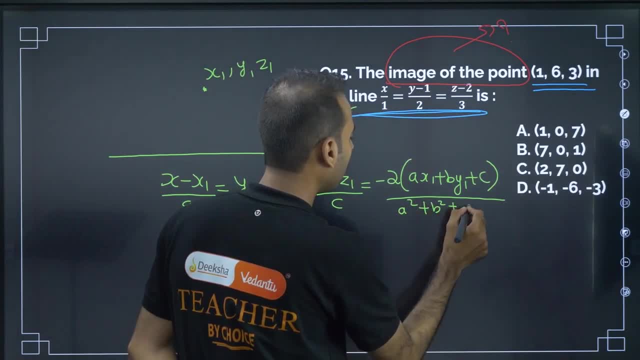 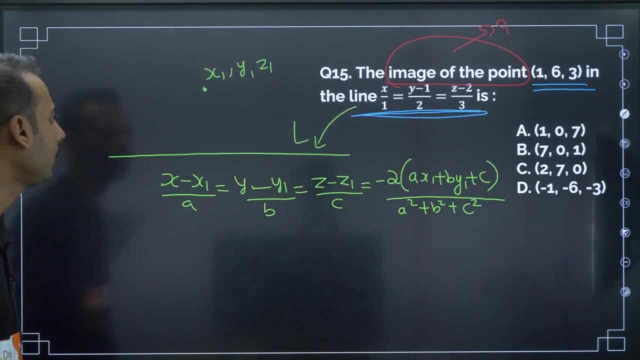 by a square plus b square plus c square. image of the point one, six, three in the line. is this concept you can use, or else we are having one more concept. what is that concept? foot of perpendicular. you have to find how to find foot of perpendicular, you assume so there. 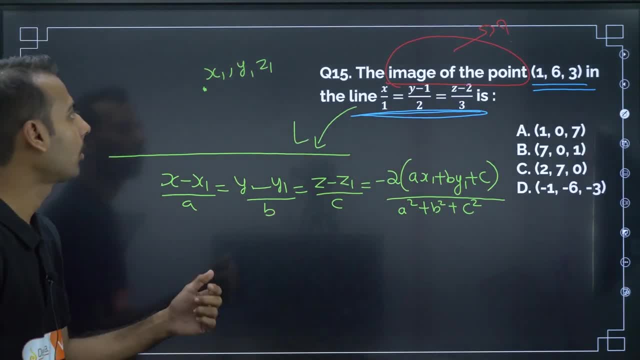 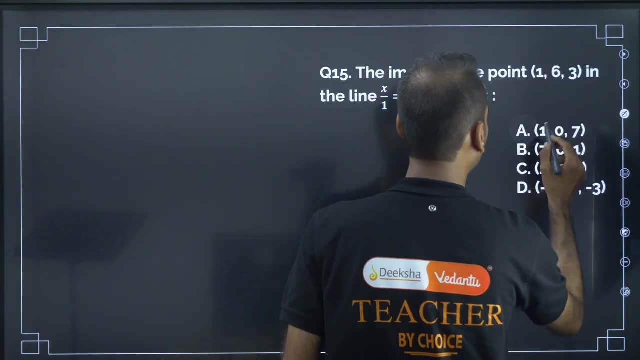 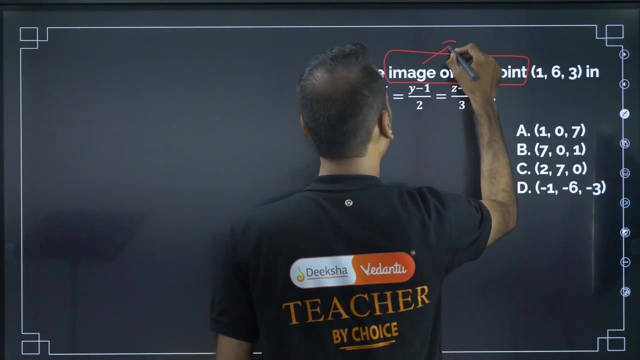 is one more method also. using this also, you can solve, or else one more method is also there. what is that one more method? let me erase all in con slide and let me. what is the question? image of the point. they are talking about. image of the point one, six, three, one. 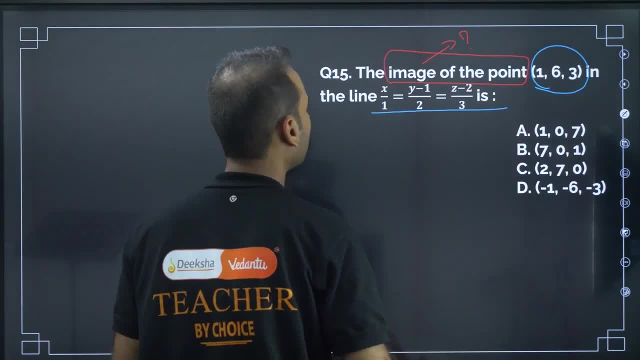 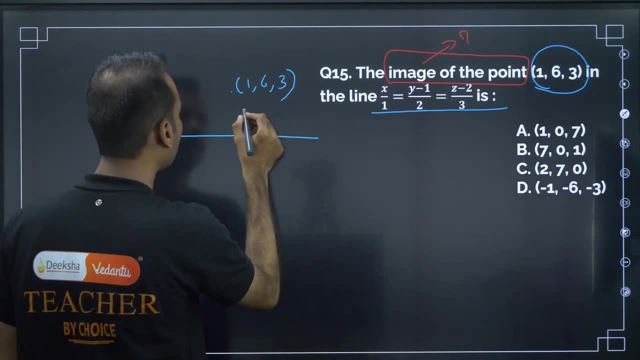 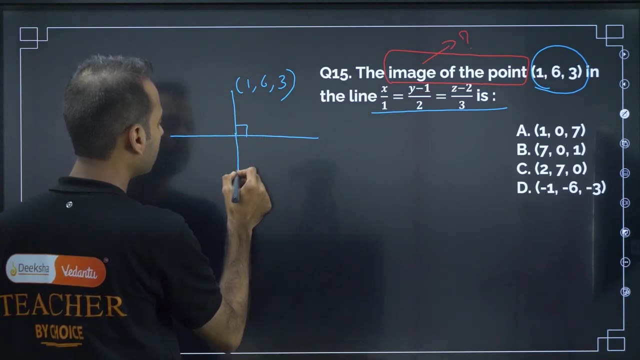 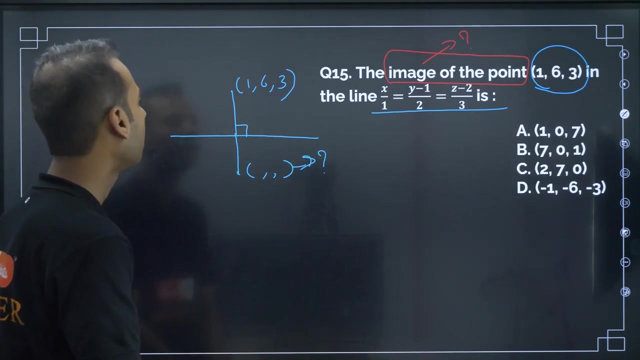 six three. one six three in the line. they are talking about image one six three in the line. this one line they have given. yes, We are asking to find image of the point 1, 6, 3 in the line how to find image of the. 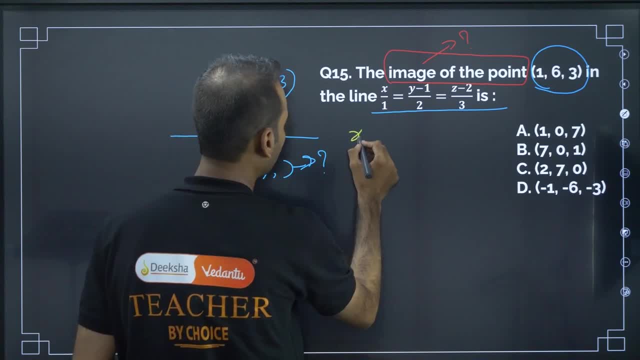 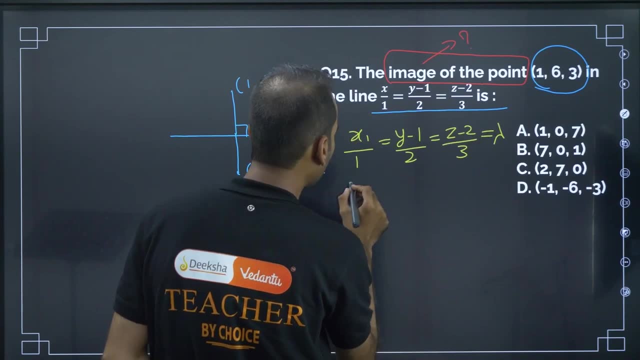 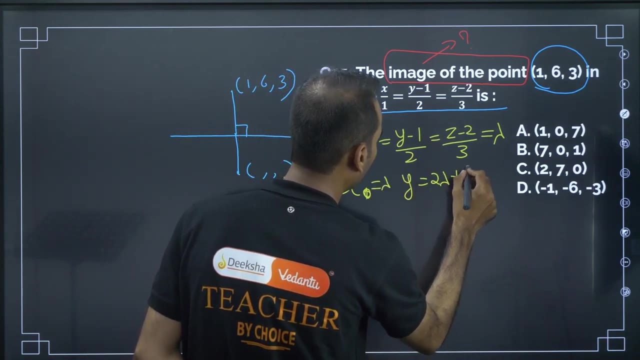 point in the line. Now let me consider given question: x by 1 is equal to y, minus 1 by 2 is equal to z. minus 2 by 3 is equal to lambda. so x is equal to lambda, y is equal to 2 lambda plus 1, z is: 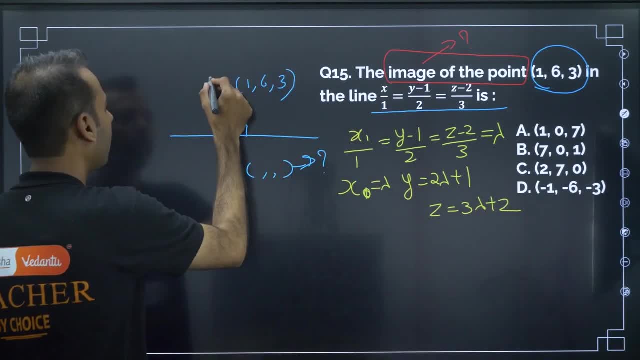 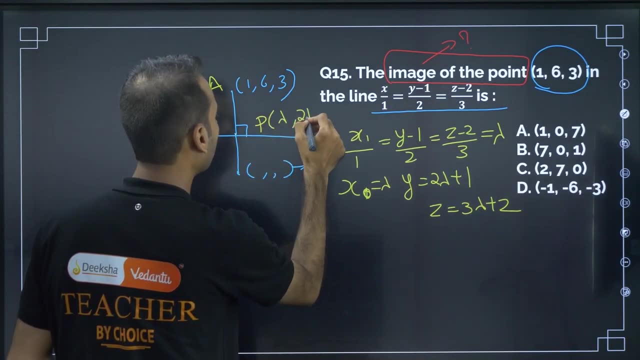 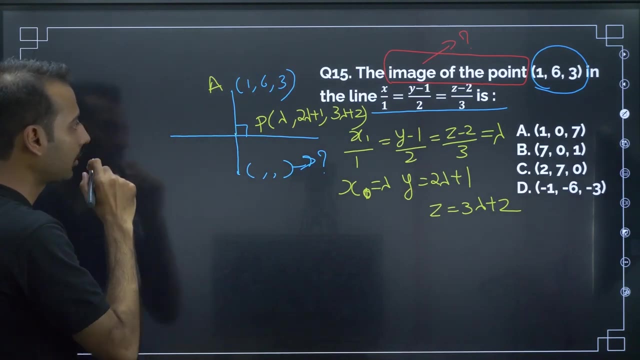 equal to 3 lambda plus 2.. So if I name this as A and if I name this as P, any point P will be in the form of lambda: 2 lambda plus 1 and 3 lambda plus 2.. So now, if I go for direction ratios, direction ratios. 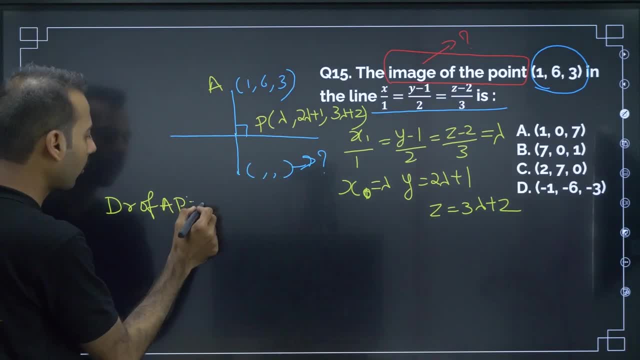 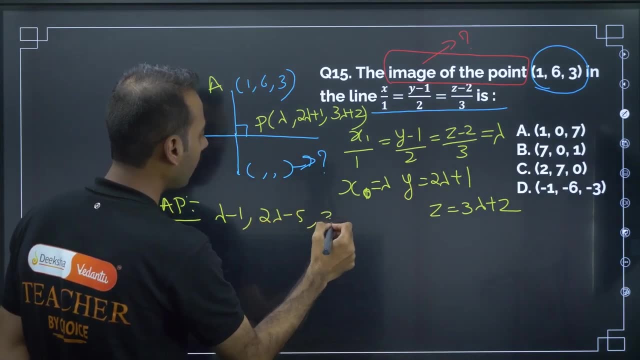 Direction ratios of A- P. in one of my previous question we have already discussed how to find lambda minus 1. that we have to do, and then 2 lambda minus 5, 2 lambda minus 5 and 3 lambda plus 2 minus 3 is 3 lambda minus 1.. 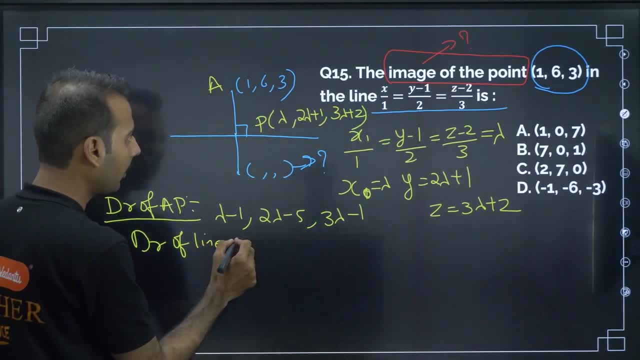 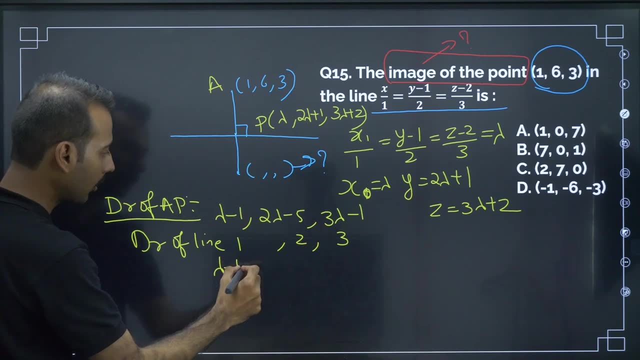 What about direction ratio of line? direction ratios of line is 1,, 2, 3.. Now these two lines are perpendicular. so if I take dot product, lambda minus 1 plus 2, lambda minus 5 plus 3, 3 lambda minus 1.. 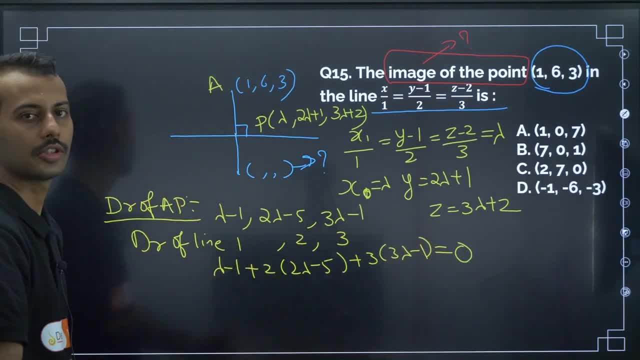 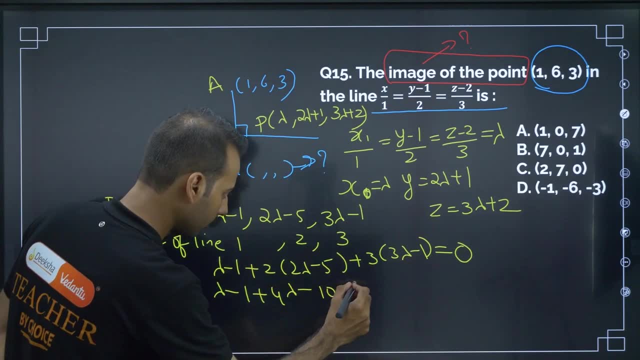 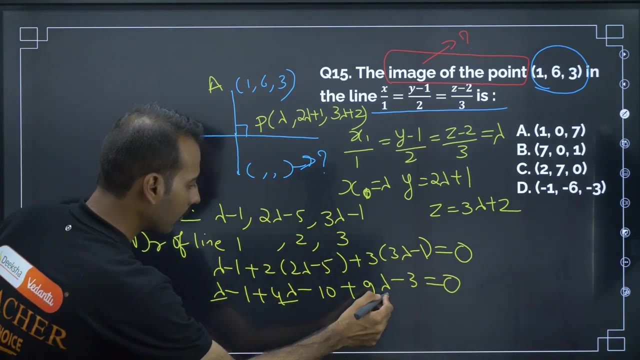 Is equal to 0, A1, A2, B1, B2,, C1, C2. just now, one problem, we have done that is same concept: lambda minus 1 plus 2 to the. Now, from here, if I try to find lambda, lambda is 14 lambda. 14 lambda is equal to 14, which. 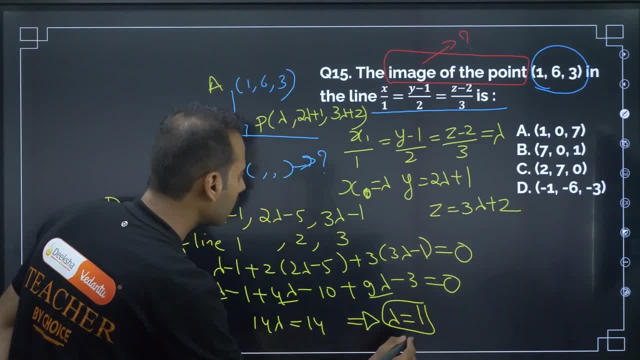 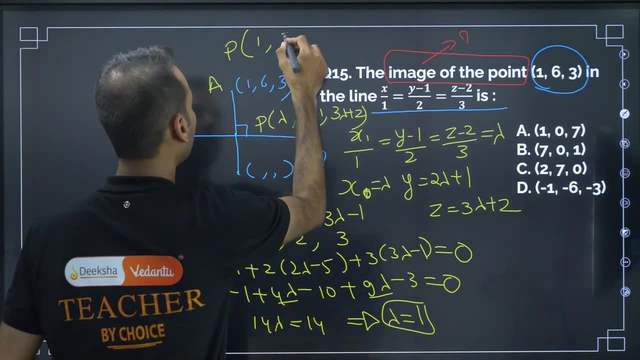 implies lambda is equal to 1.. If lambda is 1,, if I place here this P point becomes: lambda is 1.. 2 lambda is 2 plus 1, 3, 3 lambda is 3 plus 2, 5.. 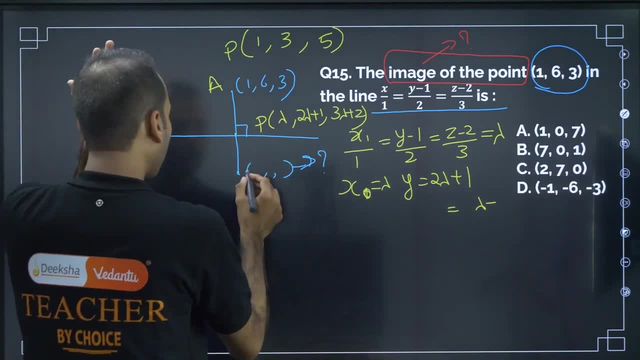 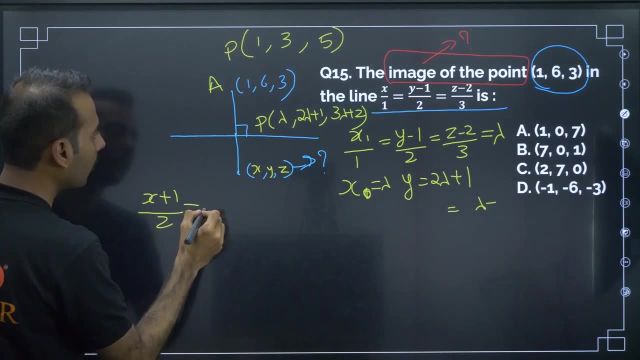 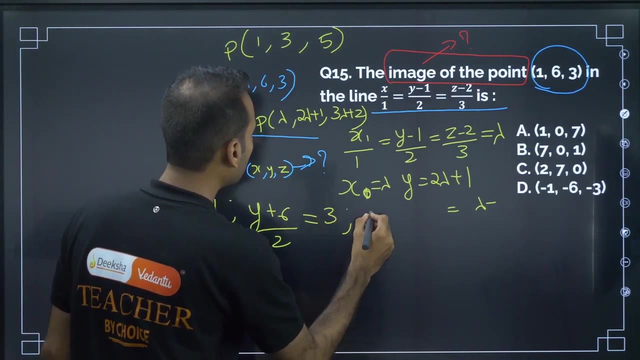 So let me remove all these things from here. Now, if I want this- x, y, z- what I will do? I will write: x plus 1 by 2 is equal to 1, y plus 6 by 2 is equal to 3, z plus 3 by 2 is equal to 5.. 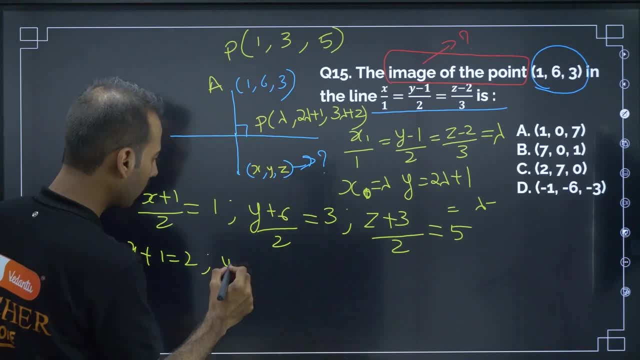 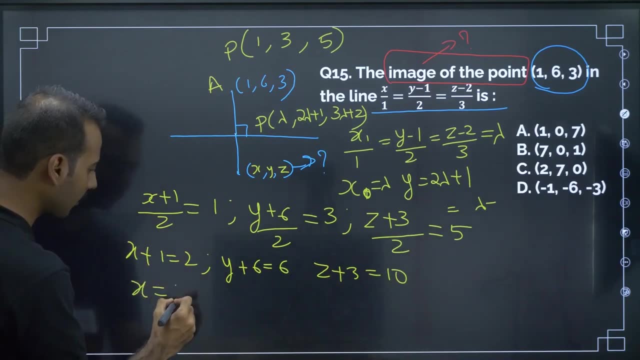 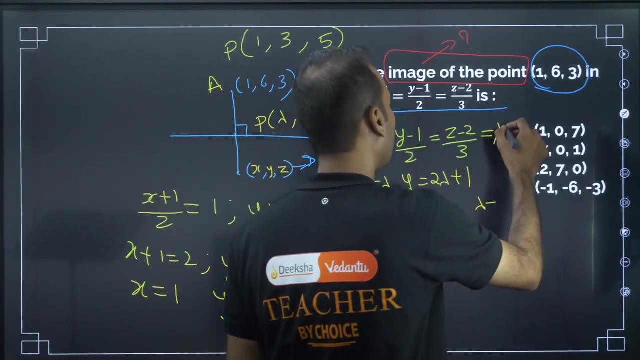 So x plus 1 is 2, y plus 6 is 6, z plus 3 is 10.. So, if I simplify this, x is 1, y is 0, z is 7, 1, 0, 7. is there any such option? 1, 0, 7. 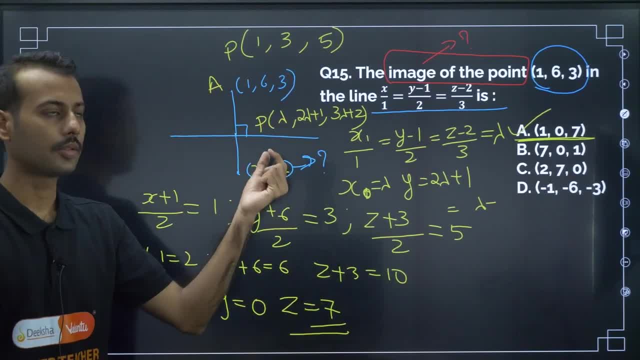 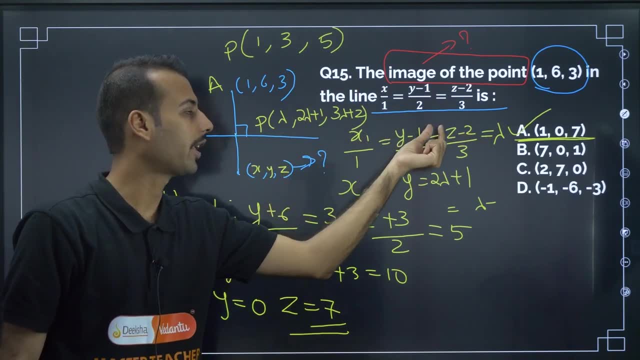 is the option. I hope you might have understood. It is very easy: question the image of the point, one point they have given in the line. they have given this line. So you equate this to lambda, So you will get x, y, z values. 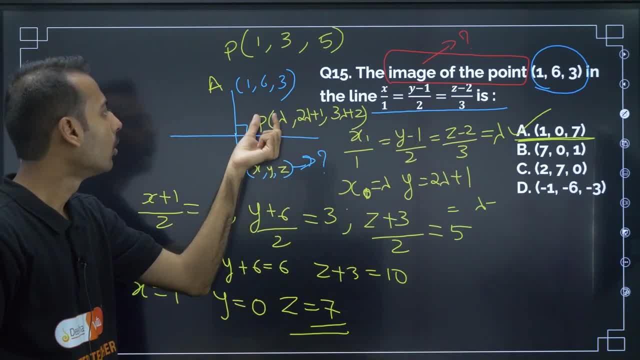 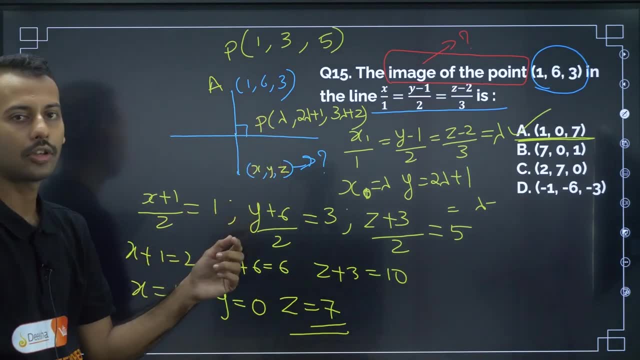 x, y, z means any point lying on that line will be in this form. Now direction ratios of this AP. you find direction ratios how to find AP: x2 minus x1, y2, y1.. You will get direction ratios. in previous slide I have written all AP direction ratios. 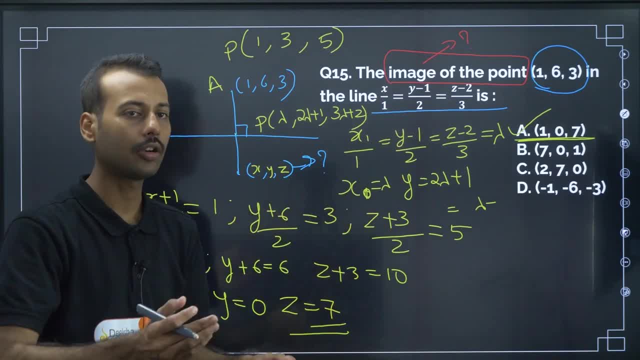 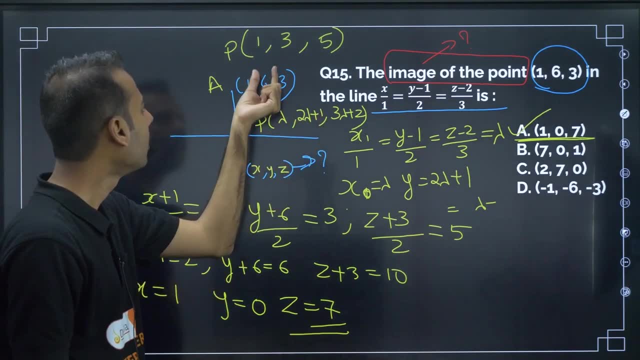 you know, and this line direction, ratios a1, a2, you use that condition, you will get lambda value. After getting lambda value, you substitute here. The moment you substitute, you will get this point. If this point is known, this P is midpoint, This P is midpoint of this point. 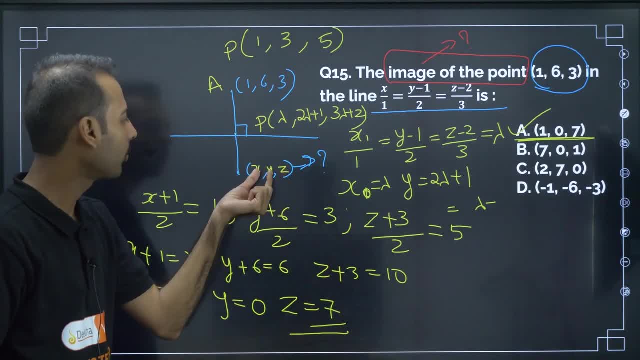 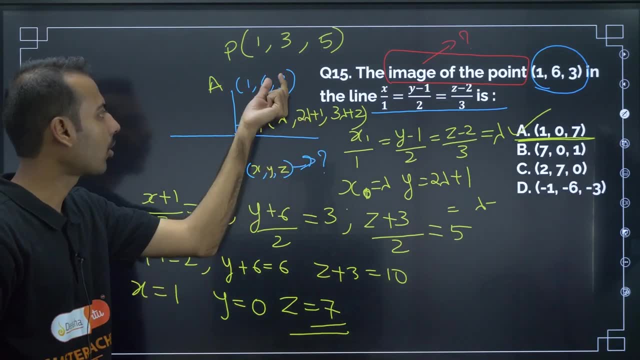 This point and this point. So you use midpoint formula. What is midpoint formula? This coordinate plus this coordinate by 2 is equal to this. This coordinate plus this coordinate by 2 is equal to this. So this coordinate plus this coordinate is equal to this. 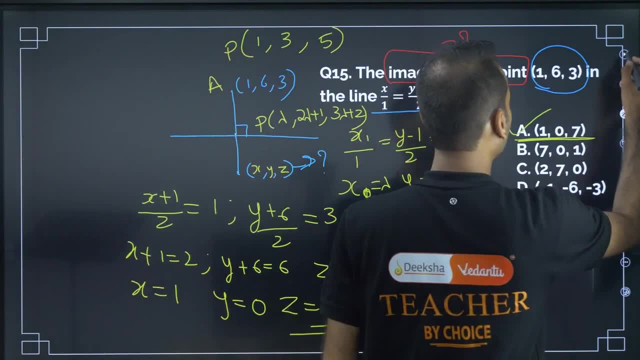 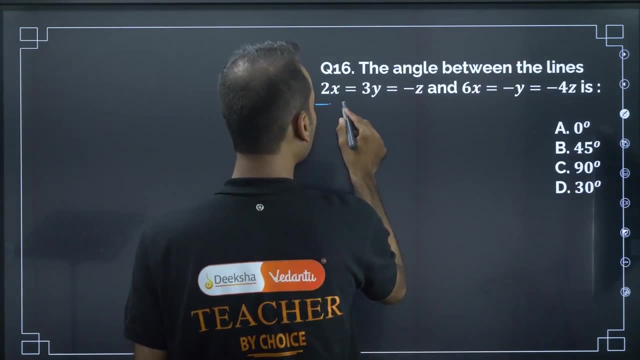 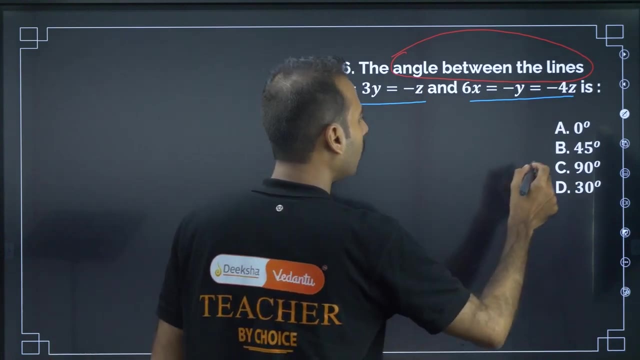 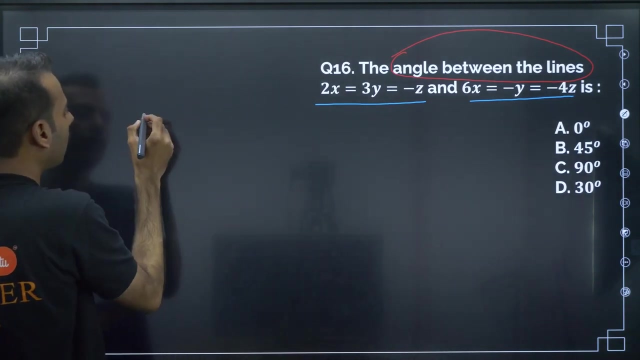 So and then you keep solving, you will get the answer. very easy question just time: consuming The angle between the lines, the angle between lines. they have given two lines and what are they asking? They are asking to find angle between the lines Now, whenever angle between lines. they have given angle between lines. try to recall angle. 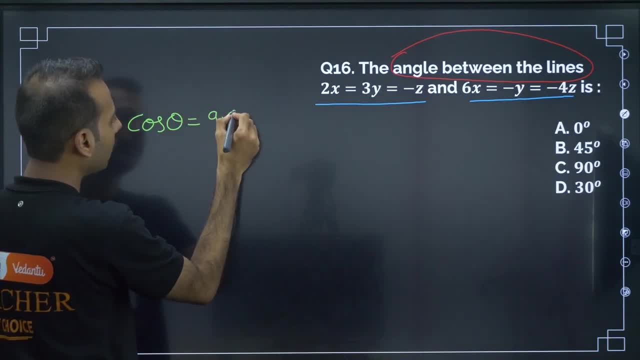 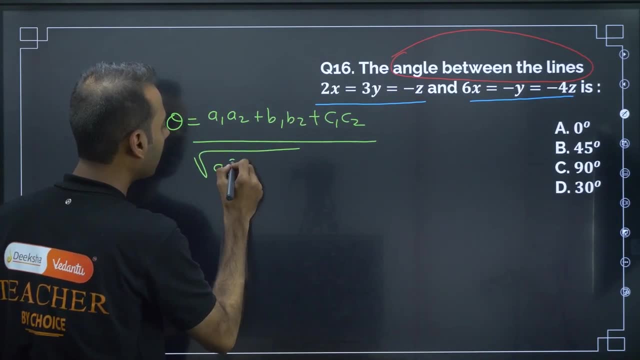 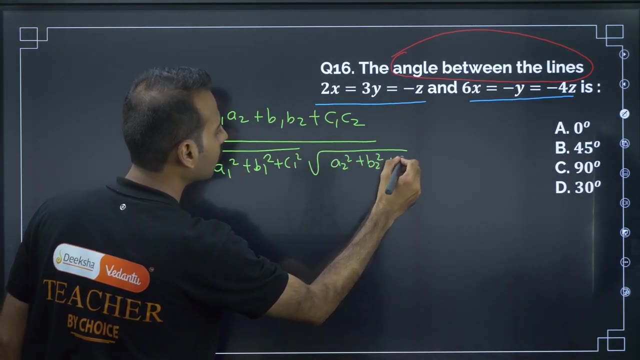 between lines. formula is given by cos. theta is equal to a1, a2 plus b1,, b2 plus c1, c2, by root of a1 square b1 square, c1, square root of a2 square, b2 square c2, square angle between: 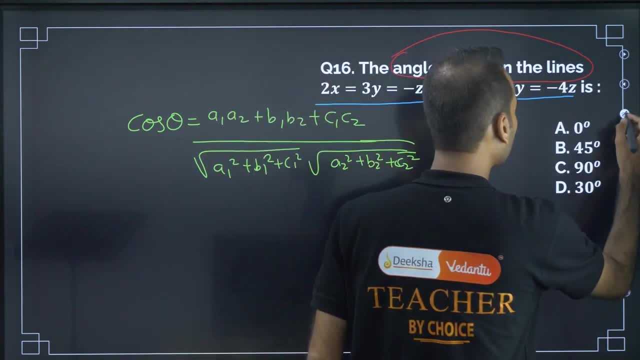 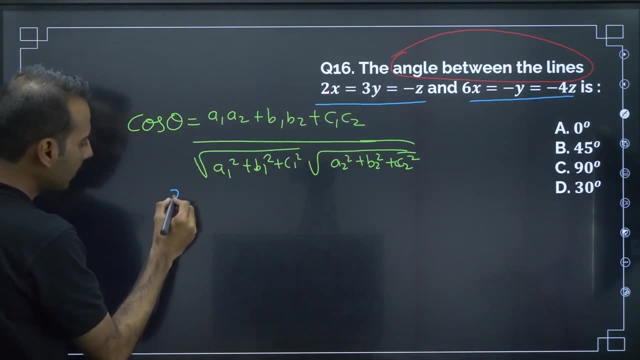 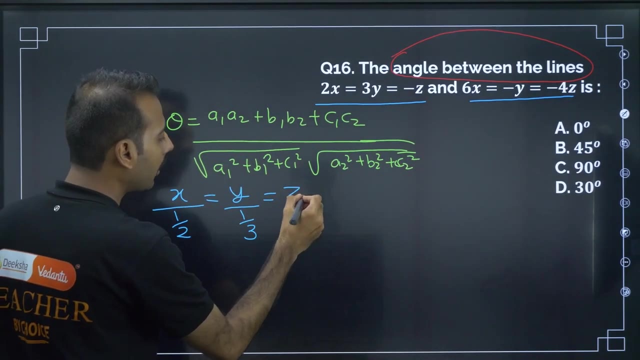 the lines. This is what is the angle between this line. Now let me consider that, given line 2x minus 3y, rather than writing that 2x, let me write this x, as 1 by 2 is equal to y, 1 by 3 is equal to z by minus 1 and x divided by 1 by 6: i. 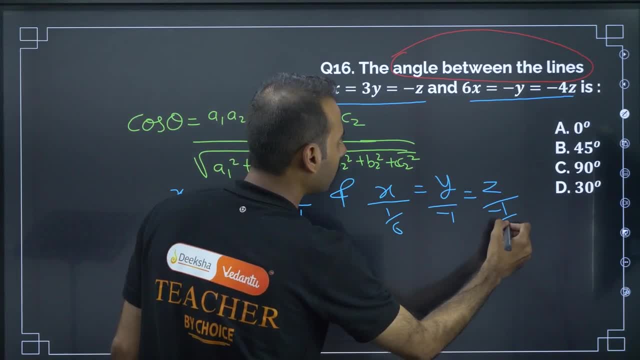 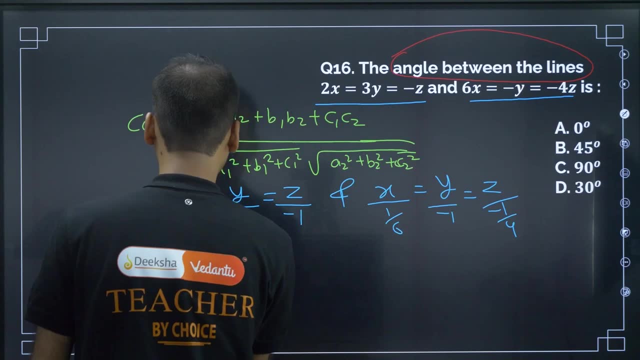 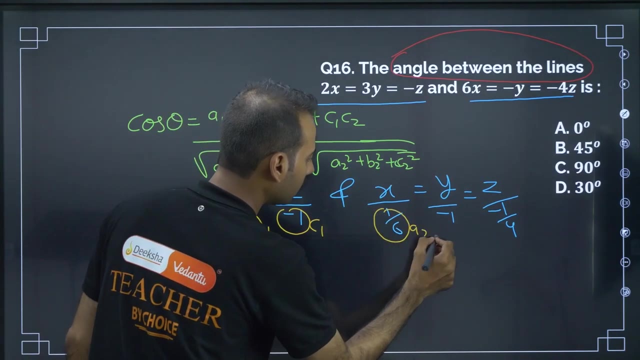 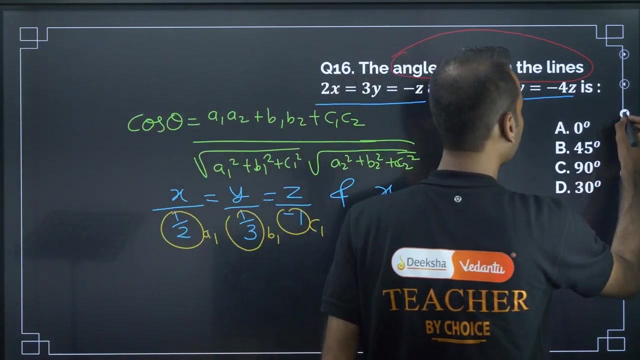 by minus 1 is equal to z by 1 by 4.. Same equation only. You can write it like this Now: a1, b1, c1. you already know This is a1, b1, c1, a2, b2, c2, a2, b2, c2. angle between them is given by cos theta. 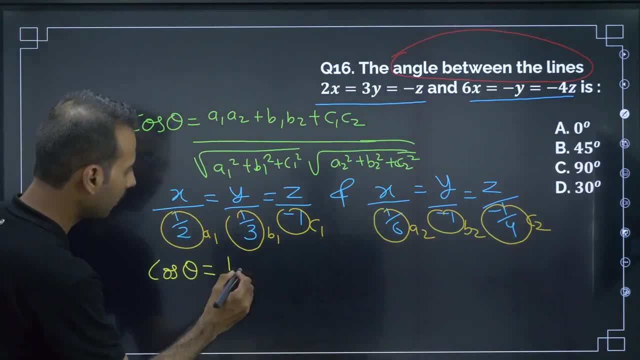 So cos theta is equal to cos, theta is equal to a1, a2.. b1, b1, c2. a1, b1, c2.. So this is a1, b1, c2, a1, b2, c2.. So this is a1, b1, c1.. 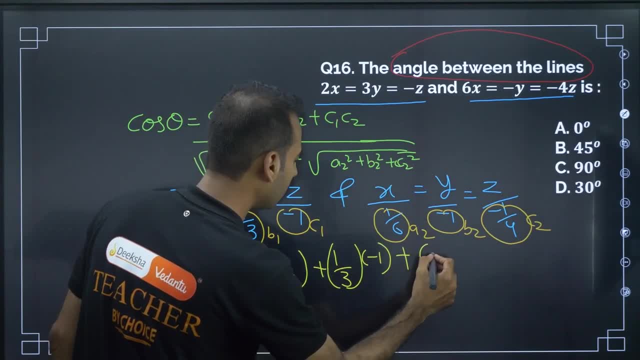 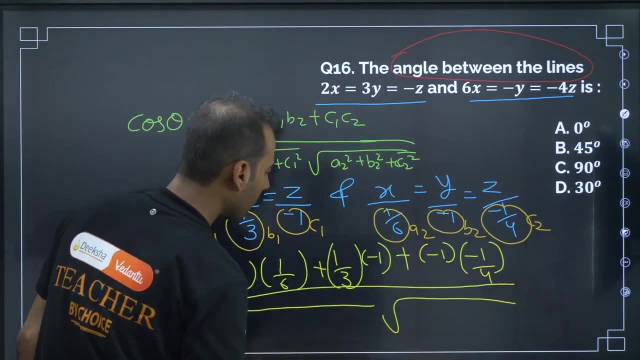 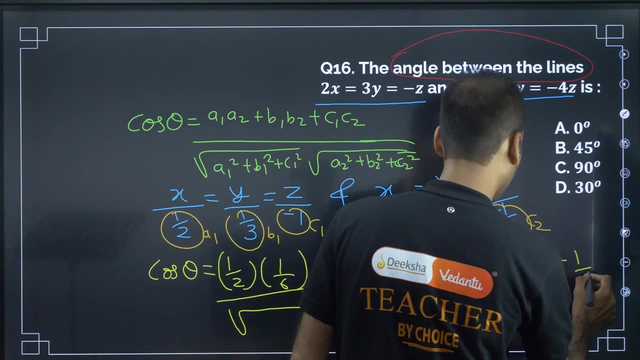 This is a1, b1, c2.. b, 2, c, 1, c, 2 minus 1 by 4 by, and root of all those things you solve, you solve. So this is 1 by 2 L, 1 by 2 L, and this is minus 1 by 3, and this is plus 1 by. this is plus 1 by. 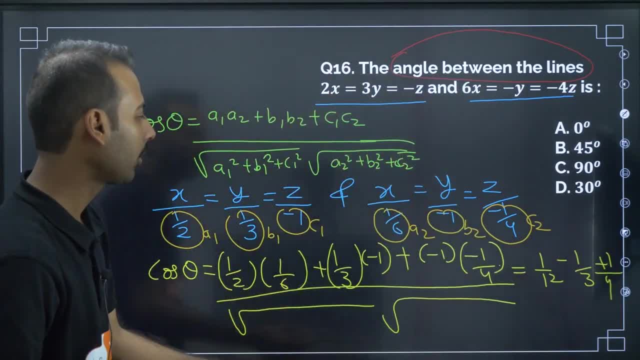 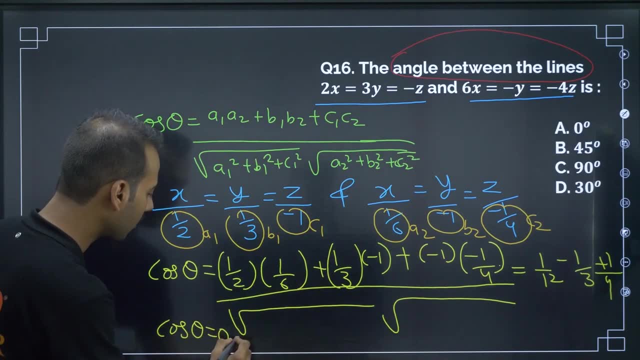 4. Now, the moment you solve this, this, you will get 0.. So cos theta, and anyways 0 divided by anything is 0. So cos theta is equal to 0, which implies theta is equal to 90 degrees. 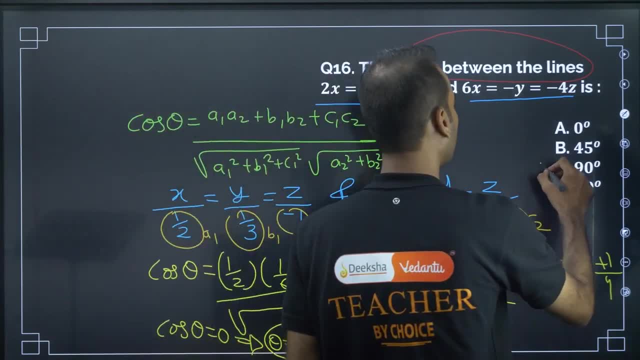 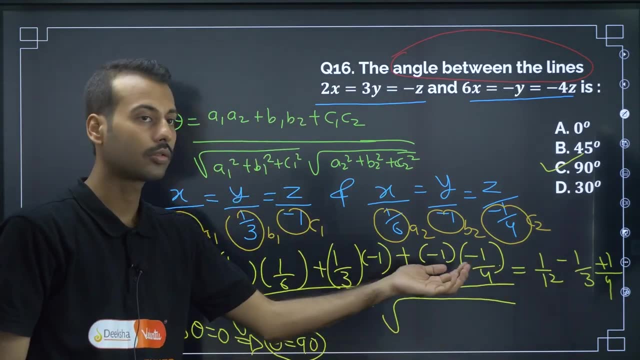 So is there any such option? theta is equal to 90 degrees. c is the answer. I hope everybody knows how to solve. simplify this, only simplification, part, only addition. subtraction that to just LCM and subtraction, addition that you have to do If anybody does not know that you can. 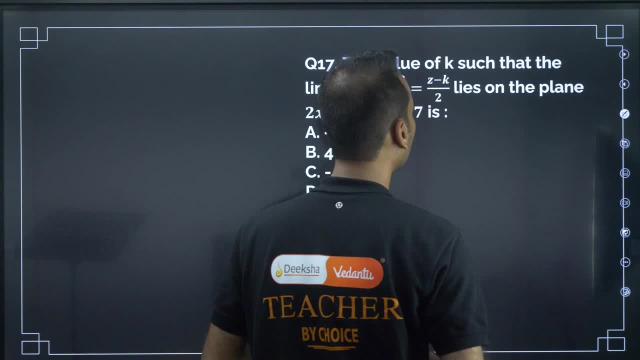 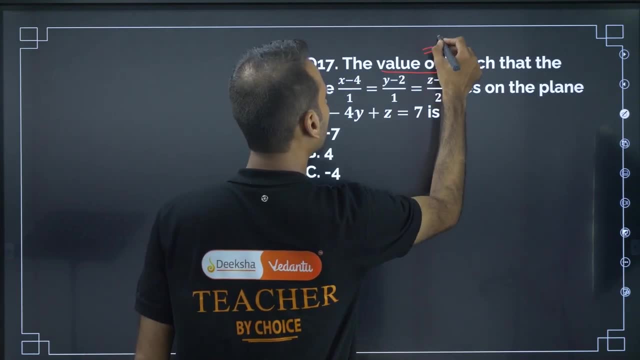 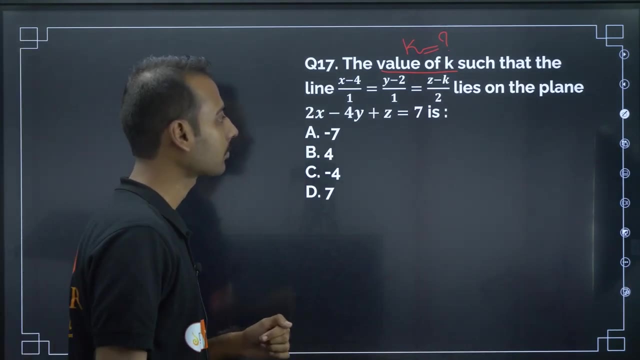 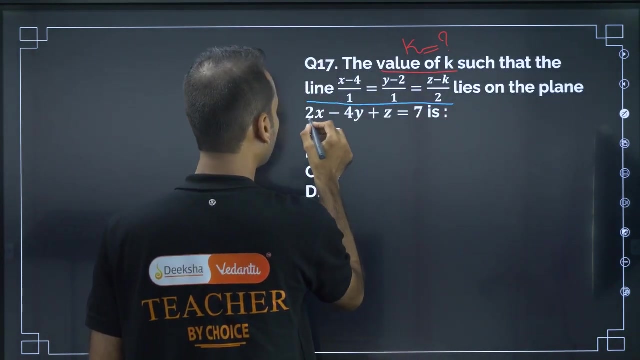 add one comment. I will solve it there. I will explain you The value of k. next question. next question is the value of k. They are asking this. k is equal to what such that line lies on the plane, some information given information line. there is one line lies on the plane. it is lying on the plane, the 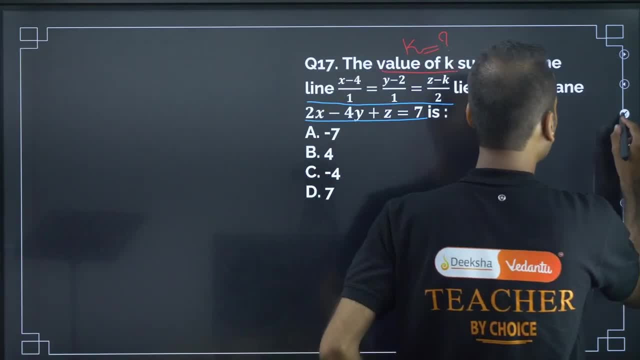 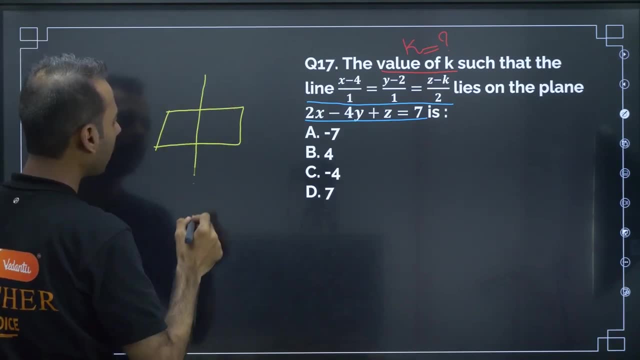 value of k they want. Now, see here, line is lying on the plane, there is one plane and there is another plane, And that is the line of k which actually lies on the plane. So, plane and there is one line, there is one plane, there is one such that the value of k such, 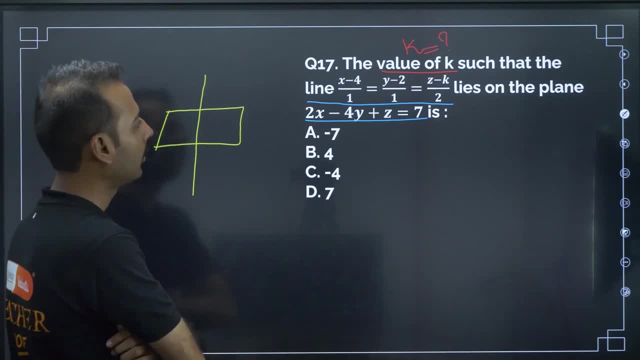 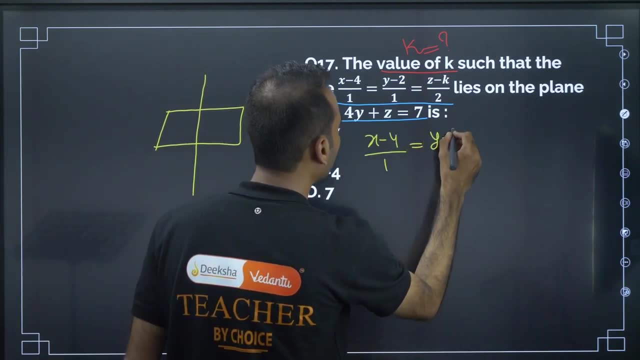 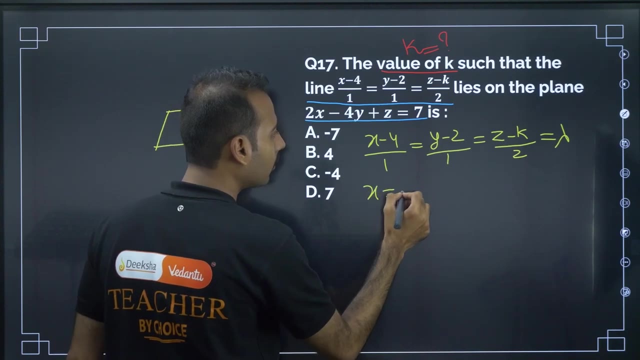 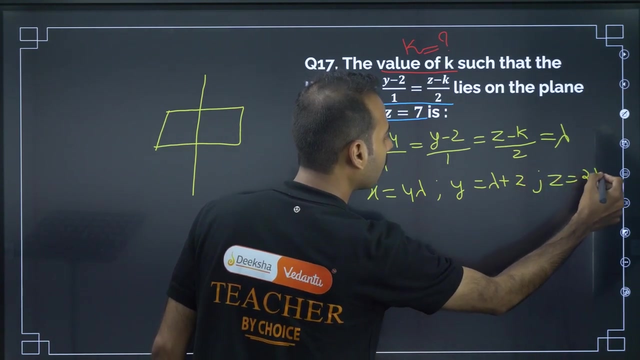 that line lies on the plane. Now for that line. let me consider that line. x minus 4 by 1 is equal to y. minus 2 by 1 is equal to z. minus k by 2 is equal to lambda. So x is equal to 4 lambda, y is equal to lambda plus 2. z is equal to 2 lambda plus k: 2 lambda. 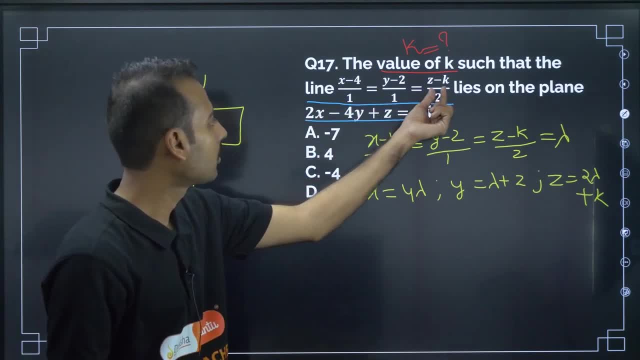 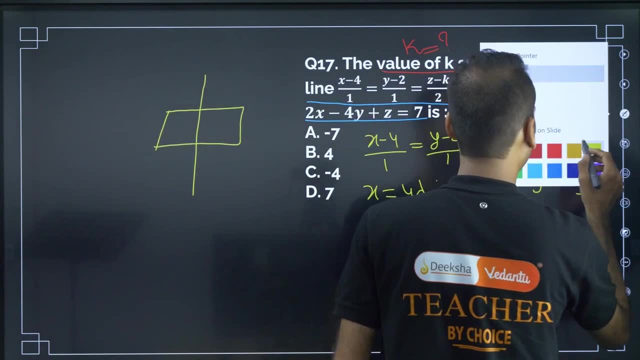 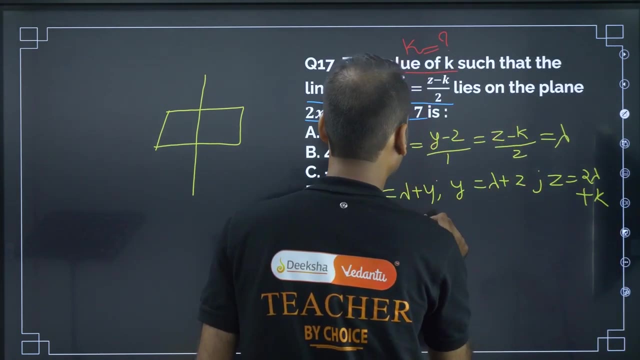 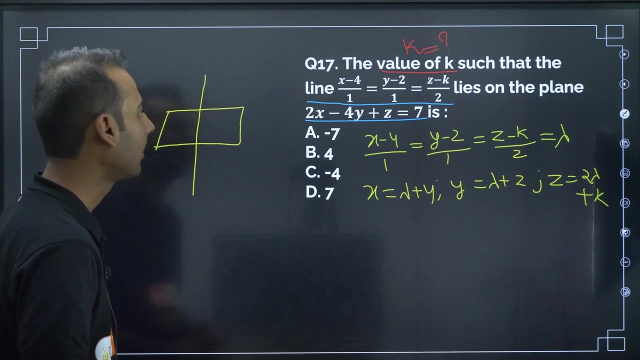 plus k. if I equate this to lambda, this becomes lambda plus lambda, not 4. lambda, lambda plus 4, my bad. So and y is equal to lambda plus 2, z is equal to 2. lambda plus k lies on the plane, So 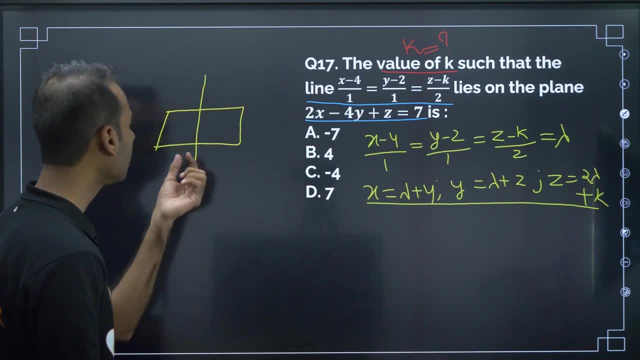 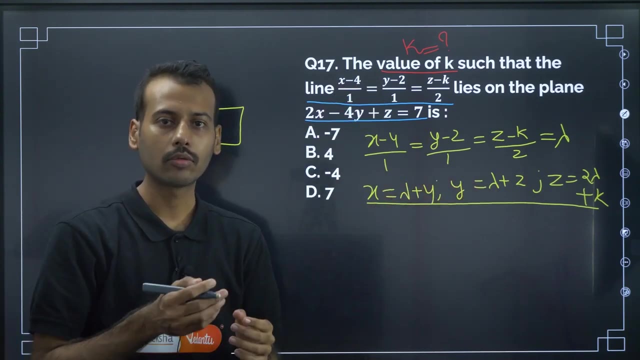 these are the points on the line and this point on the line- let me consider that will also lie on plane. So this has to satisfy equation of plane. also once again, core concept, logic. what is the logic share this point x, y, z, I found means I am finding one point on. 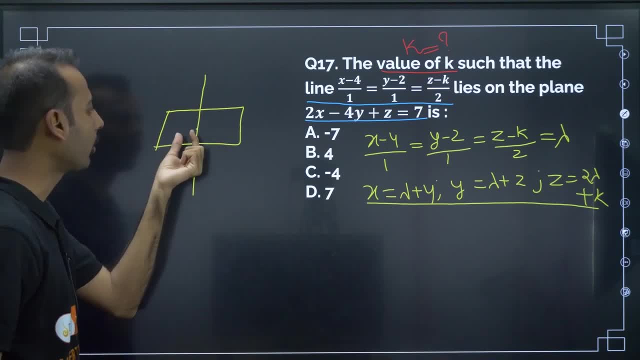 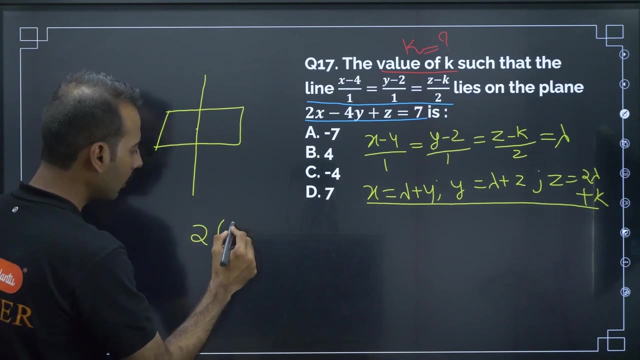 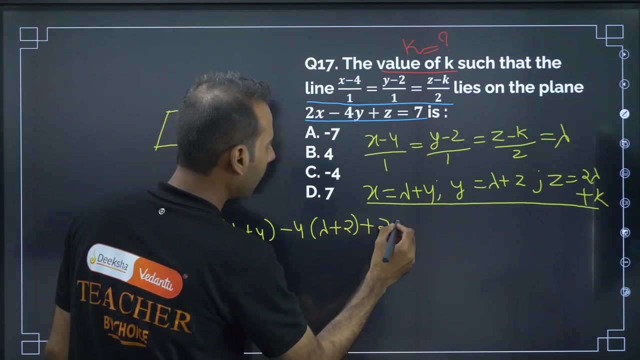 the line. So let me say that point somewhere here: Tthat point on line, that point on that line is passing through that plane, that line is. that means that point also has to satisfy equation of plane. So if I substitute here, if I substitute here, this becomes 2 lambda plus 4 minus 4 lambda plus 2 plus z, 2 lambda. 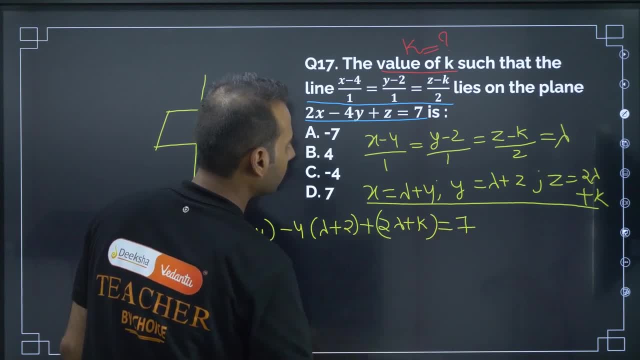 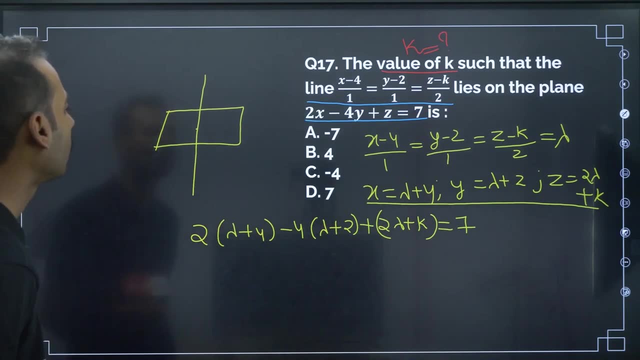 plus k is equal to 7.. value of k. the value of k such that line lies on the plane. Next, if I try to simplify this here, there are two unknowns and one equation. Let me simplify this. what will happen? we will see. 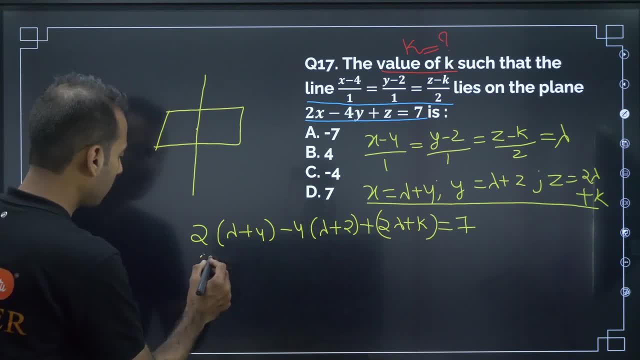 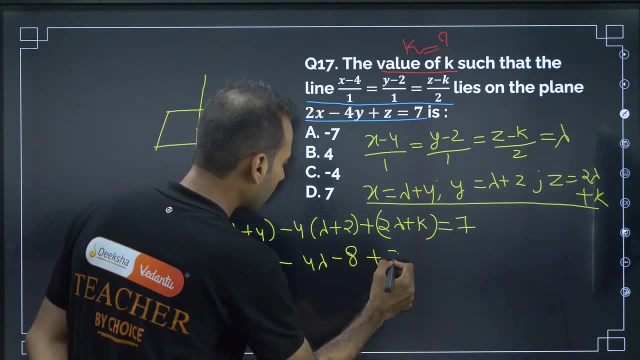 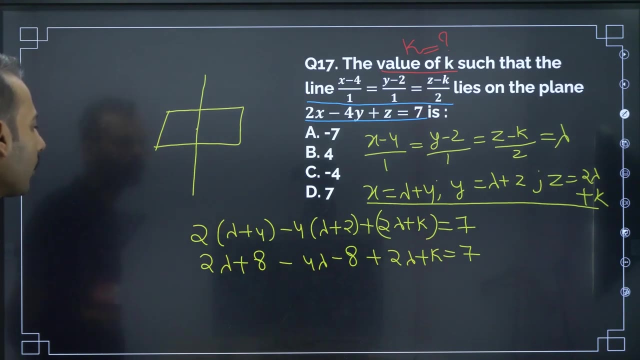 2 lambda plus 8 minus 4 lambda minus 8 plus 2 lambda plus k is equal to 7.. So plus 8 minus 4 lambda minus 8 plus 2 lambda plus k, So anything gets cancelled. 2 lambda positive, negative. this. 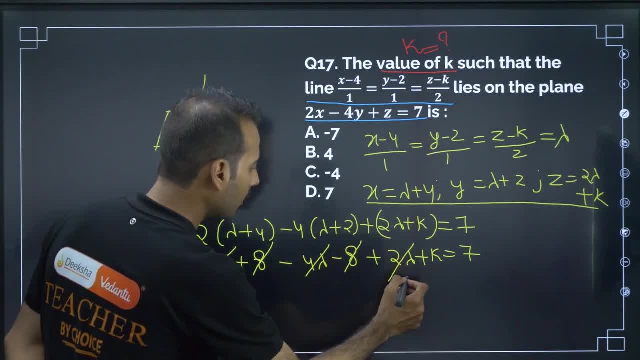 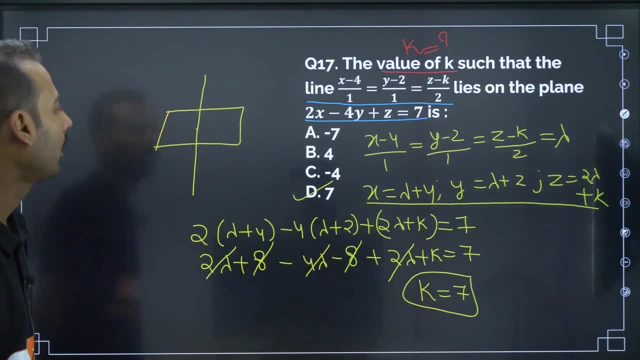 will get cancelled. positive, 8, negative, It gets cancelled. so we are left with: k is equal to 7.. So is there any such answer? d is the answer. moving on to next. moving on to next very easy question. see here what we have to do: the value. 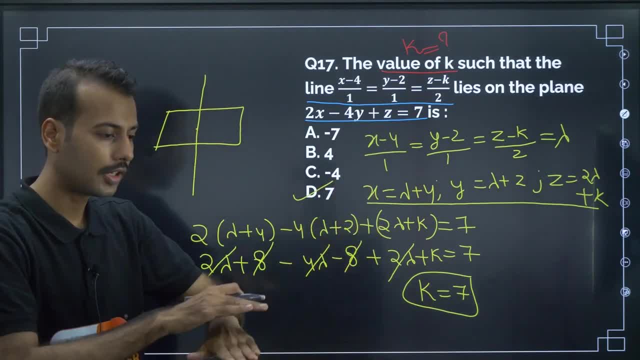 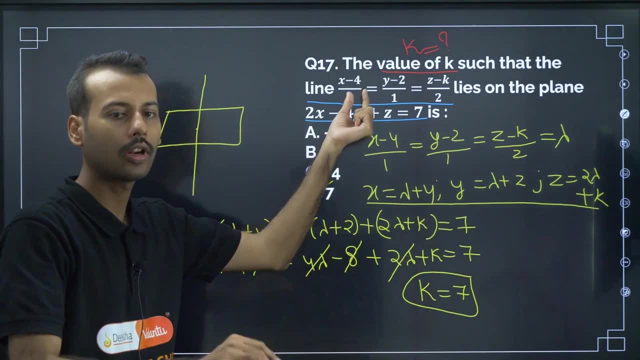 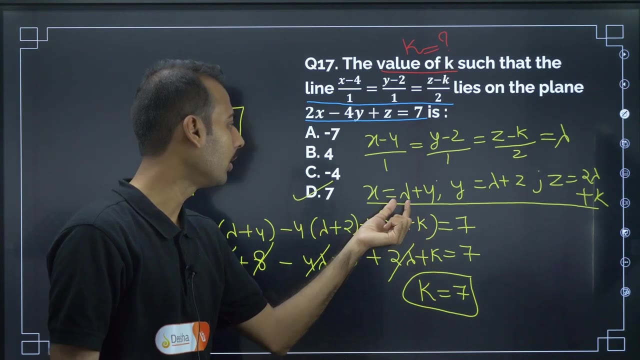 of k. they are asking to search that this line lies on the plane. that means there is one. one plane in that one line is passing lies on the line, passes on them. I am considering one point on line. hmm, any point on the line will be in this form. that will also satisfy equation of 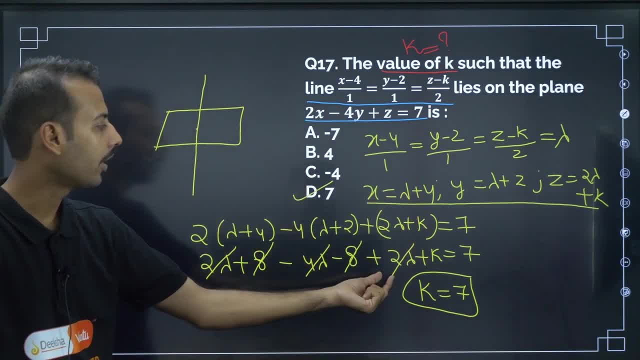 plane. So we are left with k is equal to 7.. So we are left with k is equal to 7.. So is there any point on this plane? So this point I am substituting in this plane and then, finally- I am simplifying- I will get some value of k. that's it. Moving on to next question, the locus represented by 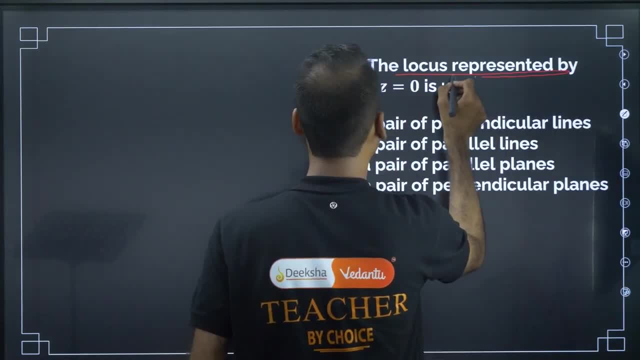 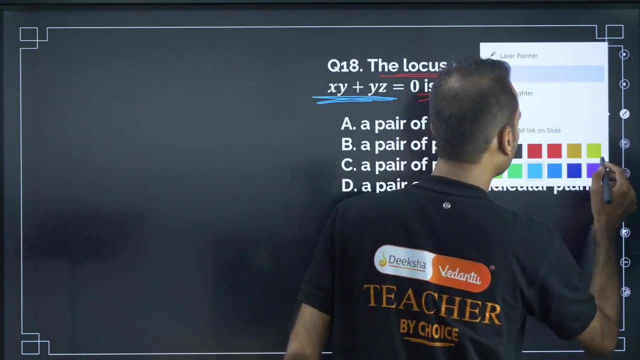 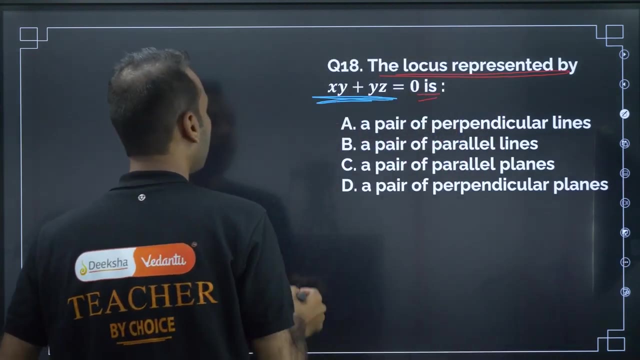 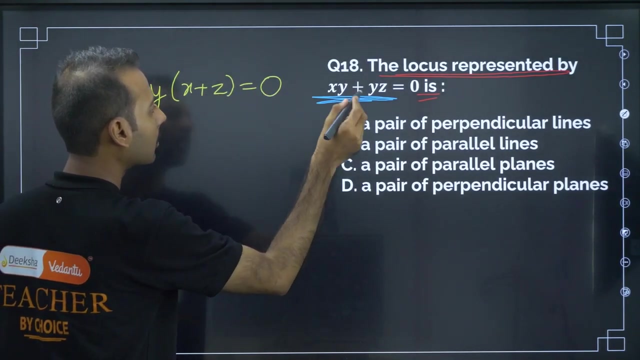 they are asking. the locus represented by what is this? they have given some plane. x, y plus y. z is equal to 0, is So what is the question here? the locus, if I take y common from these two equations I am left with x plus z is equal to 0.. The locus represented by this, what is this? 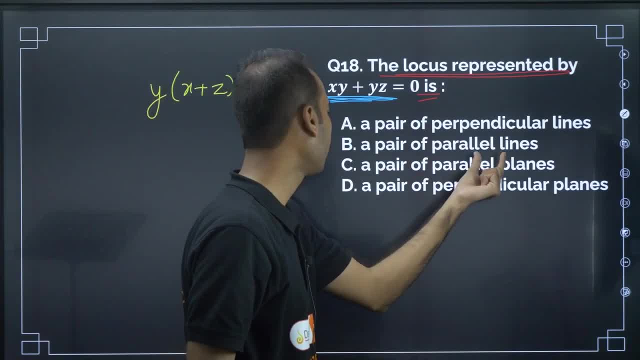 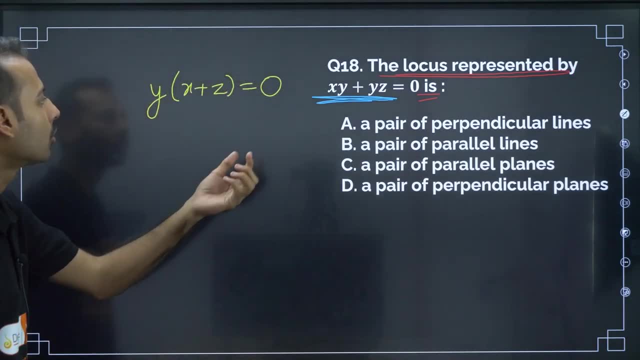 representing pair of perpendicular lines, pair of parallel lines, pair of parallel planes, pair of perpendicular planes. So, whether it is planes, lines, perpendicular, parallel, what type of it is? So that given equation- only I am taking y, common x plus z I am left with- is equal to 0, which implies 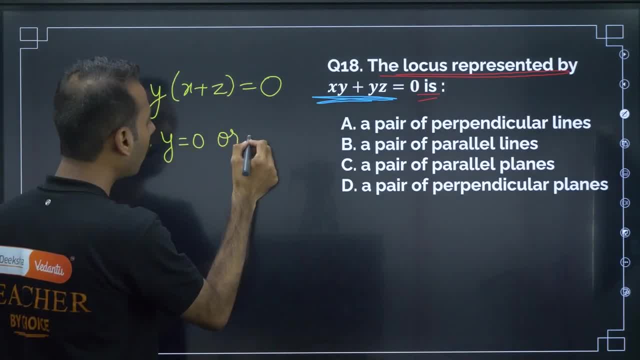 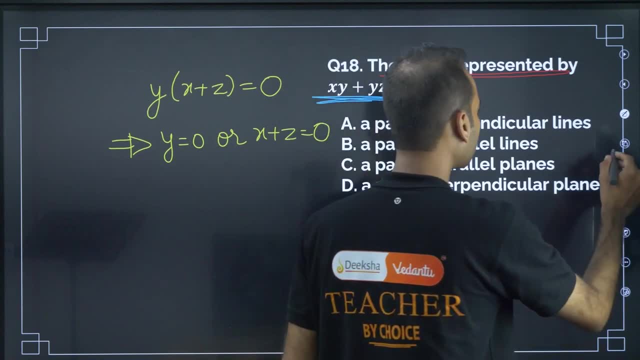 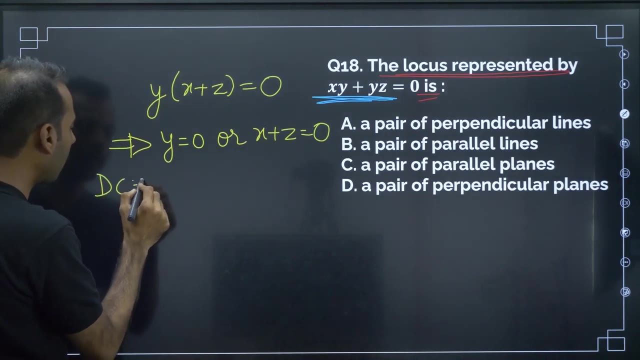 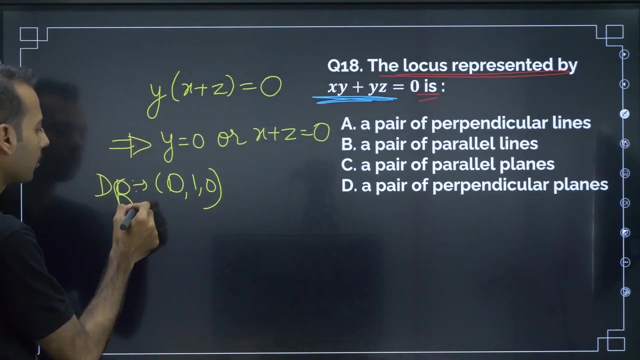 what does this imply? this imply y is equal to 0, or this is x plus z is equal to 0. Or this is equal to 0. Now, x is equal to 0 means what are the direction cosines of this? direction cosines of this are 1, sorry, 0, 1, 0. direction cosines or direction ratios of this is 0, 1, 0. 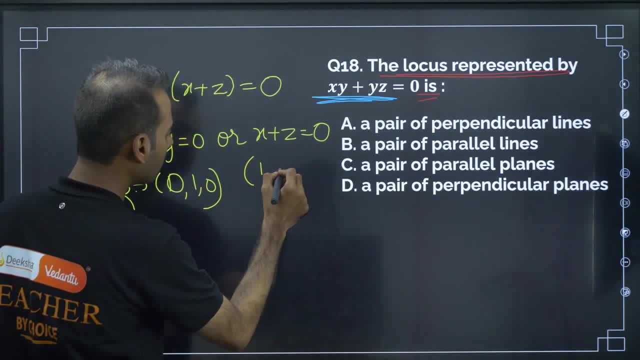 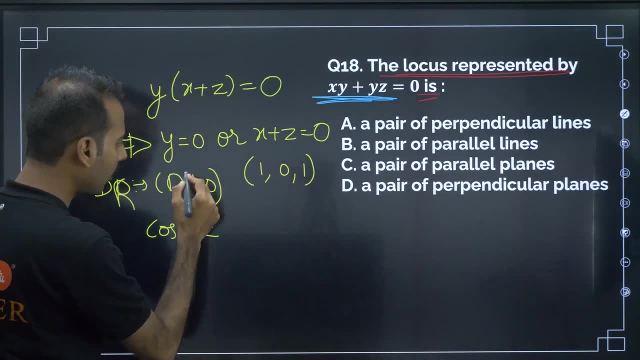 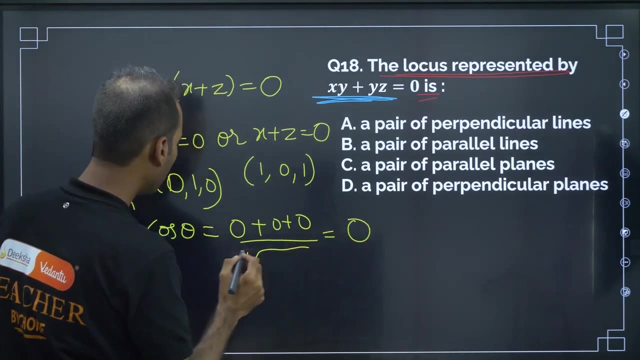 Next for this direction ratios are 1: 0, 1. direction ratios for this is now: if I take cos cos theta is equal to 0, 0, 0, by whatever it is, it is 0 cos theta is equal to 0. this implies theta is equal. 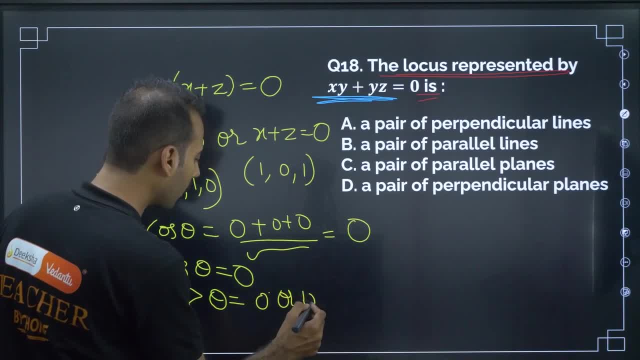 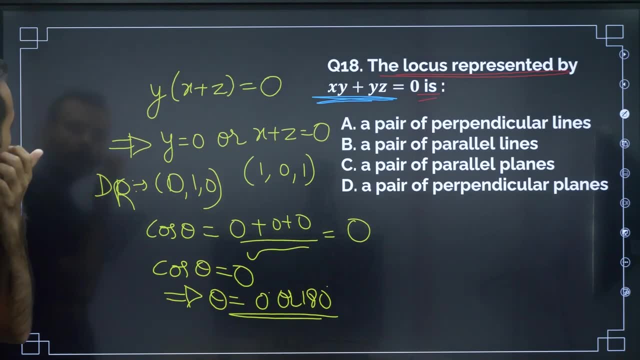 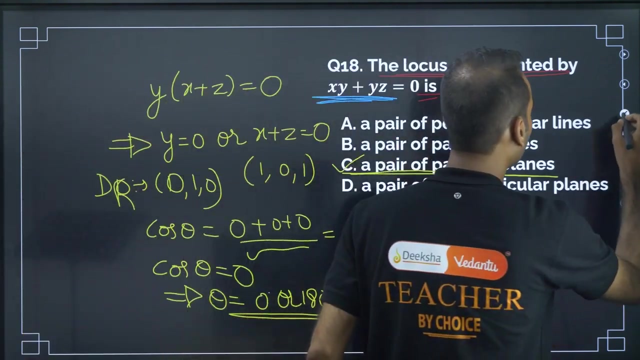 to theta is equal to 0 degree or 180 degree. This means what? 0, 1, 0 cos theta is equal to 0 means these are representing pair of parallel planes. pair of parallel planes. cos theta is equal to 0. COs theta is equal to 0. sorry, 1 small mistake. cos theta is equal. 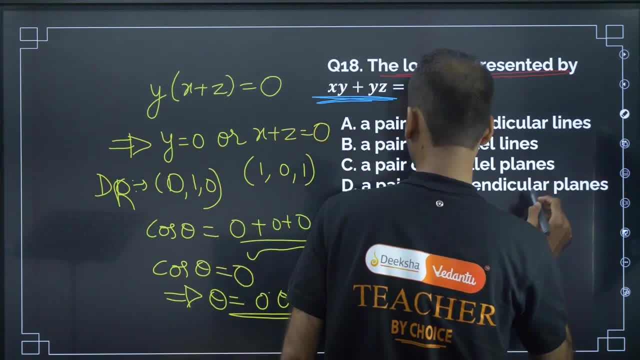 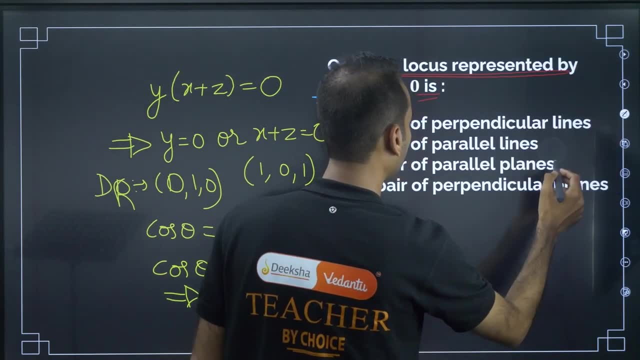 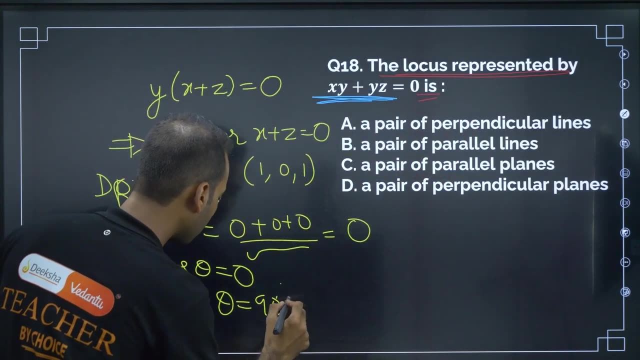 to 0. error is there? theta is equal to 90 degrees. theta is equal to 90 degrees. Here cos, theta is equal to 0.. theta is equal to 90 degrees, So theta is equal to 90 degrees. means pair of perpendicular. 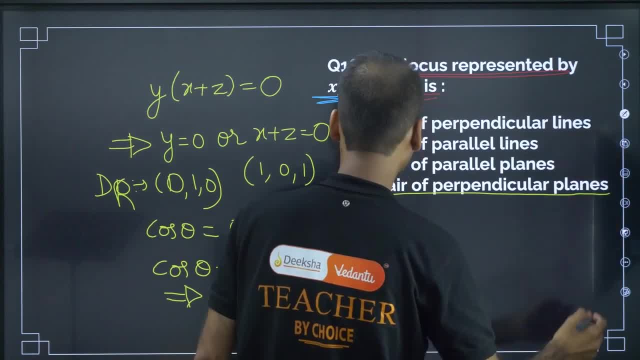 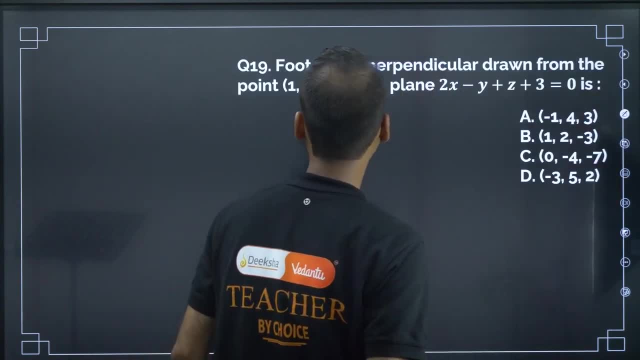 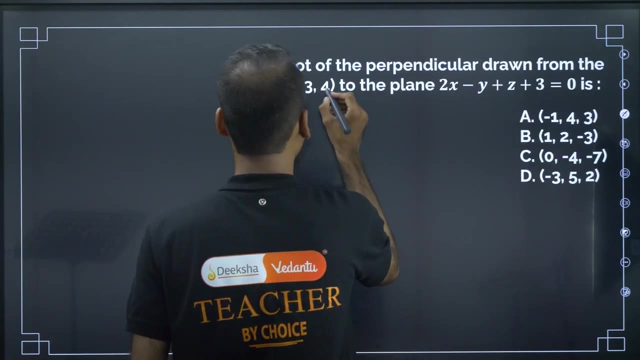 planes. this is pair of perpendicular planes. cos theta is equal to 0, when is 0? theta is equal to 90 degrees. So pair of perpendicular planes. moving on to next question, The foot of perpendicular drawn from to the plane is: what are they asking? They are asking to find. 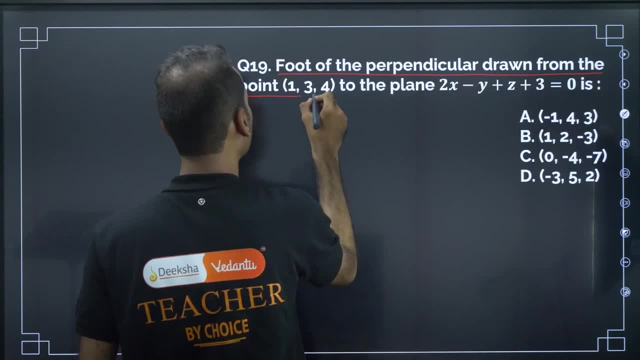 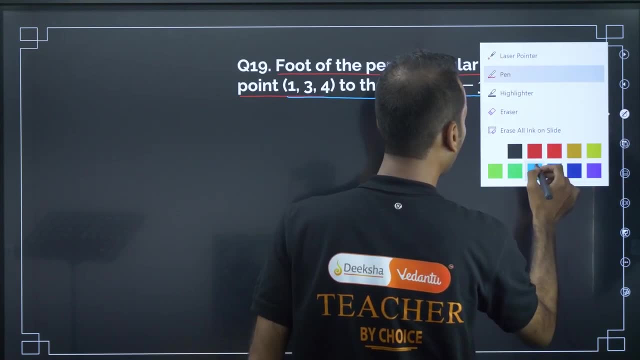 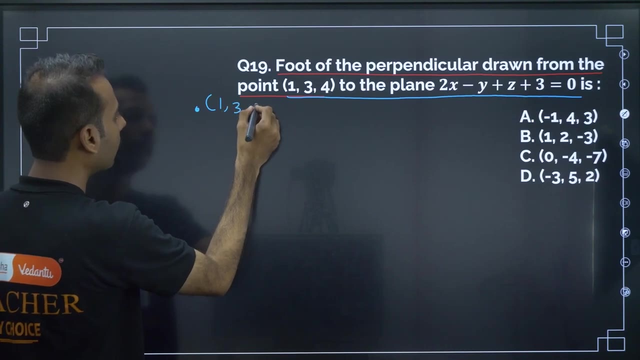 the foot of perpendicular drawn from point one point they have given from point to the plane is. So if I draw the diagram, things will be clear. the foot of drawn from point one point is there 1,, 3,, 4. one plane is also there: 2 x minus y, 2 x minus y. 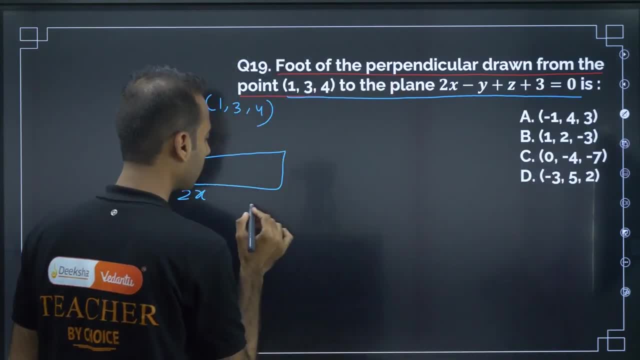 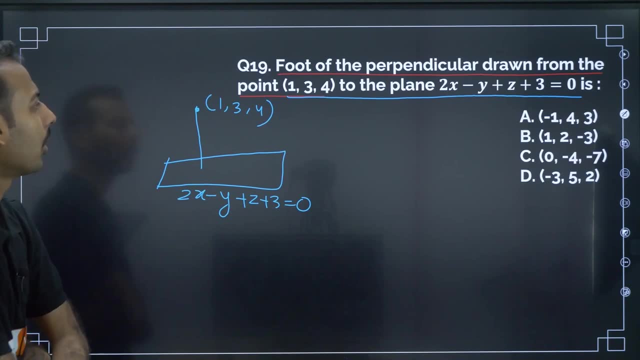 2, x minus y, plus z plus 3, is equal to 0.. Foot of perpendicular drawn from point to the plane. they are talking about foot of perpendicular. what are they talking? they are talking about foot of perpendicular drawn from point to plane. So if I name this as a, if I name this, 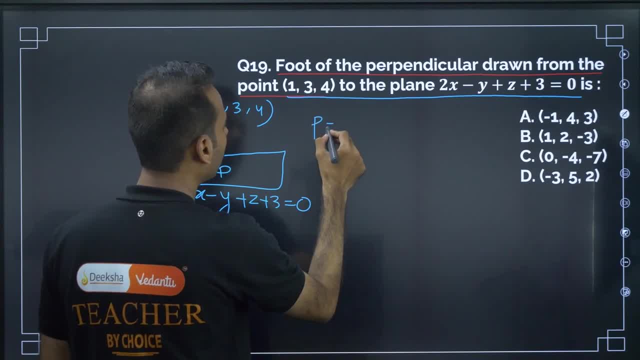 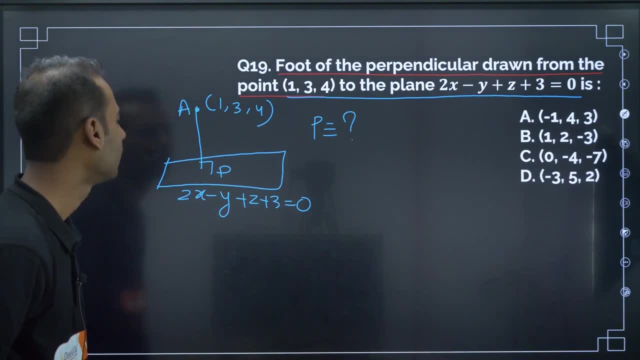 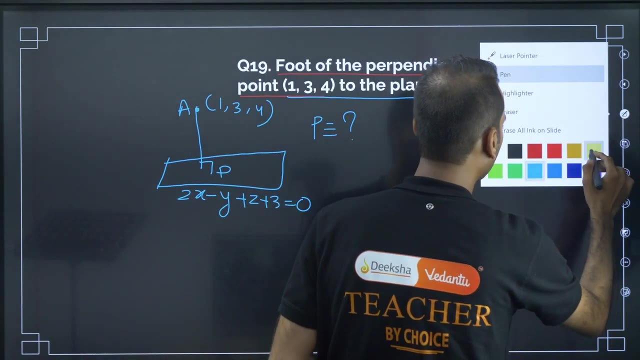 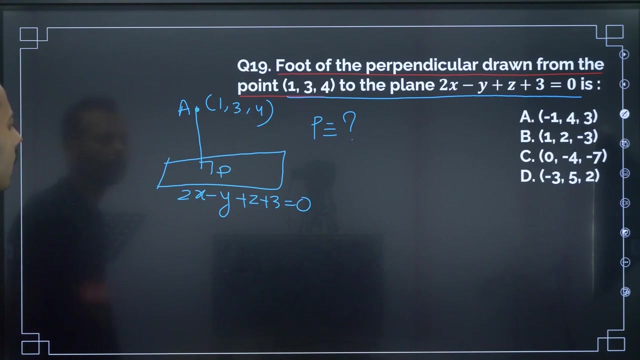 as p, foot of perpendicular drawn from point to plane. What are they asking? Foot of perpendicular drawn from point to the plane is So. they are asking this: how to solve this problem whenever foot of perpendicular they are asking to the plane, One plane they have drawn, 2 x minus y plus z plus 3 is equal to 0. Let. 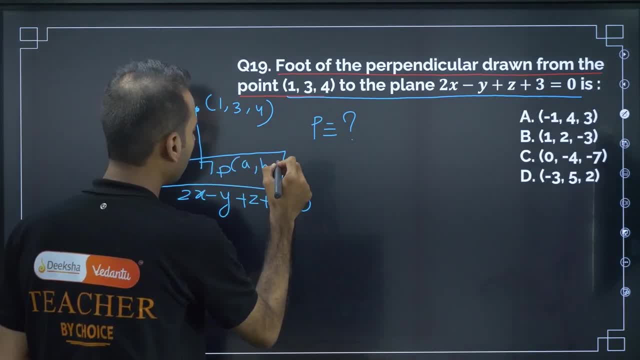 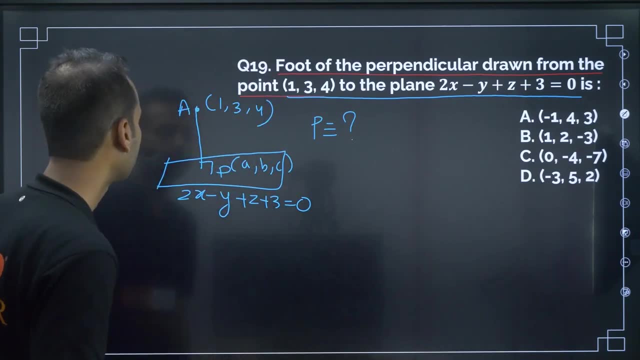 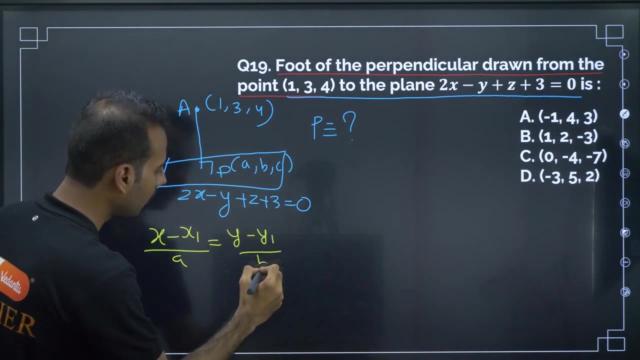 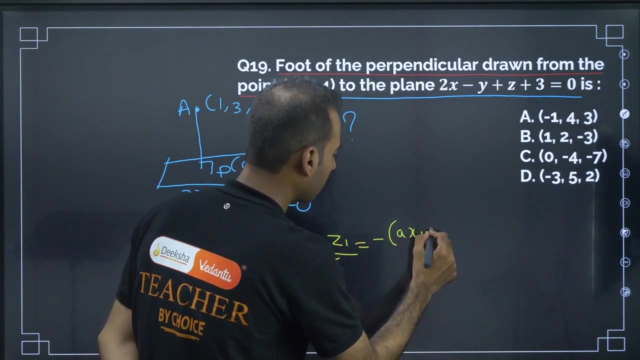 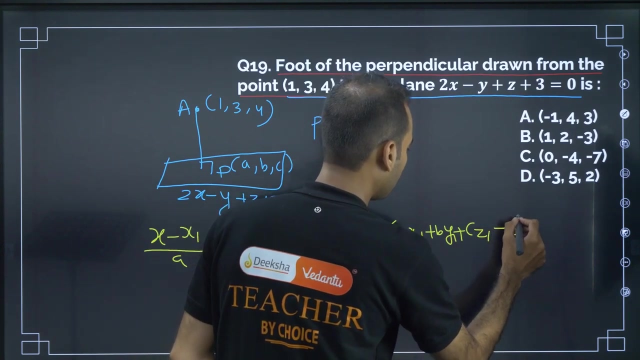 Let me go through the formula, if I name this as a, b, c, to find there is one formula. try to recall that formula x minus x 1 by a is equal to y minus y 1 by b is equal to z minus z 1 by c is equal to minus a. x 1 plus b, y 1 plus c z 1 c. z 1 minus d plus d by a square. 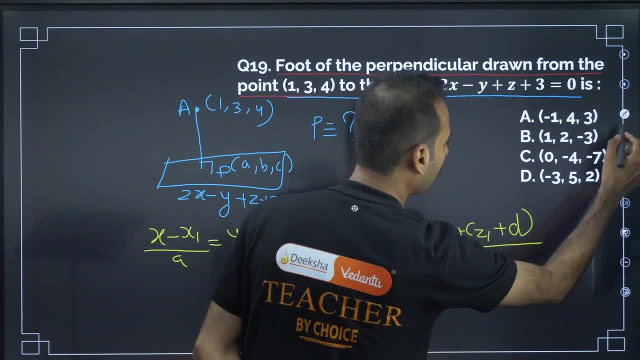 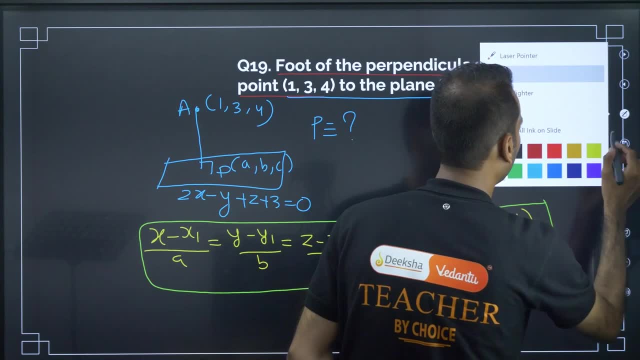 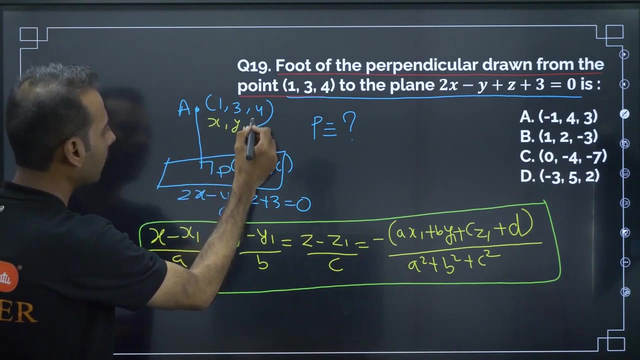 plus b square plus c square. Try to recall this synopsis point. try to recall this synopsis point: x minus x 1.. So if I mark this as x 1, y 1, z 1, by mark this as this will be x minus. 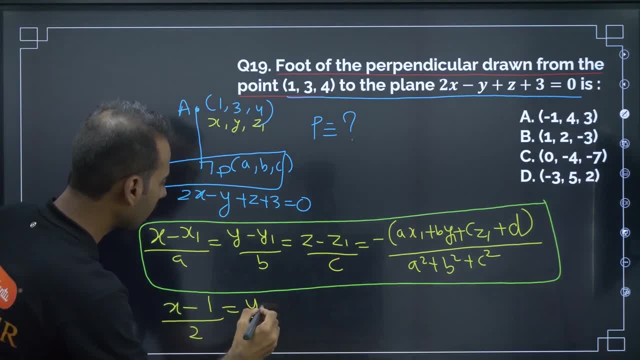 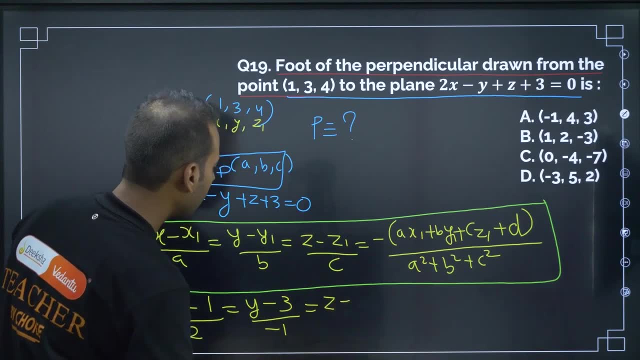 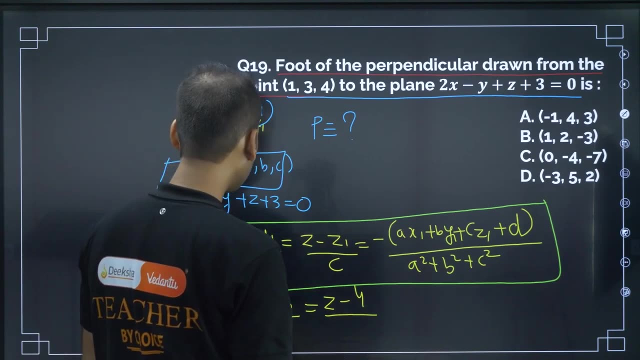 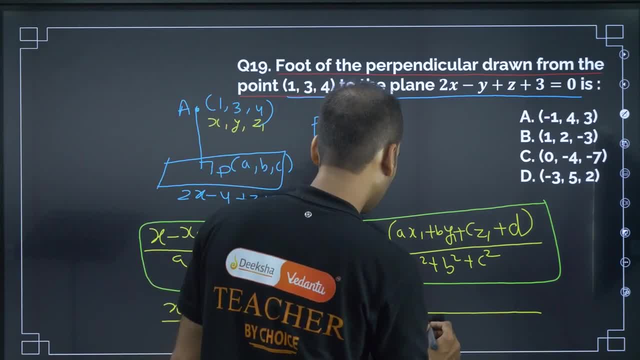 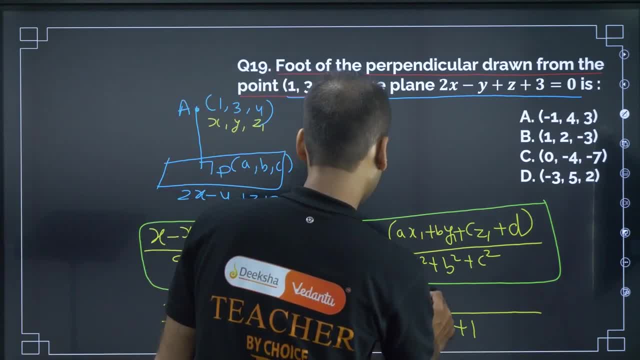 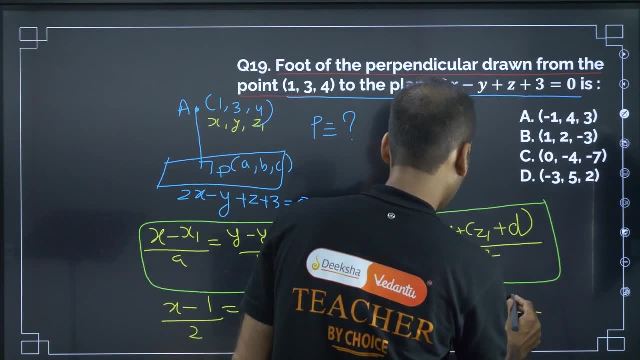 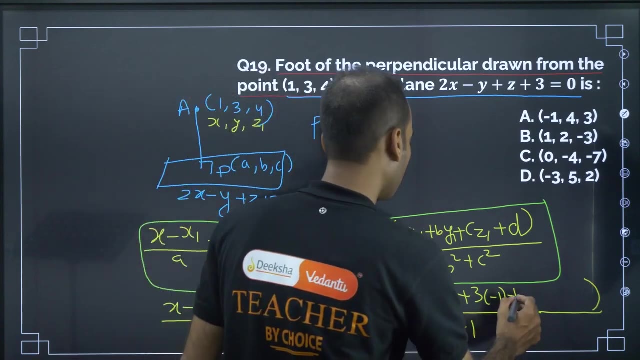 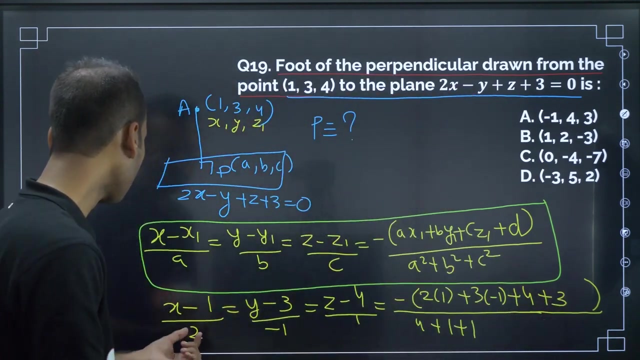 we have to substitute all this, So this becomes: 2 x 1 is 1 plus b, b is 3 and minus 1 plus c is 1, c is 1, c, 1 is 4 plus d plus d is plus. Now this equation we have to solve. 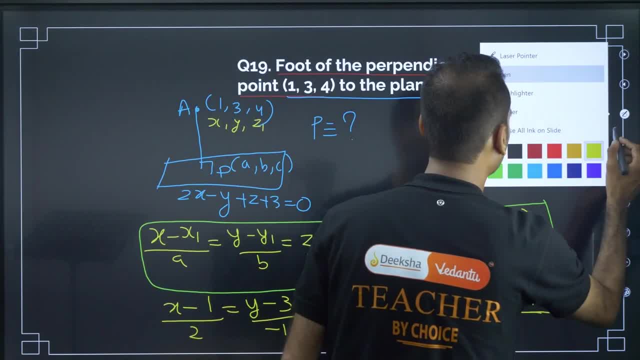 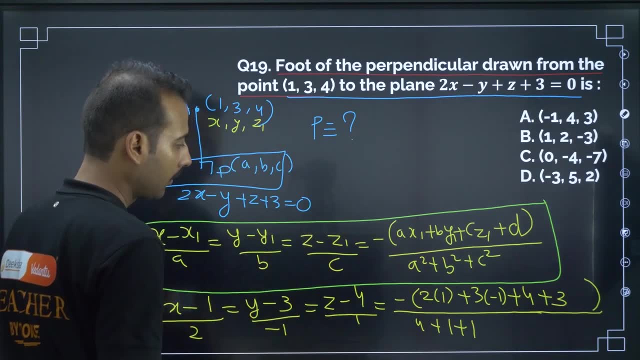 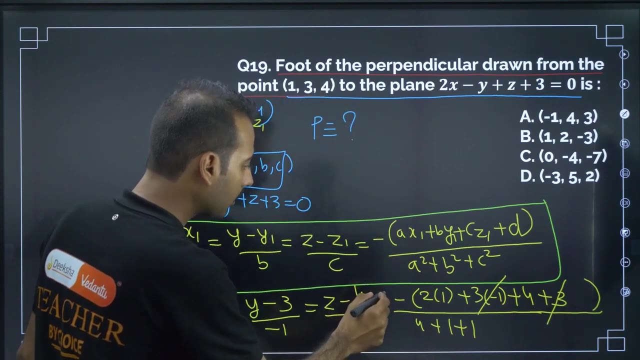 and then we will get some x, y, z value. So for that let me erase few things, or else here only, if I simplify: Positive 3. positive 3. 3 and negative 3 get cancelled minus 2 plus 4, negative 6 by positive 6, we are left with 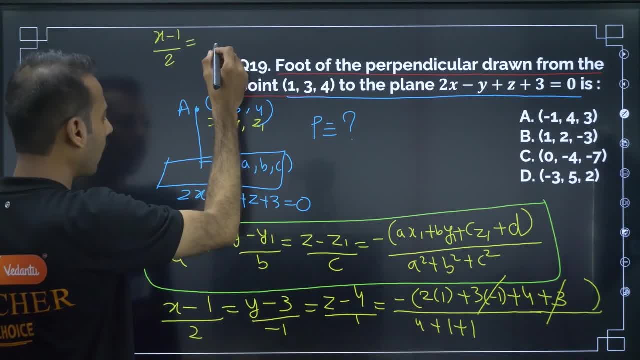 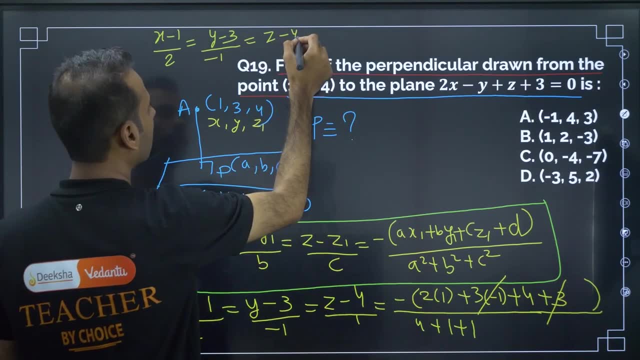 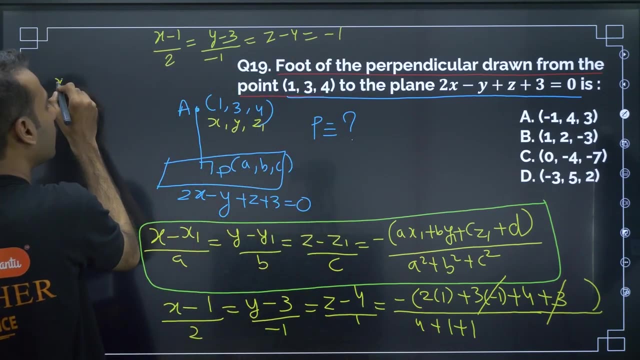 x minus 1 by 2 is equal to y minus 3. y minus 3 by minus 1 is equal to z minus 4 is equal to is equal to minus 6 by 6 is minus 1.. That means x is equal to minus 2 plus 1 is minus. 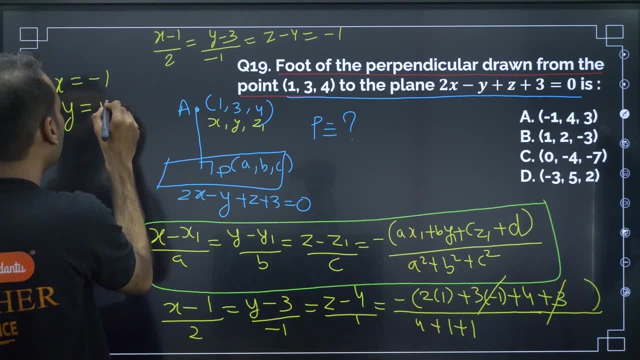 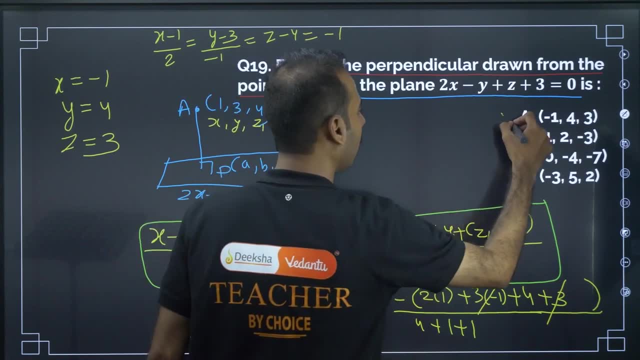 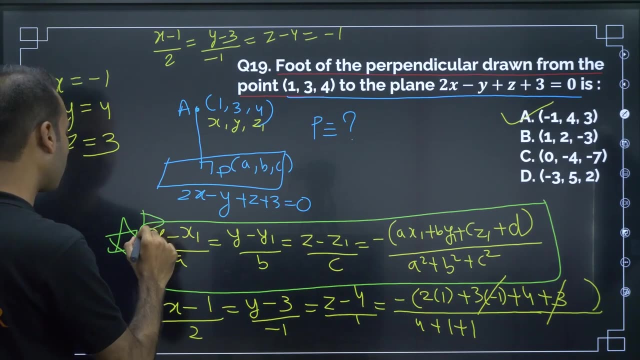 1. y is equal to 1 plus 3 is 4. z is equal to 1 plus 4 is 3 minus 1. 4. 3 is the answer. So the synopsis is this. this is the synopsis. very, very important synopsis there are so. 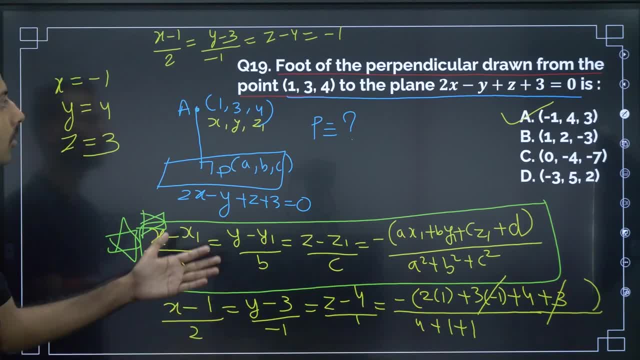 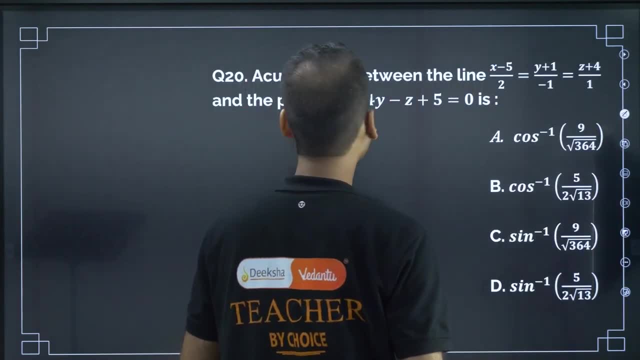 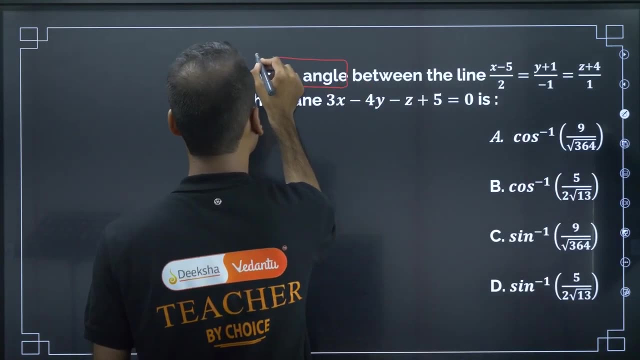 many problems based on this x minus x, 1 and all these things just go through this. if you know this formula, this problem, you can solve it easily. Moving on to next, the acute angle between line and plane is: So what are they asking acute angle? they are asking acute angle between: 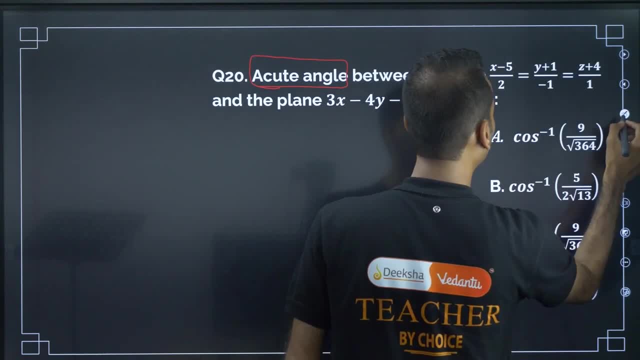 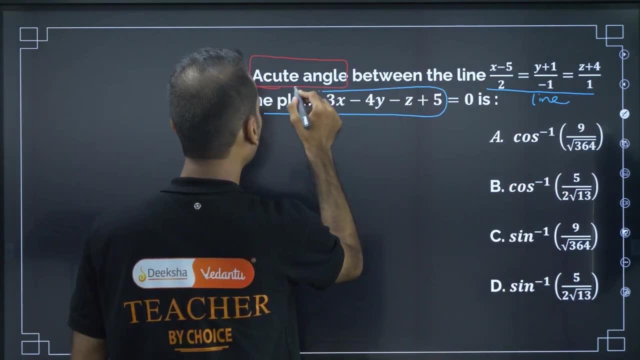 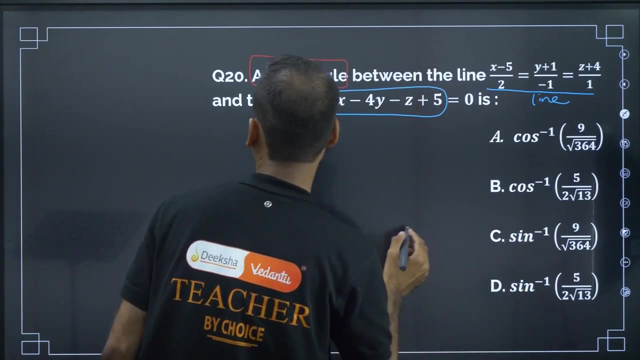 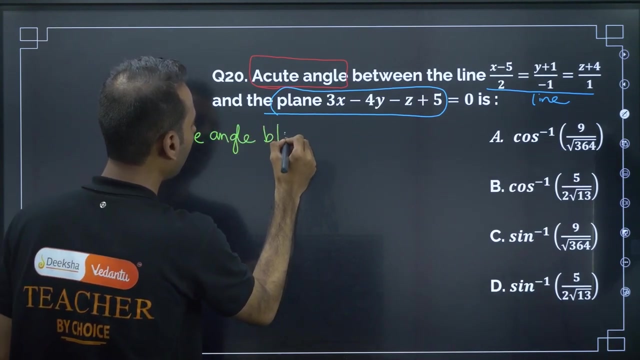 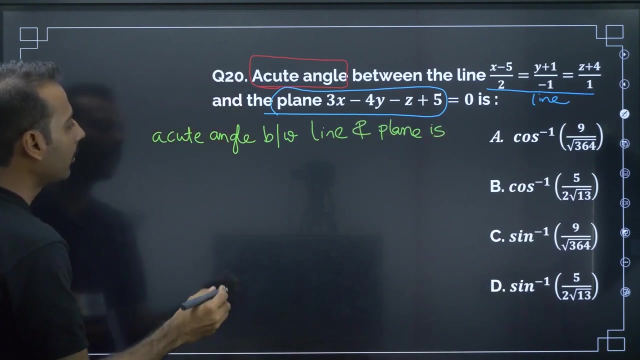 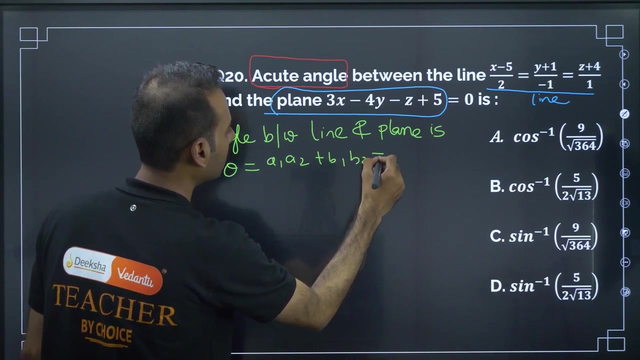 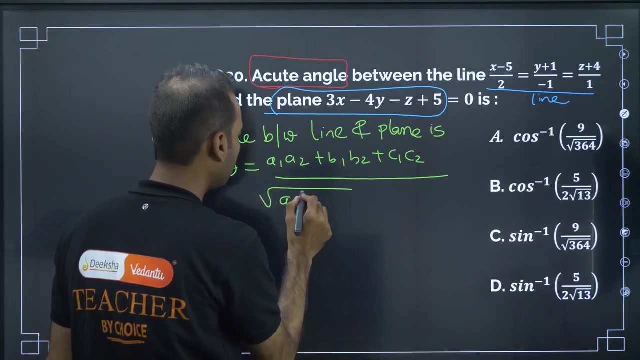 between what one? between line, between line and plane? they have given one plane. acute angle between line and plane is, So try to recall the formula: acute angle. acute angle between line, entire line and plane, between line and plane is acute. angle between line and plane is sin. theta is equal to a: 1 a, 2, b, 1 e, 2, c, 1 c, 2 by root of a: 1 square one. b 1, c 1, root of a 1, a 2, b 1, e 2, e caps a 1 square b 2 square c 1, and we just multiply them, Timeline these: I mean n angle and n angle in a way by magnitude sine t of e 1, that means minus 1 in错 and the 32 percent of the basic mod of a 1, which is 1.e square. So, since we have got r square s and for Boyan here red was because r square s, which is going to be 5, we are going to be for r square c and then gradually you will have the 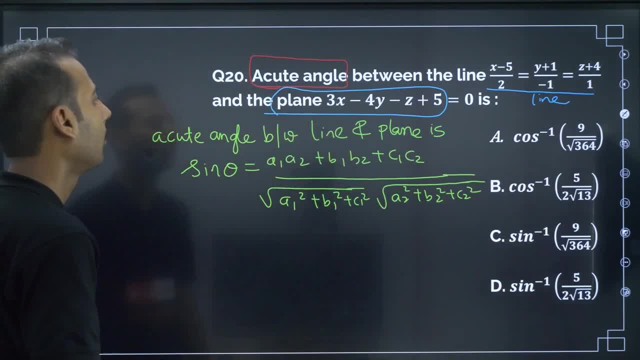 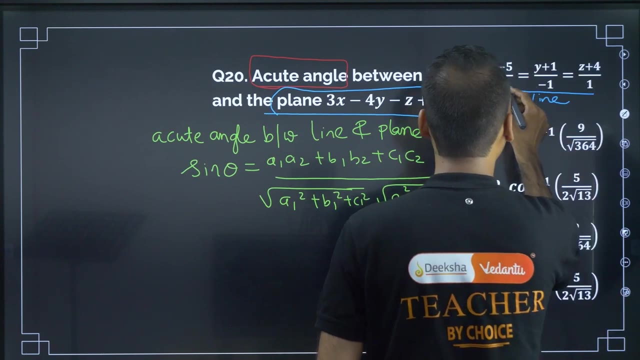 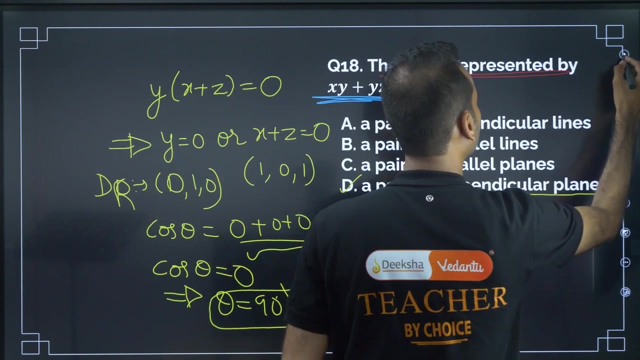 c 2 square. cute angle between this line and this plane is. So they are talking about. cute angle between line and plane is. Now we know few things from the synopsis. try to recall the synopsis for this. you mark this as a 1, b 1 and c 1 and this as c 1.. Also, 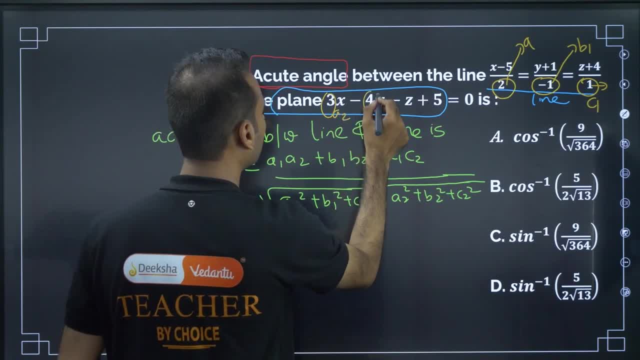 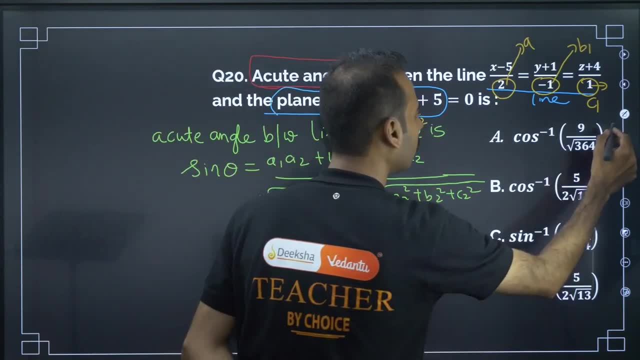 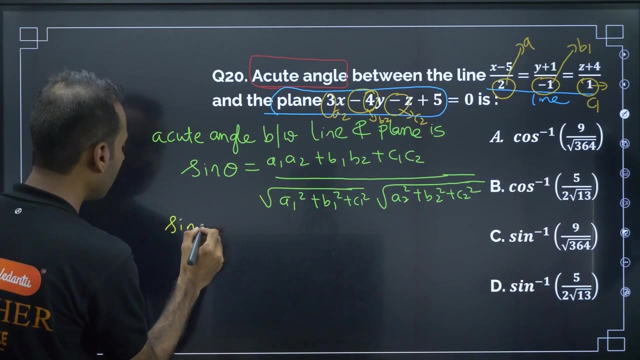 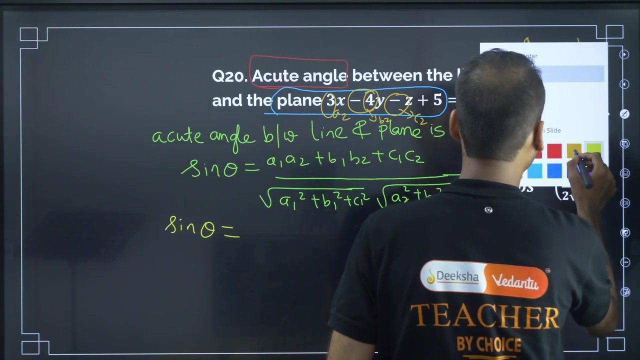 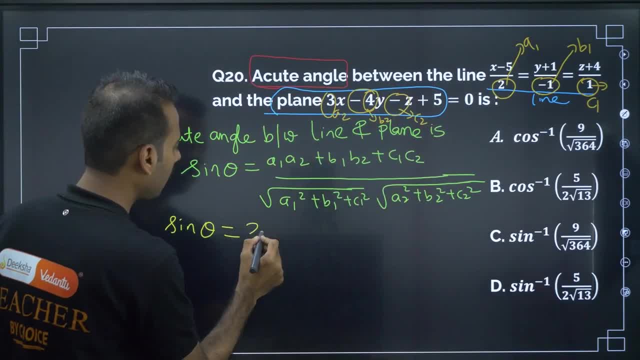 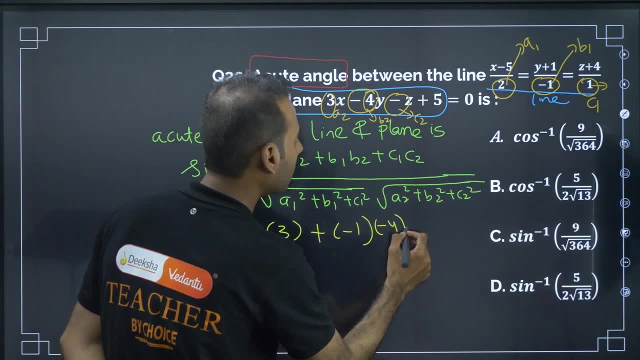 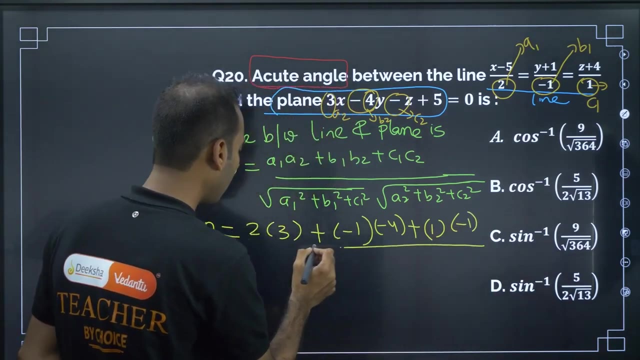 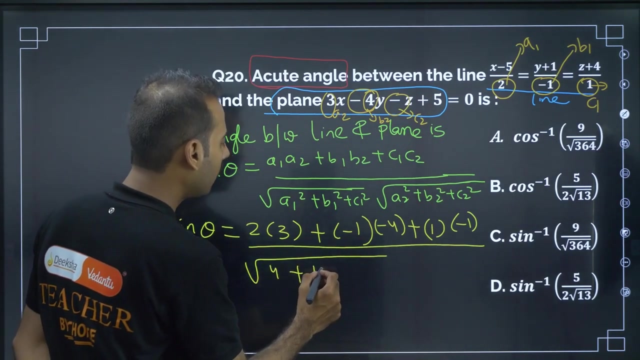 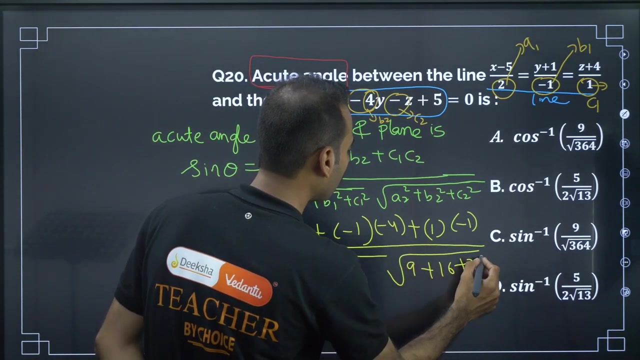 1 is a1 is 2, a2 is 3, 2, 3, b1 is minus 1, b2 is minus 4, c1 is 1, c2 is minus 1. by root of a1 square, b1 square, c1 square. a1 square is 4, 1, 1. root of a2 square is 9, 16, 25.. 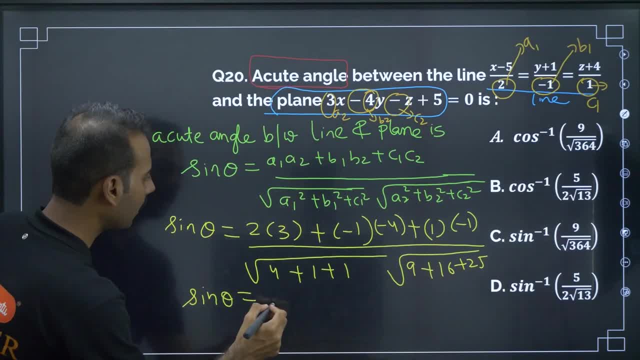 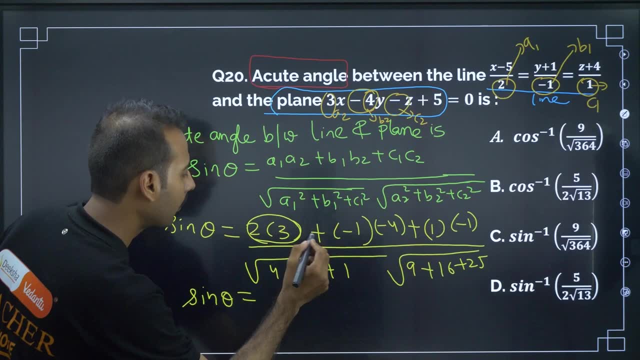 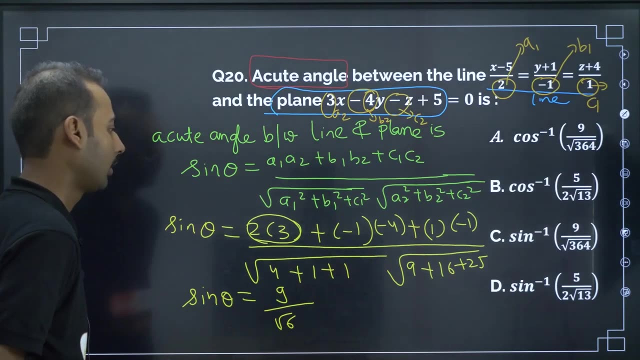 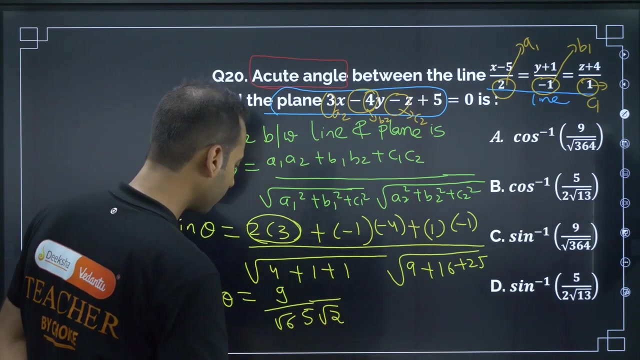 So sin theta is equal to sin theta is equal to. so if I solve this, 6, 6 plus 4, 10 minus 1, 9 by root of 6 root 20.. So root 50, root 50 can be written as pi root 2, pi root 2.. 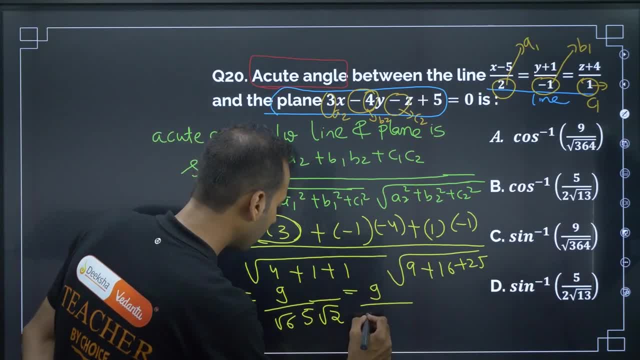 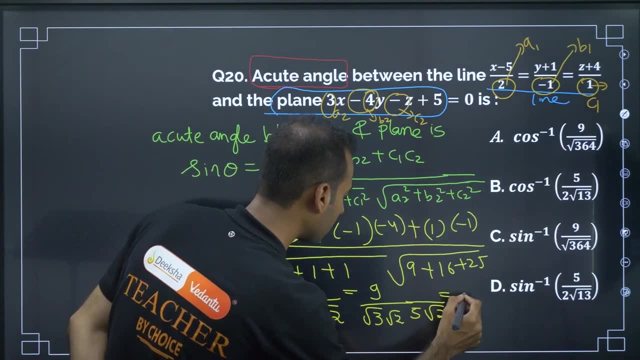 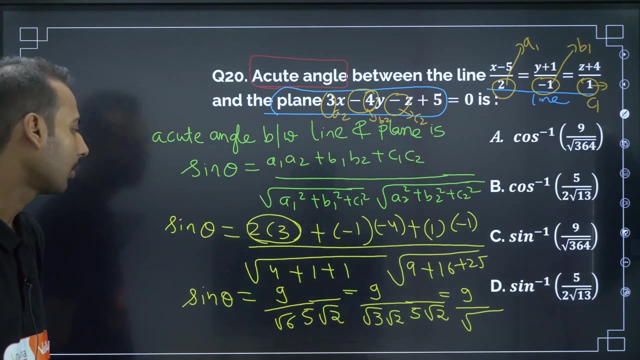 So sin theta can be written as 9 by root, 3 root 2 and then pi root 2, or else this can be written as 9 by root of. if you multiply everything what you will get, 6 to the power 12.. 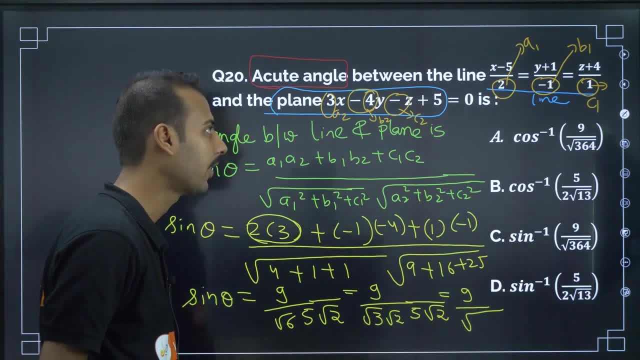 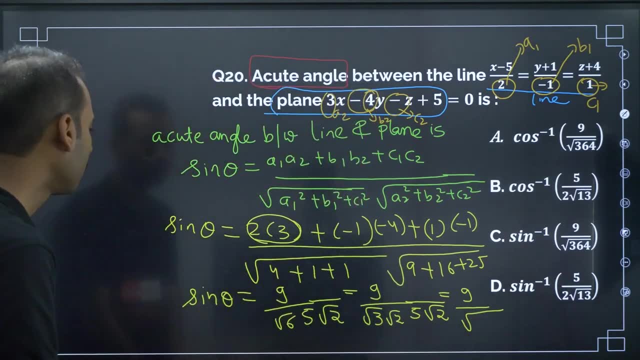 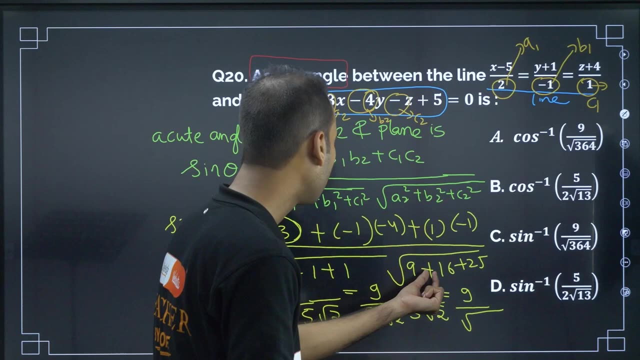 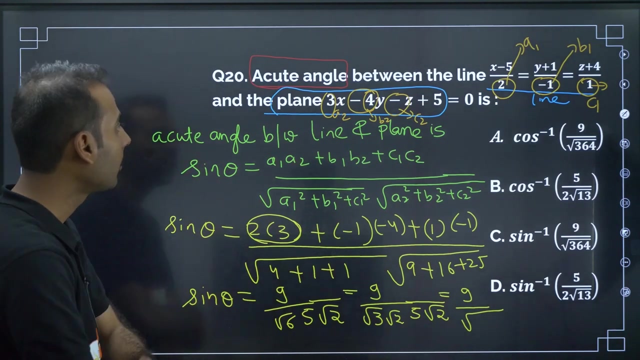 12 into 25,, 25, 12, I think it will be 300.. Once you check sin, theta is equal to 9 by- I hope there is no calculation error- 16, a2 square b2 square, 9, 16.. 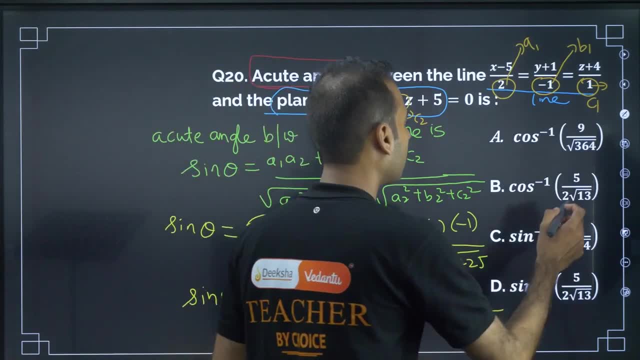 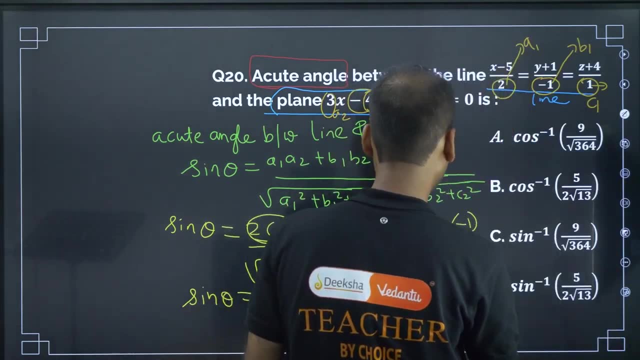 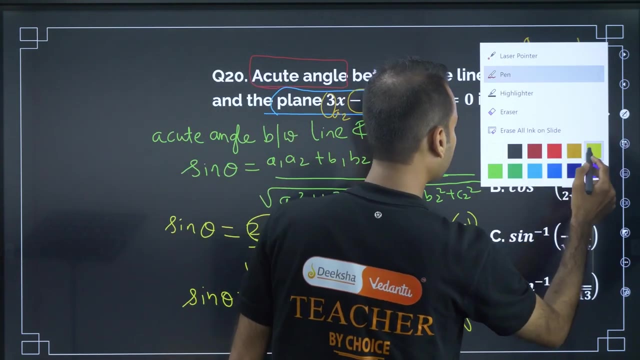 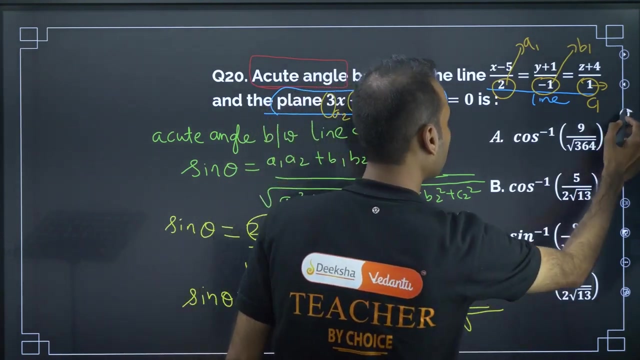 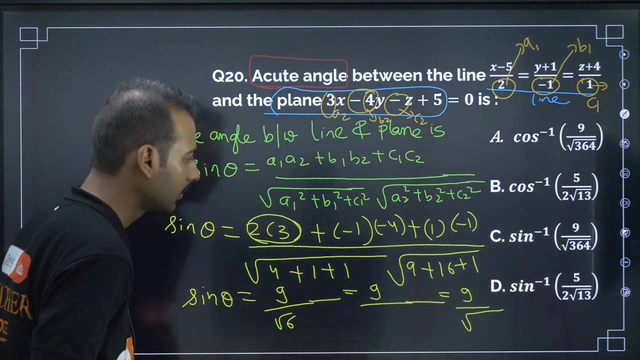 Ok, Ok. Ok, Ok, There is some calculation error. by mistake. I have written this Error. what is this? Here? it should be 1, 1. So root 6 and root 26. 26.. So this is a 2 square is 9, 16,, 9, 26, root 26.. 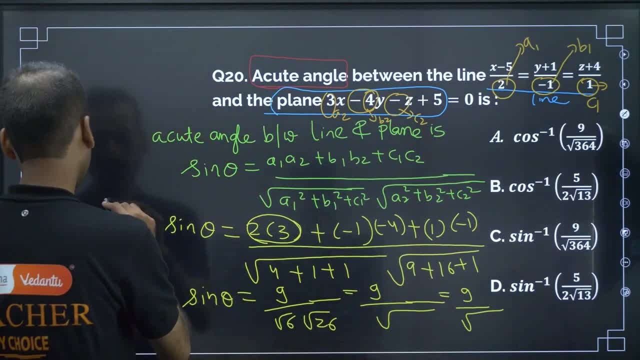 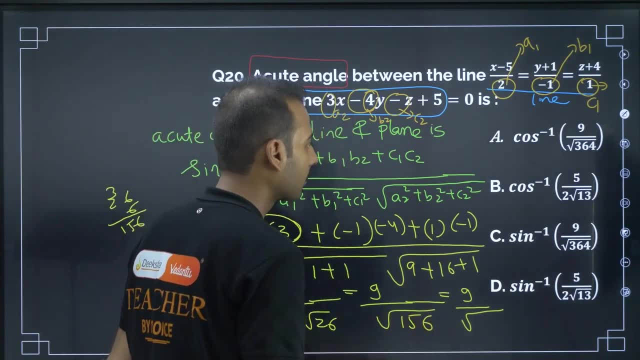 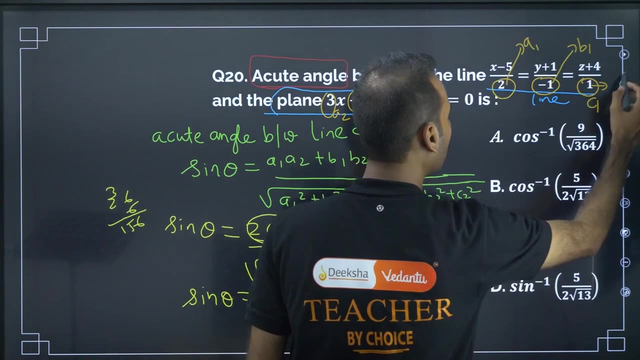 So this is 26 into 6, 26 hexa, 6 hexa 36, 3 carry 6 to the 156. So this is 156.. 9 by root of 156.. Now, if you go through the options, they are not given in terms of, let us say, if you. 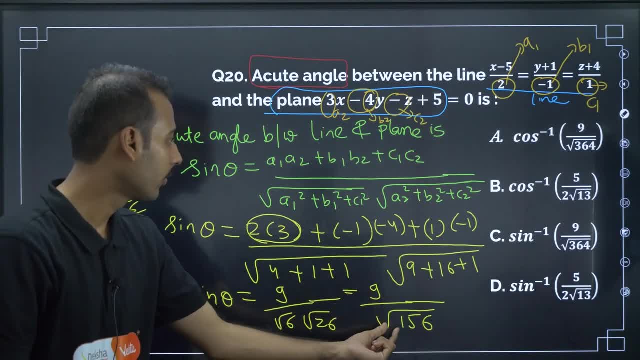 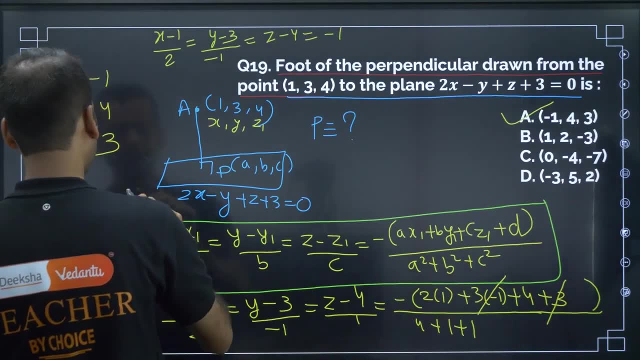 take sin theta is equal to 9 by root 26,. it is not readily available, so you can take sin theta if you are not comfortable with this. it is not readily available. Also, if you want to change your equation, you can use a temas from the first row. 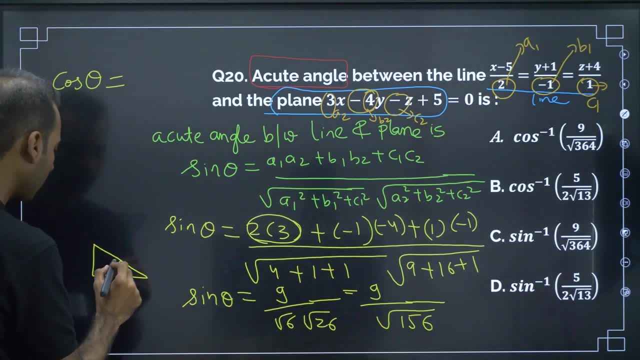 sin theta is equal to 9 by root 26,. it is not readily available, so we have to transform this to cos. So let me erase this thing. Cos theta is equal to cos. theta is equal to sin. theta is equal to 9 by root 56 means. 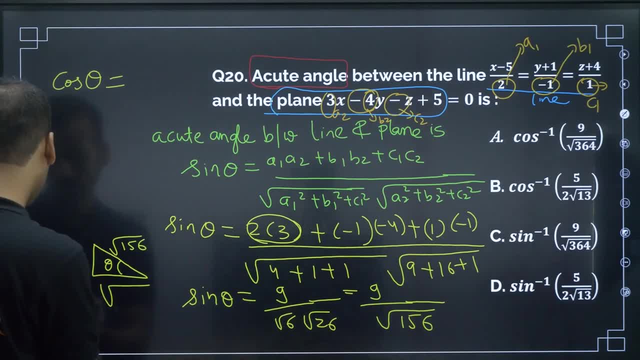 if I mark this as theta, this is perpendicular and this is 156.. Now, if I take root of 156 plus 87, 156 plus 86, 156 times zero, 817237, 237.. So let me name this as 156 minus 81, or else 15621575. 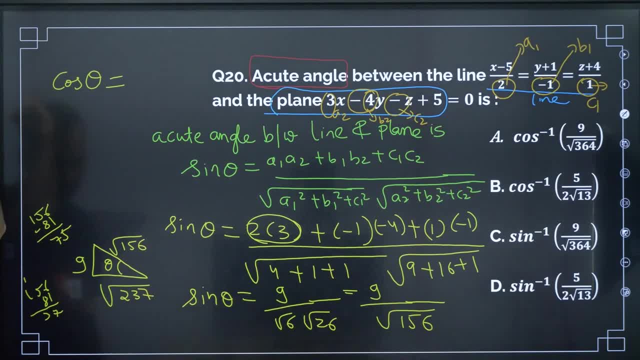 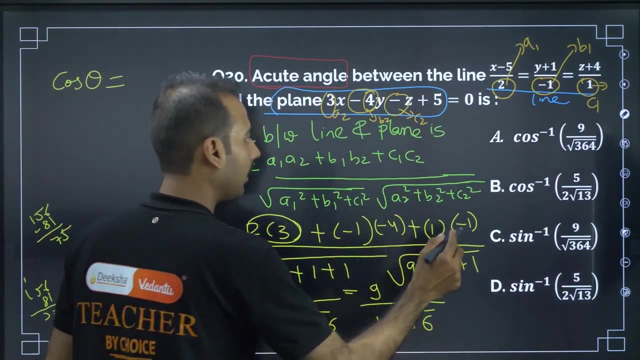 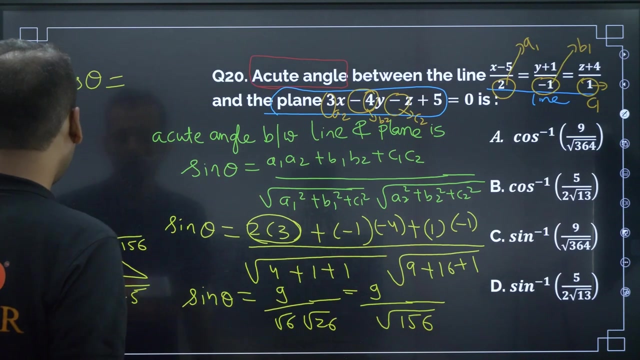 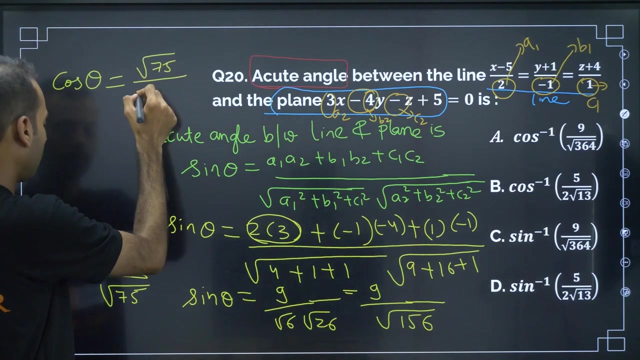 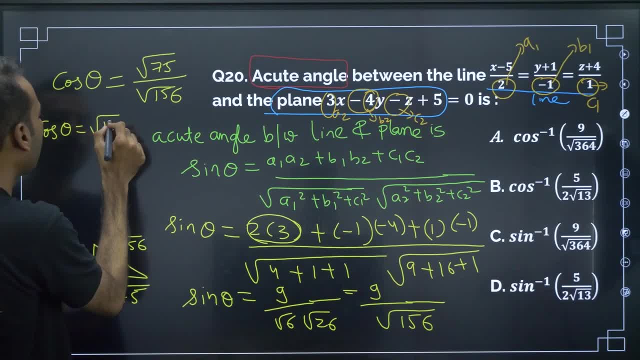 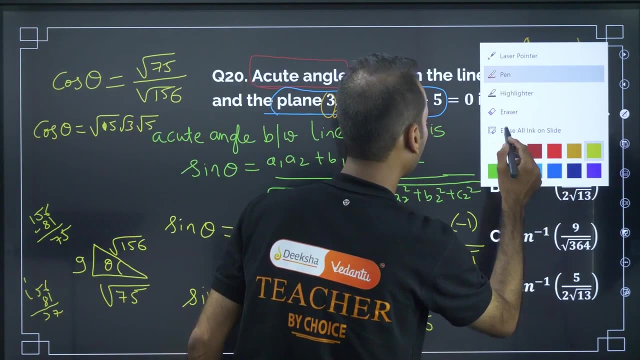 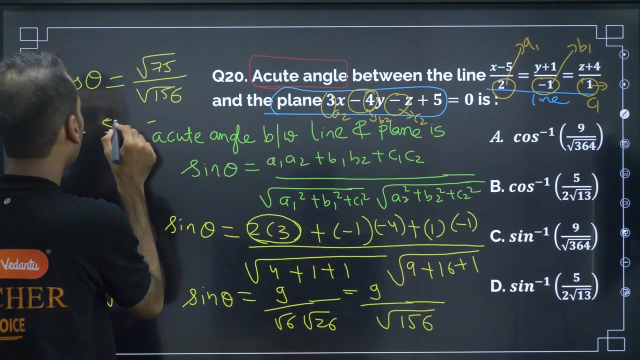 if I simplify cos theta, this can be written as root 15 or root 5, root 3, root 5, root 3, root 15, 15 phi is a phi root 3 or you can write this as phi root 3, phi root 3 and denominator. 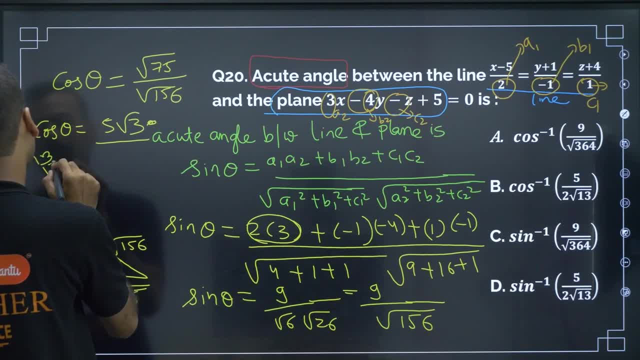 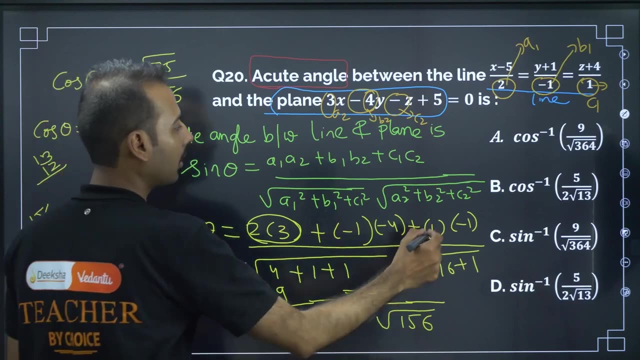 root 156 can be written as 13 into 12, 13 into 12.. So root 13, 12 can be written as 12 can be written as 15.. So this can be written as 2 root 3.. So if I cancel 2 root 3, 5 by 2 root 13, b is the 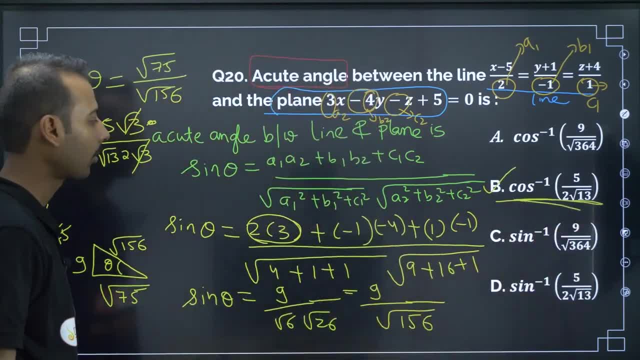 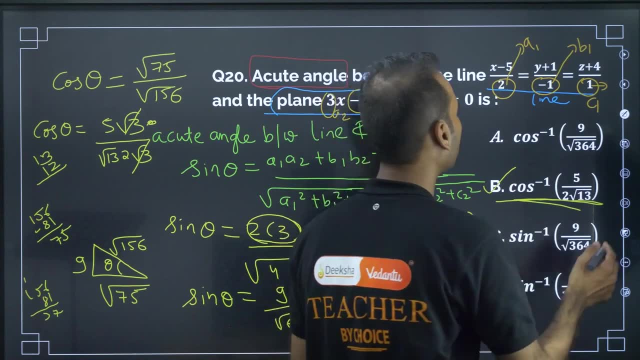 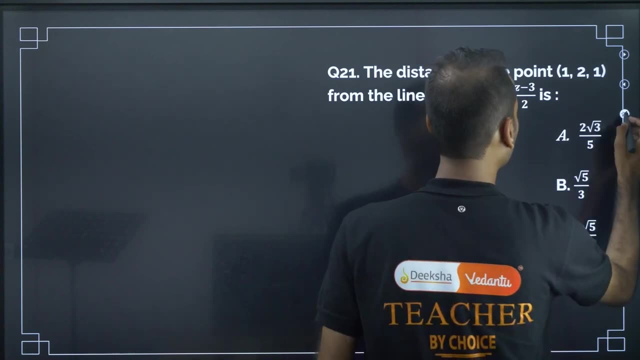 answer: 5 by 2 root 13.. It was easy problem only just sin theta. only simplification. it will take time. if you are not good in simplification, it will take time. if you are expert, then you can see your time there also. Next, the distance of the point 1 to 1 from the line is So: 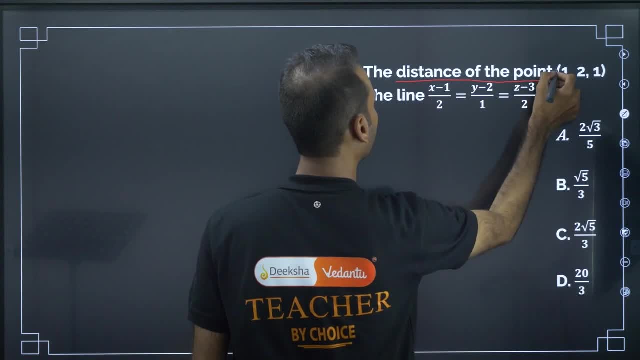 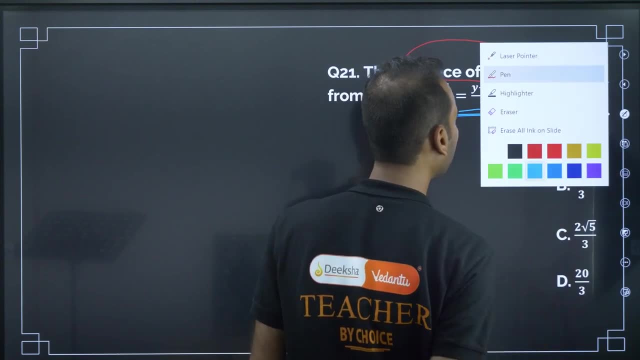 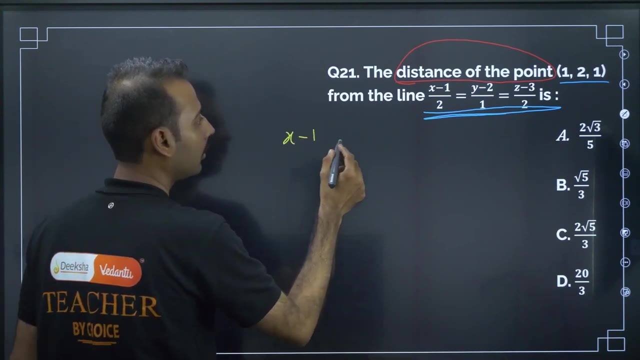 the question is, what are they asking? they are asking to find distance of the point, distance of the point From one point they have given. what is that point from this line is? So how to find distance between point and line? let me consider that line as x minus 1. this x minus 1 by 2 is equal. 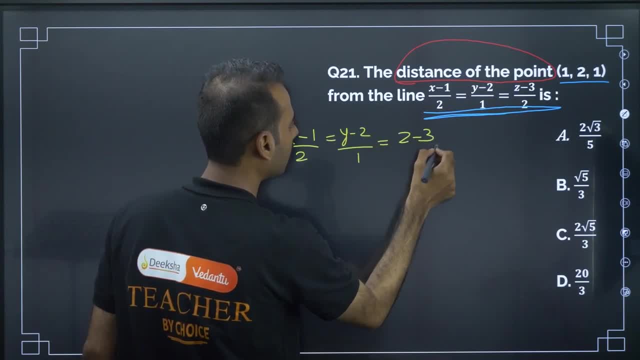 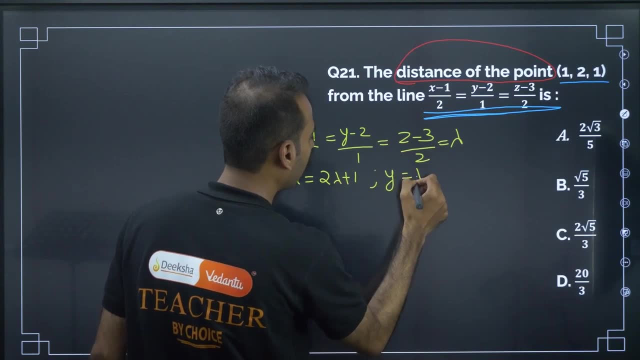 to y minus 2 by 1 is equal to z. minus 3 by 2 is equal to lambda. x is equal to 2 lambda plus 1. y is equal to lambda plus 2. z is equal to 2 lambda plus 1.. 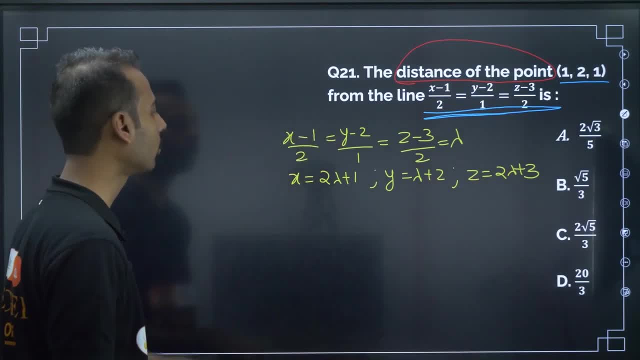 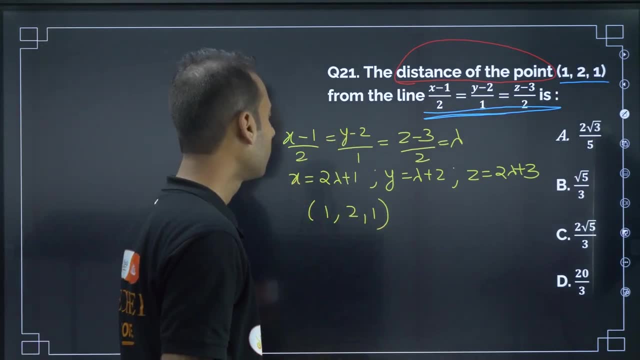 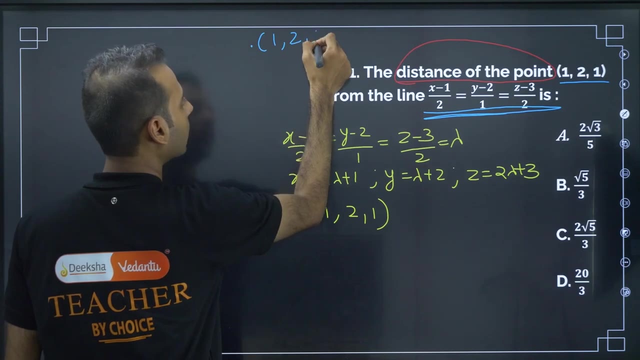 The distance of the point 1 to 1,, 1 to 1 from the line, from that line is. So if I draw the diagram, maybe things will be clear. 1 point: they have considered 1, 2, 1 and one line. 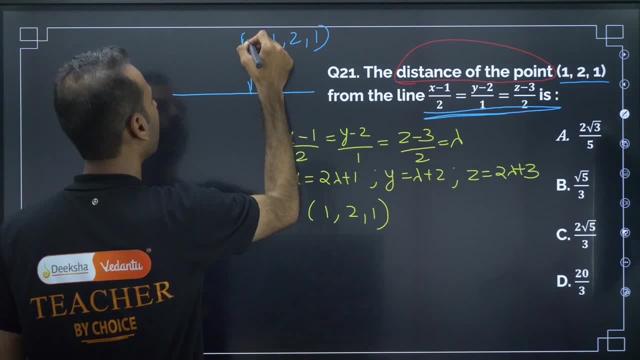 they have considered. let me mark this as A and let me mark some, point P and that line for which x, x. we got this as P points. they have lead- series from point and now from point they have a gap. If we call refugees or whatever, is there somewhere P will come. I won't e this, just e. let me talk about here and calculate a value from a value from thecedar or looking for the above. I can put P to E. dot were the two people And you can see that I can. 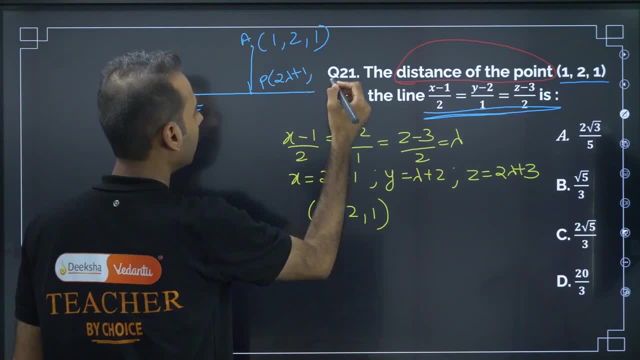 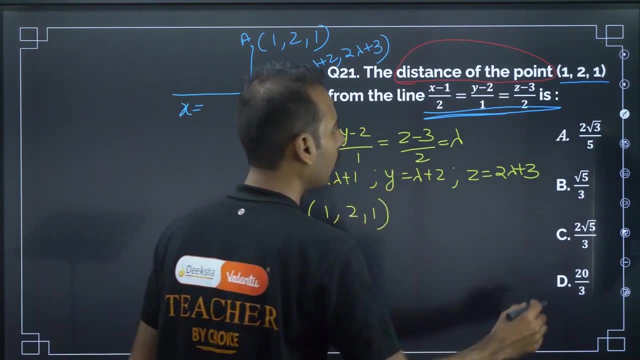 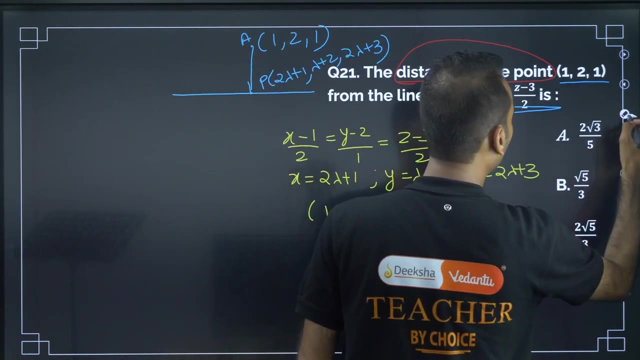 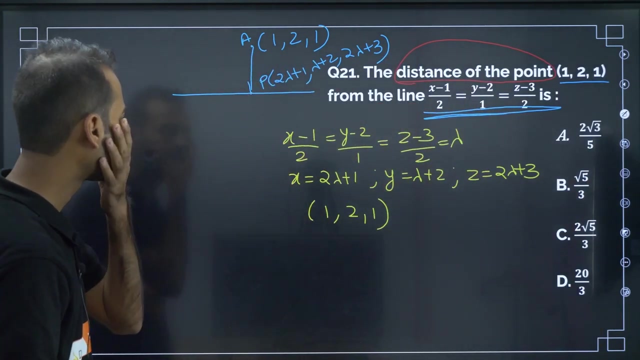 so this point will be 2 lambda plus 1 and lambda plus 2, and then 2 lambda plus 3. let me remove off this now. in one of our previous problems we have already did such type. the distance of the point from this line is so. so if i 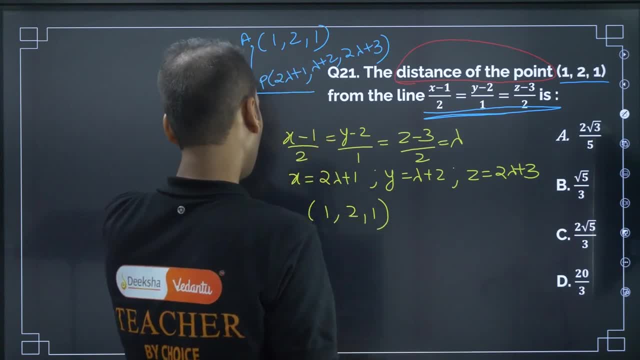 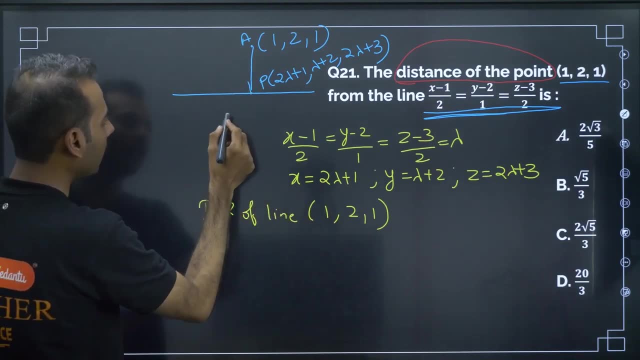 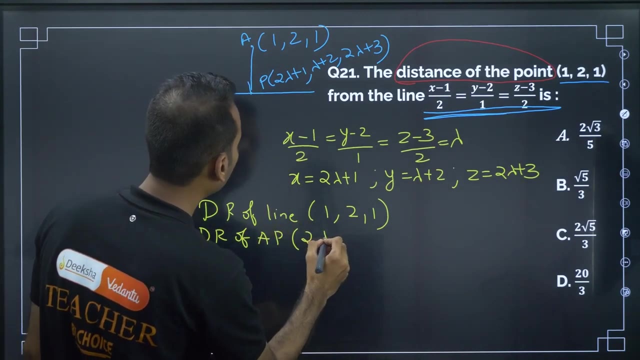 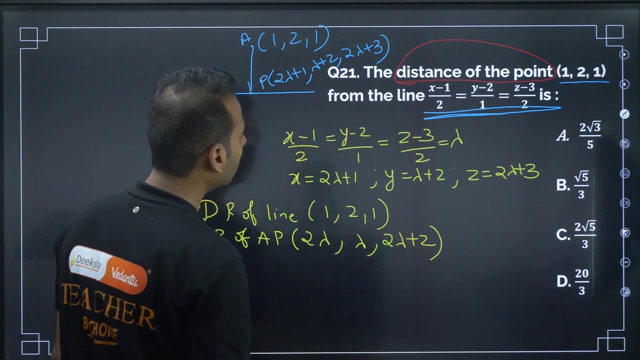 huh now, direction ratios of direction ratios of line. is this direction ratio of ap. direction ratio of ap is 2 lambda, 2 lambda lambda plus 2 lambda. 2 lambda plus 3 minus 1. 2 lambda, 2 lambda plus 2, 3 minus. 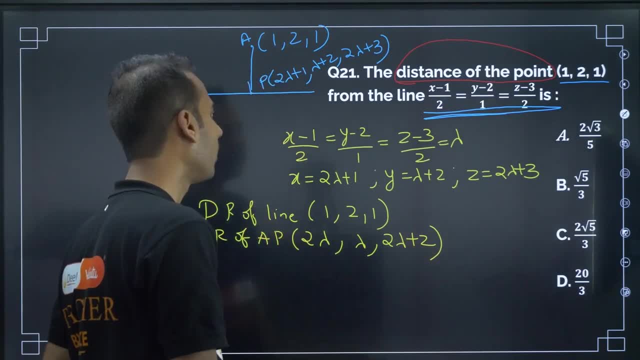 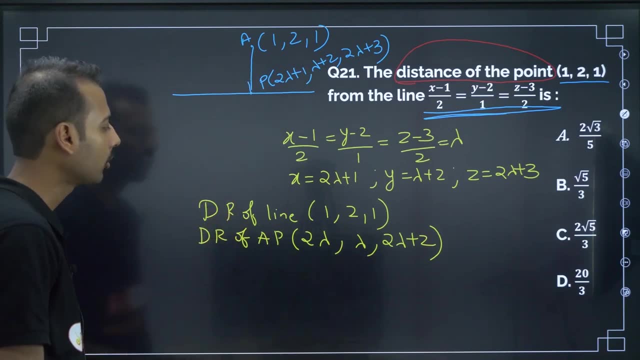 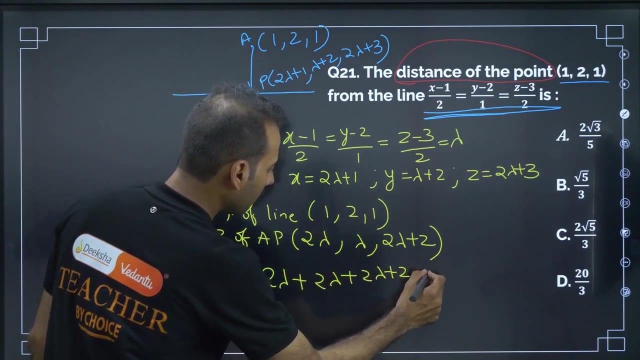 his of pedir 1 is 2.. So direction ratio of line, direction ratio of AP. we got this Also. now you try to recall, these two lines are perpendicular. these two lines are perpendicular, that means cost will be 0. So 2 lambda plus 2 lambda plus 2 lambda plus 2 is equal to 0, 2 lambda. 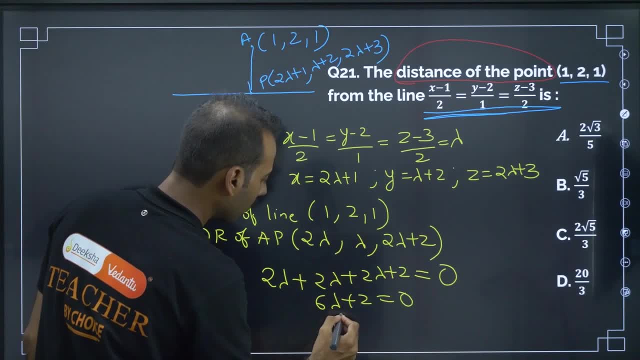 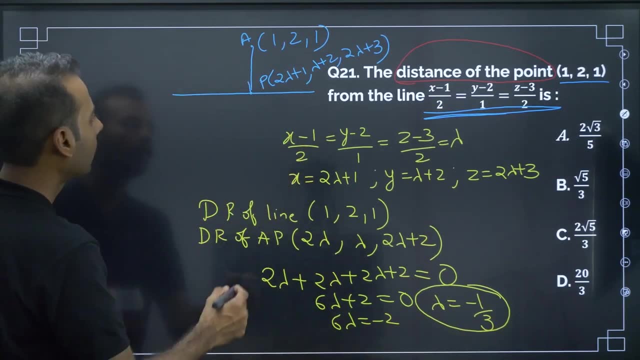 2 lambda, 6 lambda plus 2 is equal to 0. So 6 lambda is equal to minus 2 lambda is equal to minus 1 by 3, that is equal to 1.. If I substitute this P, P point becomes: where is? 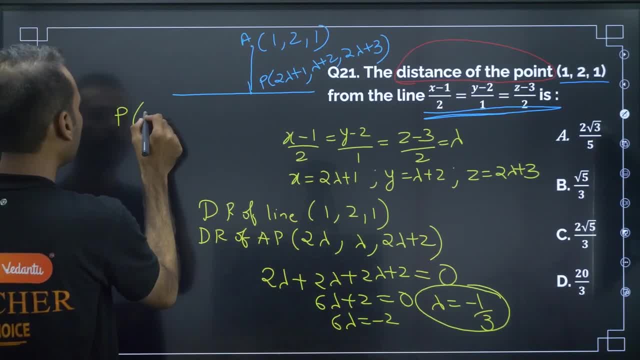 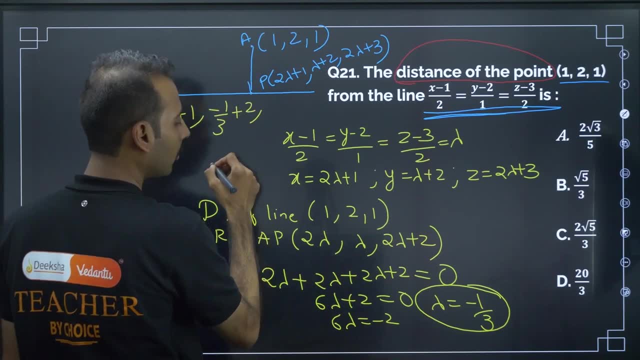 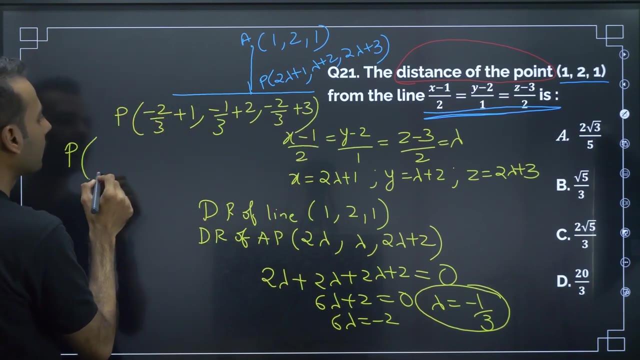 this P point. P becomes 2 lambda. 2 lambda is 2 by 3 plus 1, lambda is minus 1 by 3 by 3 plus 2, 2 lambda is minus 2 by 3 plus 3.. So P point becomes, if I simplify this, minus. 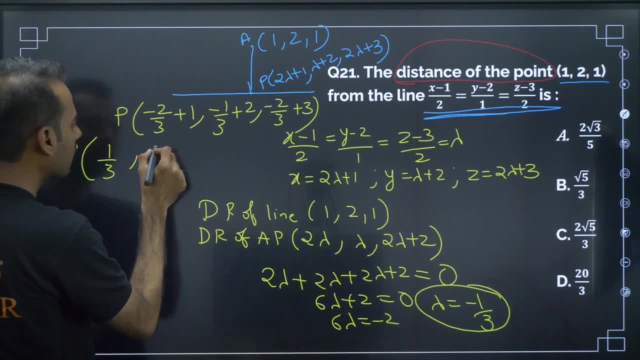 2 plus 3 is 1 by 3. Next, minus 1 plus 6. 5 by 3 minus 2 plus 9 is 7 by 3. So P point is minus 2 plus 3, 3, 1. So I hope all this. 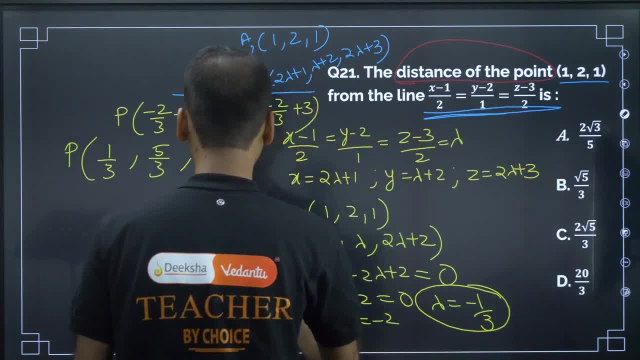 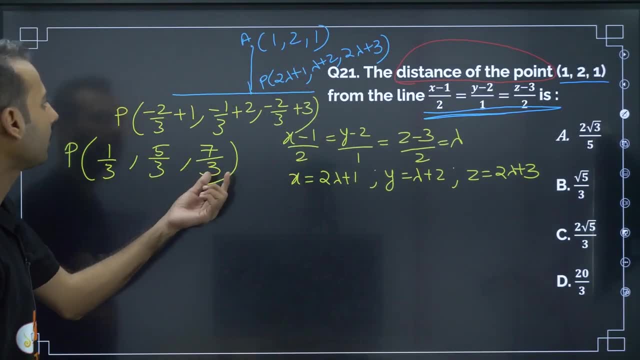 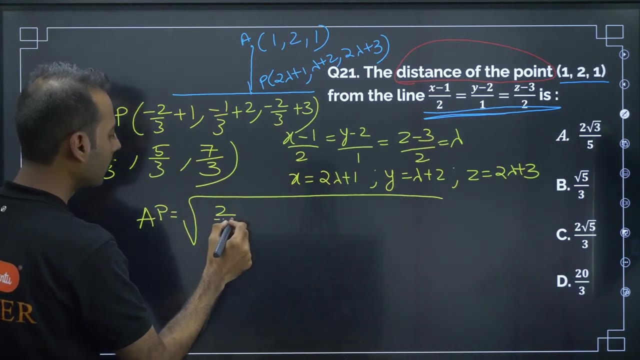 is correct. Moving on to let me remove some things: direction ratios, all this just space constraint. because of space, P: 1 by 3,, 5 by 3,, 7 by 3.. Now AP: for AP, if I use distance formula, root of 1 minus 1 by 3 is 2 by 3.. So P point is minus 2 plus 9 is 7 by 3.. So 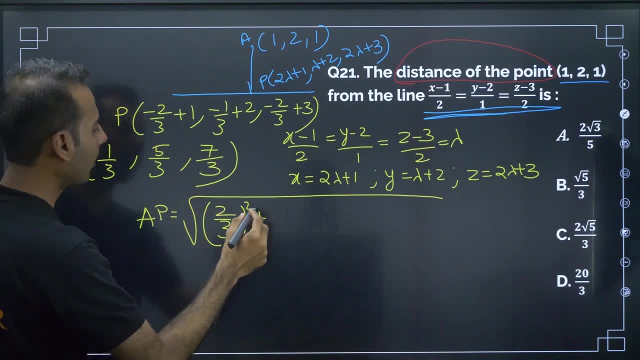 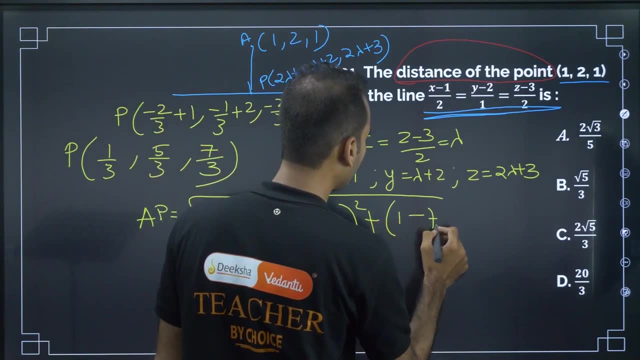 P point is also for less than or equal to 1 by 3 square plus 0.. If I Tom A dot Wash, 2 by 3 square plus 2 minus 5 by 3, 1 minus 5 by 3 square plus 1 minus 7 by 3: 1 minus 7. 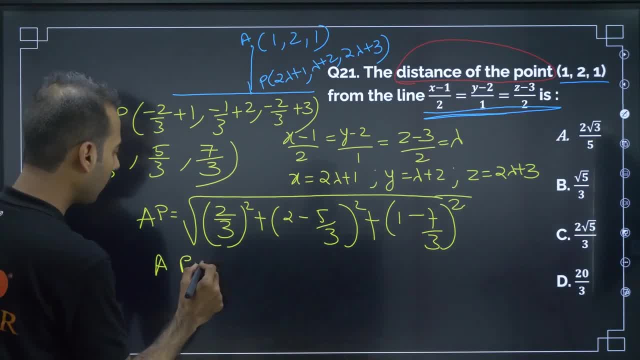 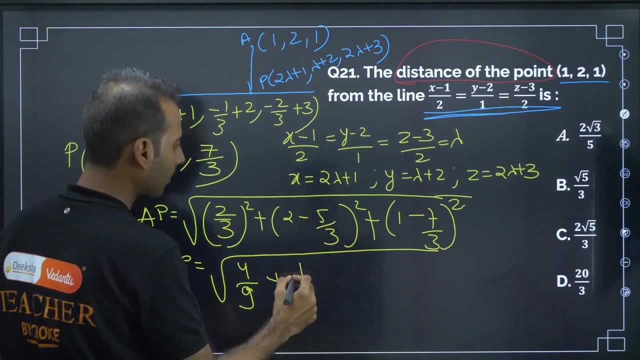 by 3 square, So AP is equal to root of 4 by 9. 4 by 9 plus 6 minus 5 is 1 by 3 square plus 3 minus 7 minus 4 minus 9, 4 by 9.. If I draw this in this formula, I have to find the components. 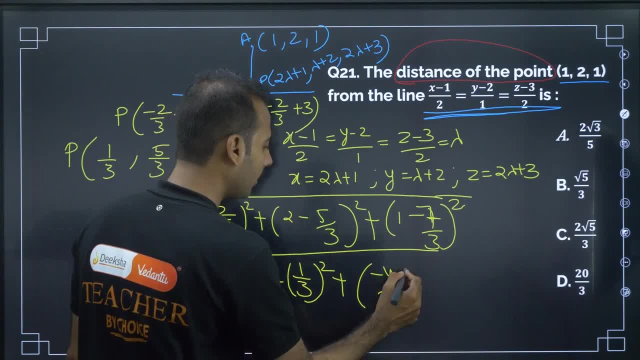 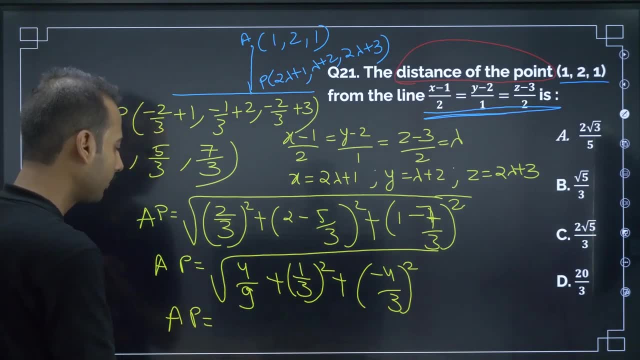 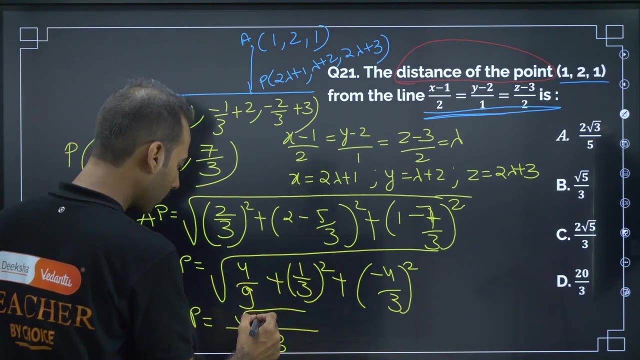 are like that: Ok minus 4 by 3 square. So a p is equal to, p is equal to. if I take l, c, m, this will get 3 under root of 3 in the numerator 4 plus 1 minus 4 square becomes plus 4 square plus. 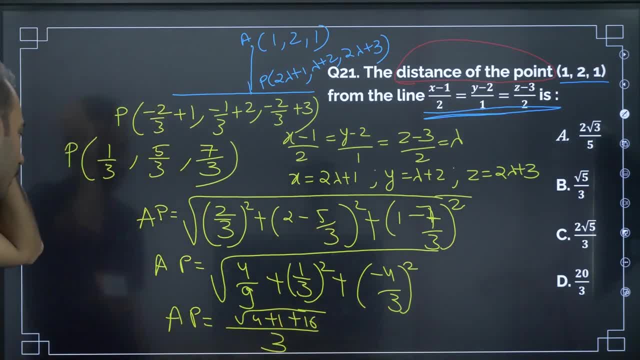 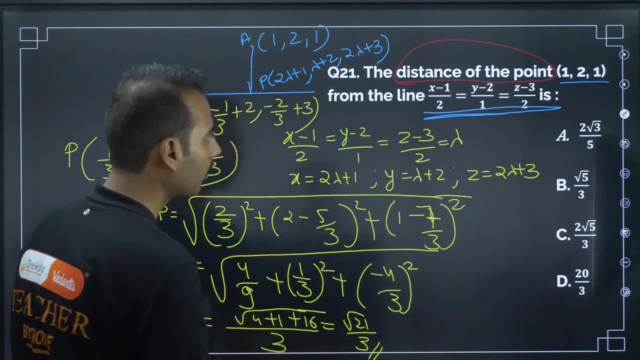 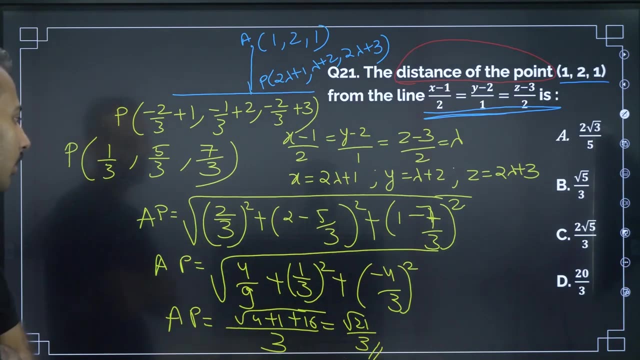 16. So 4 plus 16 plus 5, root 21, root 21 by 3. is there any such option? root 21: the distance of the point from the line, root 21 by 3.. I hope all the calculation, everything, is correct. 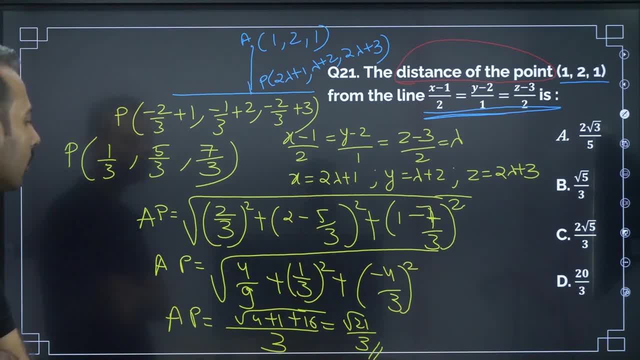 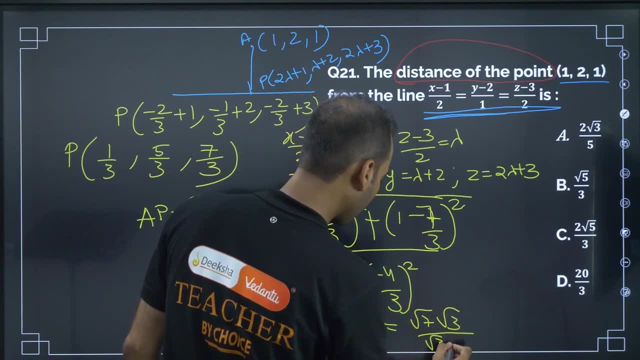 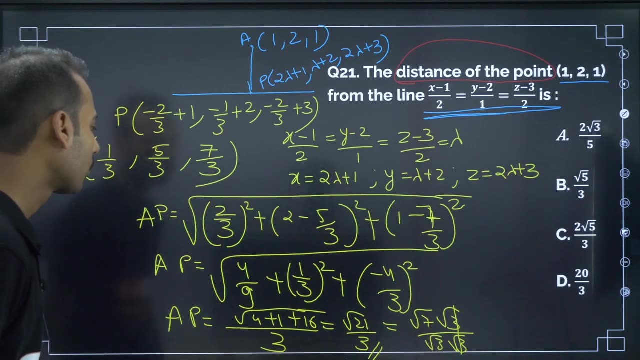 there is no mathematical error: 16 plus point For this 21. we can read this as root 7, root 3 and root 3. 3. So root seven by three. is there any such option lose 1 by 3 is also not there. 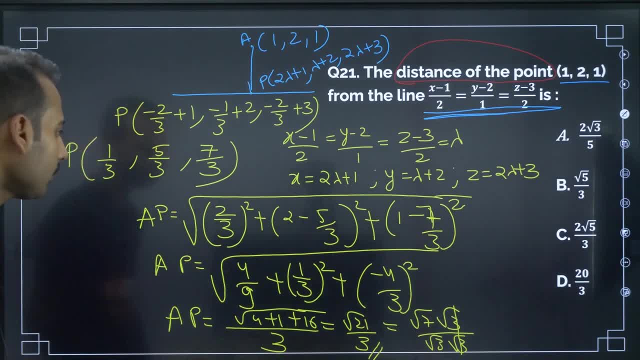 So roots 7 by 3. there is no such option like this, So let me go through this problem and I will give you answer in next. I think there is some mathematical letter or option might be wrong. I will clarify if anybody wants. I am sorry, trabalalee Посacked. 0.00552277. identification Z, manufactures mode. 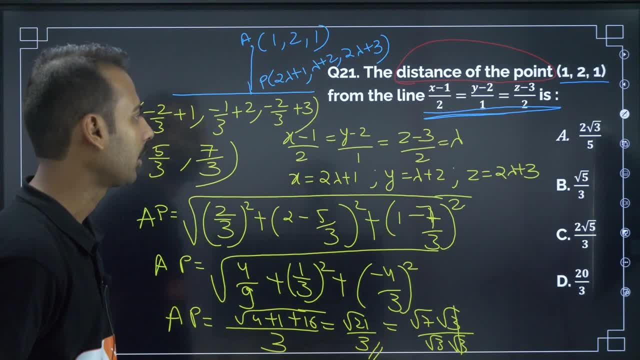 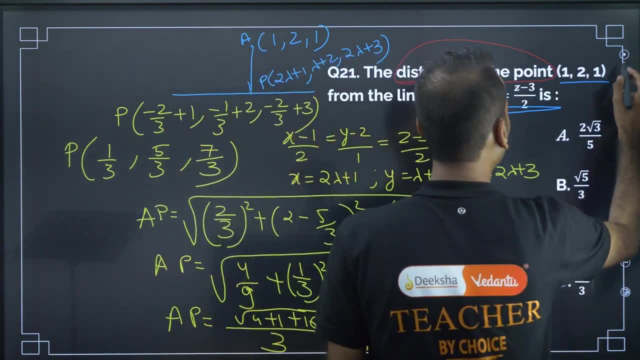 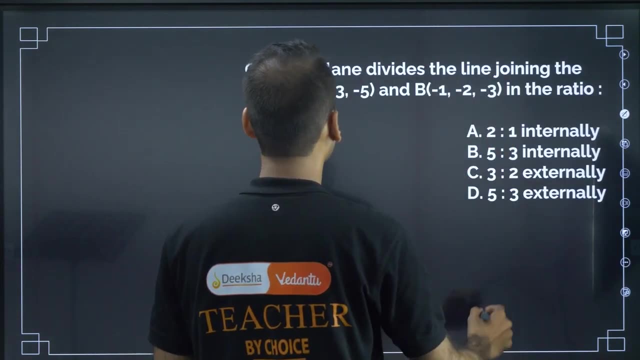 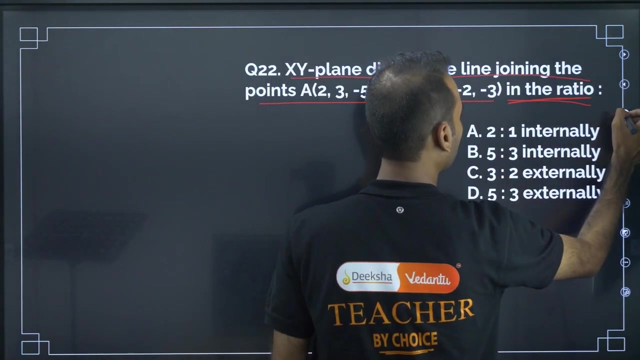 answer. just add one comment in comment also i will respond and also, and also in next video if it is possible, i will make. moving on to next question: the x- y plane divides the line joining. so what is the question in the ratio? in the ratio, x- y plane divides line joining the points in the ratio, what is the question? 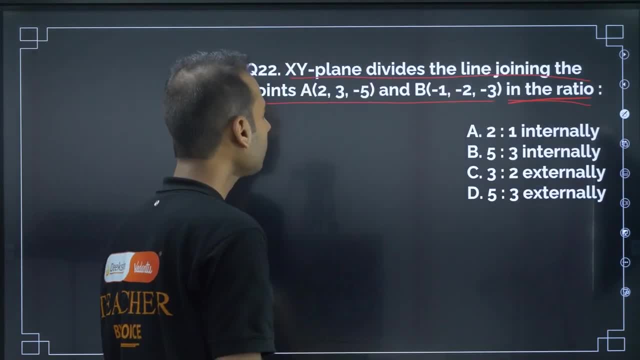 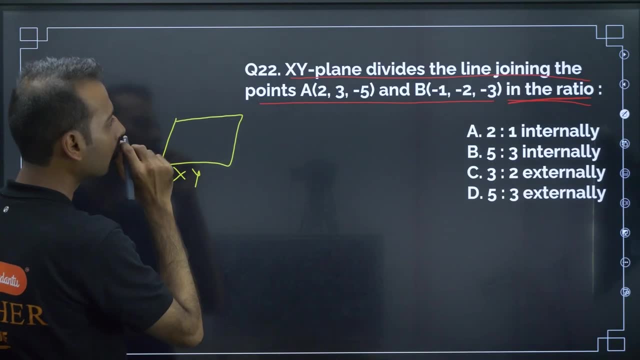 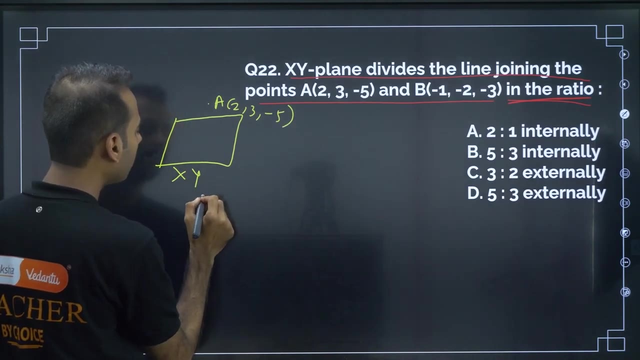 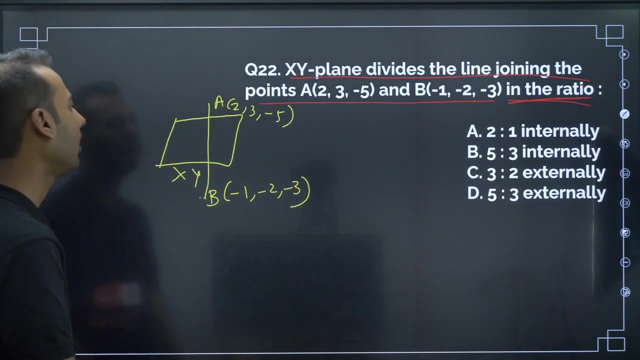 x y plane. there is one plane x y plane divides the line joining the points a, 2, 3 minus 5 b. b is one point minus 1 minus 2 in the ratio. there is one point x y plane divides the line joining the points 2, 3 minus 5 b in the ratio. 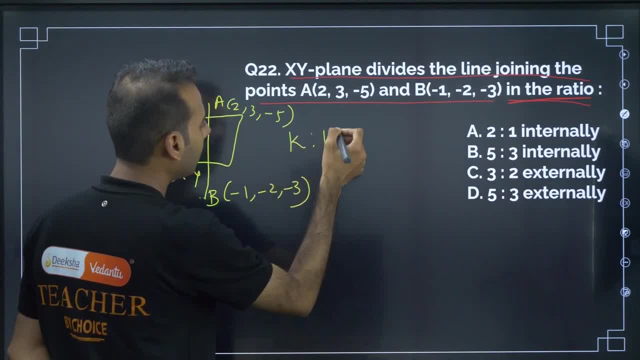 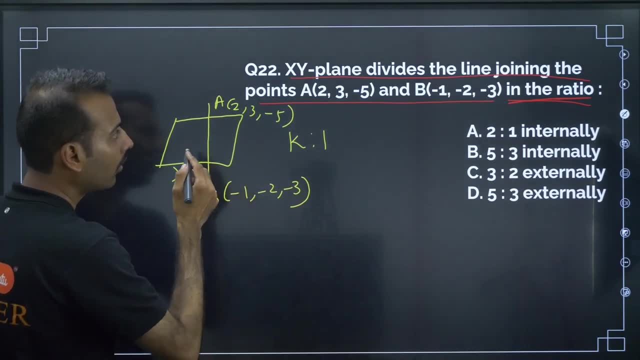 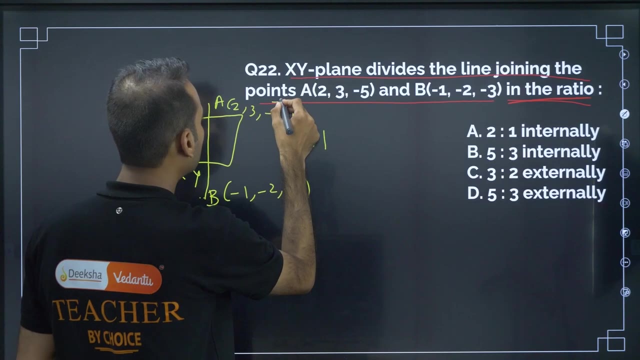 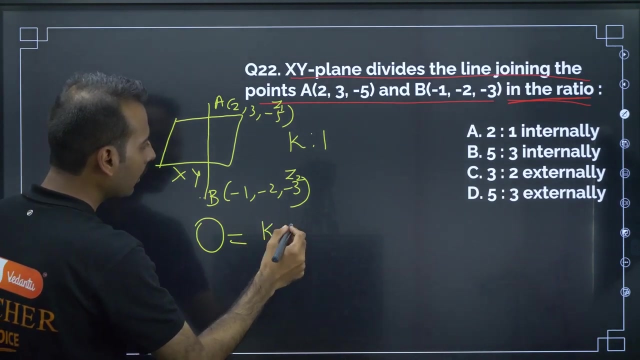 let me assume that point. it is been divided in: k is to 1 ratio. now we already know section formula, section formula x. y plane means z coordinate is 0, z coordinate. if i take z coordinate and z 1, if i mark this as z 2, x 1, y 1, z 1, x, 2, y, 2, z 2, so k, z 2 plus. 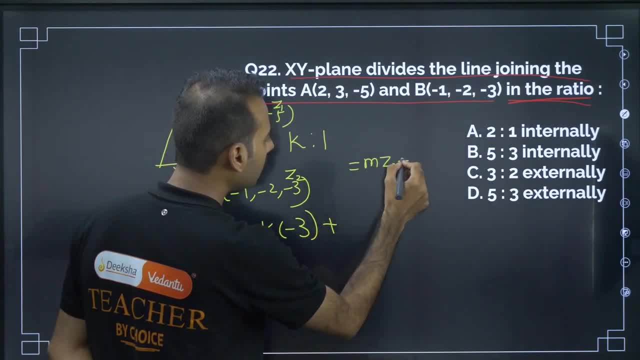 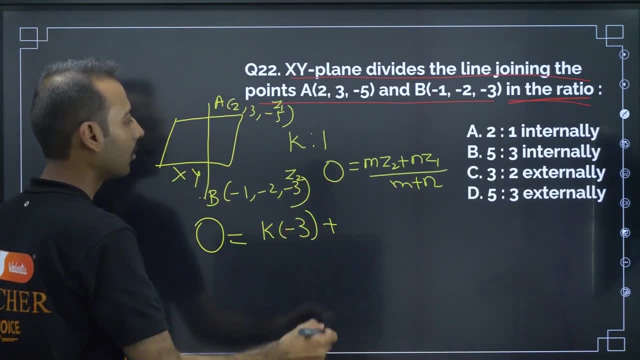 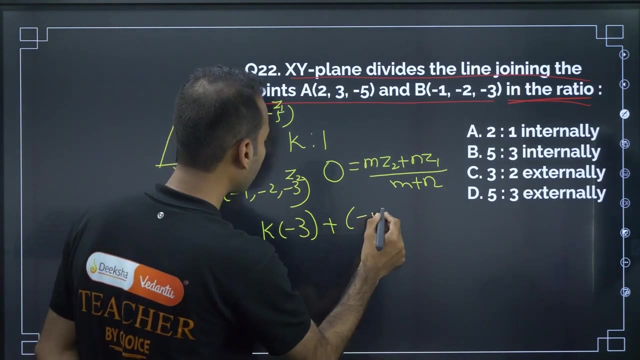 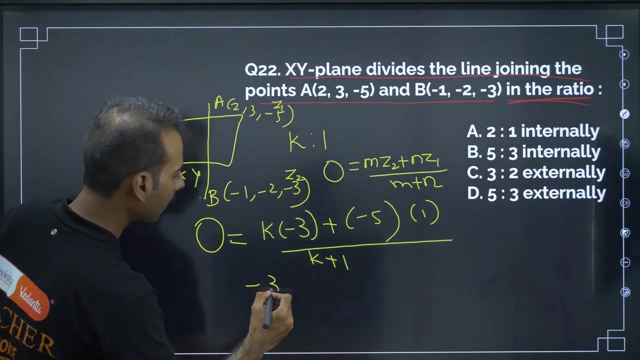 m z 2 plus n z 1 by m plus n. so this is equal to this is 0, only z coordinate. i have considered n, n is z, 1 is minus 5, n, e is 1, so m plus n means k plus 1, k plus 1, if i transpose negative. 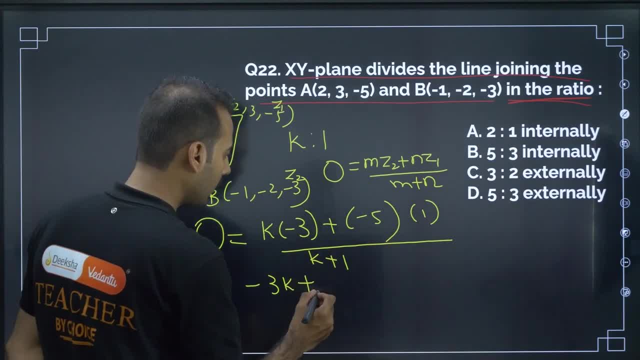 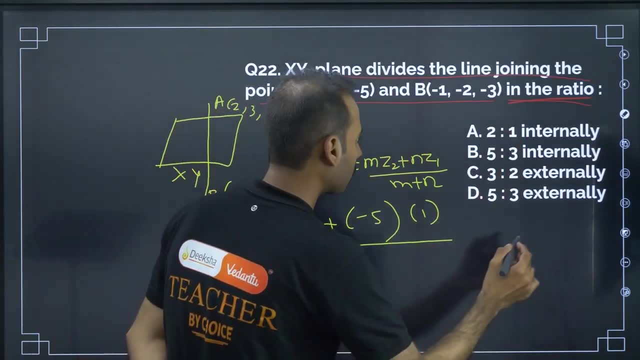 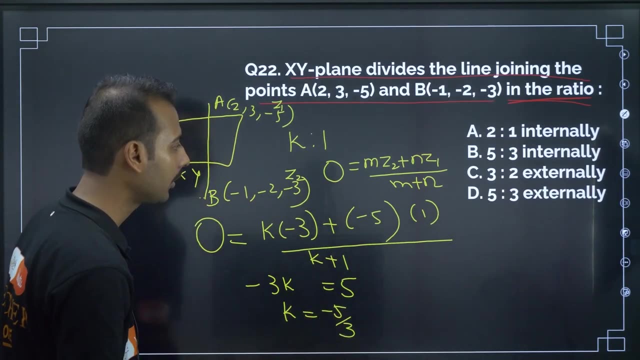 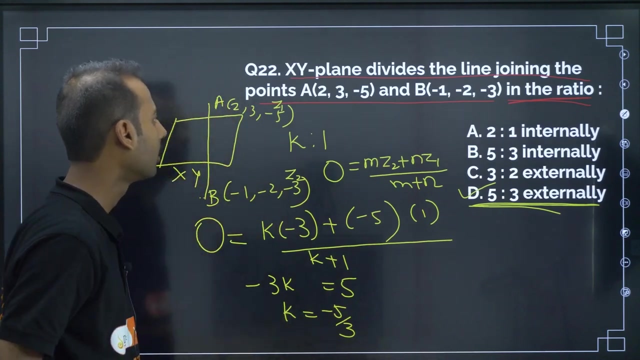 3 k negative. 3 k is equal to, is equal to 5 if i, if i- i am just simplifying that equation nothing creative. so k is equal to k is equal to minus 5 by 3 k. 5 by 3. that means 5 is to 3 externally, externally. so 5 is 2, 3 externally. is the answer just. 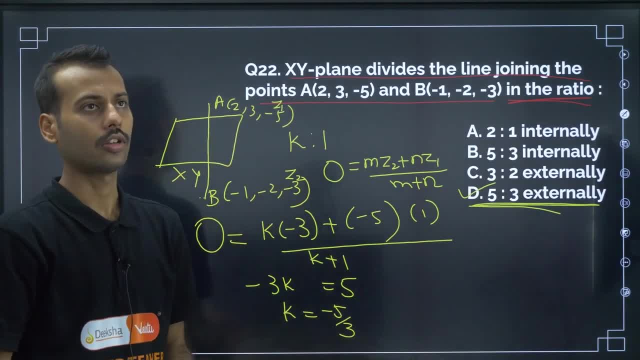 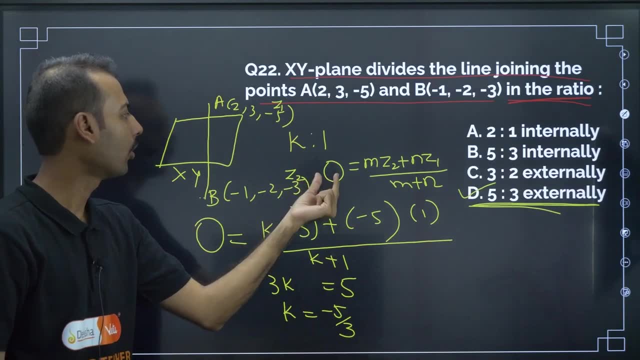 we just have to use section formula. what is section formula for straight lines? we have already studied in 10 standard same, only extended version. i am assuming k is to 1 and then we already know that z coordinate is 1, only reach percent k is equal to zero. so 10 x 3 concom标. 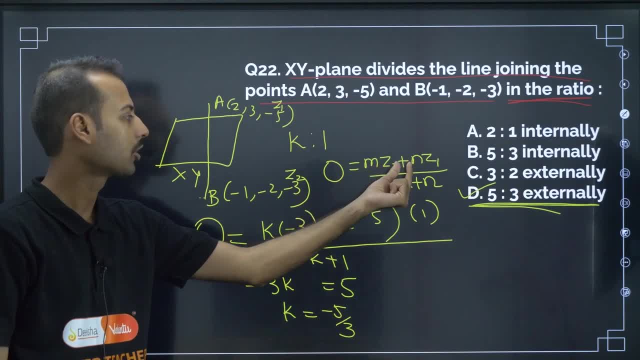 zone only being returned to. c is equal to 0, k is just to x, because if we exchange both, n is 0, in for x, y plane, z coordinate is 0.. So m x 2 plus n, m, z 2 plus n, z 1 by m plus n. 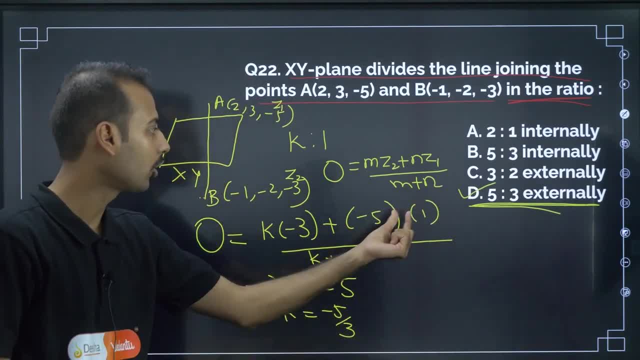 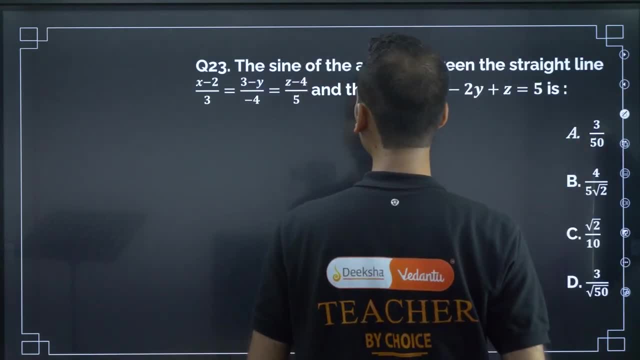 k a plus 1. all that I have simplified. and that, Since it is negative, negative means what externally? if it is positive, then it is internally. Going on to next question, the sign of angle between the plane is: So what are they asking? 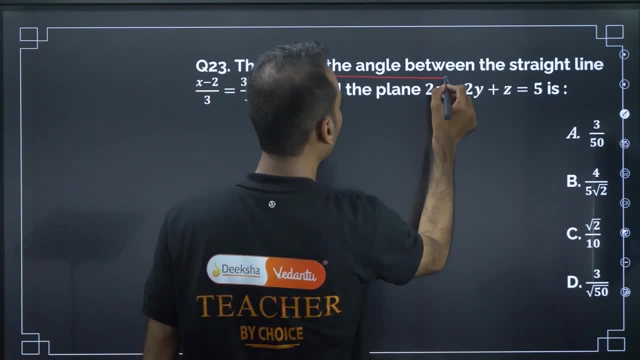 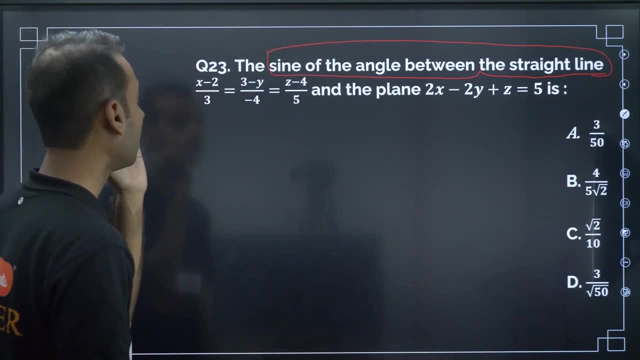 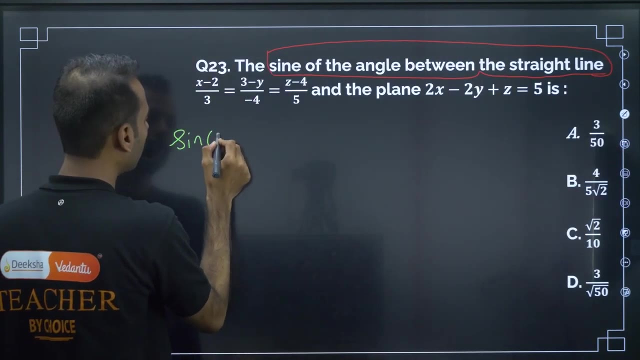 the sign of angle between. they are asking sign of angle between the straight line. they are asking sign of angle between the straight line x minus 2 and the plane is. So what is the formula? Sign of angle is sin theta is equal to what Sign of angle between a? 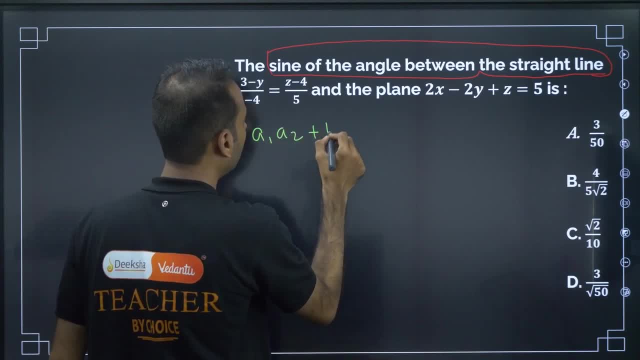 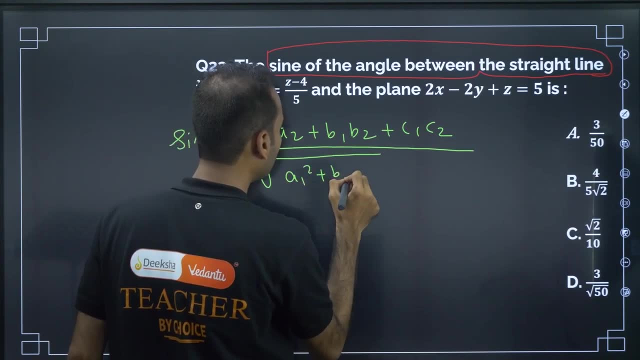 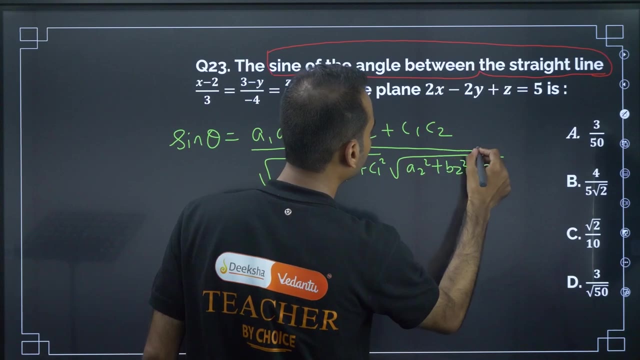 1, a 2, b 1, b 2, c 1, c 2. by root of a 1 square. b 1 square. c 1 square. root of a 2, b 2, b 1 square. b 2 square, c 2 square. Now, what are they asking? They are asking to 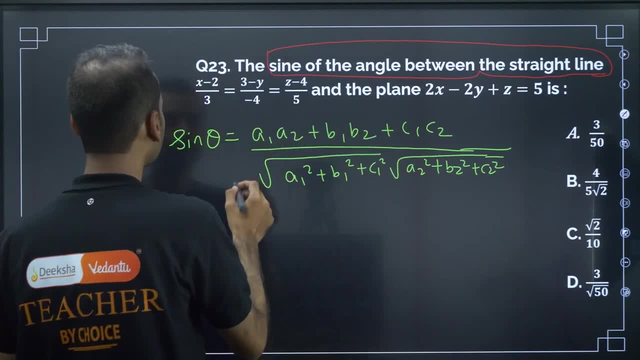 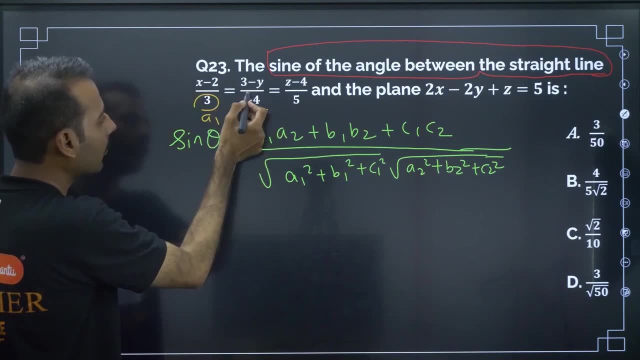 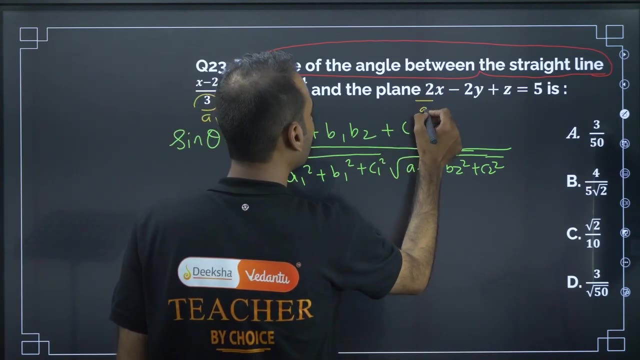 find sign of angle. Now from this, this is a 1,. this is, if I make this plus, the reason why I am making this plus. if I take minus common, this becomes b 1, c 1 and a 2, a 2,. 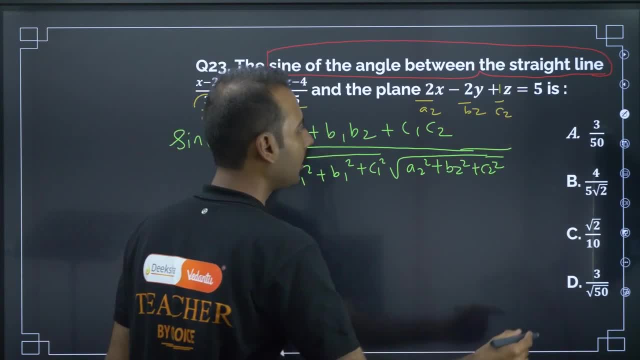 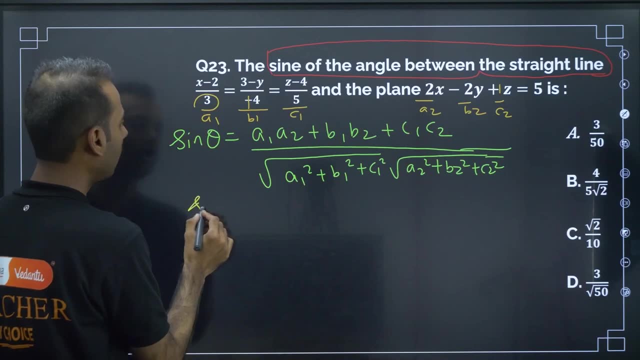 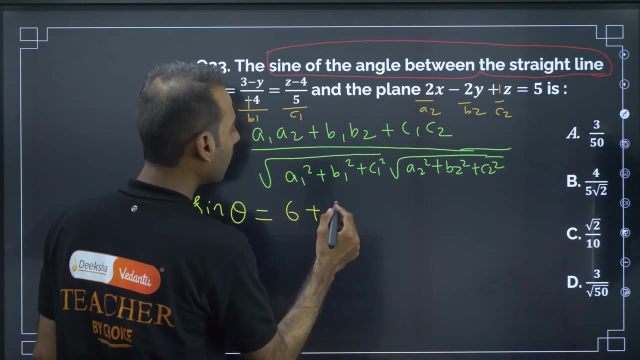 b 2 and this 1 is c 2.. So sin theta, sin theta angle is sin of angle. sin theta a 1, a 2, a 1, a 2 is 3 to the power 6, b 1, b 2 is 4 minus. 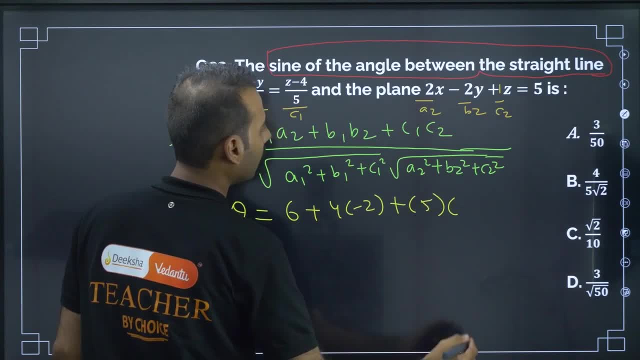 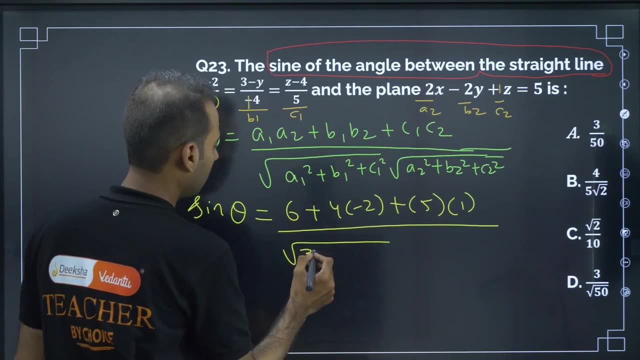 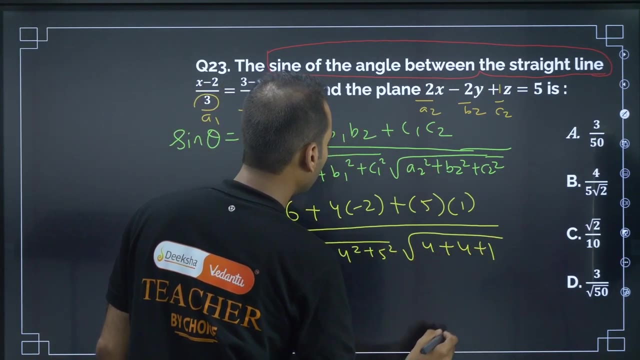 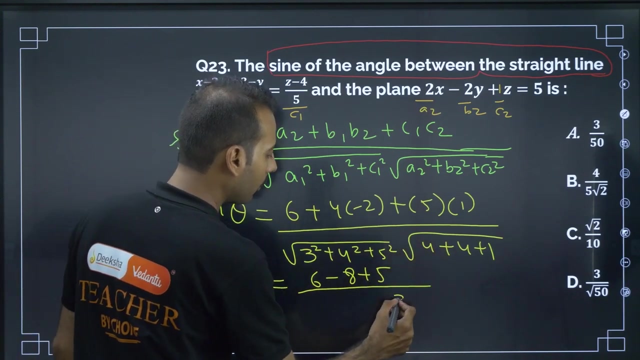 2 plus pi, pi c 2, c 2 is 1 by under root of 3 square 4 square 5 square under root of 4, 4, 1.. So 6 minus 8 plus 5 by root of 4, 4, 3, this is 3, 8, 9, 3.. Now what about this? 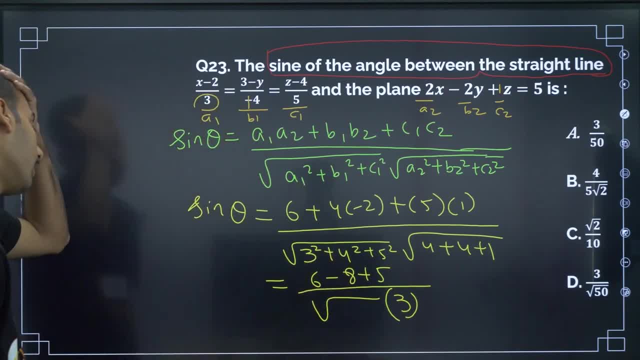 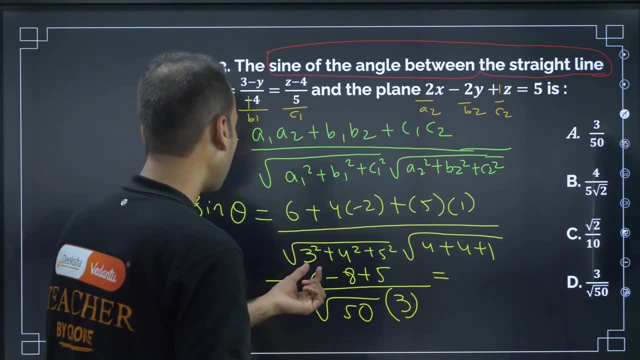 under root of 2, 25,, 25,, 25,, 50. So 6 minus 8 is minus 2,, 6 plus 5 is 11, 11 minus 8 is 3, 3 by 3 by. 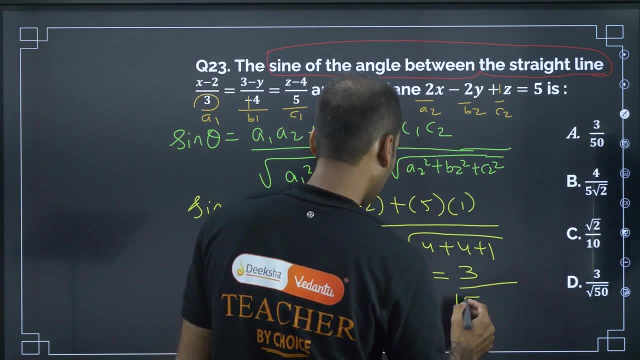 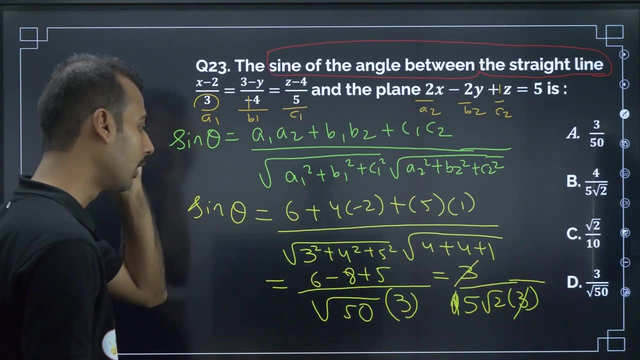 5 root 2. pi 3 is a 15.. Let me write 5 root 2 and 3 here, as it is 3 and 3. if I cancel, I am left with 1 by 5 root 2. there is no such readymade option. 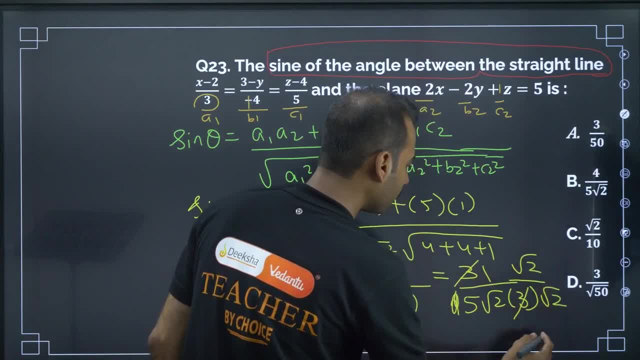 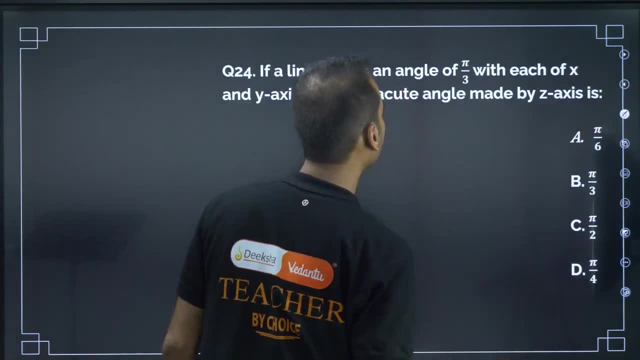 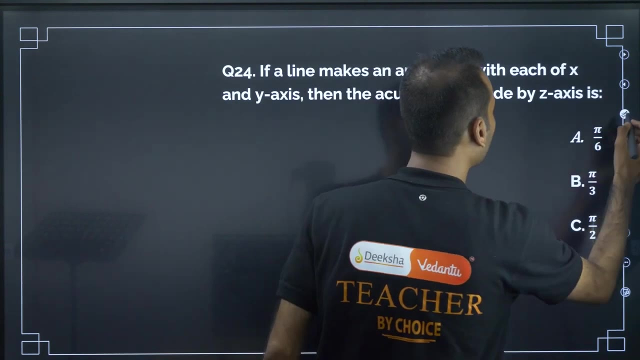 So let me multiply with root 2 and let me multiply with root 2. this becomes root 2 by 5. 2 is a 10.. Is there any such option? C is the answer. Moving on to next question, If a line makes angle pi by 3 with each of x, y, then acute angle made by z axis is very 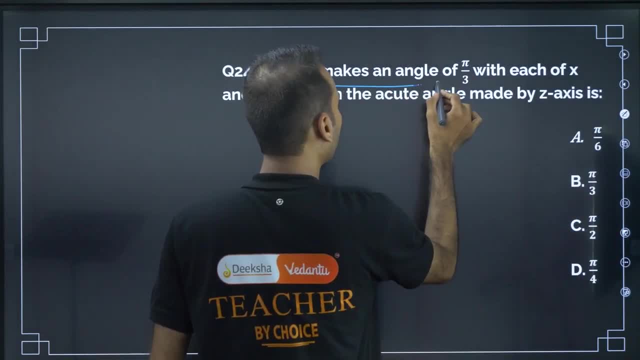 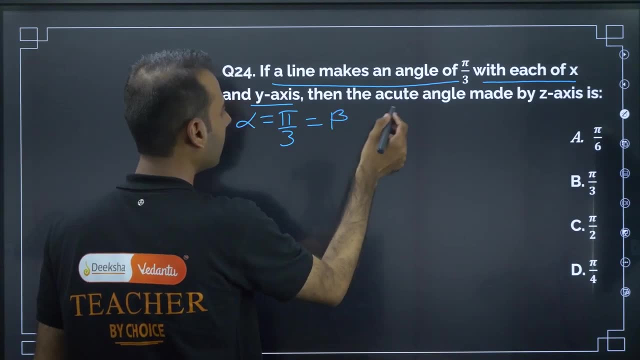 easy question. So if you go through the question, if a line makes angle pi by 3 with each of x and y axis, So alpha is equal to beta is equal to pi by 3.. The angle made by z axis: 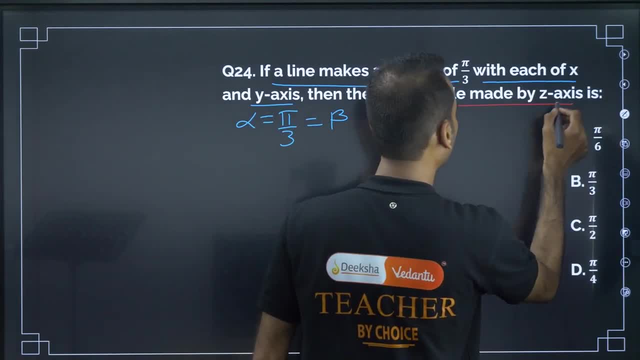 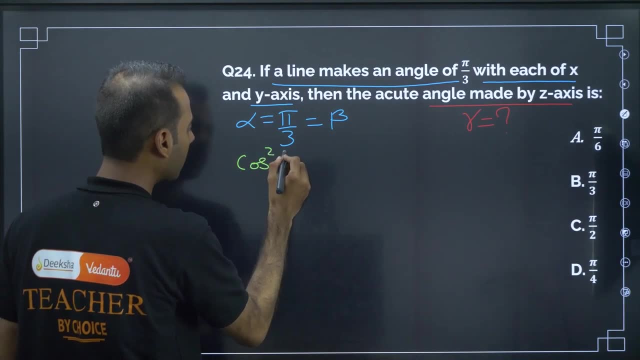 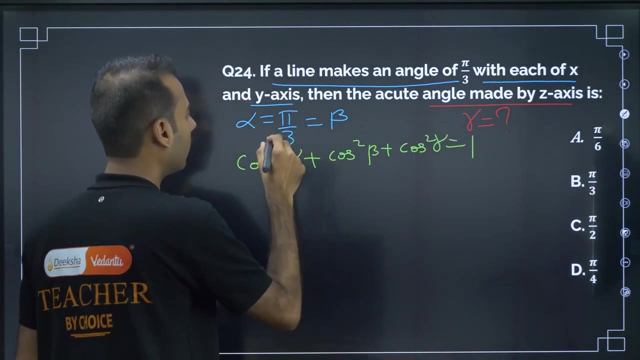 angle made by z axis. what are they asking? they are asking gamma. now one relation. we are already aware. what is that relation? try to recall this relation, very easy, very famous: cos square alpha plus cos square beta plus cos square gamma. cos square gamma is equal to 1. now cos pi by 3. you. 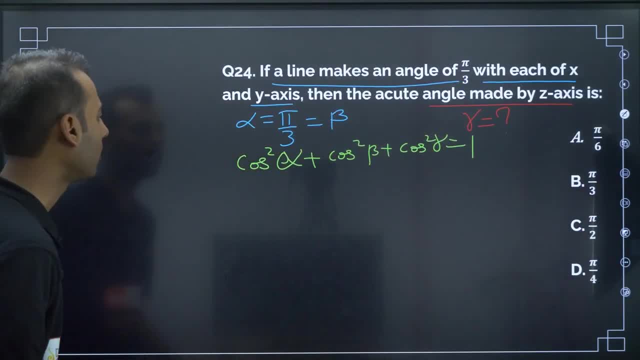 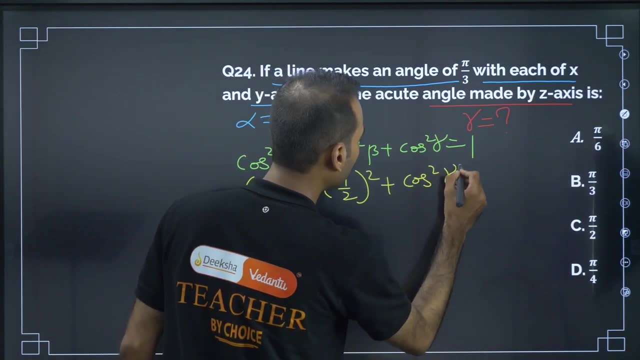 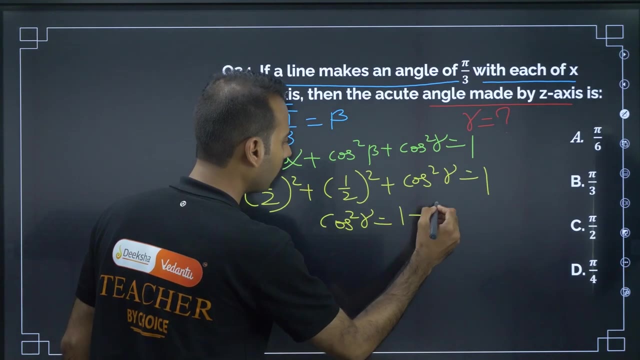 place all these values. cos pi by 3 is 1 by 2. 1 by 2 square plus 1 by 2 square plus cos square gamma is equal to 1, so 1 by 2 is 1 by 4. 1 by 4 is cos square gamma. if you transpose all this to other. 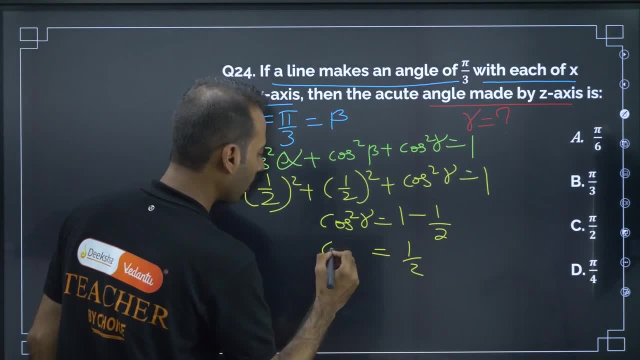 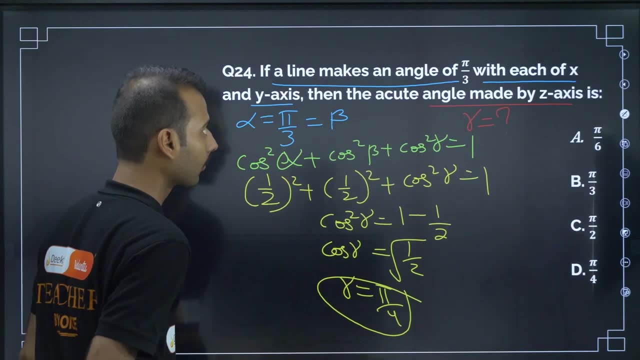 you will get 1 minus 1 by 2, which is equal to 1 by 2. cos cos, gamma is equal to under root. so gamma is equal to pi by 4. d is the answer. moving on to next question, the distance of the point from the. 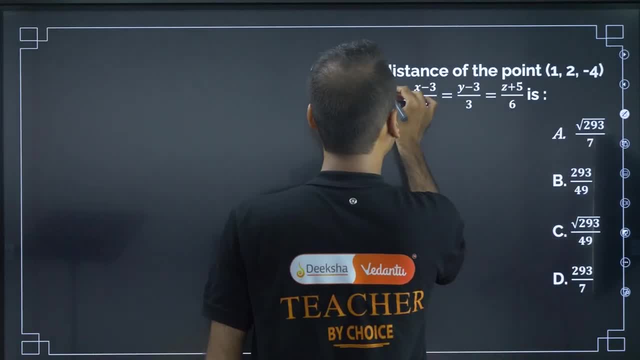 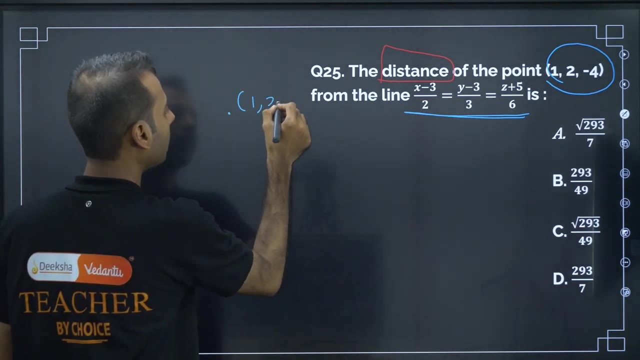 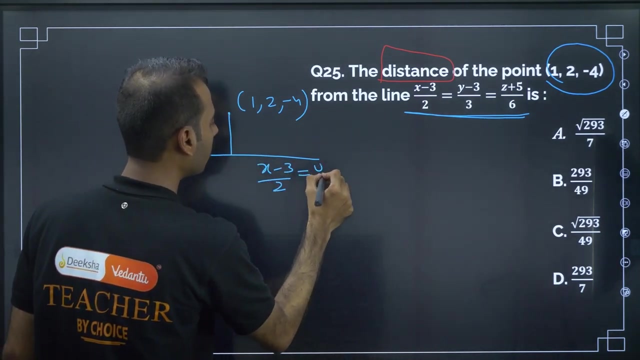 line. so what are they asking? they are asking to find distance. they are asking to find distance of point, of what of point? from line. so they are talking about distance of point. what is that? point 1, 2 minus 4 from line line is x minus 3 by 2 equal to y minus 3 by 2 is equal to. 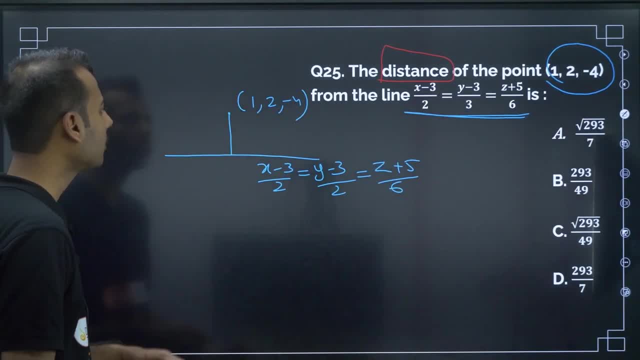 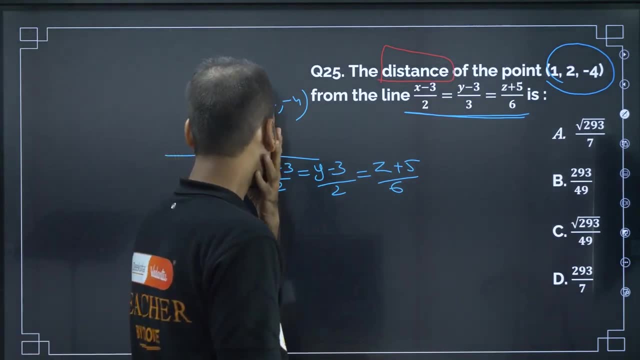 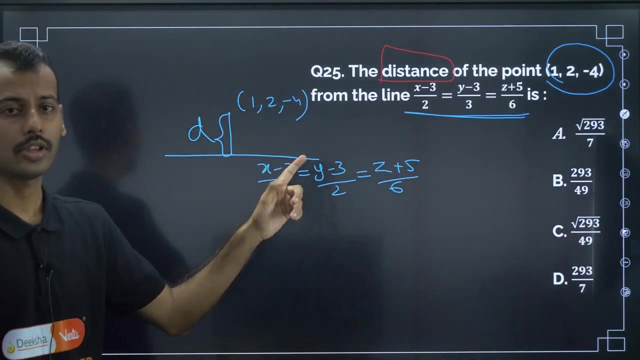 z plus 5 by 6 distance they are asking to find. this distance of this point from this line is: what is the distance of this point from this line? so for that, what i will do, i will go for this. see this: you observe this question multiple times in this session, only this. based on this concept, we are getting multiple. 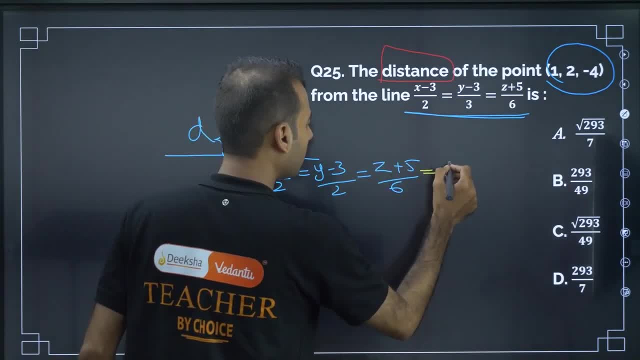 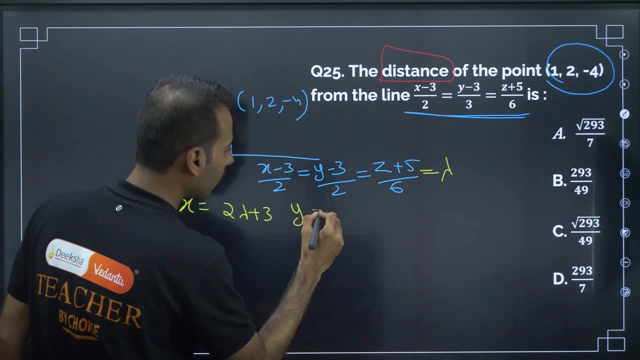 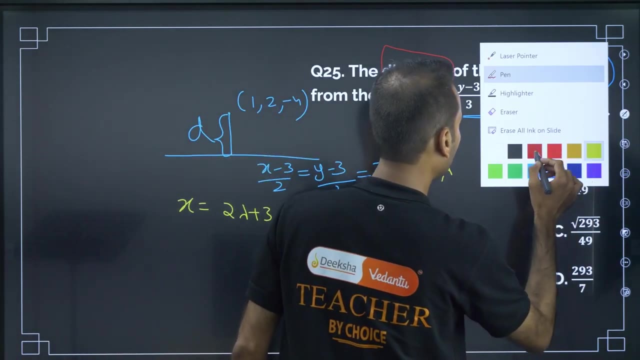 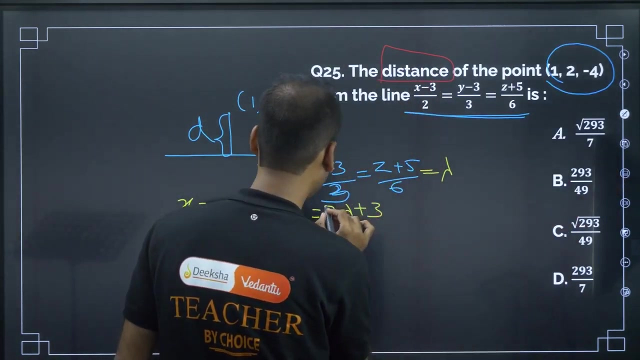 times means very important concept, so you should practice this at any cost. now this i will equate you to lambda. so x is equal to 2 lambda plus 3. y is equal to 2 lambda plus 3. this is 3- some mistake i have done. this is 3, so this is 3 lambda plus 3. 3 lambda plus 3, z plus 5 by 6 is z is equal to 6. 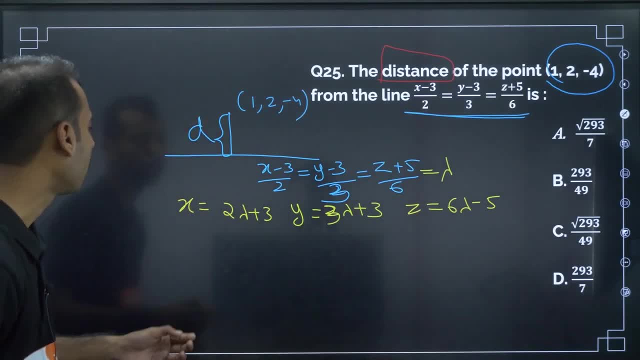 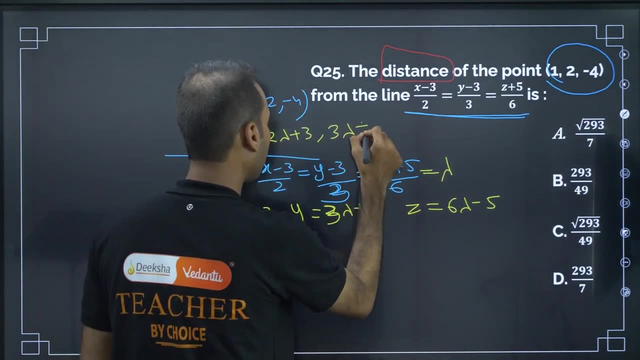 lambda minus 5, z is equal to 6 lambda minus 5. now this point. if i mark some arbitrary point, say p, 2 lambda plus 3, 3 lambda plus 3 and 6 lambda minus 5. now if i talk about direction, ratios, direction, 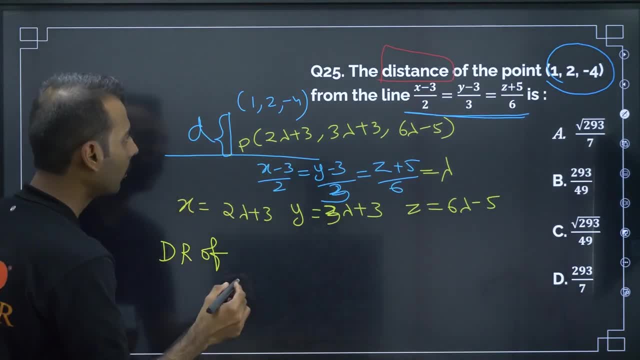 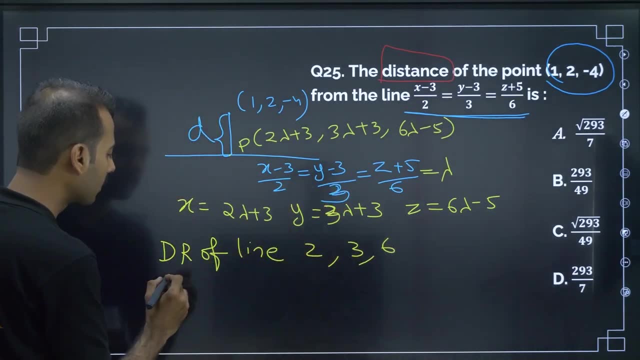 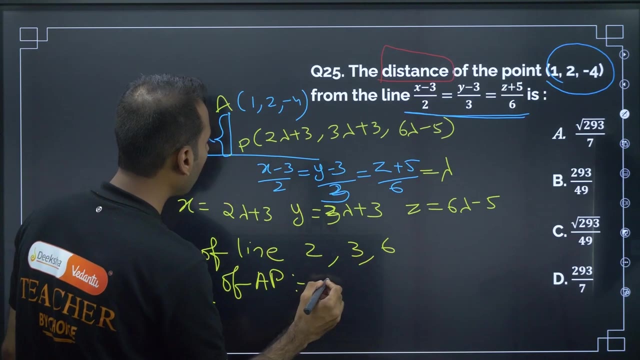 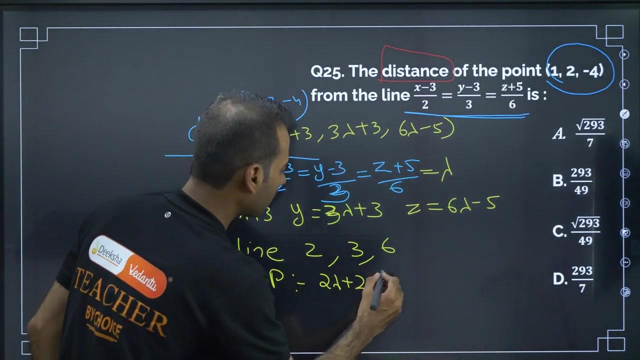 ratios of direction. ratios of line. first let me write line line is 2, 3, 6. direction ratios of line is now direction ratio of. if i mark this as a direction ratio of a p, direction ratio of a p is 2 lambda plus 2. how to find direction ratios i already explained. 3 minus 1 is 2, 3 lambda plus 1. next, 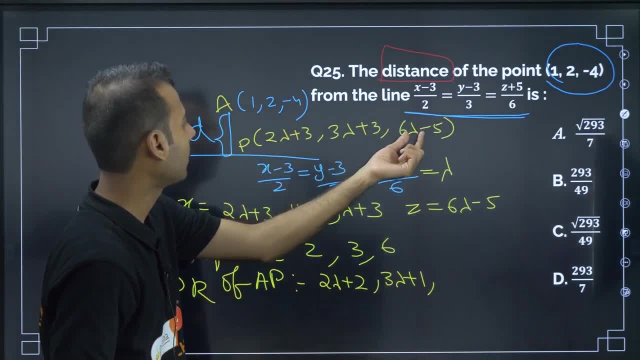 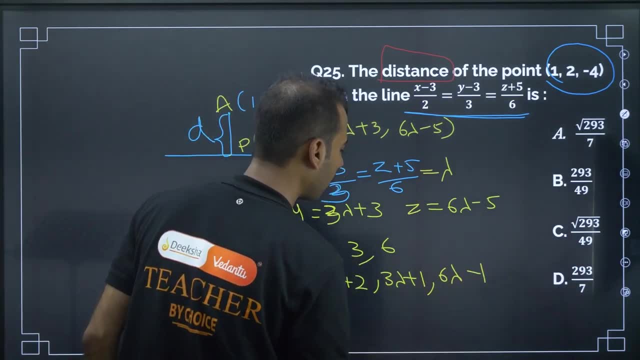 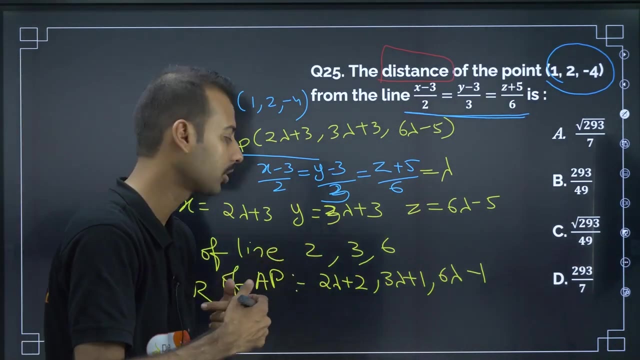 3 lambda plus 1, next 6 lambda minus 5 minus minus. so this becomes 6 lambda minus 5 plus 4 is minus 1, so 6 lambda minus 1. again go for same concept. this line and this are perpendicular, so you multiply this and equate it to 0: a1, a2 plus b1, b2 plus c1, c2 is equal to 0. 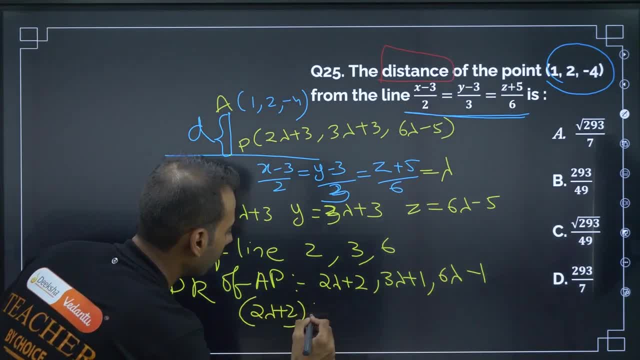 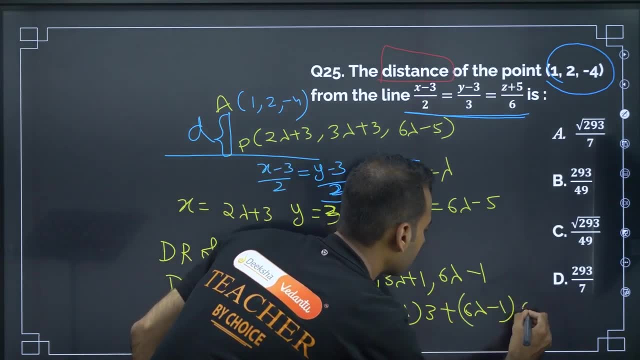 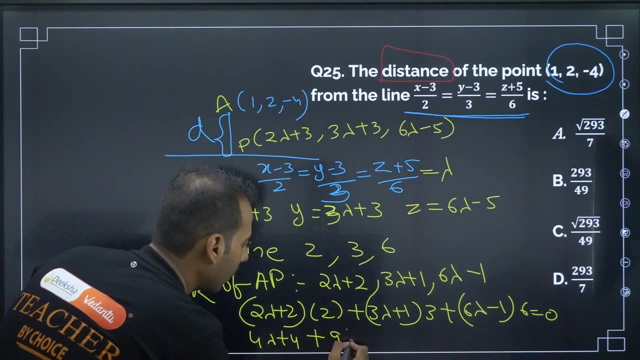 so 2 lambda plus 2, 2 lambda plus 2. you multiply with this: 3 lambda plus 1, 3 plus 6 lambda minus 1, 6 is equal to 0. now, if i multiply this: 4 lambda plus 4, 3 lambda, 9 lambda plus 3. 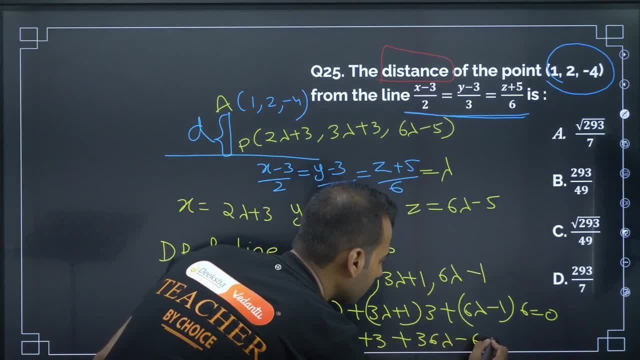 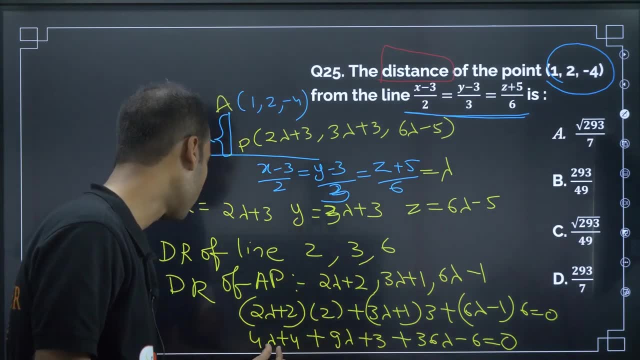 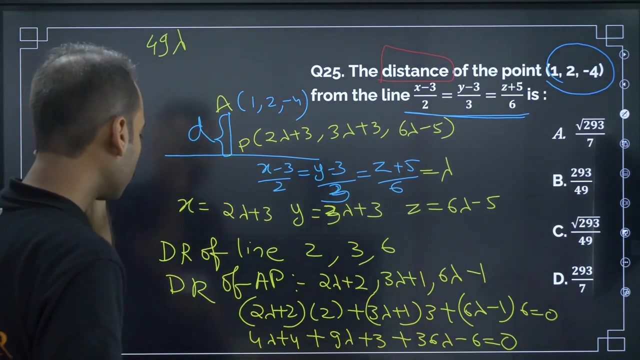 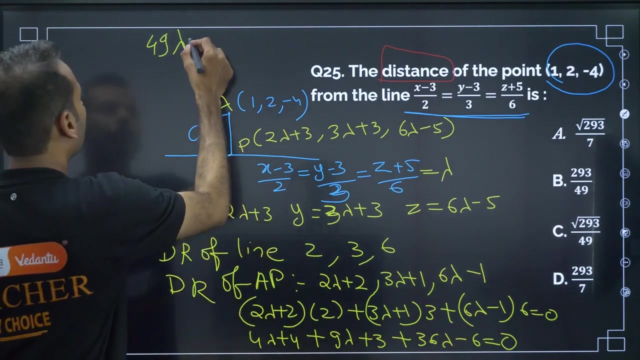 plus 36 lambda minus 6 is equal to 0. now 4 lambda, 9 lambda, 49 lambda- i think it should be 49 lambda. see here: 49 lambda, 49 lambda. and then 4, 4, 3, 4, 3, 4, 3, 7, 7 minus 6 is 7 minus 6 is 1, equal to 0. 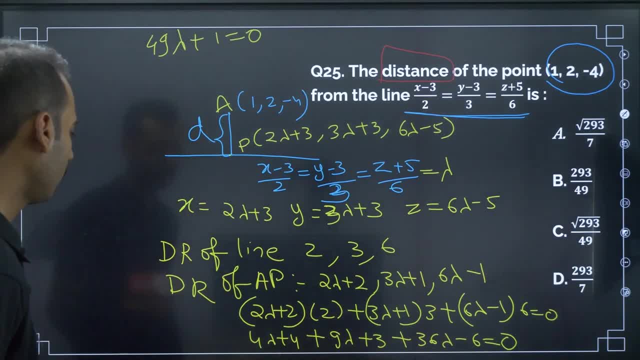 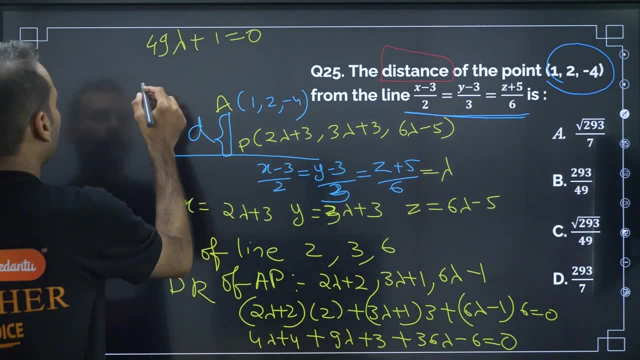 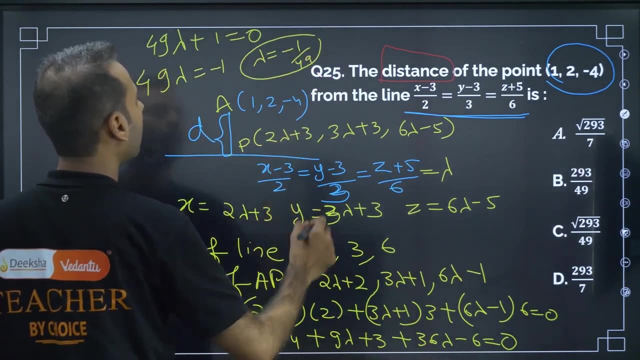 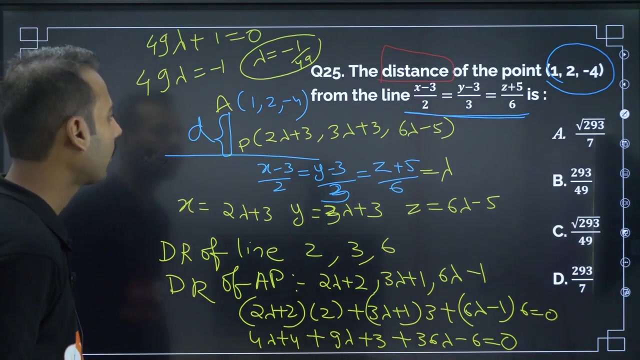 one minute. let me check whether everything is going correct or not. so 49 lambda, 49 lambda is equal to minus 1, which implies lambda is equal to minus 1 by 49. lambda is equal to minus 1 by 49. now you place this lambda in. you place this lambda in p and then 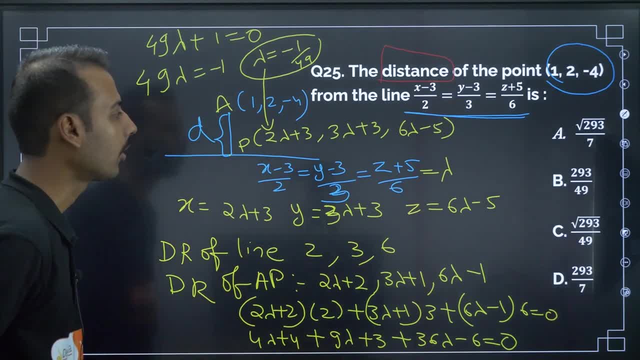 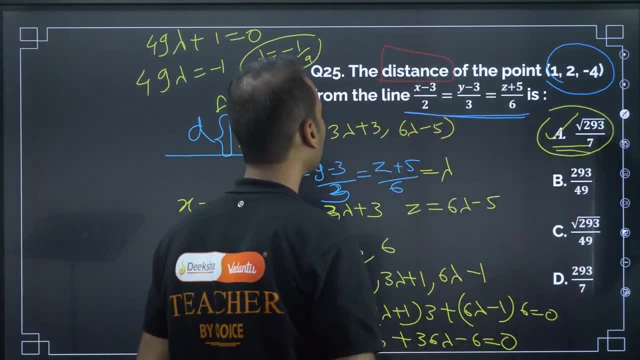 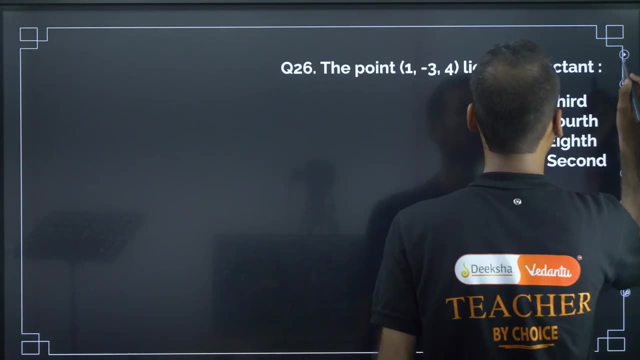 you will get p and then use distance formula. finally you will get the answer. i think the answer should be root of 293 by 7, just substitution part. i am leaving it to you. if you want explanation for that also, you ask me in comment section. i will explain that also next. moving on to next. 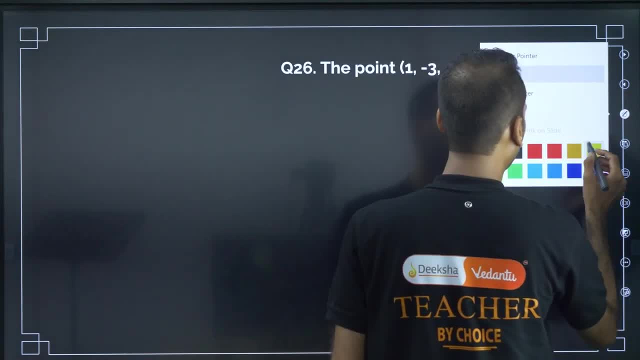 question. the point 1 minus 3 is equal to 0, so 0 is equal to 0 and 0 is equal to 0 and 0 is equal to 4. this is direct question. for direct question, we can't do anything. the point minus 3: 1: 4. 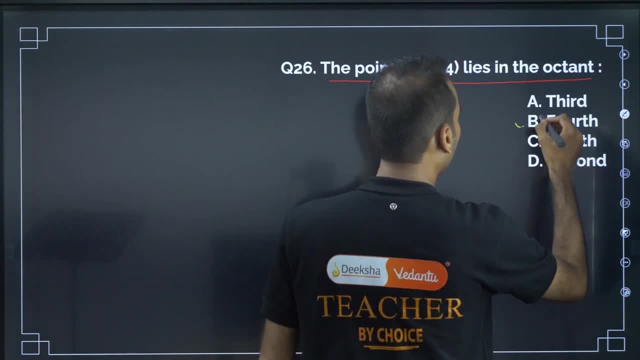 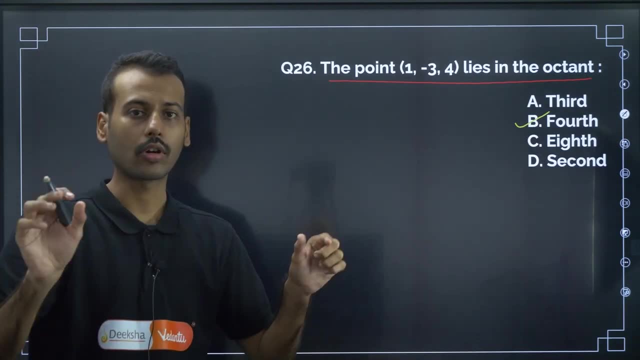 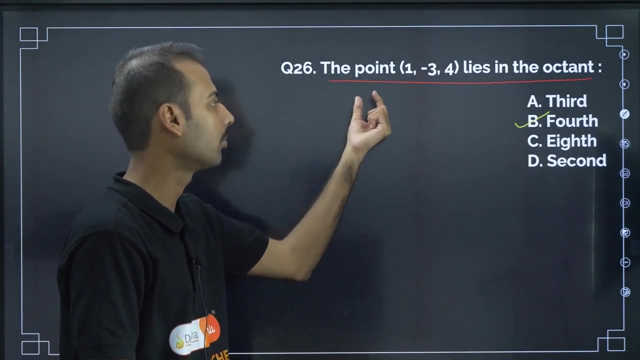 lies in which point this octant, fourth octant. so introduction to the dimensional geometry. first, p, u, c, those eight quadrants, all that that you have to memorize because, as per the customs of maths and the traditions of maths, we are having some plus plus, plus plus minus. 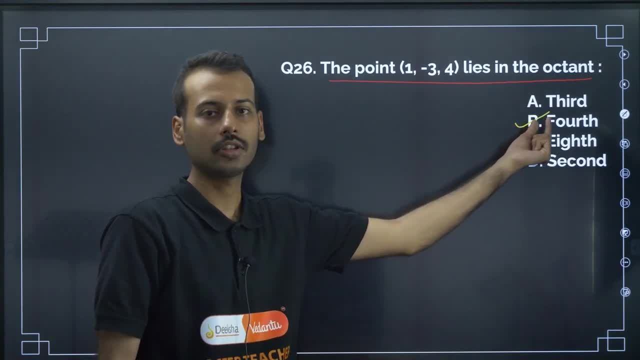 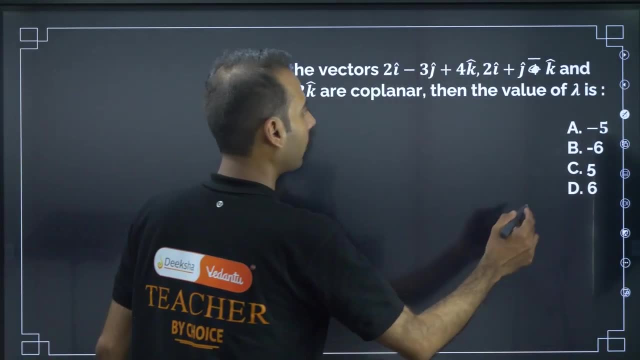 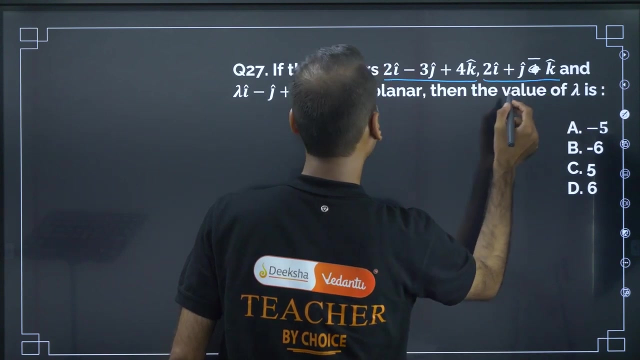 minus all those signs you have to remove. so this is fourth explanation we can't give. it is like that. only next. moving on to next question, if the vector is two minus three- some information they have given- they are asking to find the value of two minus three, four, three. 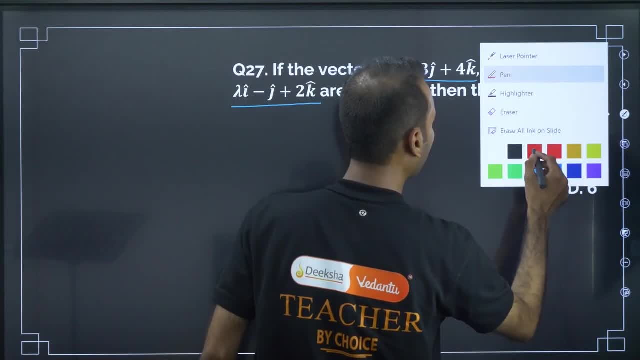 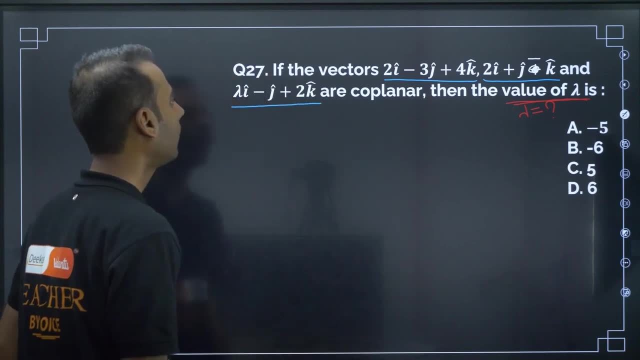 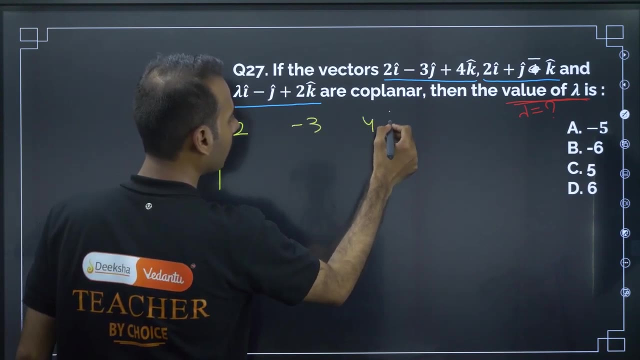 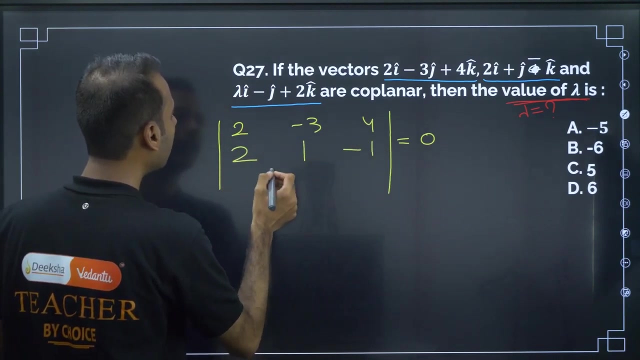 and lambda r coplanar, then the value of lambda is. then the value of lambda is: what is the value of lambda? they are asking to find this- if the vector is 2 minus 3, 4. so just take the coefficients of 2 minus vectors and equate that to 0. this is the condition for coplanarity: 2, 1 minus 1. lambda minus 1. 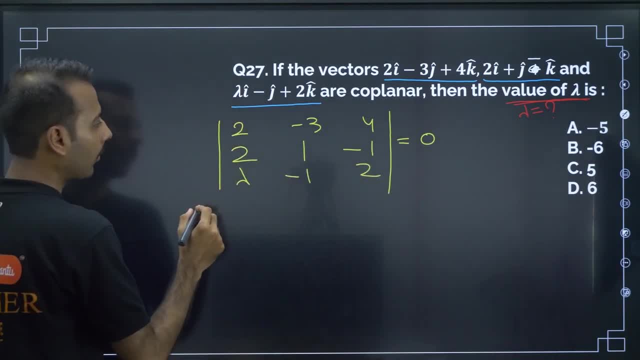 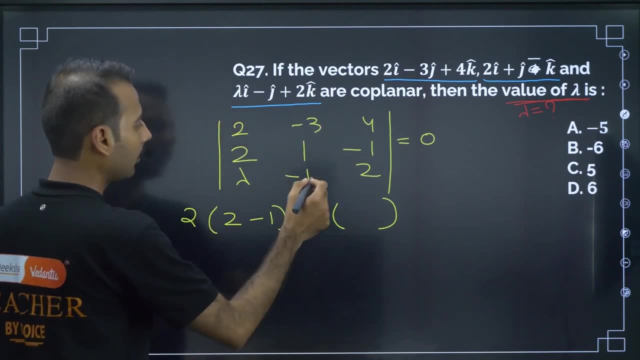 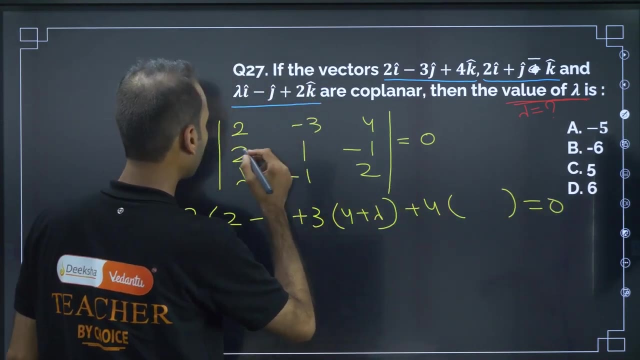 2 is equal to 0. are coplanar, then the value of lambda is so 2, 2 minus 1 plus 3 plus 3, 4 plus lambda plus 4 plus 4 is equal to 0 plus 4 minus 2 minus lambda. minus 2 minus lambda is: 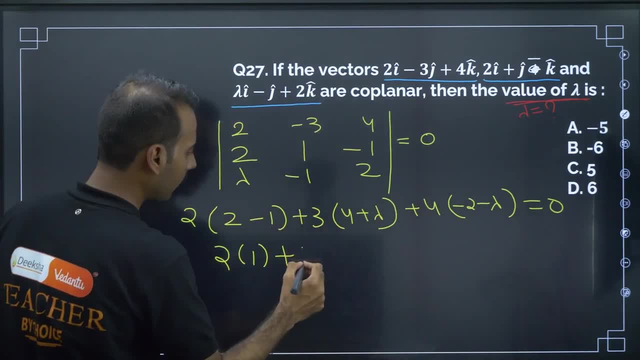 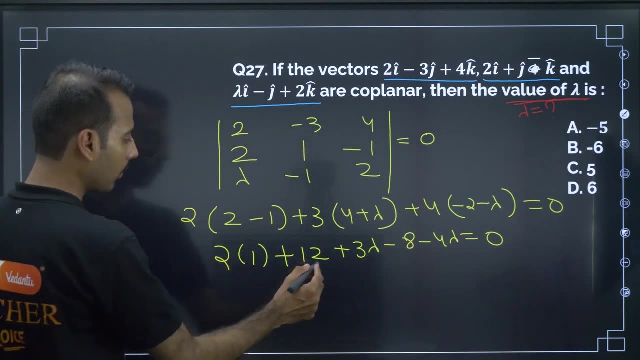 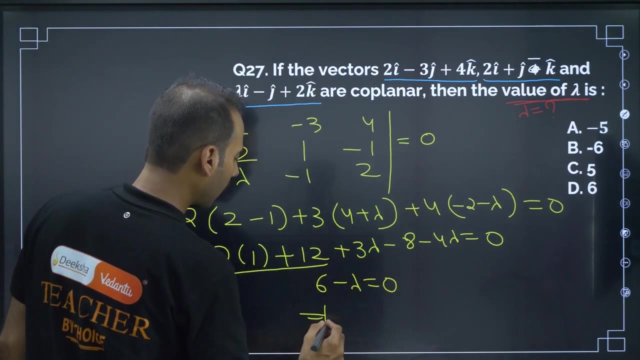 equal to 0. so if I simplify, 2, 1 plus 3, 4's are 12 plus 3. lambda minus 8 minus 4 lambda is equal to 0. next, 2 plus 14, 14 minus 8 is 6 minus lambda is equal to 0, which implies lambda is. 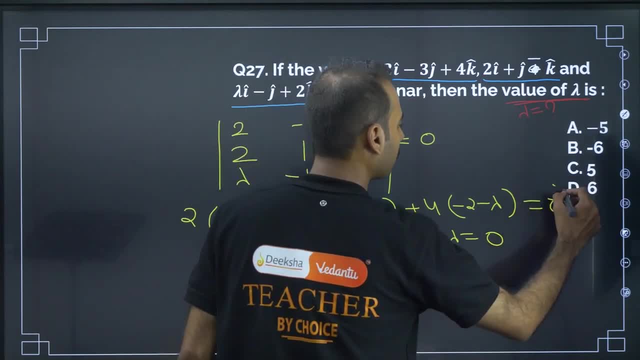 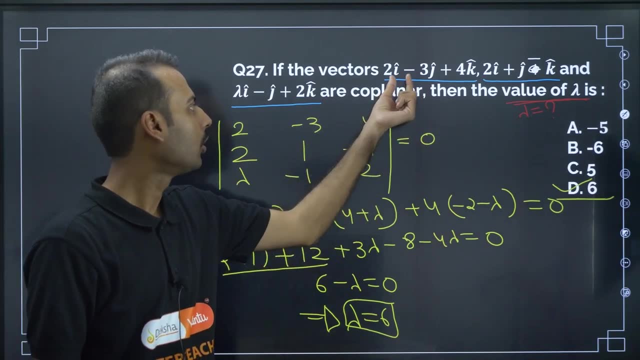 0 is equal to 6, which implies lambda is equal to 6, so d is the answer. so in this question we are supposed to use the condition for coplanarity. whenever condition for coplanarity is there. you just write the coefficient of i, j, k, and that determinant is equal to 0. you equate this. 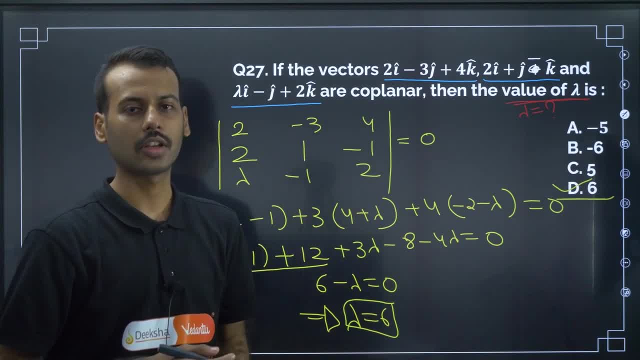 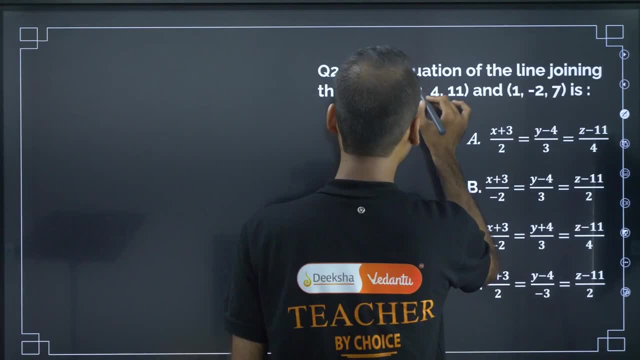 because if a, b, c are said to be coplanar, if their scalar triple product is 0. so scalar triple product means we have to solve in this way. finally, the answer is 6. what are they asking? the equation of line joining the points two points. 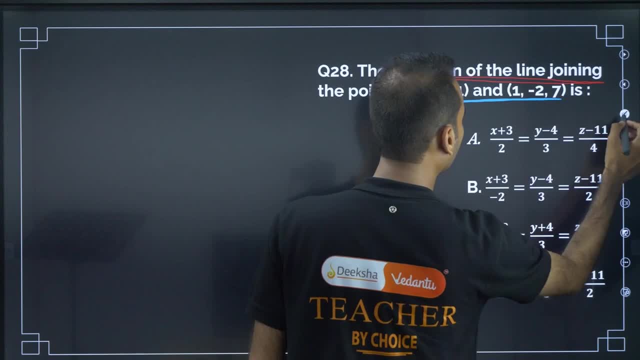 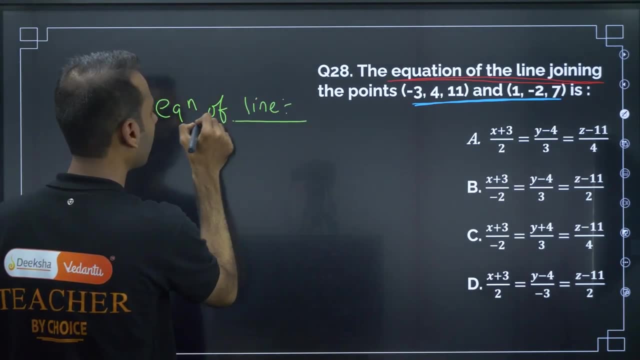 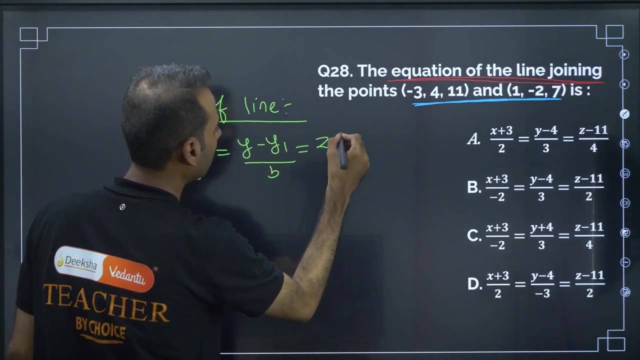 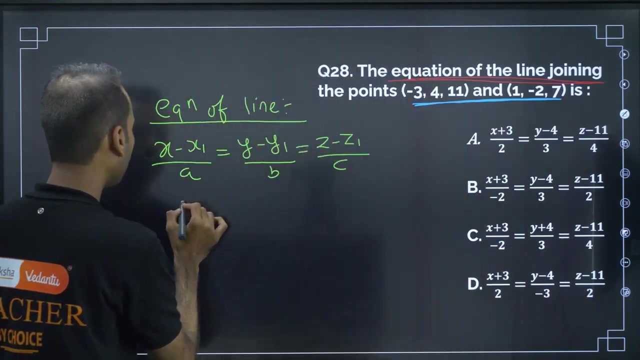 they have given the equation of line joining. try to recall the equation of line. equation of line. equation of line is: x minus x, 1 by a is equal to y minus y. 1 by b is equal to z minus z, 1 by c. equation of line joining the points. so if I find a b c from here, a b c, x, 2 minus x, 1, 1 minus. 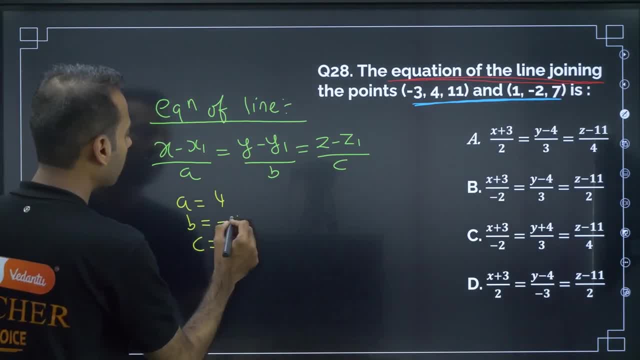 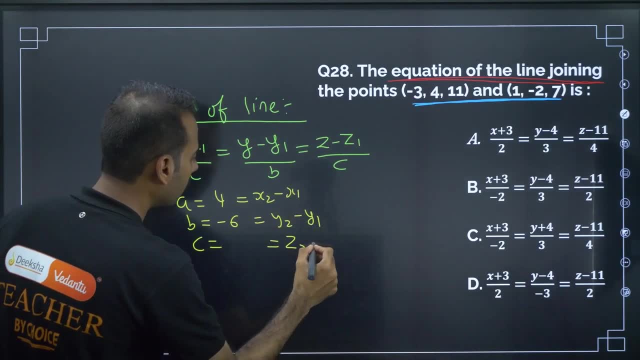 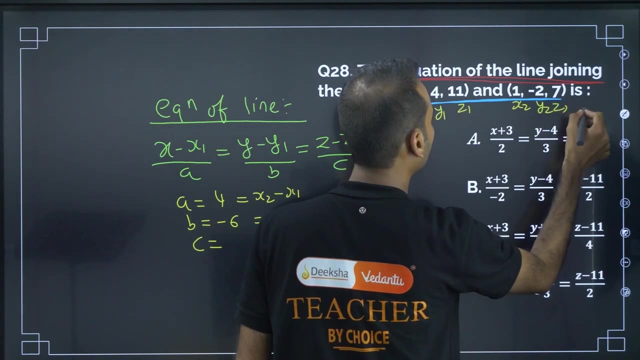 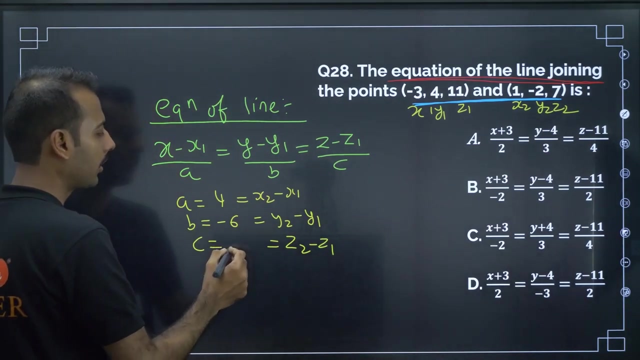 4 minus 2 minus 4 minus 6. how to find: a. this is x 2 minus x 1, y 2 minus y 1. z 2 minus z 1. this is x 1 y 1 z 1, x 2 y 2, z 2, a, b, c. so z 2 minus z 1 is 7 minus 11. 7 minus 11 is. 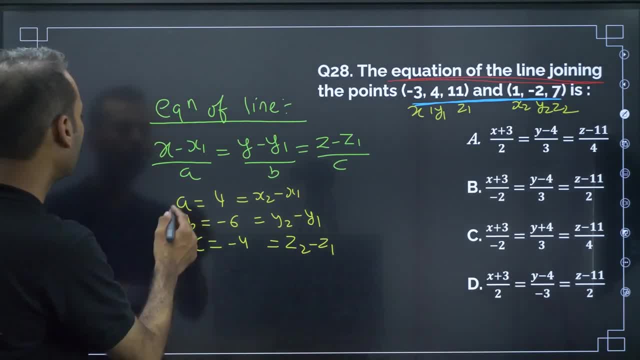 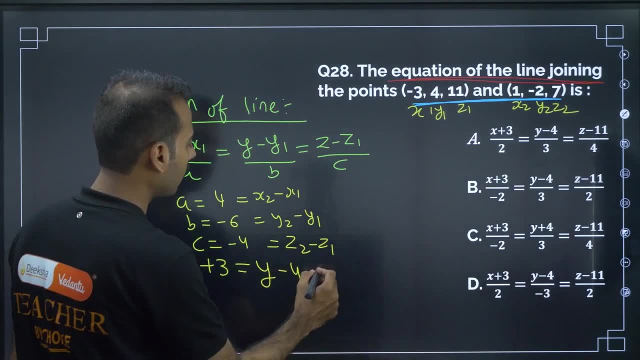 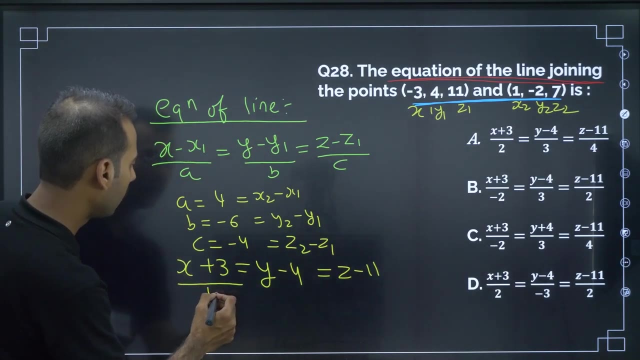 minus 4. a, b, c. we got. now you take x minus x, 1, x plus 3, y minus 4, y minus 4 is equal to z minus 11 by z minus 7. by x 2 minus x 1 is 4 minus 6 minus 4. so is there any such option: x plus 3, y minus 4. 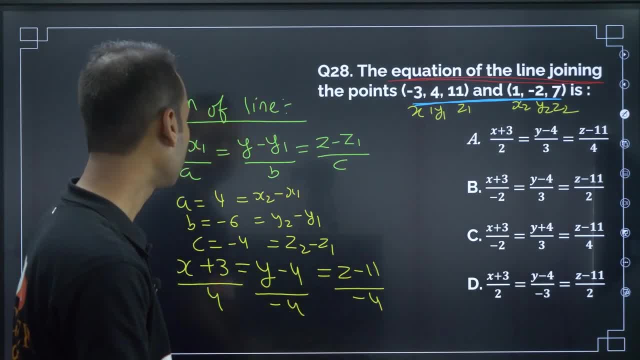 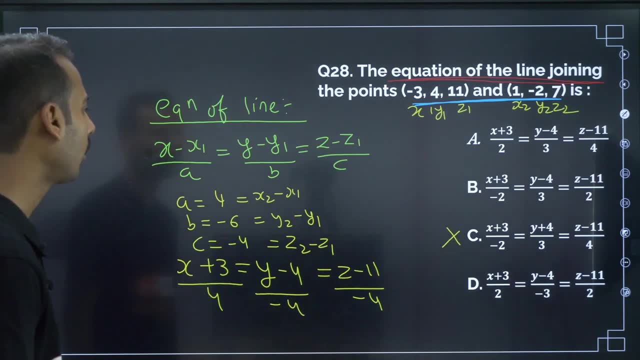 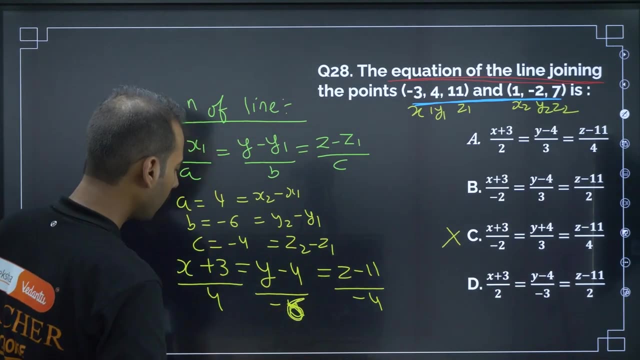 z minus 11, z minus 11, so plus 4 and has been eliminated. plus 3 minus 4, z minus 11.. Now among these, 3, b is minus 6, b is minus 6.. If I take 2 common from all this, this can be written as 2 minus 3 minus 2.. 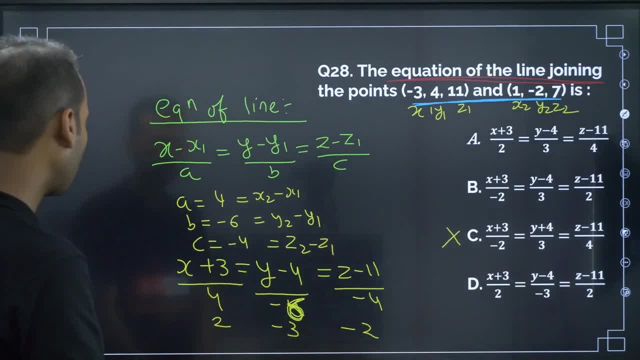 Is there any such option like this: 2, 3, 2 minus 3 minus 2, we are having 2 minus 3.. So 2, 3, 4. that means this is also eliminated. we are left with 2 minus 2, 3, 2.. So they both. 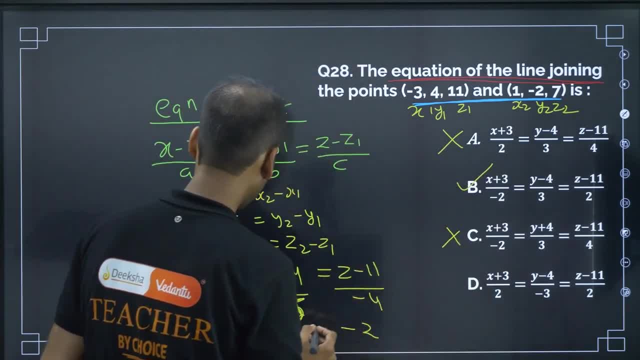 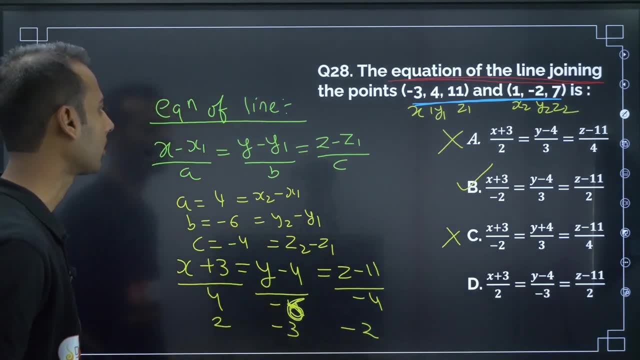 are having same sign. So this will be the answer, because if I cancel off, this will indicate direction ratios. we need to have a lot of practice to understand this problem in the sense, a lot of practice in the sense with a taking of equations, how to take. 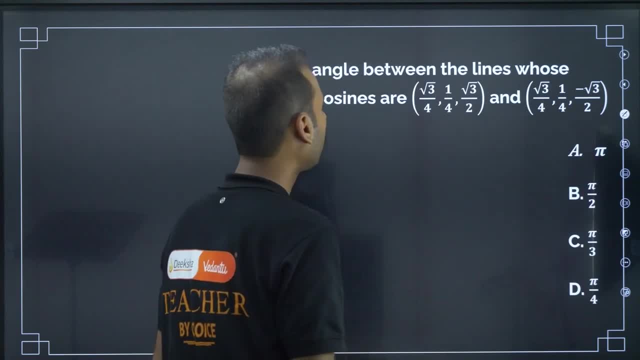 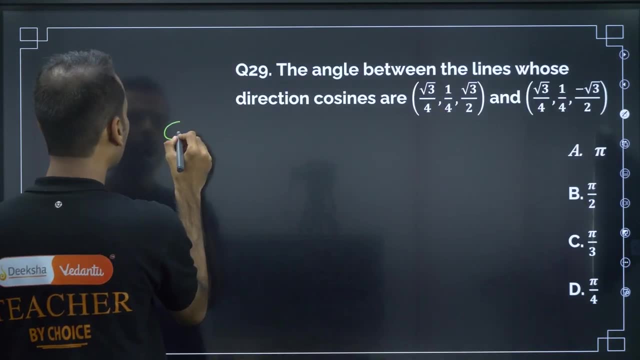 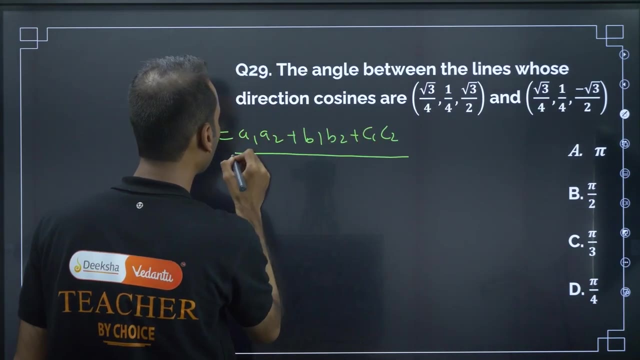 So b is the answer. next, move on to next question: the angle between the lines whose direction cosines are. This is direct question question. So cos theta is equal to once, let me write a: 1 a, 2, b, 1, b, 2, c, 1, c, 2 by root of a: 1 square. 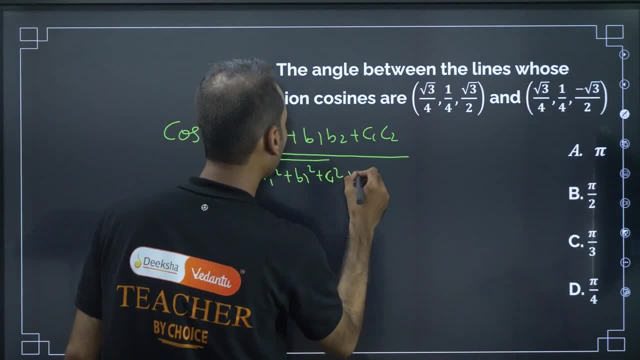 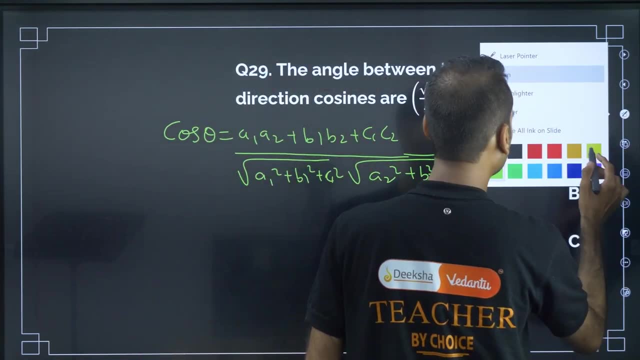 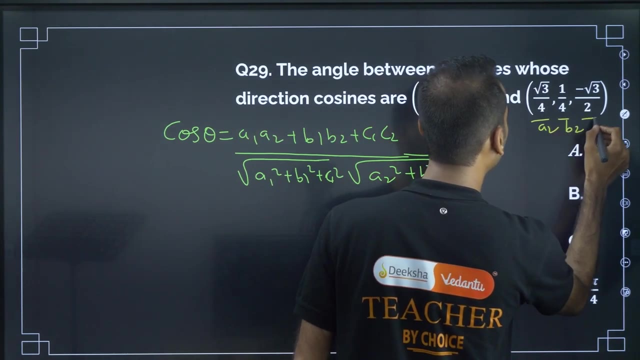 b 1 square, c 1 square, root of a 2 square. b 2 square, c 2 square. what are the direction cosines? So a 1 b 1 c 1. a 2, b 2, c 2 to b 2 c 2. the angle between the lines, the angle between: 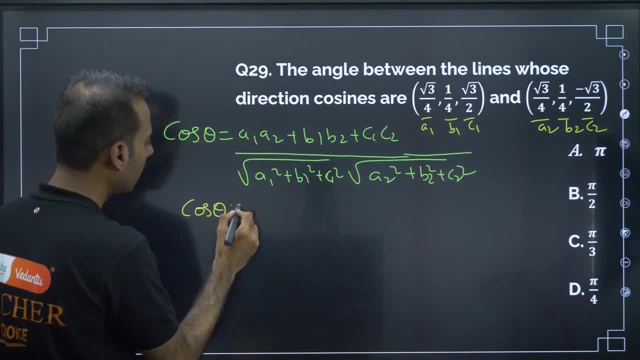 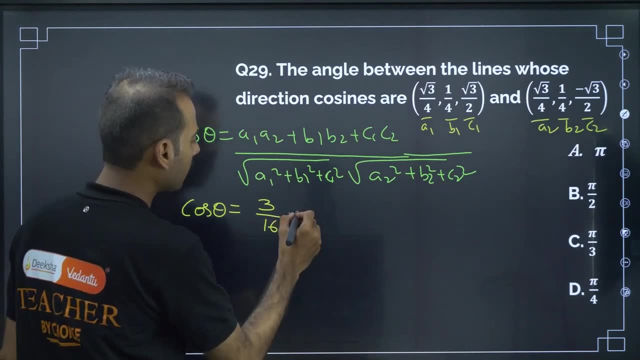 whose direction cosines are, So cos theta is equal to, I have to multiply this root 3 by 4, root 3 by 4, 3 by 16 b, 1 b, 2, 1 by 16, 1 by 16 c, 1 c, 2 minus 3 by 4 by root of. 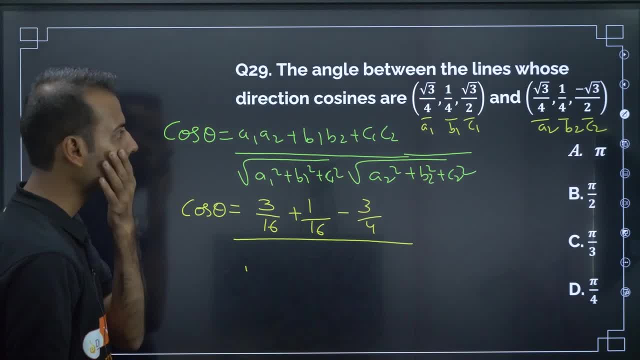 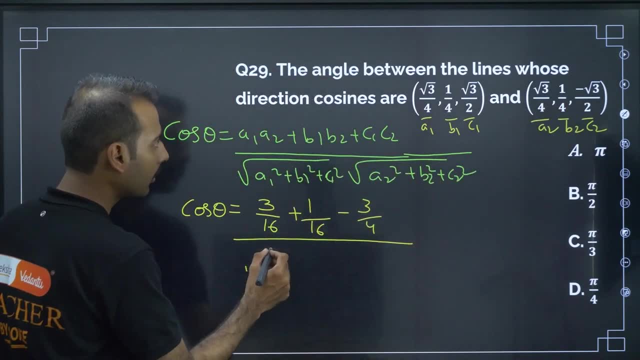 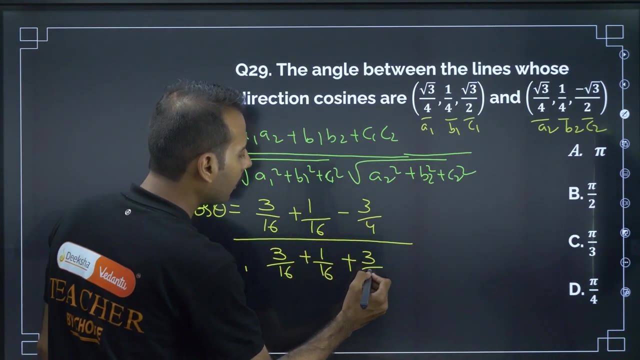 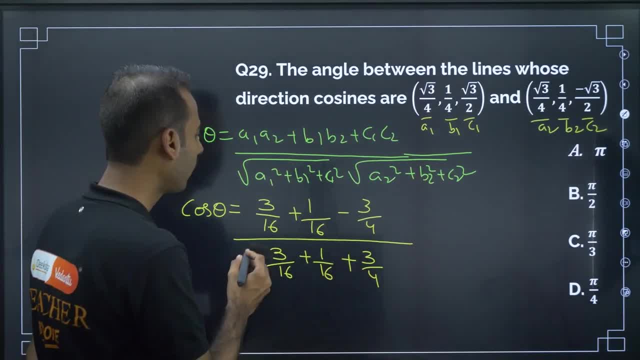 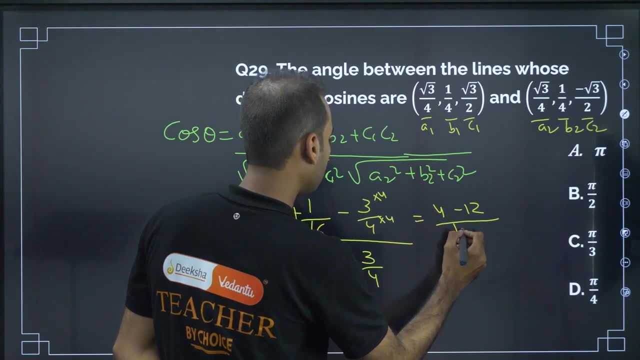 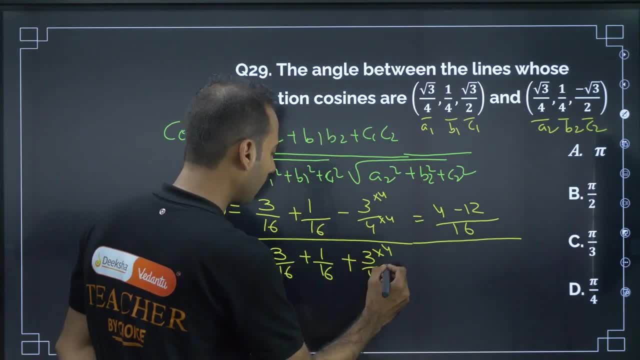 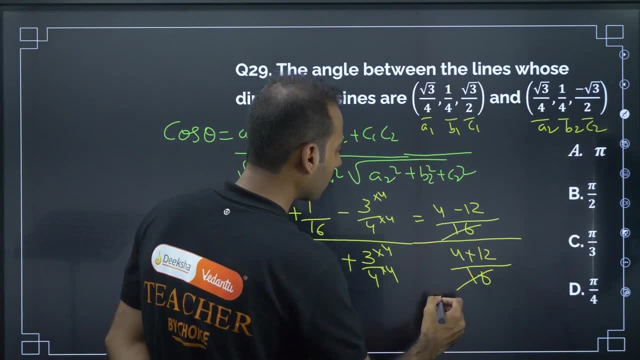 4 minus 12 by 16, divided by: if I multiply 4,. if I multiply 4, 3 plus 1 is 4, 4 plus 12 by 16,. 16 and 16 will get cancelled. here we are left with minus 8 by 4 plus 12 is minus. 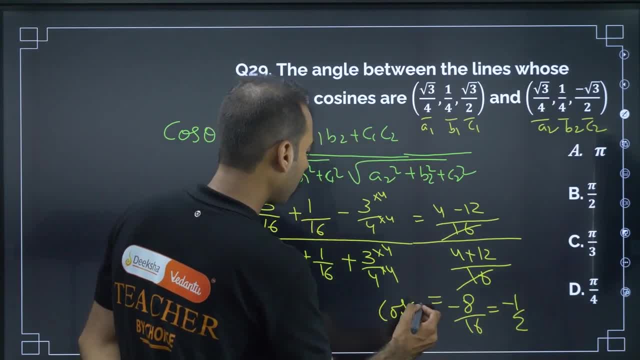 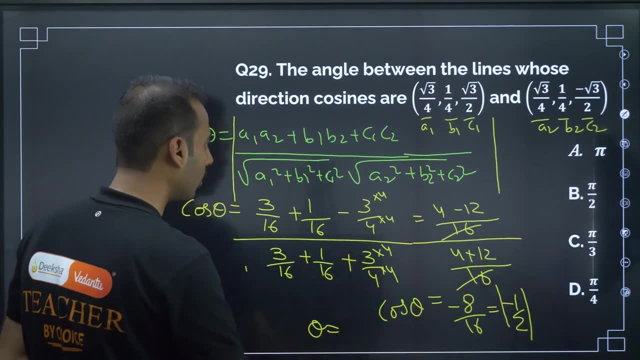 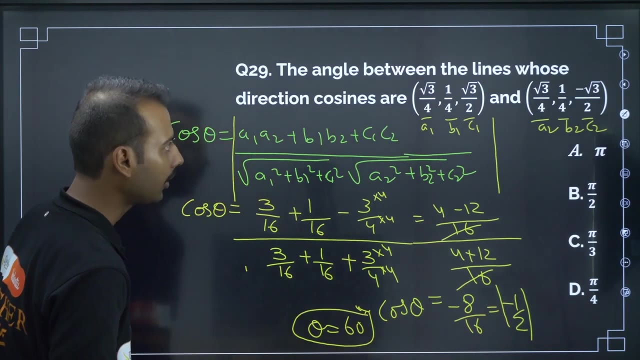 1 by 2.. So cos theta is minus 1 by 2, in fact synopsis, if you try to recall this, will be like this: which implies theta is equal to pi by theta is equal to 60 degrees. 60 degrees means pi by 3, c is the answer. Moving on to next question, if a plane meets, 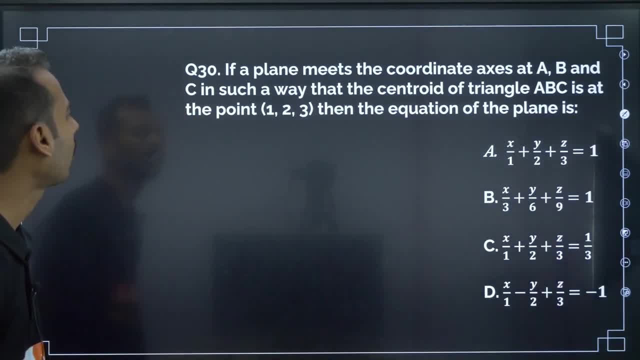 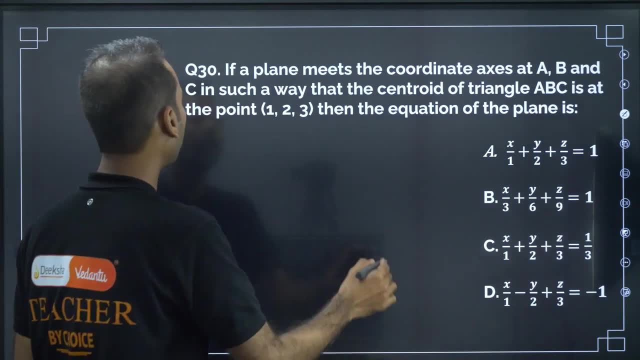 the coordinate axis at a, b, c in such a way that centroid of triangle is at the point. then the equation of plane is. so what are they asking If a plane meets the coordinate axis? equation of plane. they are talking about equation of plane. also some data they have. 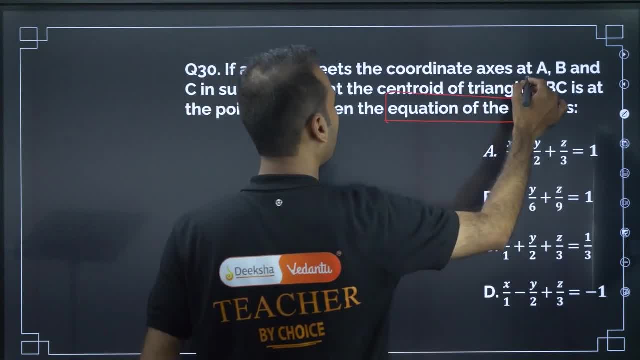 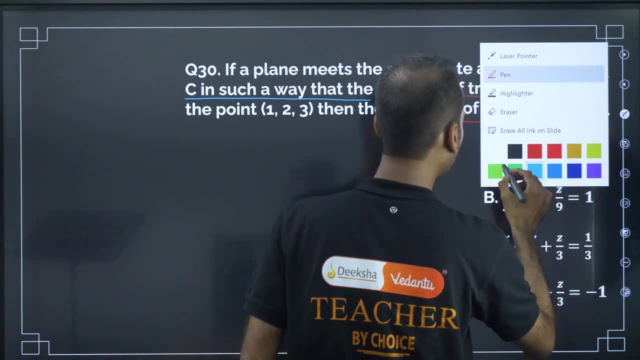 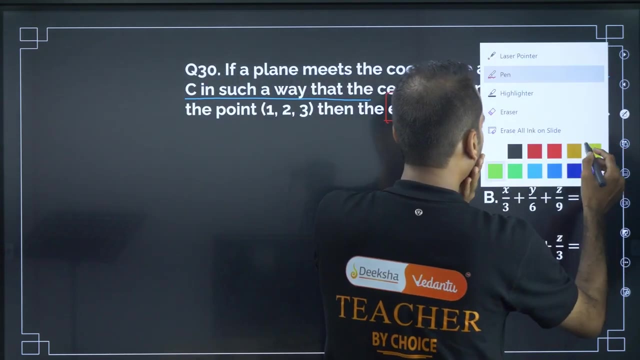 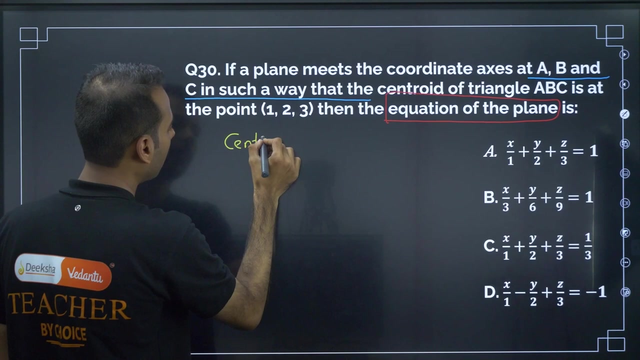 given if a plane meets the coordinate axis at a, b and c. So if a plane meets the coordinate C in such a way that centroid of the triangle is at the point now, centroid of the triangle is at the point 1,, 2, 3.. So centroid- they have given centroid- is at 1,, 2, 3 generally. 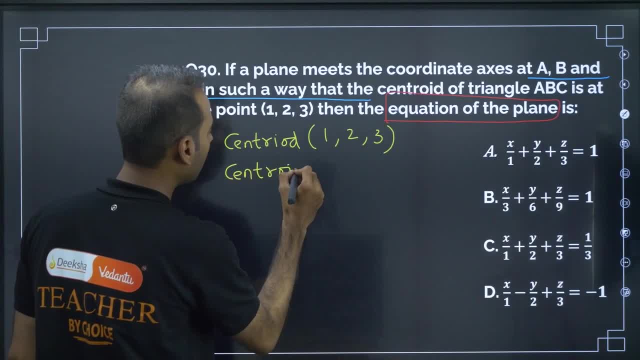 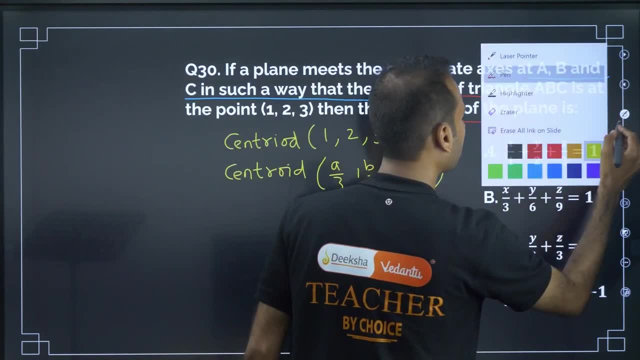 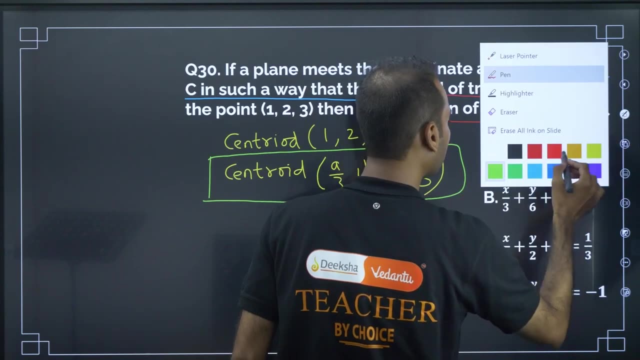 centroid is given by. centroid is given by a by 3, b by 3, c by 3. this you take as synopsis point. take this: centroid is given by a by 3, b by 3, c by 3.. Now, from this, from this: 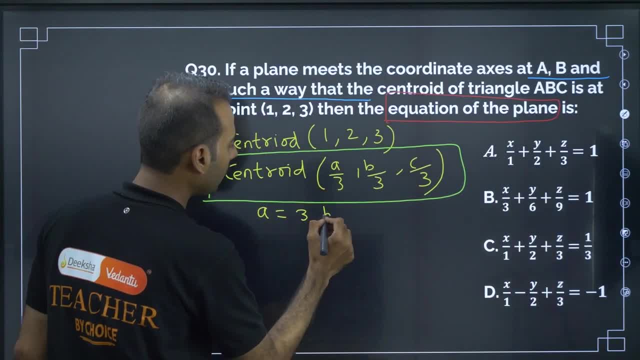 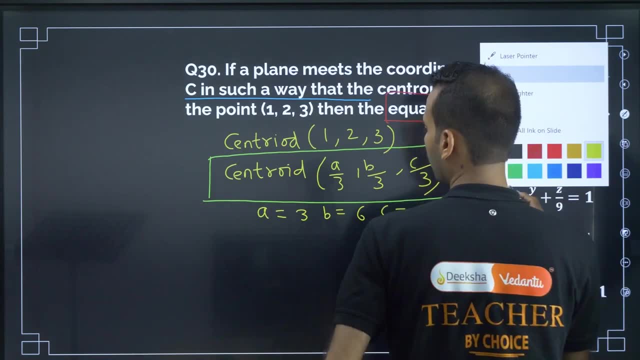 you calculate a: a is equal to 3, b is equal to 6, c is equal to 9, c is equal to 3, 3 is a, 9, a is equal to b is equal to c is equal to this one. 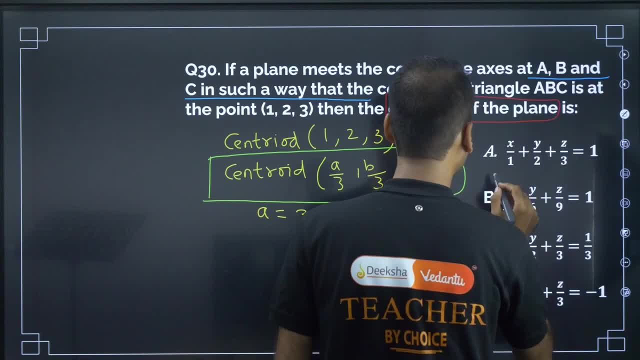 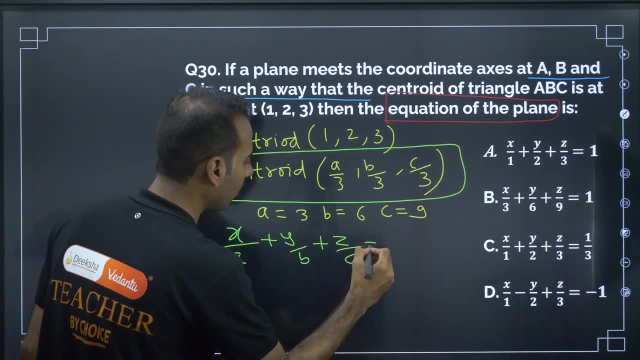 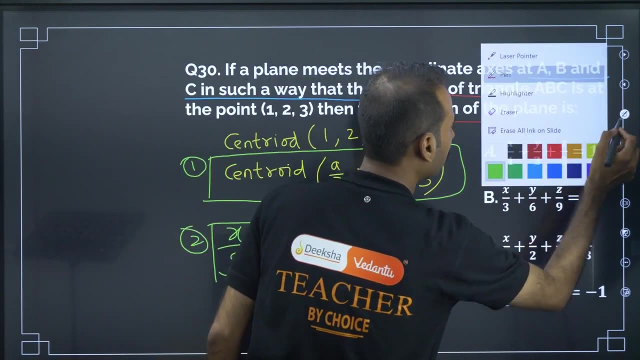 Now, what are they asking? they are asking to find centroid. Now, equation of plane. equation of plane is given by x by a plus y, by b plus z, by c equal to 1.. This is one more synopsis point. this is first synopsis point. this is second synopsis for this question. So so, 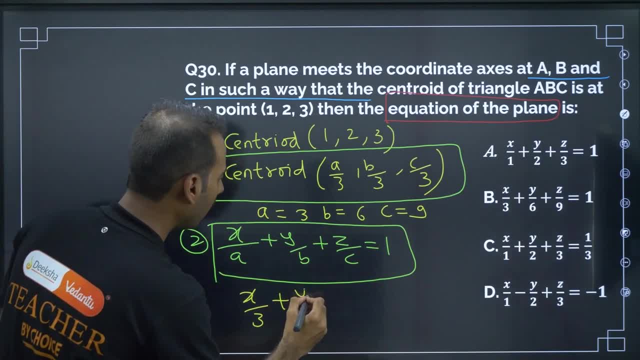 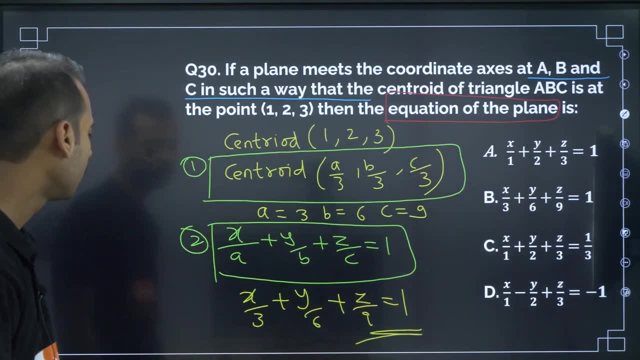 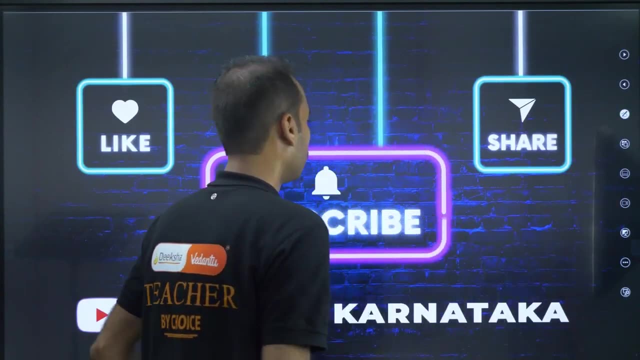 if I find x by 3,, y by 6, z by c, z by 9 is equal to 1.. Is there any such option? 3, 6, 9.. a is the answer. sorry, b is the answer. moving on to next question. Thank you very much. if 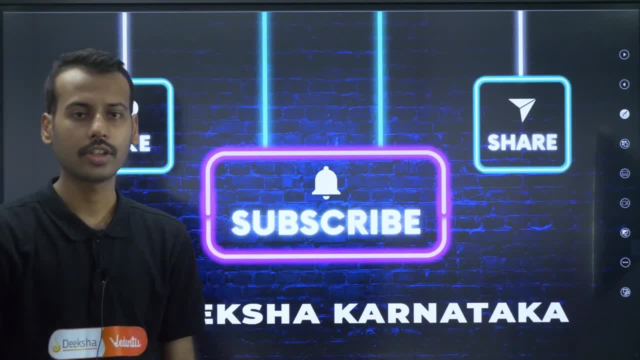 you find this video interesting, like, subscribe and share. remaining things we will discuss in the next video.